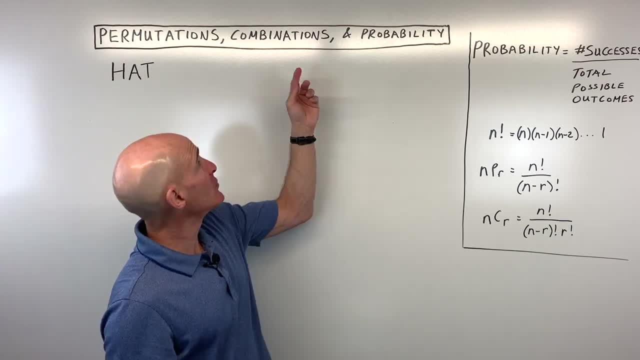 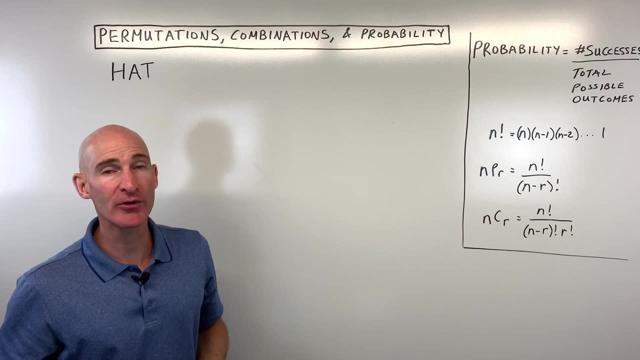 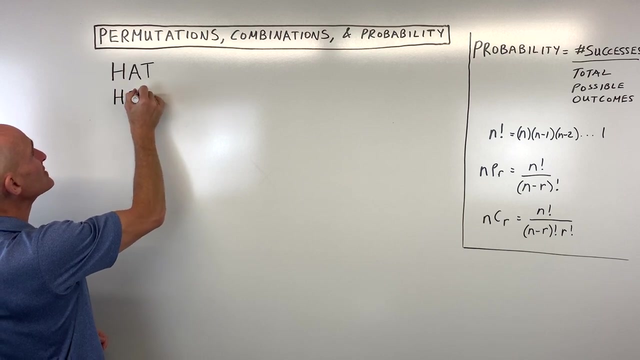 in the word hat. Now, when you think of the word permutations, permutations refers to like an ordering. So like, how many different ways can we order those letters, all three of those letters? Now, let's just go ahead and do it by hand here so we can see h a t. we could also write it as h t a. 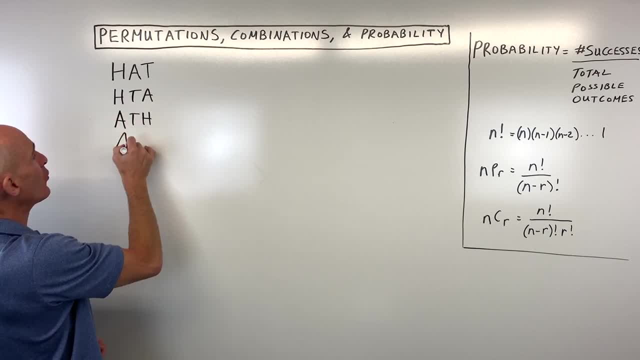 We could do a t h or a h t or what else- t a h or t h a, and those are the only possibilities. So sometimes this is referred to as a sample space Basically showing you like all the possible outcomes. but these are the permutations, the orderings. Another way to do this: you can do a tree diagram. You could say like: 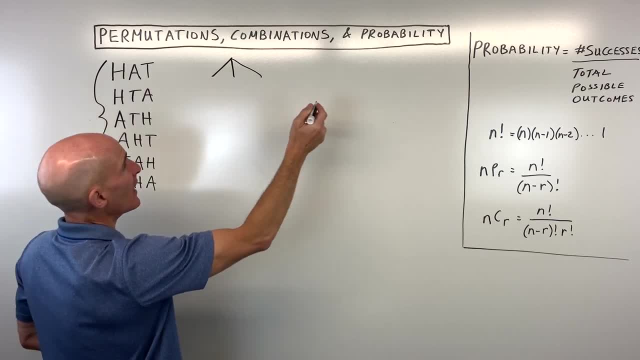 when I imagine, if I put these three letters into like a hat- Okay, like this, here's our three letters. We can say like this: I'm going to put these three letters into like a hat, Okay, like this, here's our three letters. 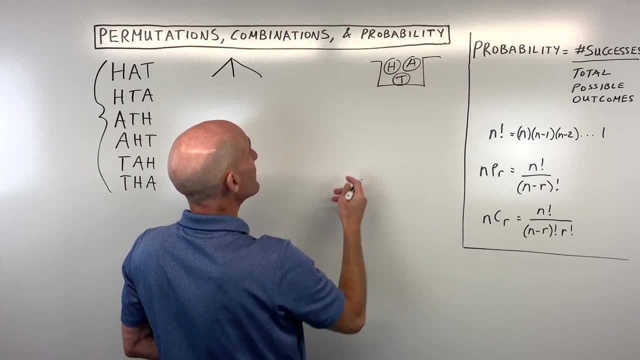 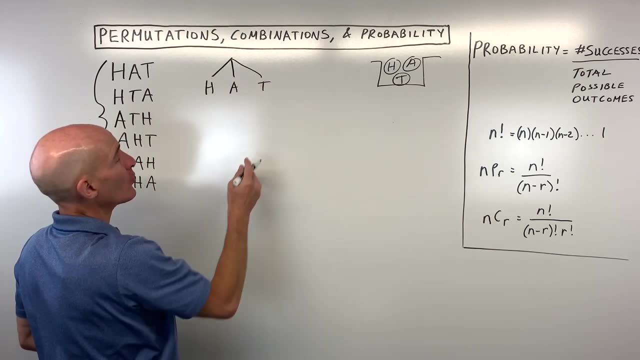 on sheets of paper, let's just say H, A and T, and what we're doing is we're going to reach into that hat and we're going to pick out a letter. So for the first letter, we could pick an H, an A or a T. 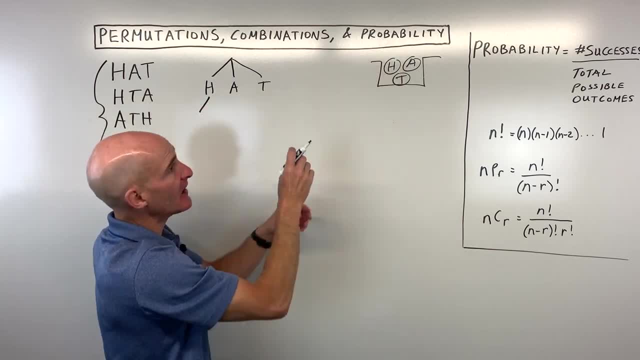 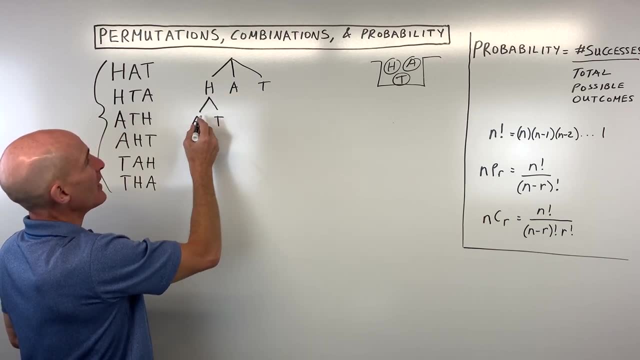 right, But if we pick an H and we set it aside when we go to pick the next letter, what can we do? Well, we could either pick an A or a T, okay, and then if we pick, let's say, an H and an A, there's. 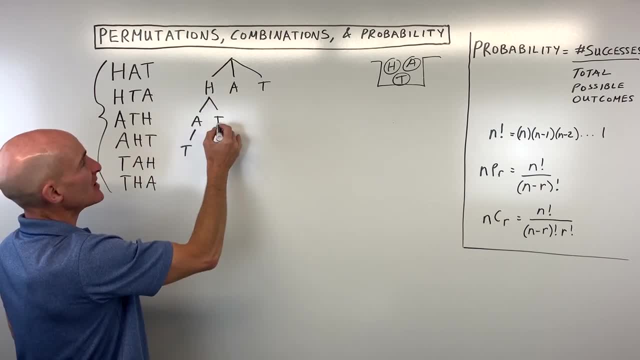 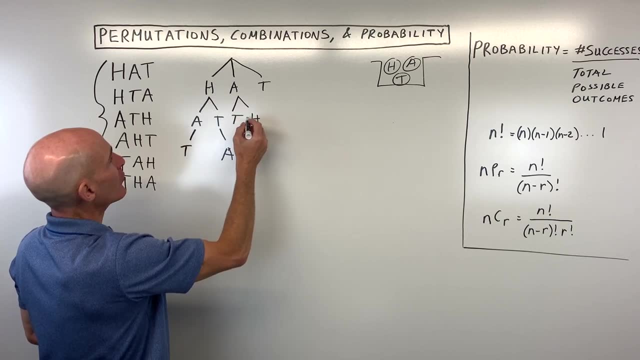 only a T left, right, Whereas if we pick an H, a T, then there's only going to be an A left and same thing over here. we could do A T or H, or if we do A T, then this would be like an H. 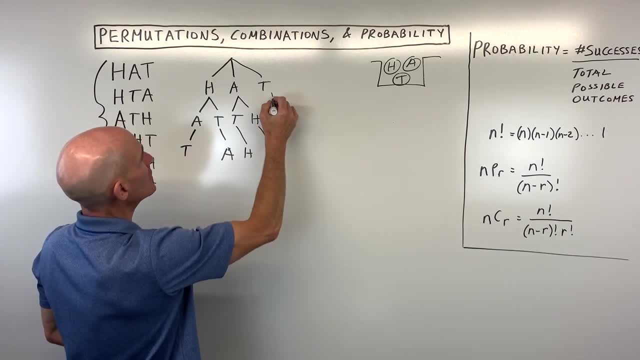 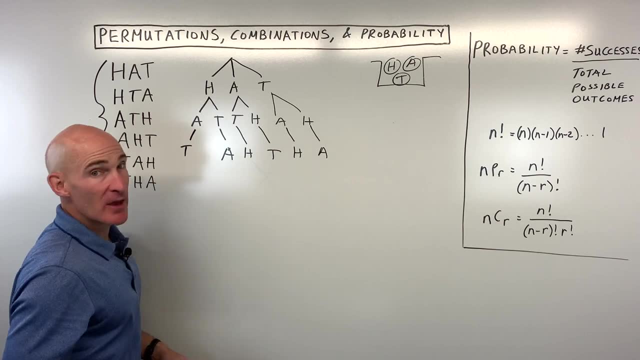 and this would be like a T. or we could do A or H and then this could be an H or an A, And so basically, if you kind of think of this as like a root, you could either go down this root- H A T. 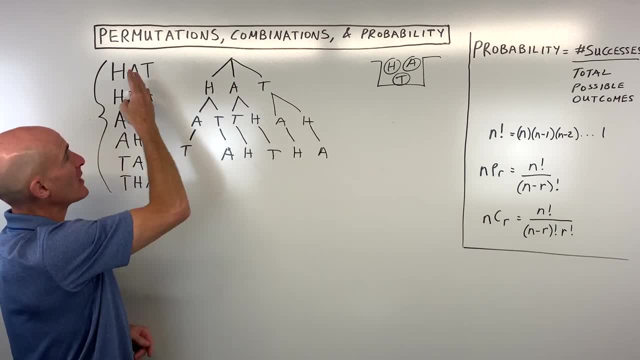 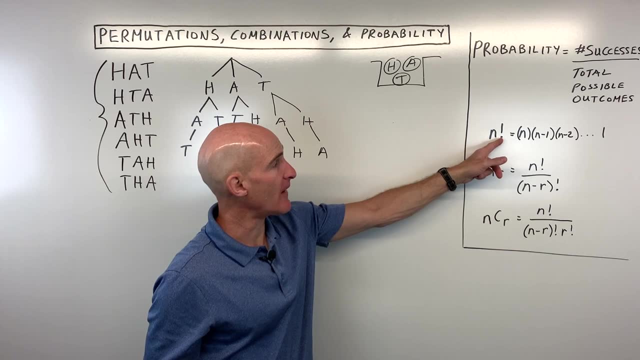 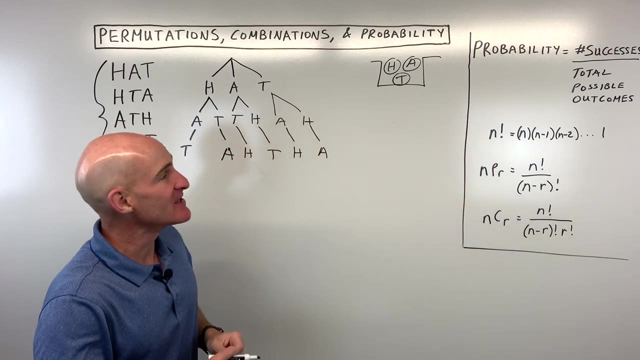 or H T A or A T H, and that's another way of getting these permutations or possible permutations. Another option is to use what we call a factorial- See that exclamation point there. That doesn't mean like, uh, yay, right, It means you take the number and you multiply down to one. 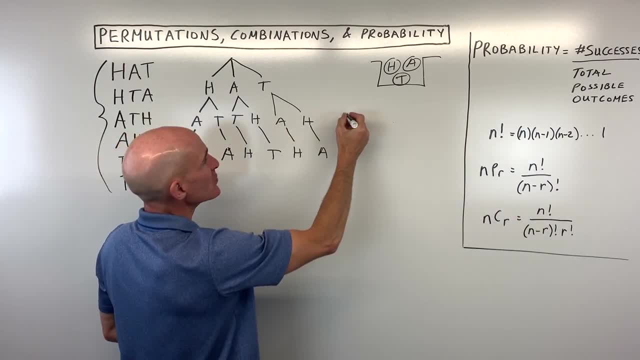 So, for example, in this case we had three letters: H, A and T. so we'd say, well, there's three possibilities for what we can pick out for that first letter. Once we pick out that first letter, we're going to have three possibilities for what we can pick out for that first letter. 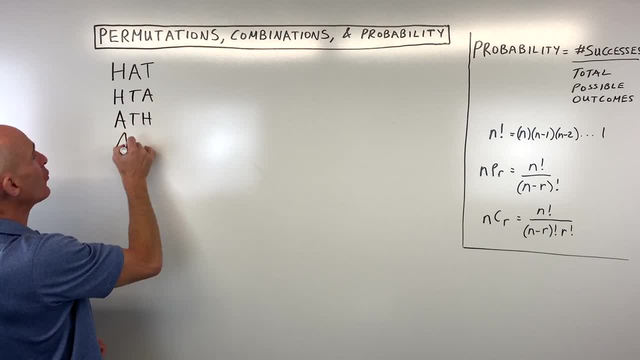 We could do a t h or a h t or what else- t a h or t h a- and those are the only possibilities. So sometimes this is referred to as a sample space basically showing you, like, all the possible outcomes. but these are the permutations, the orderings, Another way to do. 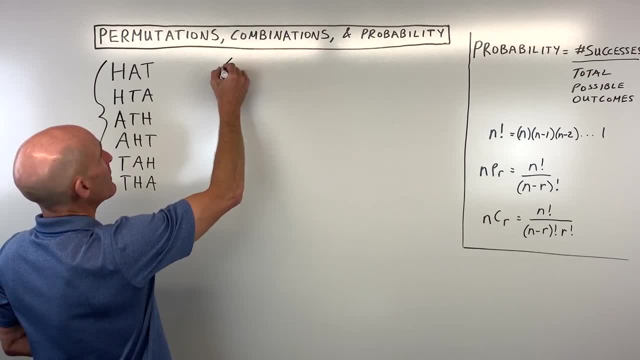 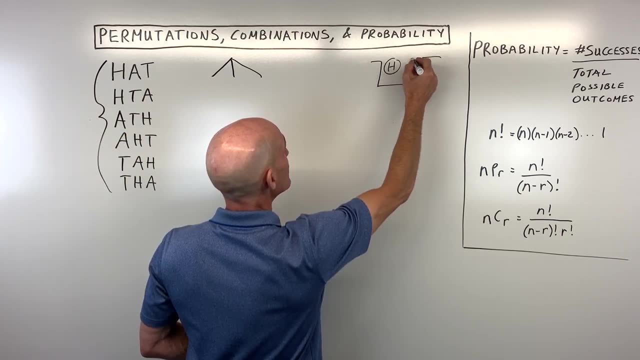 this. you can do a tree diagram. You could say like when I imagine if I put these three letters into like a hat, okay, like this, Here's our three letters on sheets of paper. let's just say H, A and T, and what we're doing is we're going to reach into that. 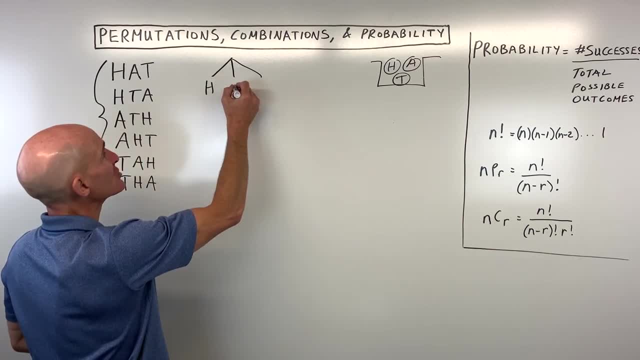 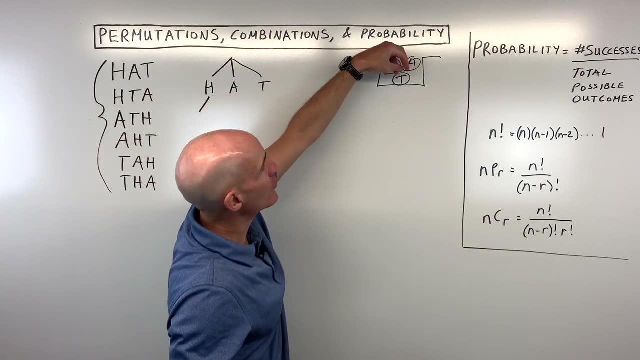 hat and we're going to pick out a letter. So for the first letter we could pick an H, an A or a T, right? But if we pick an H and we set it aside when we go to pick the next letter, what can we do? 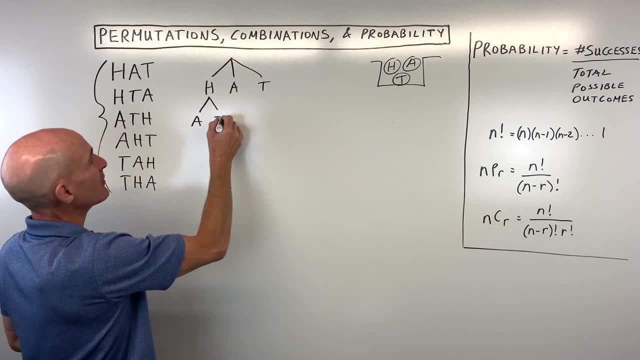 Well, we could either pick an A or a T, okay, and then if we pick, let's say, an H and an A, there's only a T left, right, Whereas if we pick an H, a T, then there's only going to be an A left. 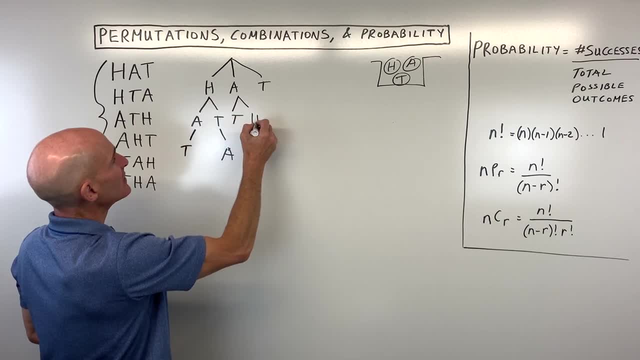 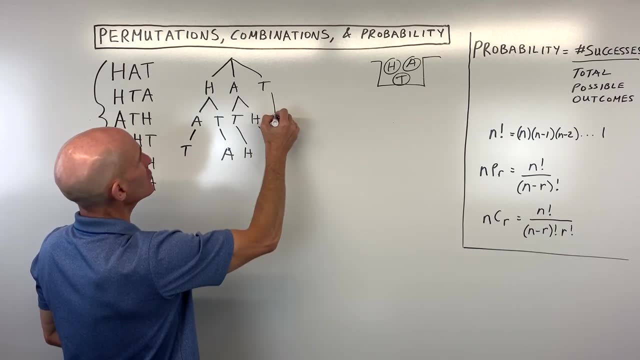 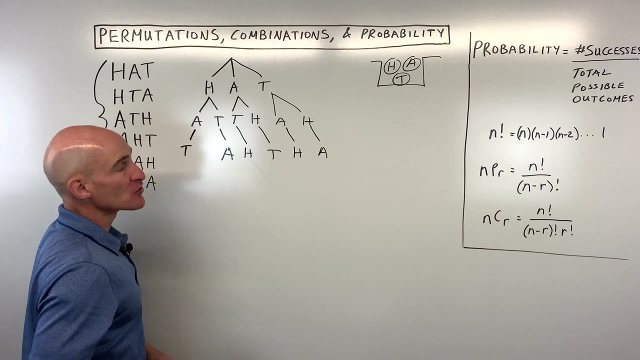 and same thing over here. we could do A T or H, or if we do A T, then this would be like an H and this would be like a T, or we could do A or H, and then this could be an H or an A, And so. 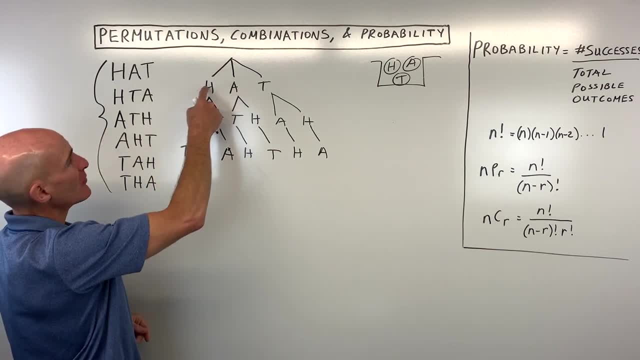 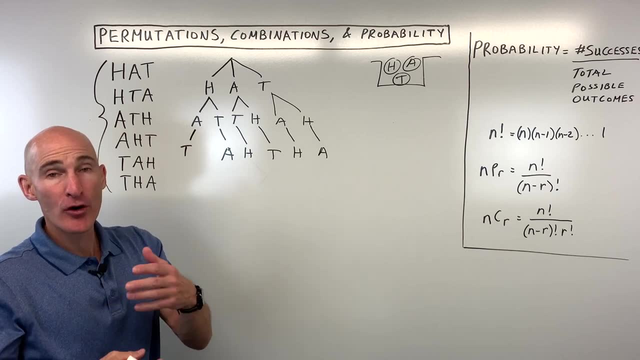 basically, if you kind of think of this as like a root, you could either go down this root- H A T or H T A or A T H, and that's another way of getting these permutations or possible permutations. 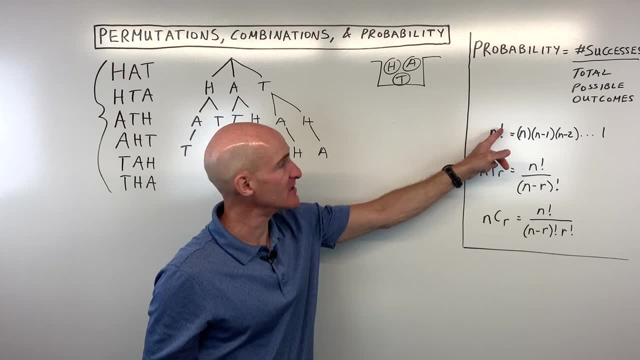 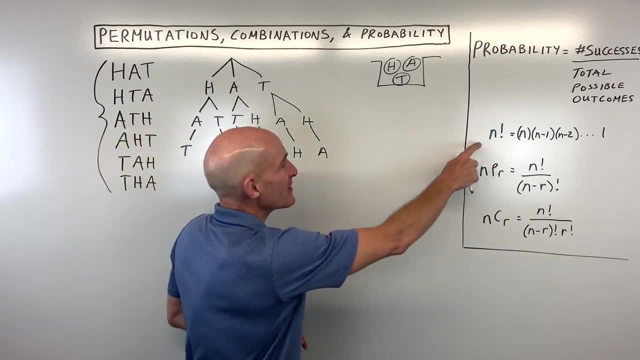 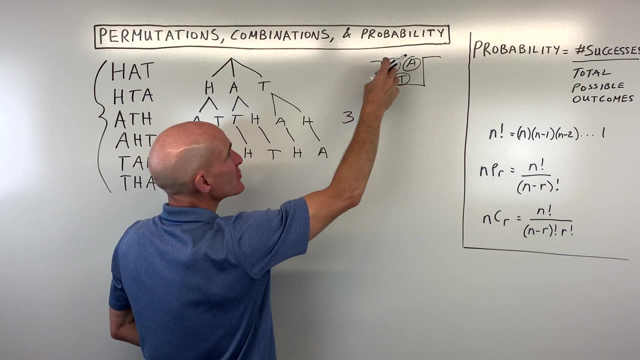 Another option is to use what we call a factorial- See that exclamation point there. That doesn't mean like, uh, yay, right, It means you take the number and you multiply down to one. So, for example, in this case we had three letters: H, A and T. so we'd say, well, there's three. 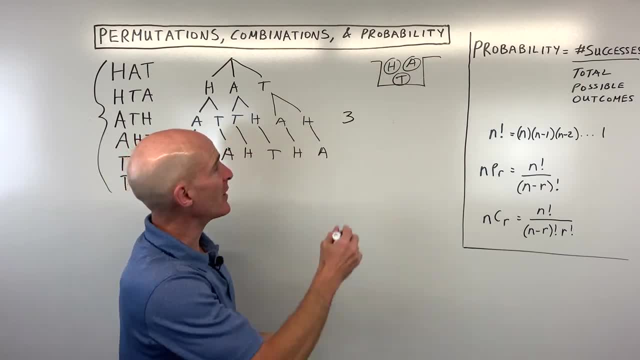 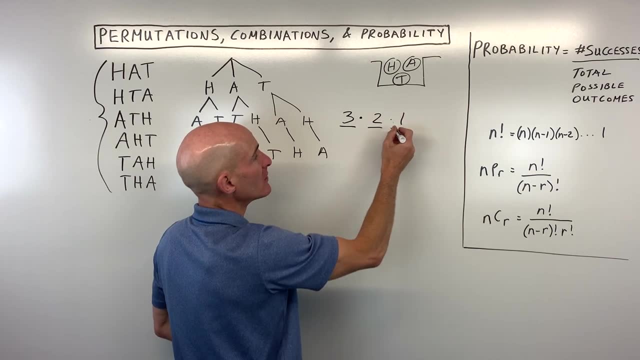 possibilities for what we can pick out for that first letter. Once we pick out that first letter, we're going to have three possibilities for what we can pick out for that first letter. There's two choices for the second letter that we pick out and then, lastly, there's only one letter. 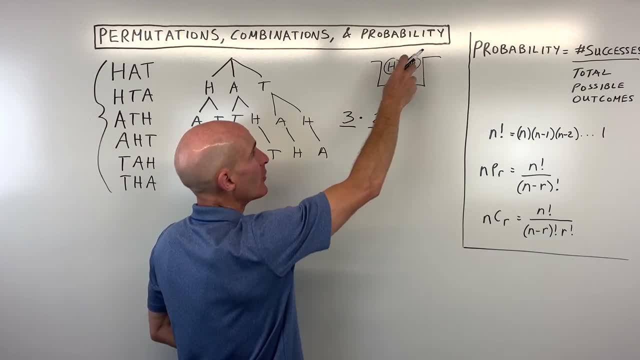 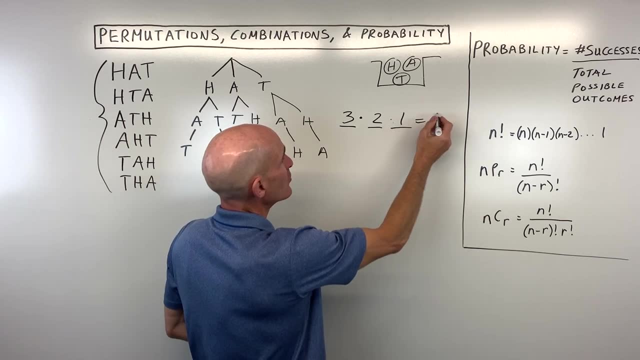 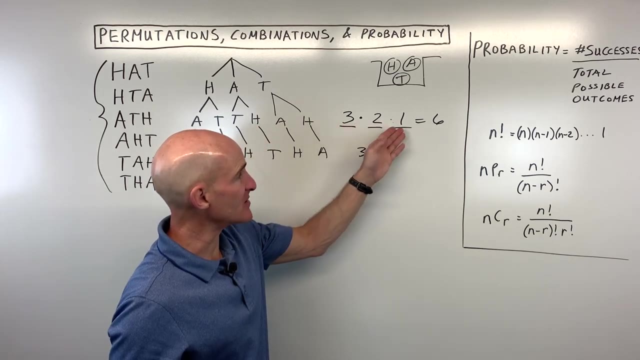 There's two choices for the second letter that we pick out, and then, lastly, there's only one letter for the final choice, and so this is really three times two times one, which is six, or you can write this in a more condensed fashion: three factorial, and that represents three times two times one. 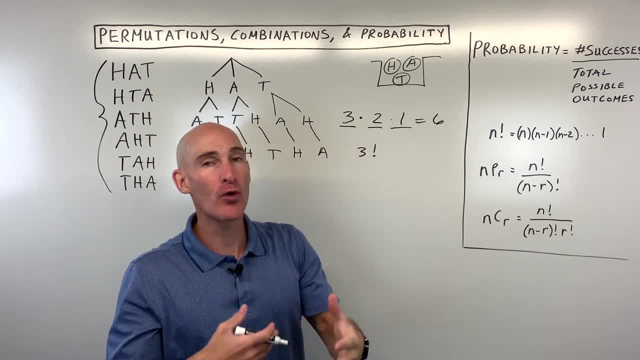 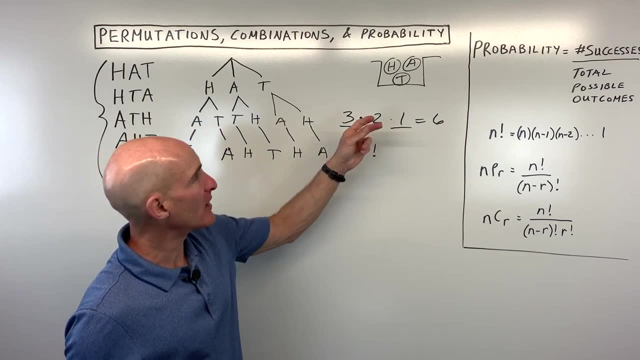 So n factorial is when you're trying to see how many different orderings there are of all n items. Now, sometimes what happens is you only want to maybe pick two of the items or one of the items, okay, or like that. So in that case you would use. 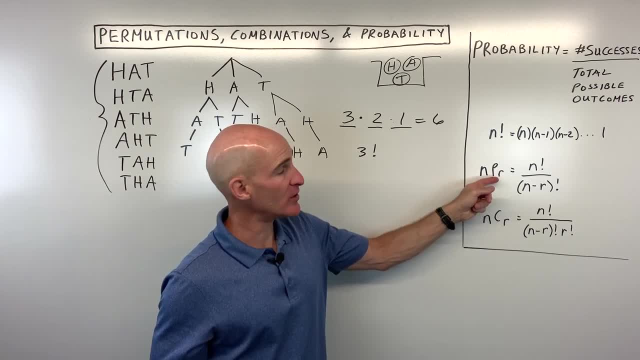 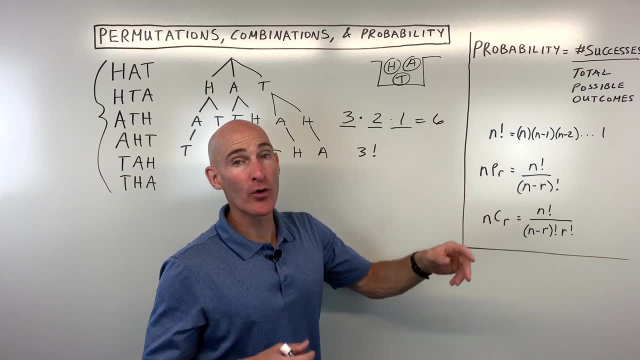 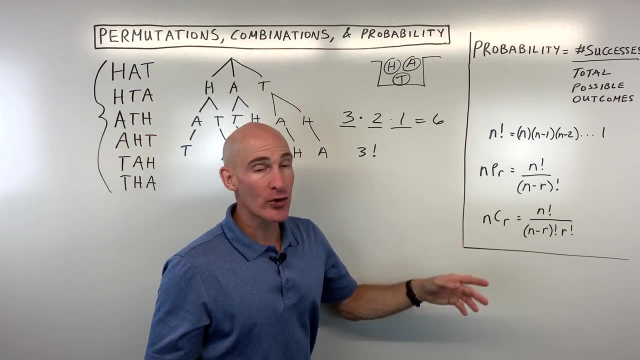 this concept here of NPR. What does that mean? It means out of n items. how many ways are there of picking r of those items where the order is important? We're also going to talk about combinations- okay, combinations, and this is when the order is not important. 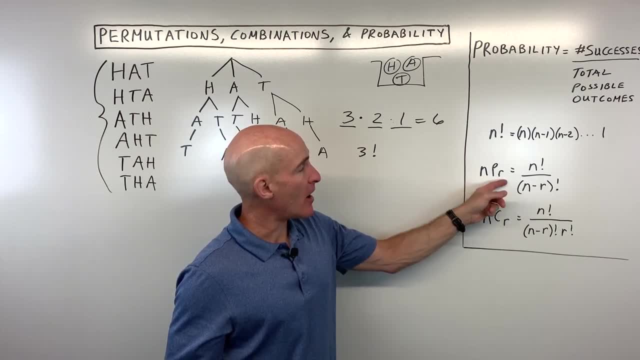 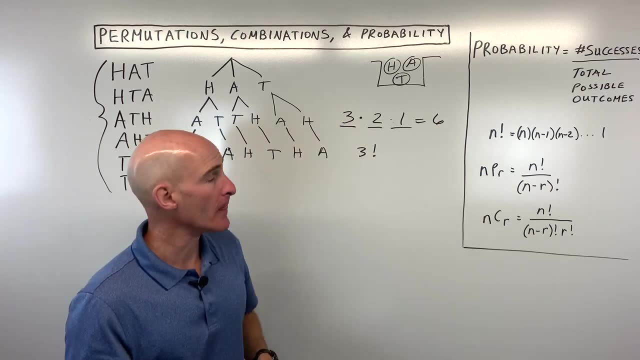 But let's talk about the permutations first. So, NPR, let's say, for example, out of the three letters here, how many ways are there to pick just two of the letters where the order is important? Well, let's try to write it out again. So what we could do is we could say: well, there could be. 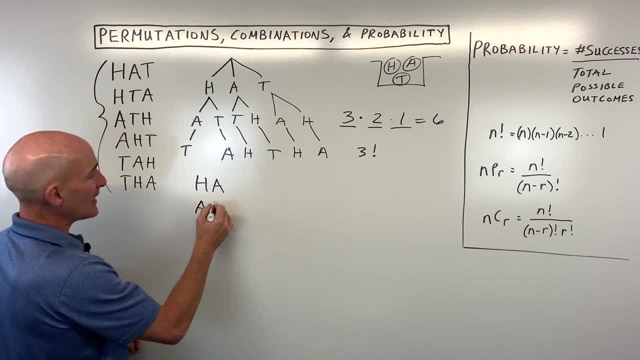 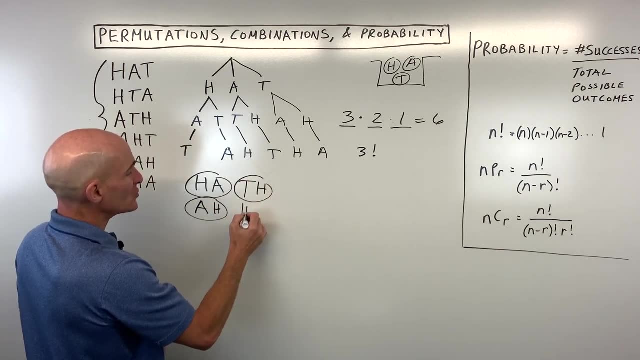 H and A, or there could be A and H, or so that's one possibility. Another possibility: we could do T and H, or we could do H and T, and we could do A and T or T and A, And so you can see here that this is. 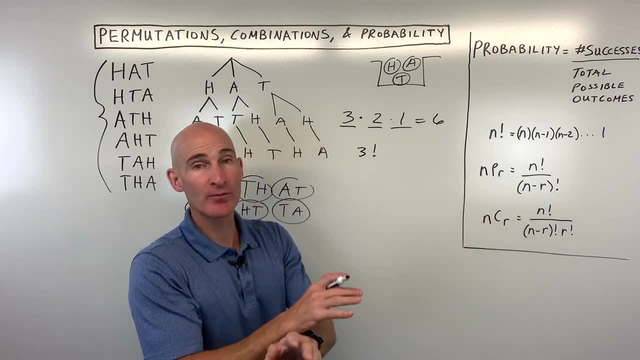 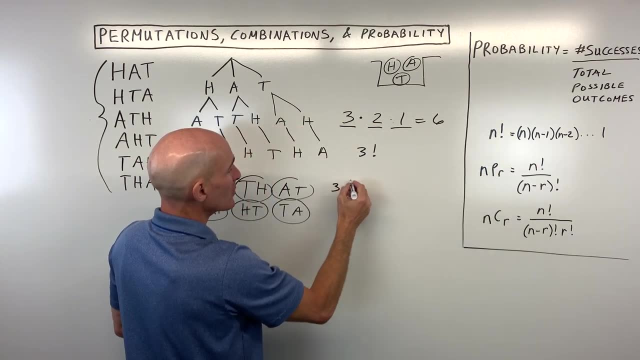 the possibility is of choosing two letters out of three, where the order is important. Now we can use this formula. This is another way to do it. You could say N factorial. so that's going to be so. we're doing 3P2 out of three items We're picking. 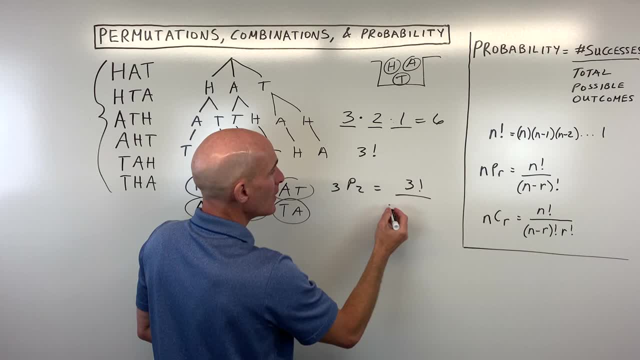 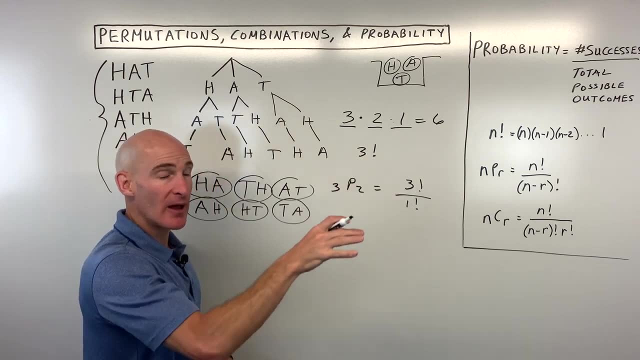 two where the order is important. So that's going to be 3 factorial over 3, minus 2, which is 1 factorial. Now remember we already talked about how factorials you multiply down to one. So this is going to be 3 times 2 times 1, which is 6, all over 1 factorial, which is just 1.. 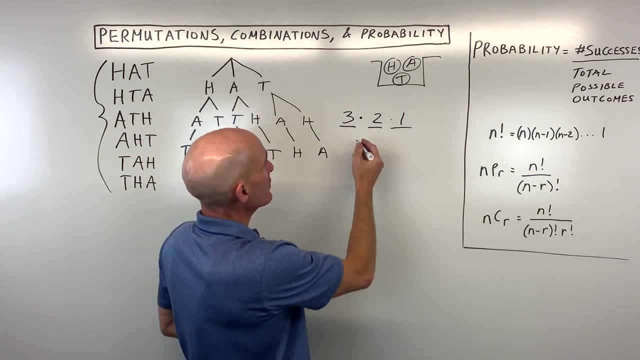 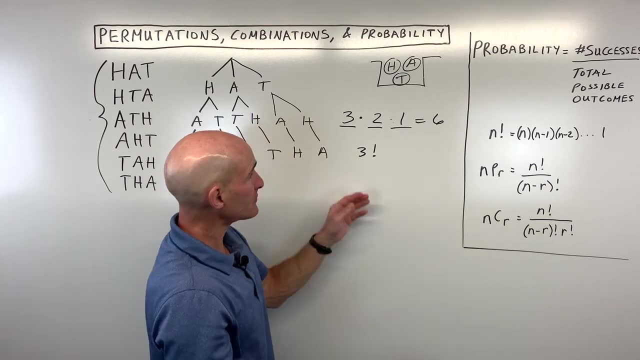 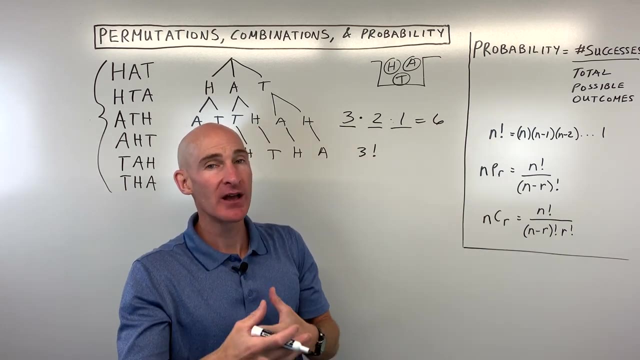 for the final choice, and so this is really three times two times one, which is six, or you can write this in a more condensed fashion: three factorial, and that represents three times two times one. So n factorial is when you're trying to see how many different orderings there are of all n items. 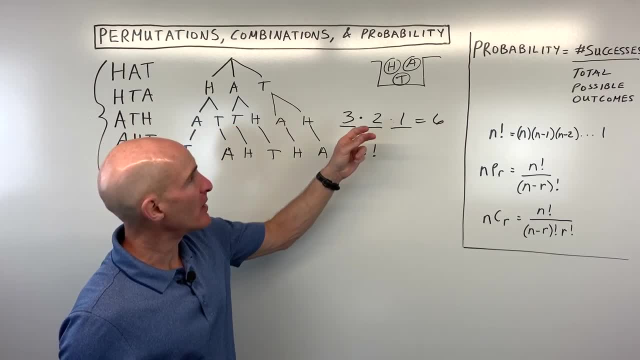 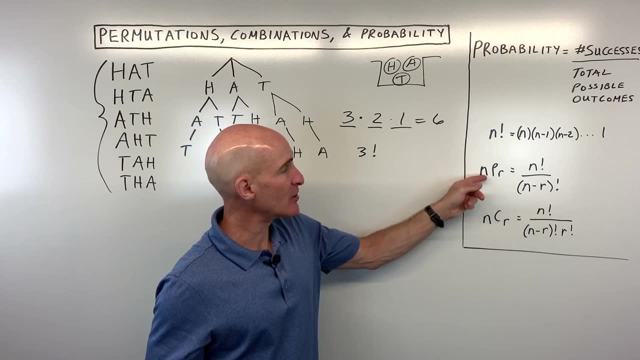 Now, sometimes what happens is you only want to maybe pick two of the items or one of the items, okay, or like that. So in that case you would use this concept here of NPR. What does that mean? It means out of n items. how many ways are there of? 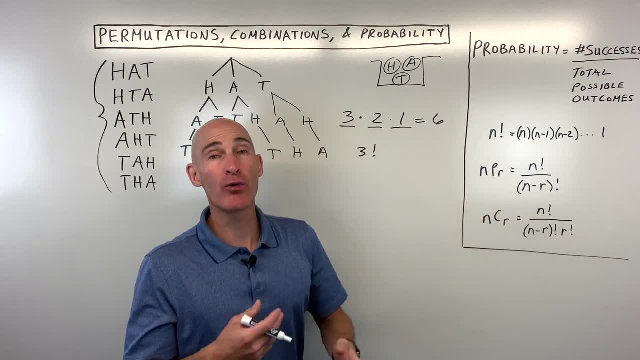 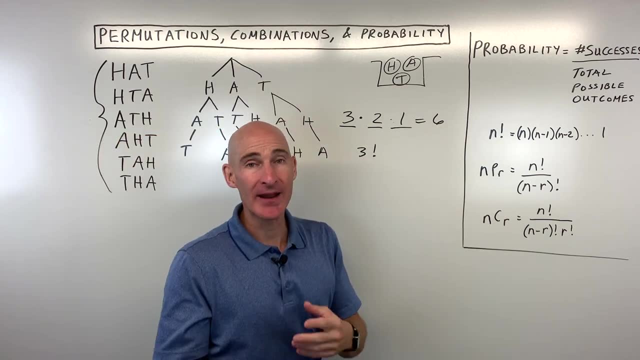 picking r of those items where the order is important. We're also going to talk about combinations, okay, combinations, and this is when the order is not important. But let's talk about the permutations first. So NPR, let's say, for example, out of the three letters here: 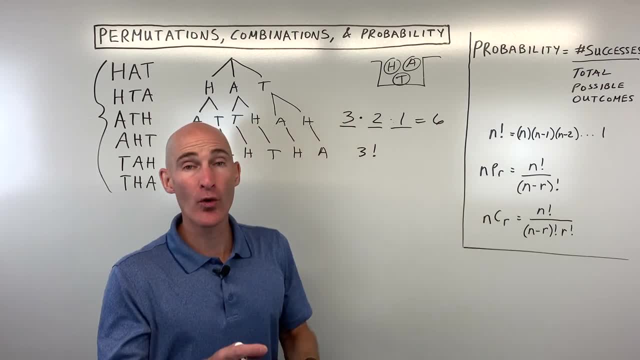 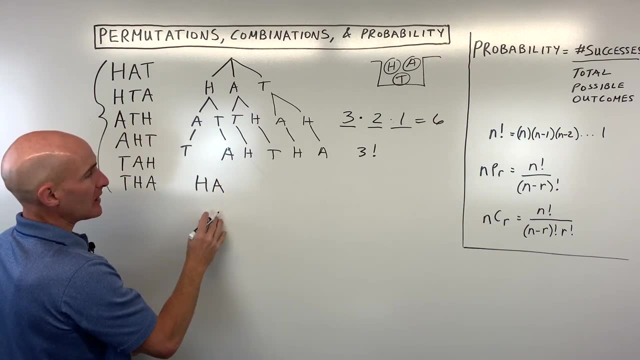 how many ways are there to pick just two of the letters where the order is important? Well, let's try to write it out again. So what we could do is we could say: well, there could be H and A, or there could be A and H, or so that's one possibility, Another possibility we could do. 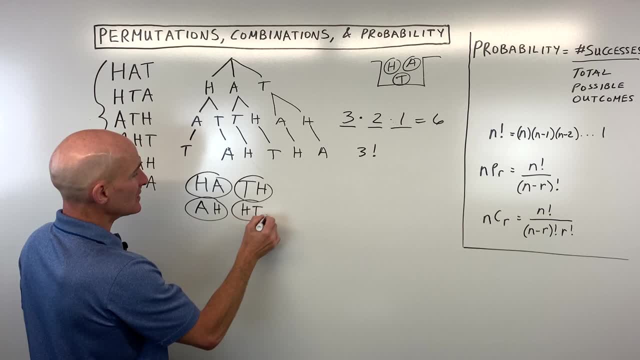 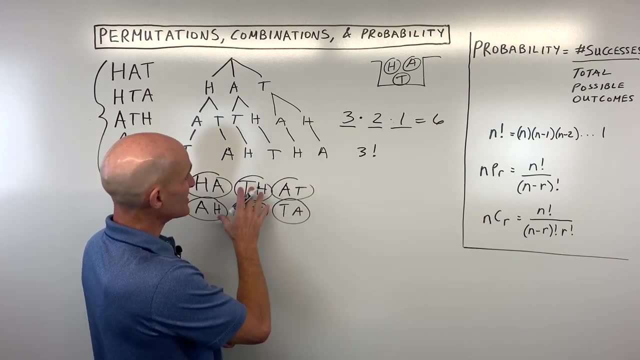 T and H, or we could do H and T and we could do A and T or T and A, And so you can see here that this is. the possibility is of choosing two letters out of three, where the order is important. 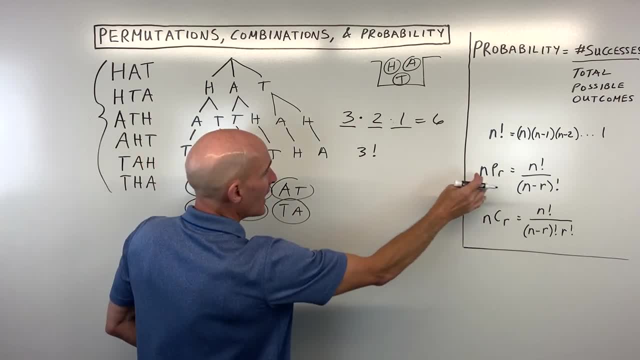 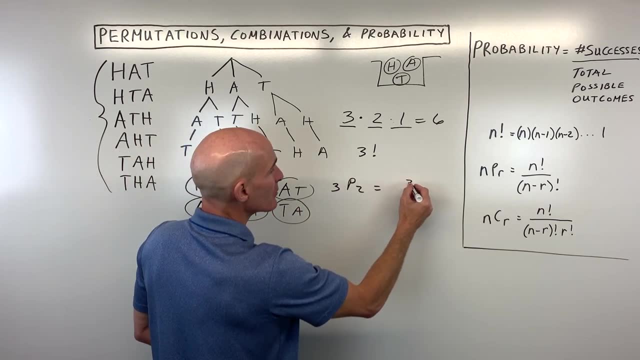 Now we can use this formula. This is another way to do it. You could say N factorial, so that's going to be. so we're doing 3P2 out of three items, We're picking two where the order is important, So that's going to be 3 factorial over 3 minus 2,. 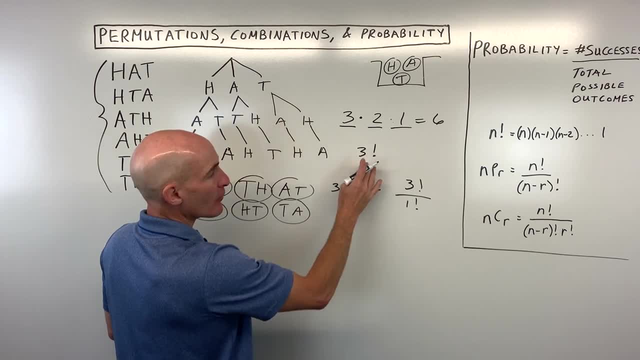 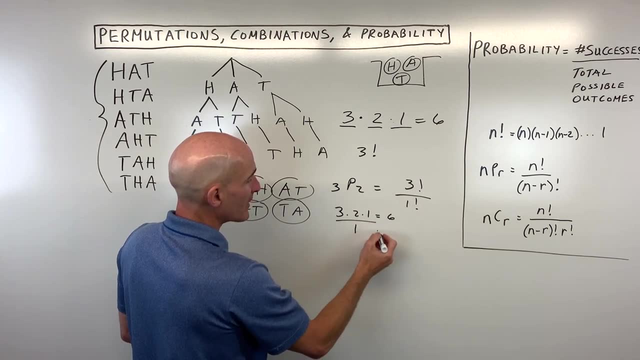 which is 1 factorial. Now remember we already talked about how factorials you multiply down to one. So this is going to be 3 times 2 times 1,, which is 6,, all over 1 factorial, which is just 1.. 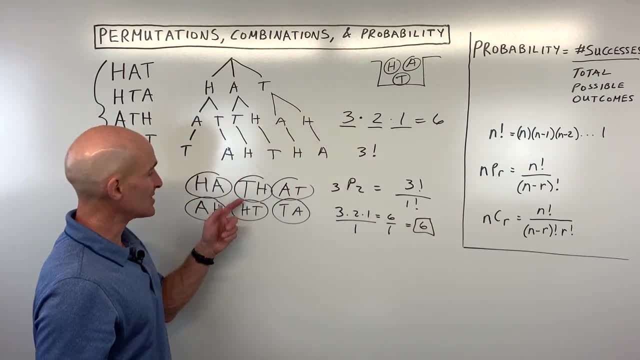 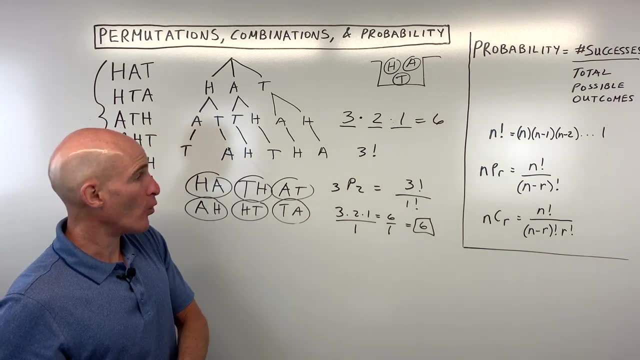 So you can see there's six different possibilities and these are the six that we just wrote down here. Now what happens if you're not concerned with the order? That's what a combination is. So if we said: how many ways are there to choose two letters out of three? 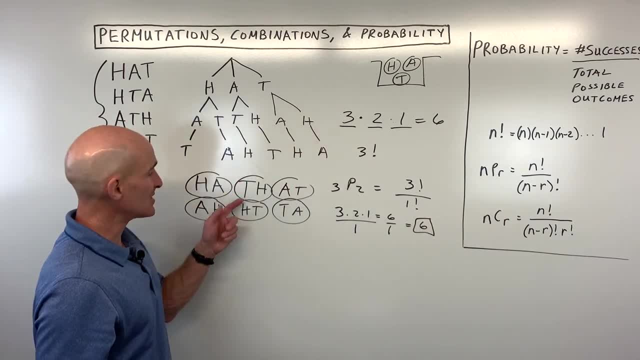 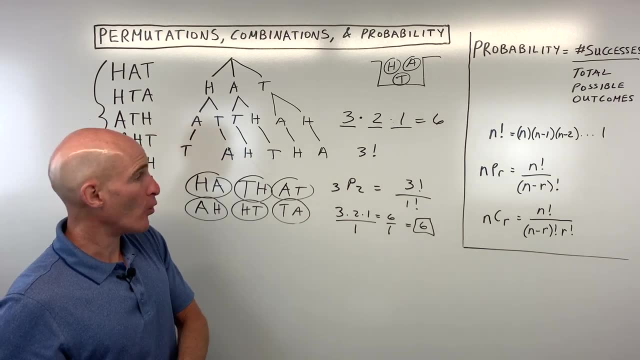 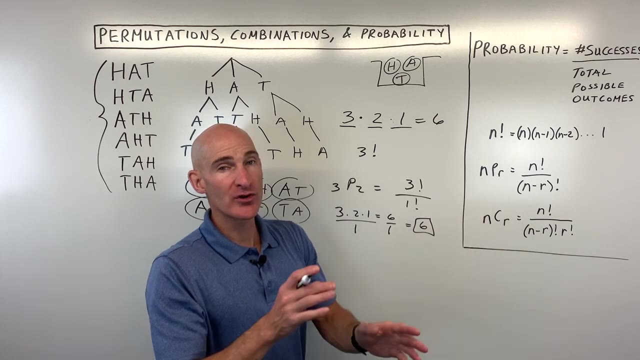 So you can see there's six different possibilities and these are the six that we just wrote down here. Now, what happens if you're not concerned with the order? That's what a combination is. So if we said: how many ways are there to choose two letters out of three where the order is not? 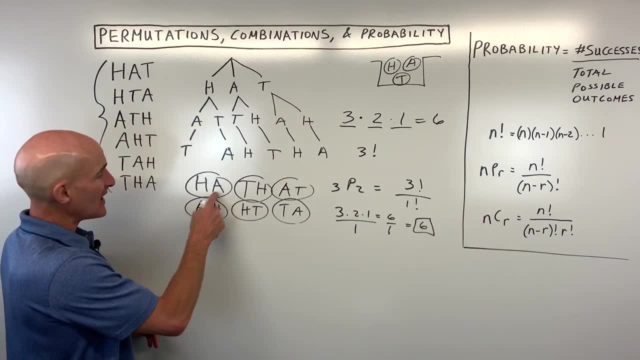 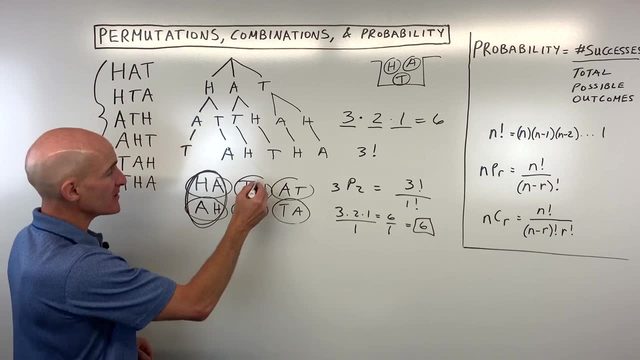 where the order is not important. what we would have is H and A, A and H. those would be like the same outcome. It's the same two letters, So you'd only count that once. T and H, H and T, Those. 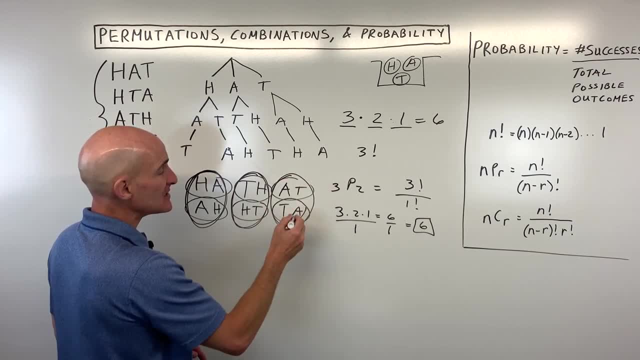 are going to be the same: T and H, H and T. those are going to be the same. T and H, H and T, those are are the same two letters. We'd only count that once. a and t, t and a. we'd only count that once. 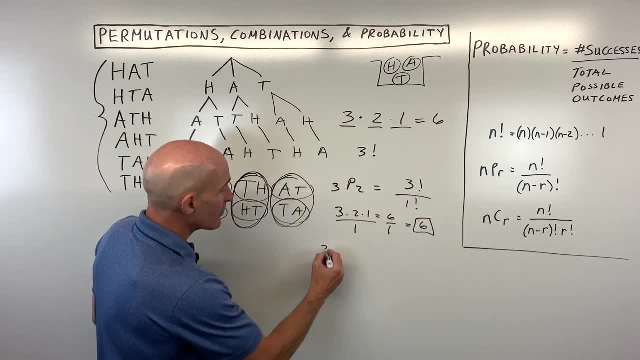 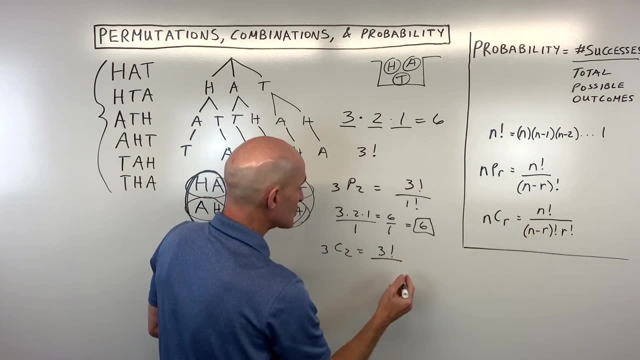 because it's the same two letters. So what we could do here, we could say 3c2, okay, 3 combination. 2 equals 3 factorial, over 3 minus 2, which is 1 factorial, and then times r factorial, which is: 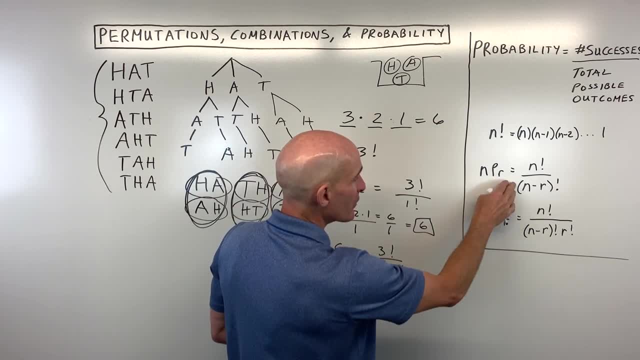 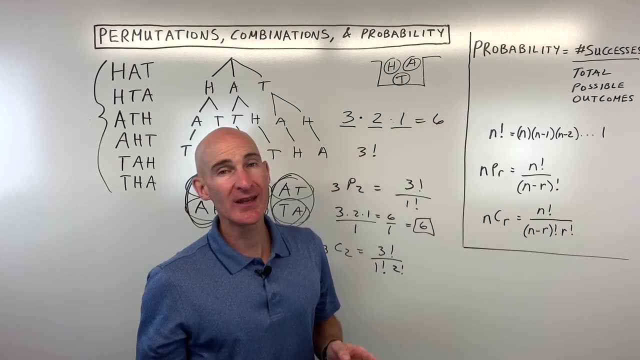 2 factorial. Now you might be saying: you know these formulas look very similar to one another. The only difference is we're dividing by this r factorial. What that r factorial is doing is it's dividing out the multiplicities, meaning that you're not going to count h and a and a and h as 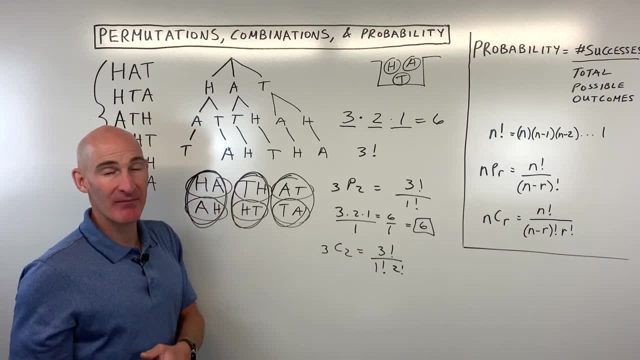 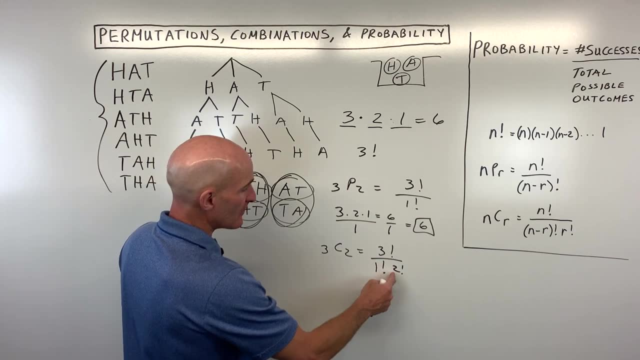 the same, I mean as two different ones. you're going to count it as the same outcome, right? So you don't want to double count, And so that's what we're doing is, we're basically saying h and a, a and h. we don't want to double count that. so we're dividing by 2: factorial. So if we simplify this, 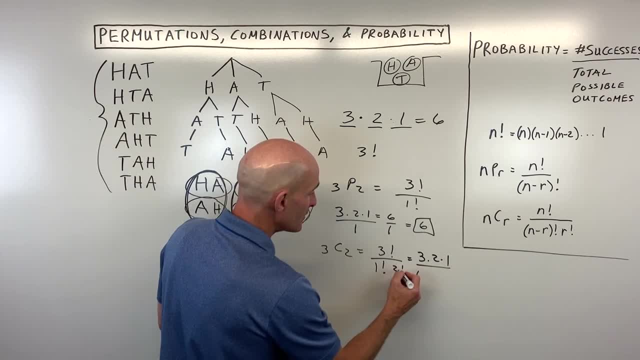 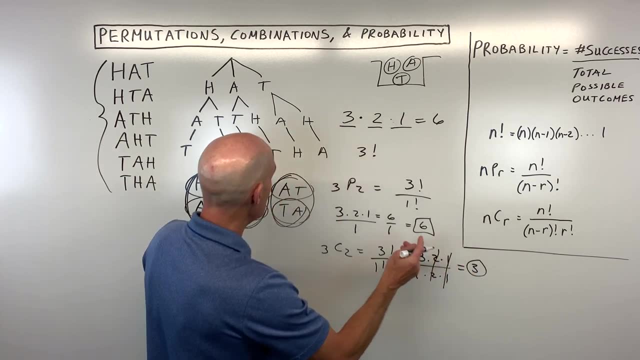 we get 3 times 2 times 1, 1 factorial is 1, 2 factorial is 2 factorial 2 times 1, you can see these are canceling and 3 divided by 1 is equal to 3, and you can see we. 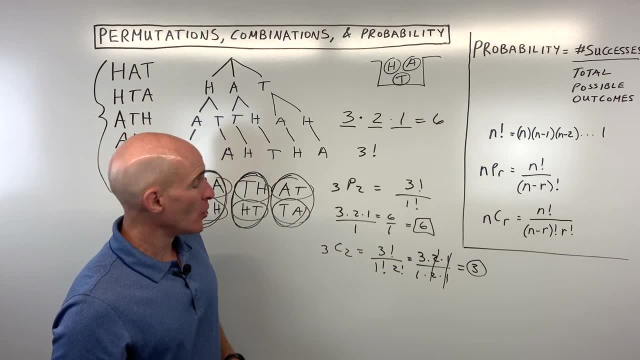 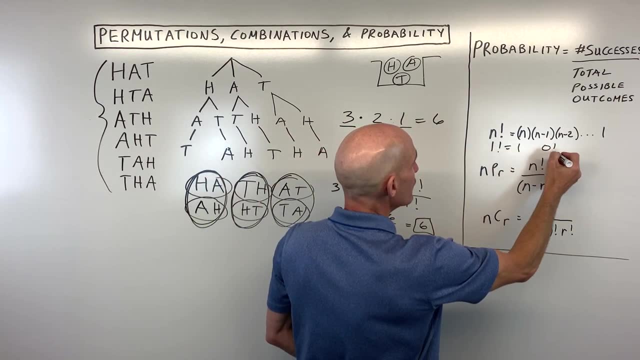 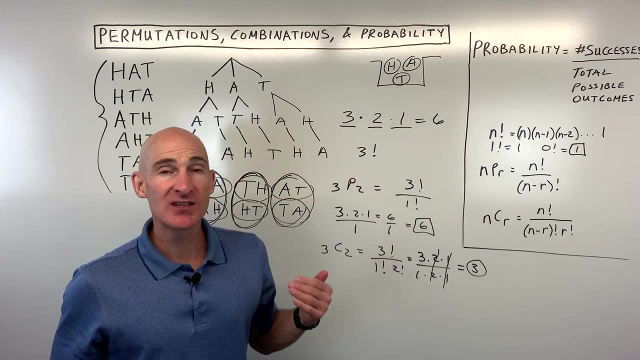 got 3 outcomes here. So one other thing that's important to remember: when you have this n factorial- 1 factorial, we said, is 1, 0 factorial- you have to memorize this one. it's also equal to 1.. So if you get 0 factorial, just realize that's 1.. So let's dive into some of the word problems. 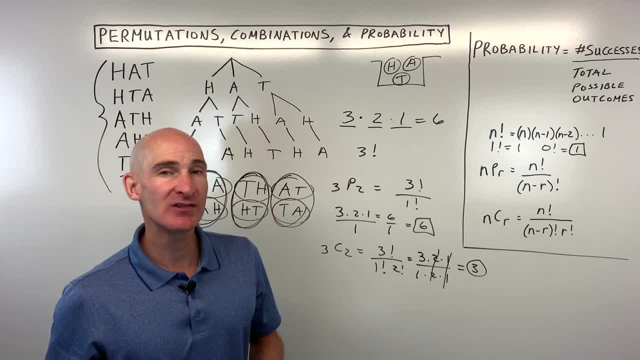 and you'll get a better feel for how to work with these permutations, combinations, factorials and e. So let's dive into some of the word problems and you'll get a better feel for how to work with even probability, which we're going to talk about in just a second. 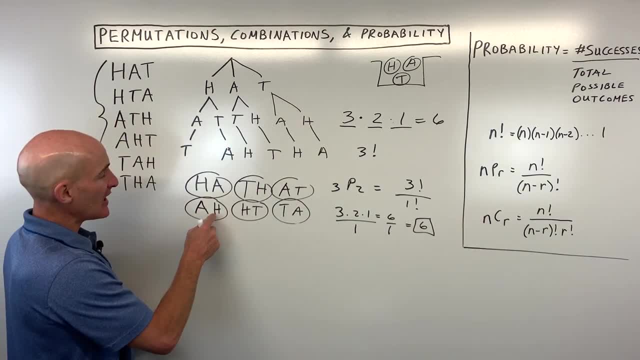 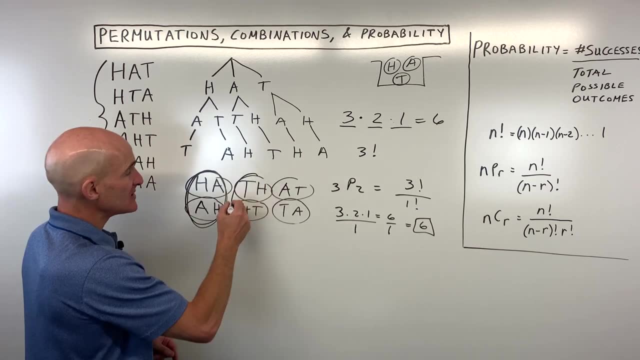 important. What we would have is H and A, A and H, those would be like the same like outcome, It's the same two letters. so you'd only count that once T and H, H and T, those would be the same letters. So what happens is only count that once T and H, H and T, those are three letters. 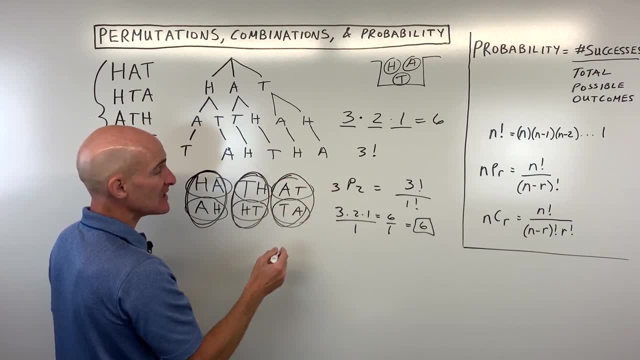 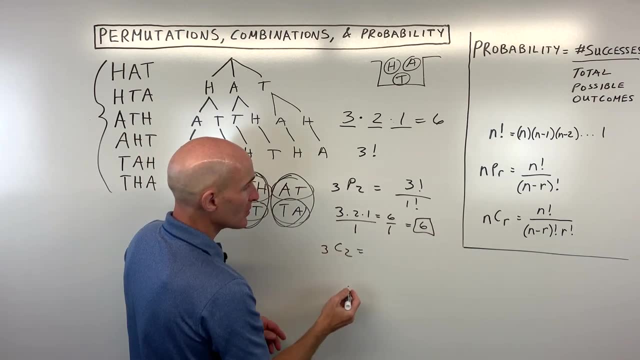 the same two letters. we'd only count that once: a and t, t and a. we'd only count that once, because it's the same two letters. So what we could do here, we could say: 3c2, okay, 3, combination 2. 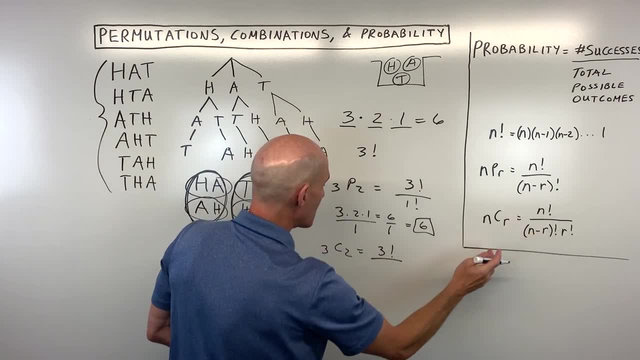 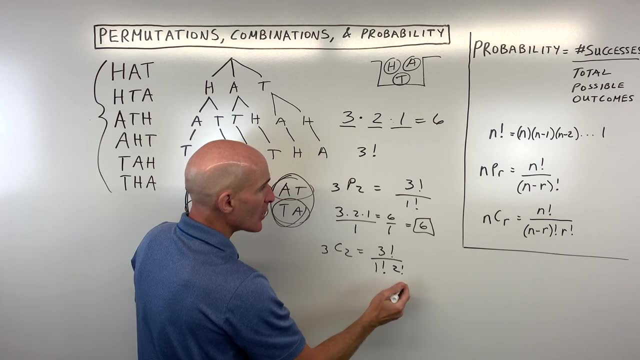 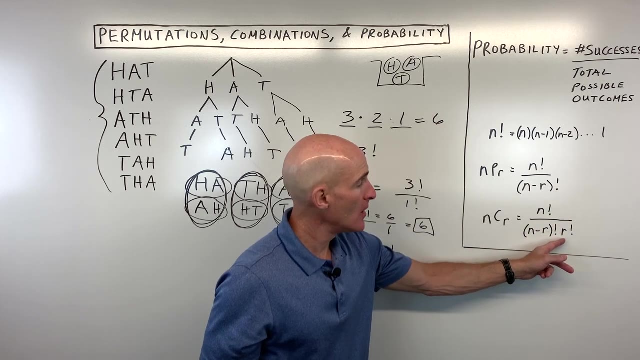 equals 3 factorial over 3 minus 2, which is 1 factorial, and then times r factorial, which is 2 factorial. Now you might be saying you know. these formulas look very similar to one another. The only difference is we're dividing by this r factorial. What that r factorial is doing is it's 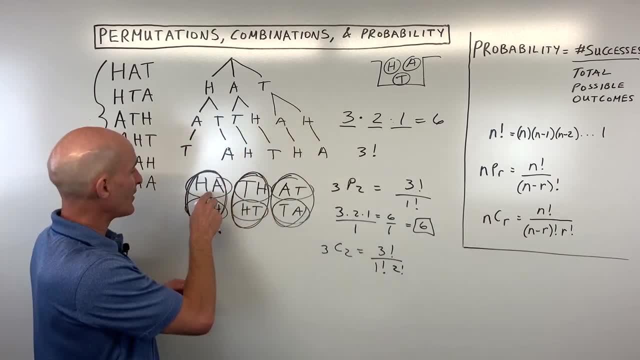 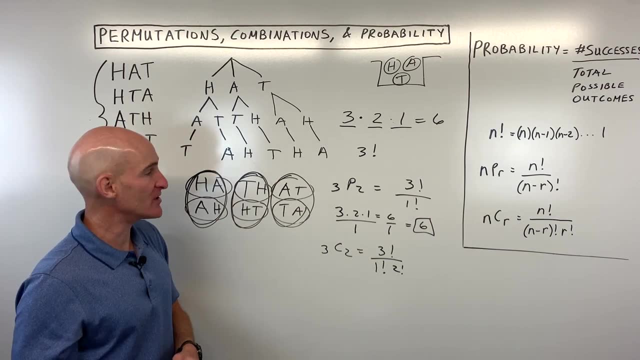 dividing out the multiplicities, meaning that you're not going to count h and a and a and h as the same, I mean as two different ones. you're going to count it as the same outcome, right? So you don't want to double count, And so that's what we're doing, is we're basically saying h and a- a. 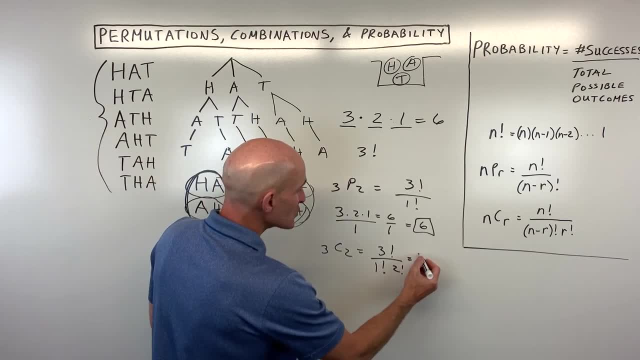 and h. we don't want to double count that, so we're dividing by 2 factorial. So if we simplify this, we get 3 times 2 times 1, 1 factorial is 1, 2 factorial is 2 factorial. 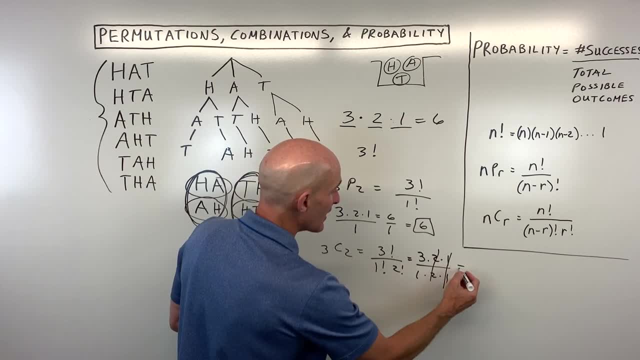 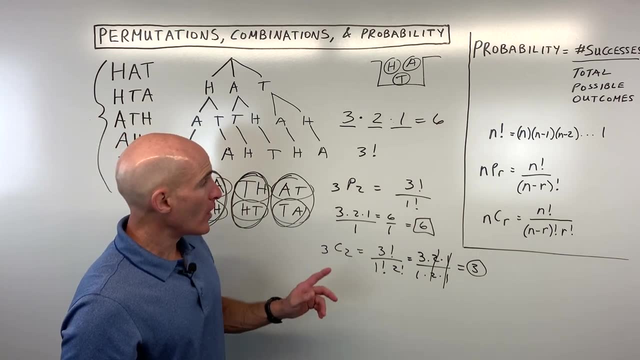 2 times 1, you can see these are canceling, and 3 divided by 1 is equal to 3, and you can see we got 3 outcomes here. So one other thing that's important to remember when you have this n. 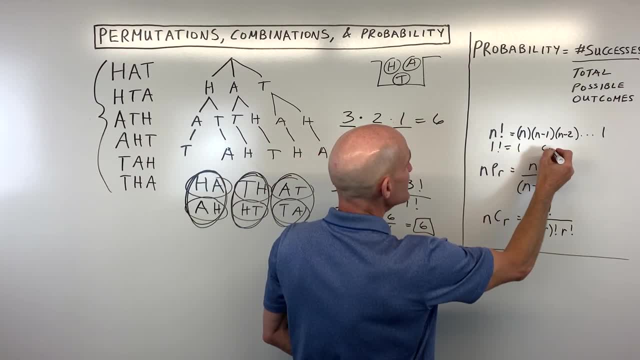 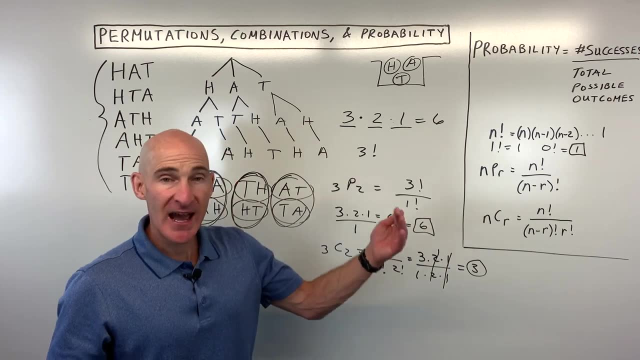 factorial. 1 factorial, we said, is 1,, 0 factorial. you have to memorize this one. it's also equal to 1.. So if you get 0 factorial, just realize that's 1.. So let's dive into some of the word problems. 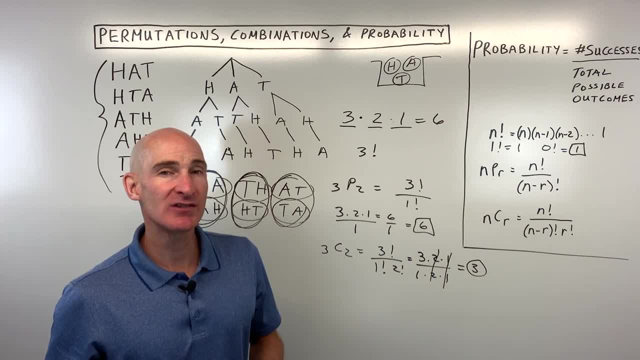 and you'll get a better feel for how to work with these permutations, combinations, factorials and e. So let's dive into some of the word problems and you'll get a better feel for how to work with even probability, which we're going to talk about in just a second. 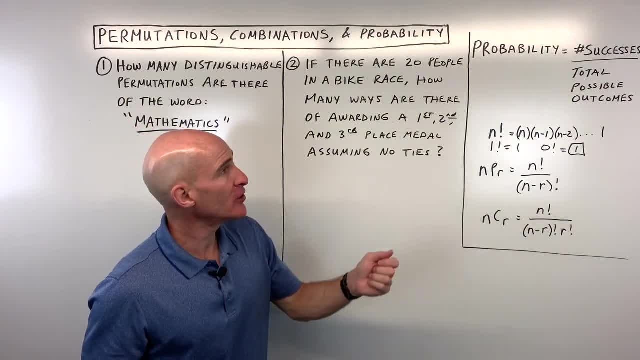 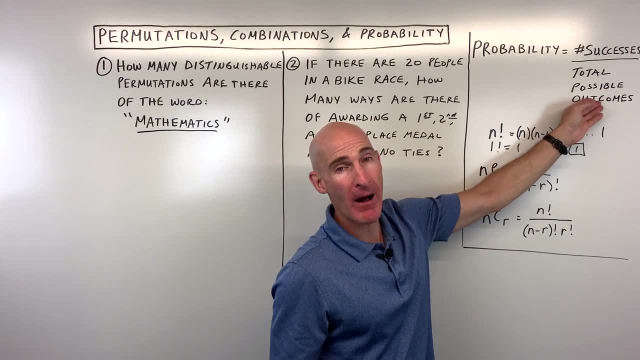 Now, when we talk about probability, what probability is? it's the number of successful outcomes, or what you're looking for, what you want, divided by the total possible number of outcomes. And that's why we're talking about permutations and combinations. first, because that 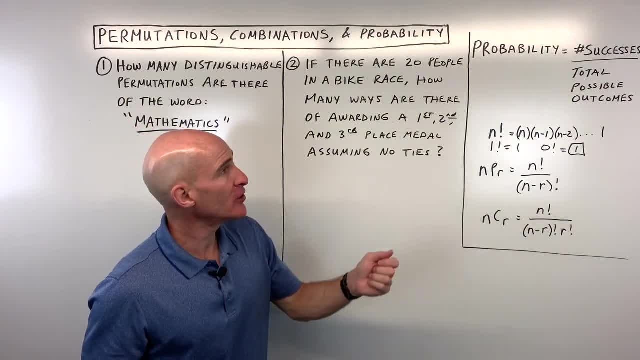 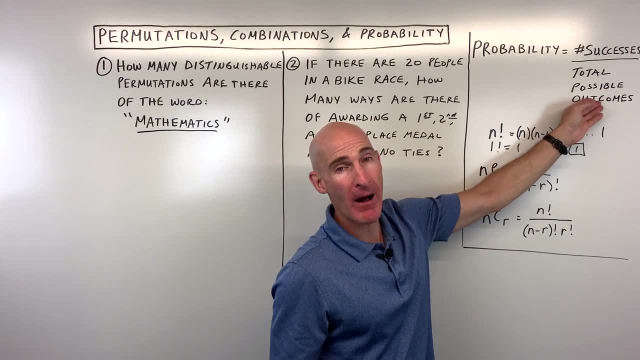 Now, when we talk about probability, what probability is? it's the number of successful outcomes, or what you're looking for, what you want, divided by the total possible number of outcomes. And that's why we're talking about permutations and combinations. first, because that 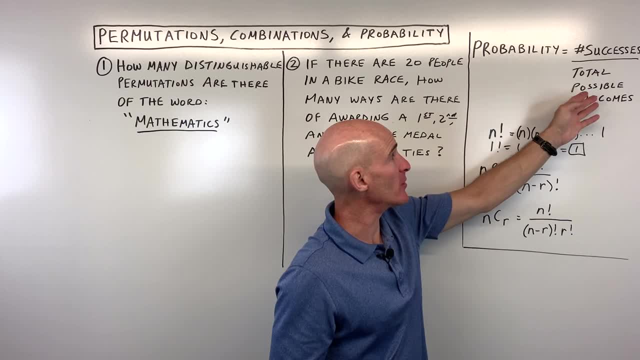 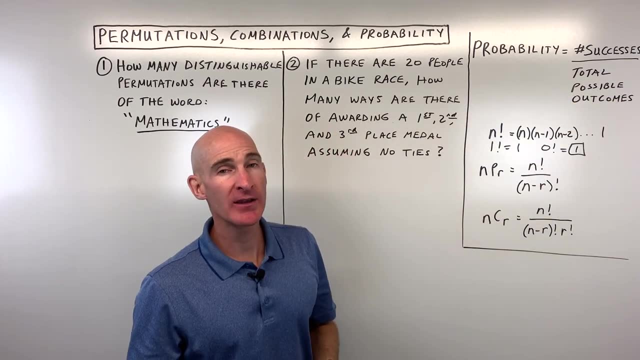 tells us the number that we're dealing with, the number of successes or the number of total possible outcomes. But when you think of probability it's written as a fraction or a decimal, unless they say what's the percent chance that something could happen. But basically probability. 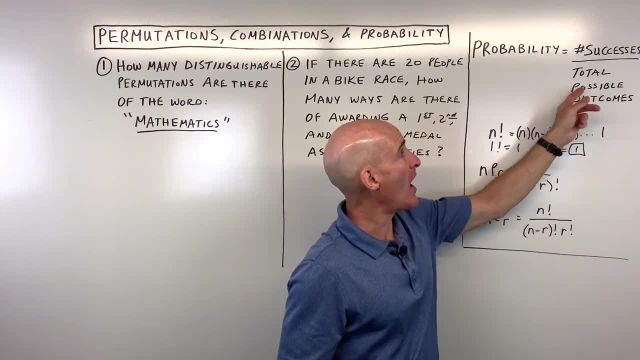 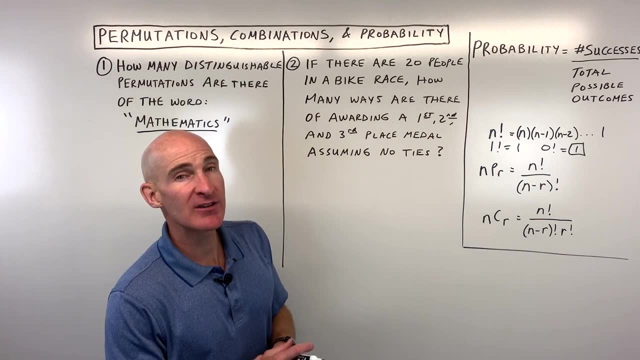 again is just talking about the number of what you want divided by the total, and that's what our permutations are going to give us, our combinations are going to give us, our factorials are going to give us. So let's dive into some word problems. When you're doing these problems, 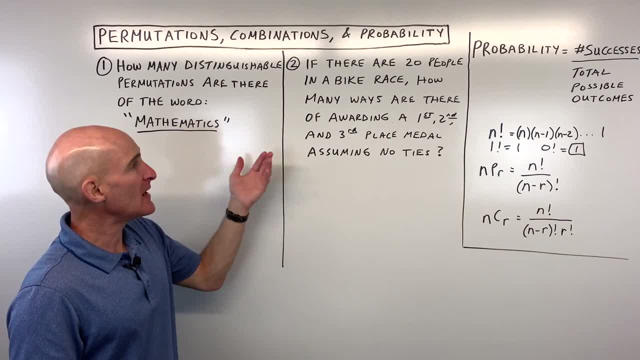 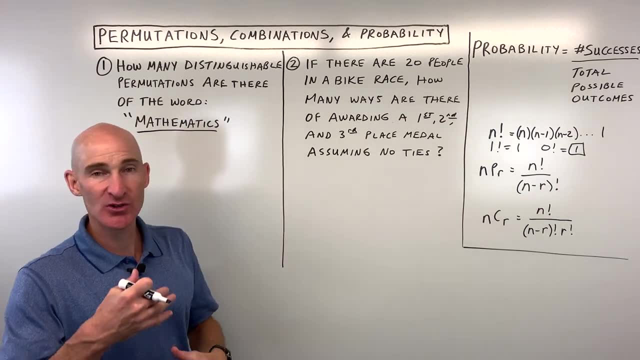 on your homework or just trying to solve problems on your own. you may not have problems that are exactly like these problems- these 15 that we're going to do- but you'll have ones that are similar. So if you understand these concepts, you can apply them to. 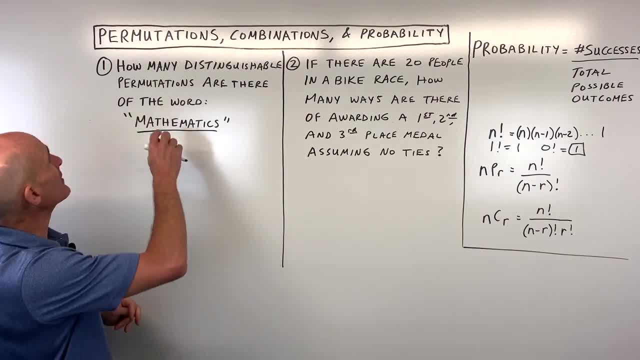 to additional problems that you're working on. So let's go through this variety of problems. So, starting with number one, it says how many distinguishable permutations are there of the word mathematics. So basically, again they're talking about permutations. that's saying 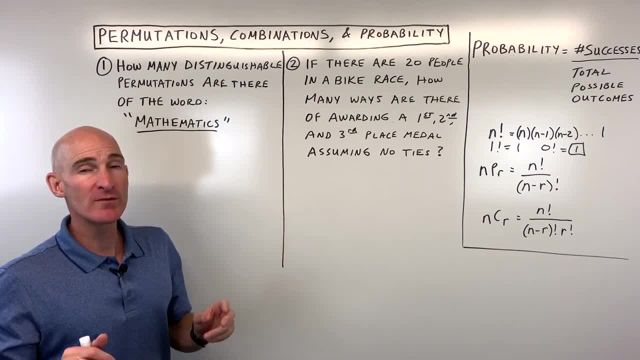 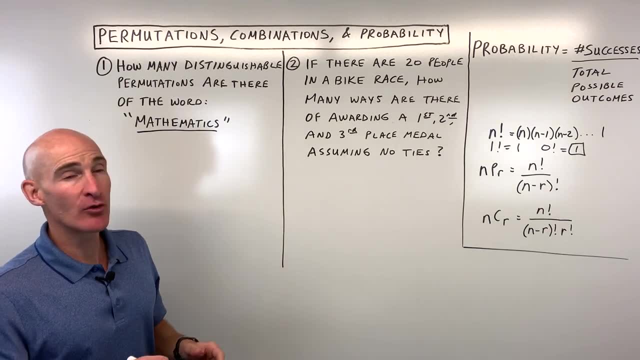 how many ways are there of ordering all these letters so that it forms a new quote, unquote word? Well, there's a lot of letters here. If we had to write them out by hand, we would grow old and and and die, because it's going to take a long time, right? 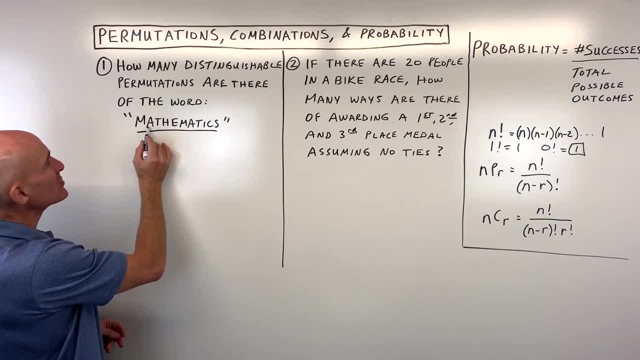 So. So an easy way of doing this is: let's count how many letters there are: 1, 2, 3, 4, 5, 6,, 7,, 8,, 9,, 10, 11.. So there's how many letters there are. 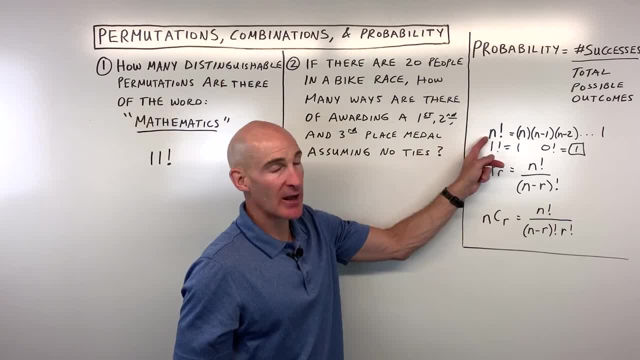 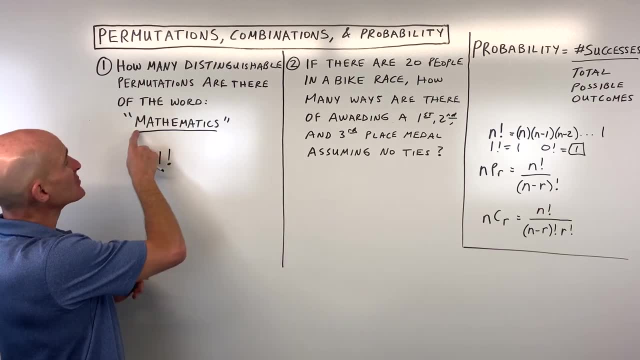 So there's 11 factorial ways. Okay, Remember we talked about n factorial. there's 11 factorial ways of ordering all those letters, but you see how there's some repetitions. We have 2ms, So we're going to divide by two factorial. 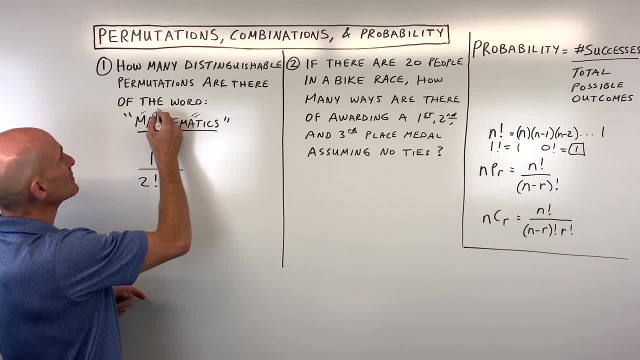 There's, uh, two a's, So we're going to divide by another two factorial. and there's, there's two t's, so we're going to divide by another two factorial. now if there was three t's, we divide by three factorial. or if there was four r's, let's say you divide by four factorial. and the reason is: 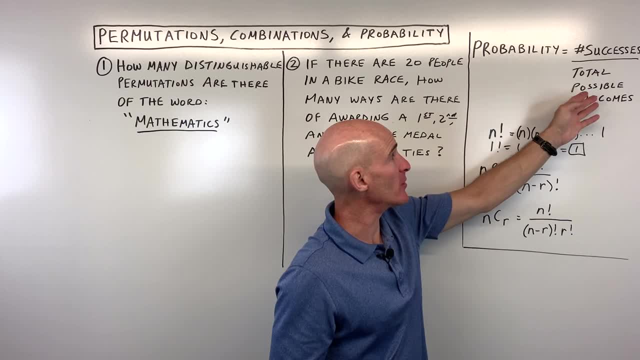 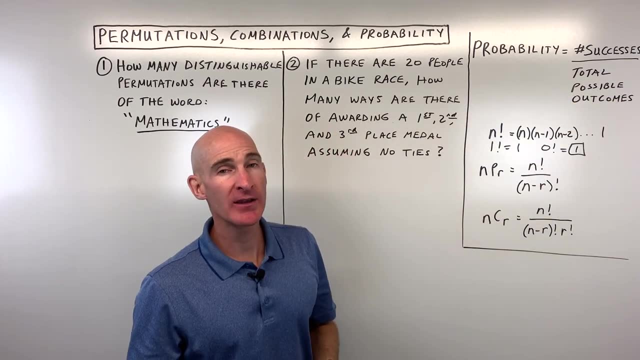 tells us the number that we're dealing with, the number of successes or the number of total possible outcomes. But when you think of probability it's written as a fraction or a decimal, unless they say what's the percent chance that something could happen. But basically probability. 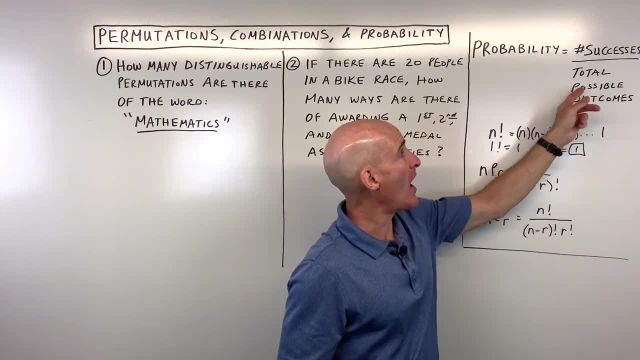 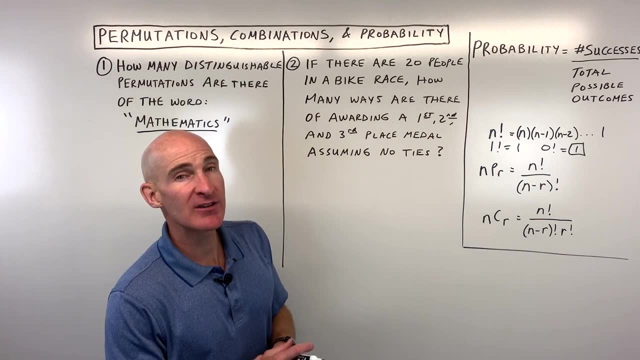 again is just talking about the number of what you want divided by the total, and that's what our permutations are going to give us, our combinations are going to give us, our factorials are going to give us. So let's dive into some word problems. When you're doing these problems, 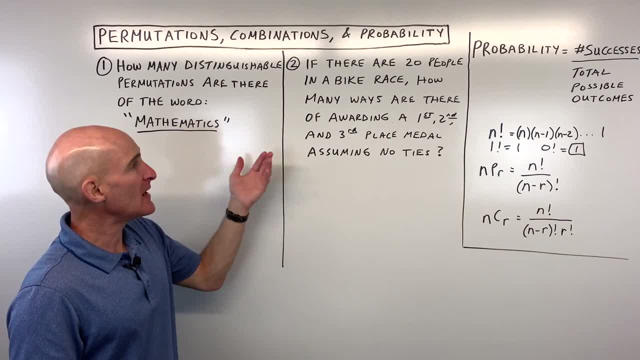 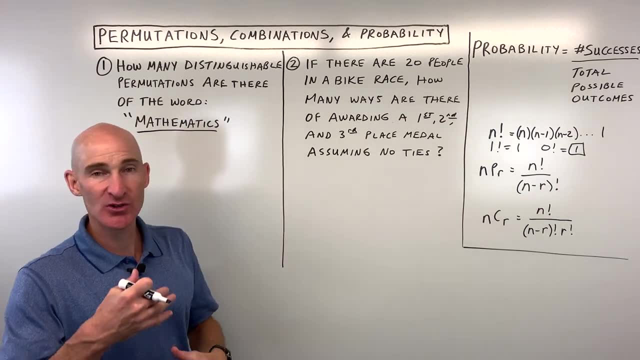 on your homework or just trying to solve problems on your own. you may not have problems that are exactly like these problems- these 15 that we're going to do- but you'll have ones that are similar. So if you understand these concepts, you can apply them to. 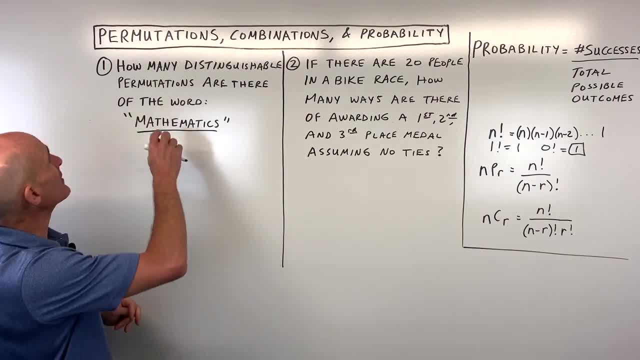 to additional problems that you're working on. So let's go through this variety of problems. So, starting with number one, it says how many distinguishable permutations are there of the word mathematics. So basically, again they're talking about permutations. that's saying 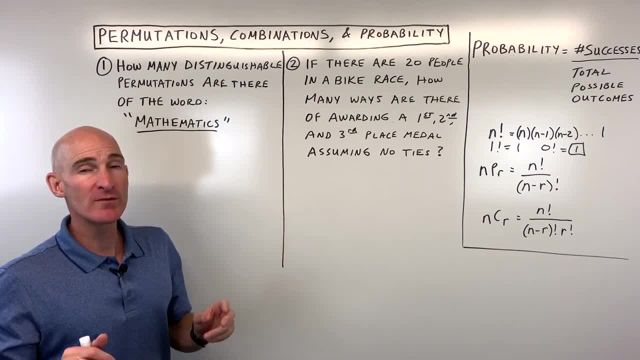 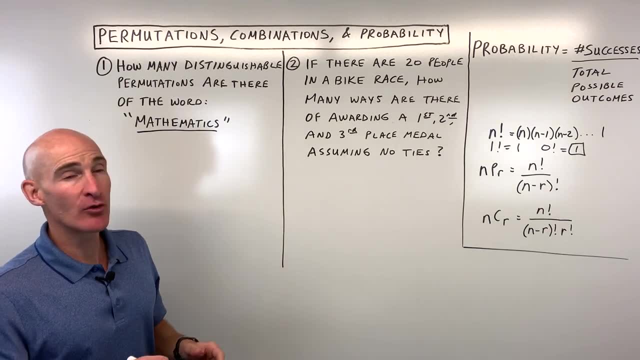 how many ways are there of ordering all these letters so that it forms a new quote-unquote word? Well, there's a lot of letters here. if we had to write them out by hand, we would grow old and die, because it's going to take a long time, right. 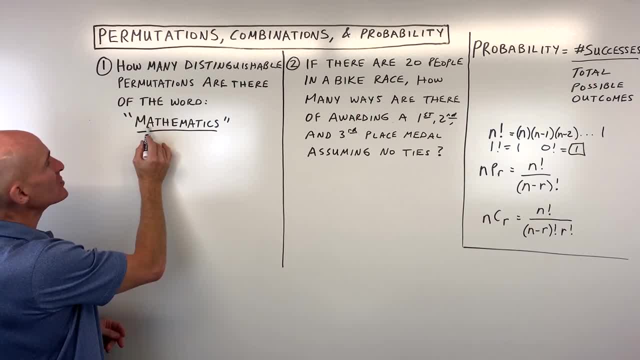 So an easier way of doing this is: let's count how many letters there are: 1,, 2,, 3,, 4,, 5,, 6,, 7,, 8,, 9,, 10,, 11.. 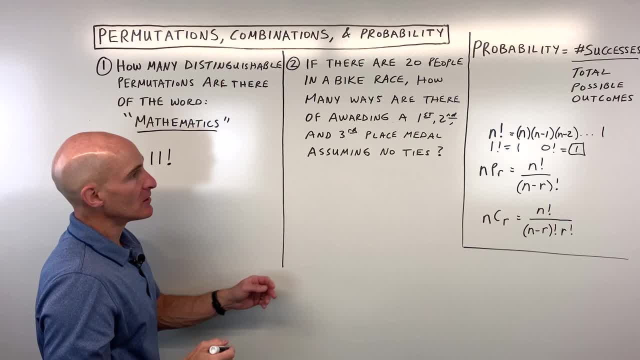 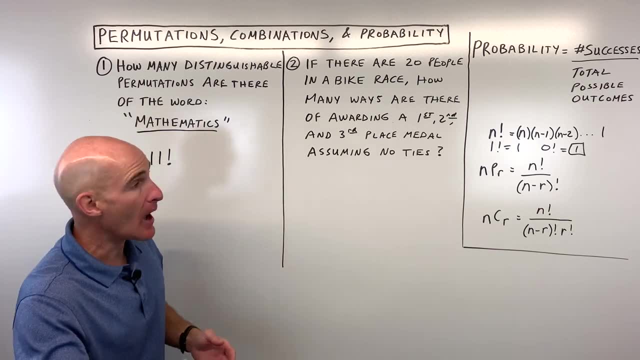 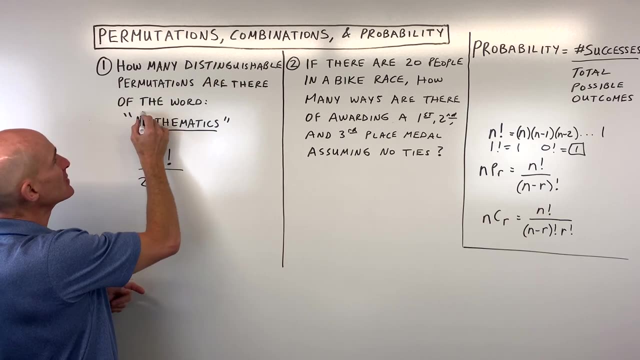 So there's 11 factorial ways. okay, Remember we talked about n factorial. There's 11 factorial ways of ordering all those letters, But you see how there's some repetitions. We have 2 m's, so we're going to divide by 2 factorial. There's 2 a's, so we're going to divide by another 2 factorial, and there's 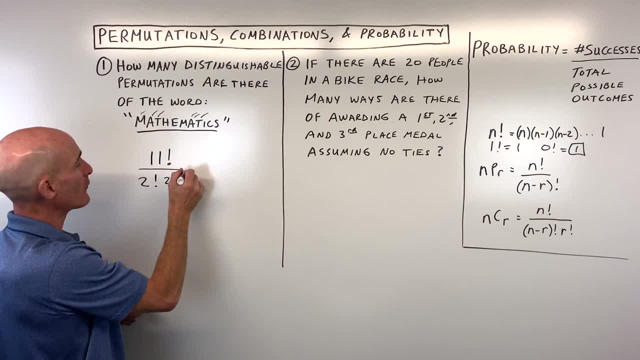 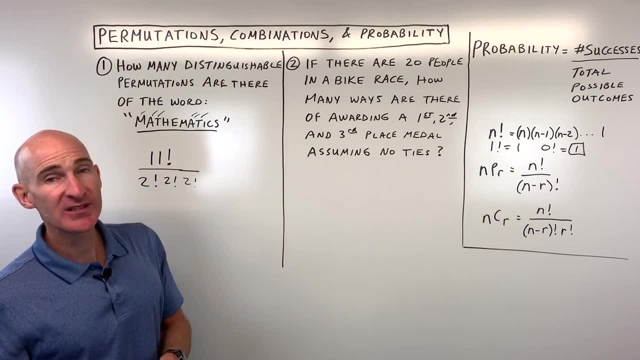 2 t's, so we're going to divide by another 2 factorial. Now if there was 3 t's, we divide by 3 factorial. or if there was 4 r's, let's say you divide by 4 factorial And the reason is: 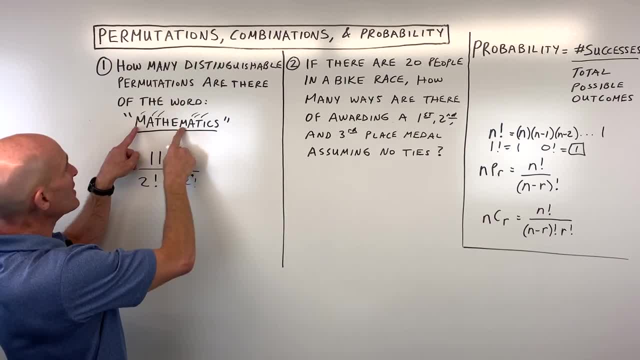 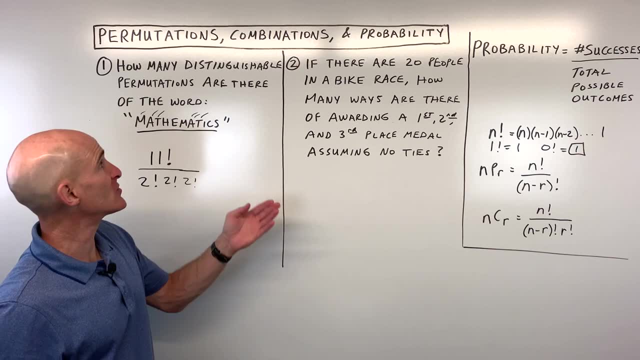 like 2, factorial is 2 times 1, meaning there's two different ways to take these m's and like interchange them, but it would form the same word mathematics. You wouldn't even know that anything was different about it. so that's why it's saying uh, distinguishable meaning. you can tell that. 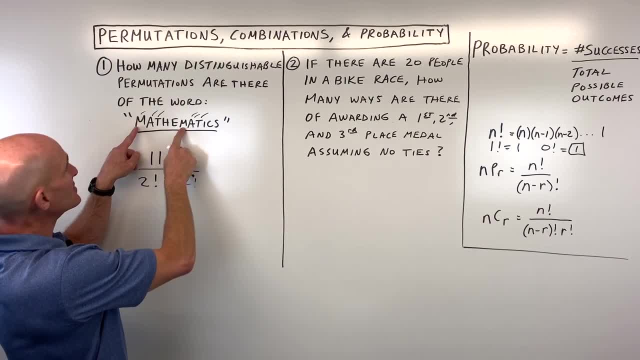 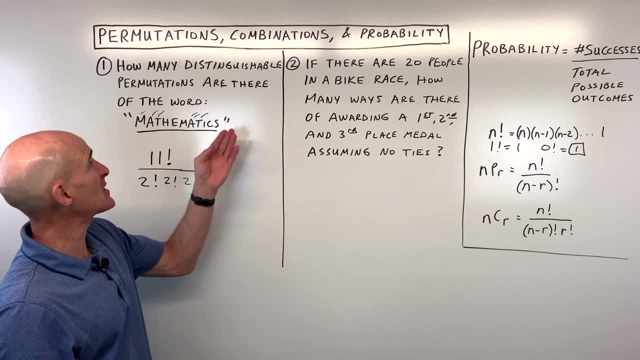 like two factorial is two times one. meaning there's two different ways to take these m's and like: interchange them, but it would form the same word, mathematics. you wouldn't even know that anything was different about it, so that's why it's saying distinguishable meaning. you can tell that. 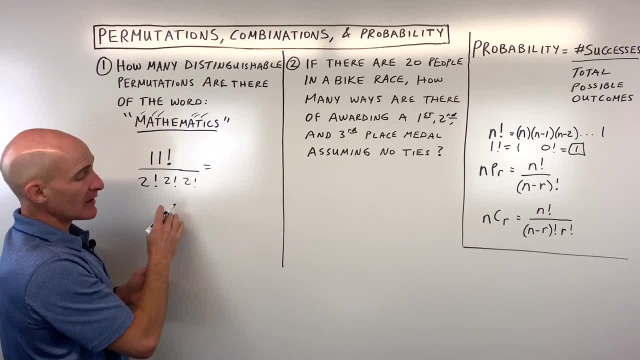 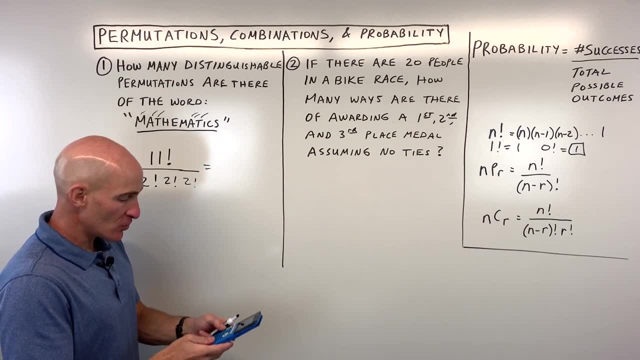 they're different. So what we're going to do now is we're going to go to the calculator. You should have a factorial by. If not, you can just do 11 times 10 times 9,, all the way down to 1.. The factorial is probably under a. 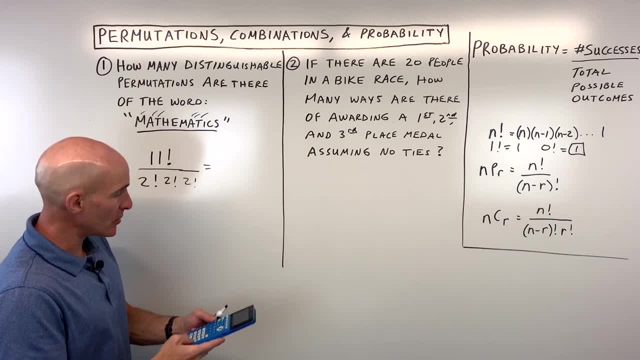 probability key that you have on your calculator. That's what mine's under. And then I'm going to divide by 2 factorial, which is 2 times 1,, 2 times 1, 2 times 1,, which is 8.. So I'm going to divide. 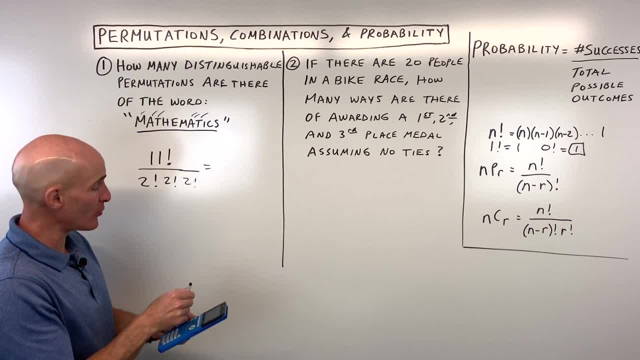 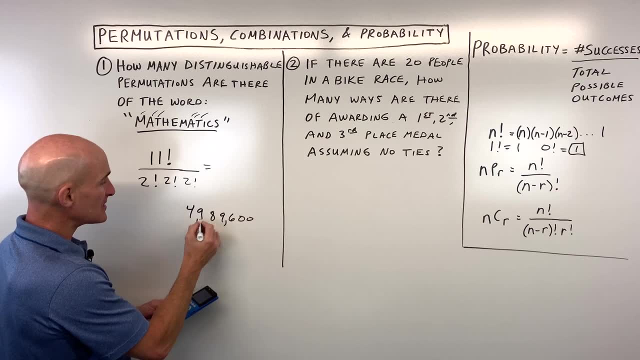 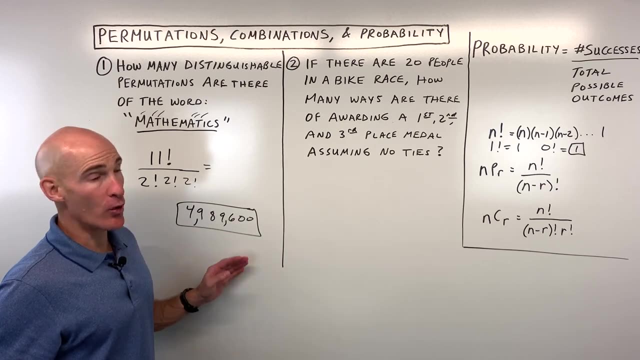 11 factorial by 8.. Not 8 factorial, but just the number 8.. And that's coming out to 4989600.. So basically, almost 5 million different ways of ordering these letters, such that it forms a new quote-unquote word. Okay, quite a few. So number: 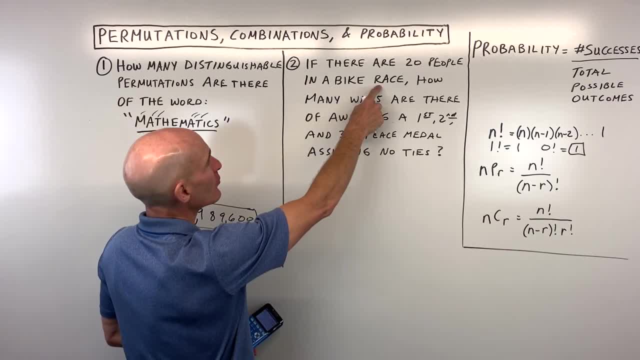 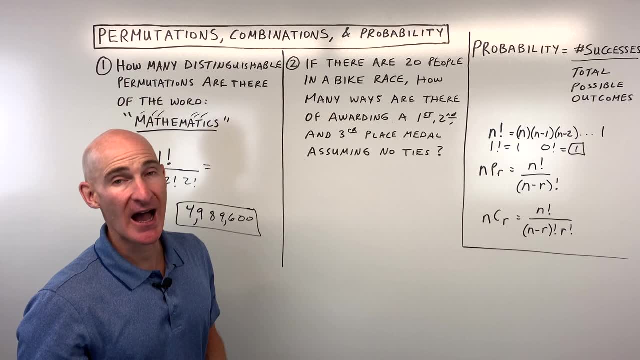 2. now Let's look at this one. It says: if there are 20 people in a bike race, how many ways are there of awarding a first, second and third place medal, assuming that there are no ties? Okay, a little bit different problem here. So now what we're trying to do is figure out. 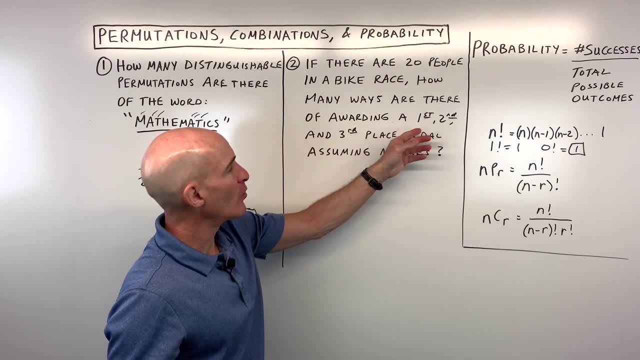 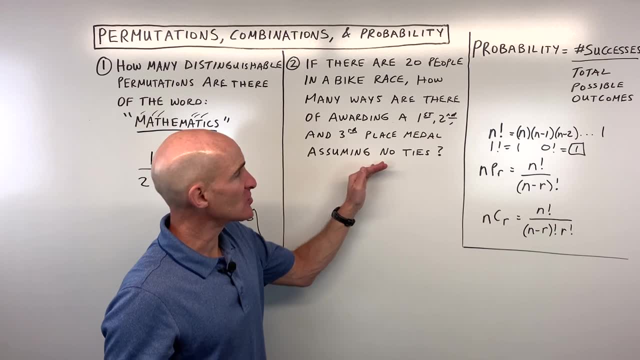 hmm, out of 20 people, we want to know how many ways there are of picking three of those people to be the first, second and third place medal winner. So we're going to go to the calculator And oftentimes what you want to ask yourself is: is the order important or is it not important? 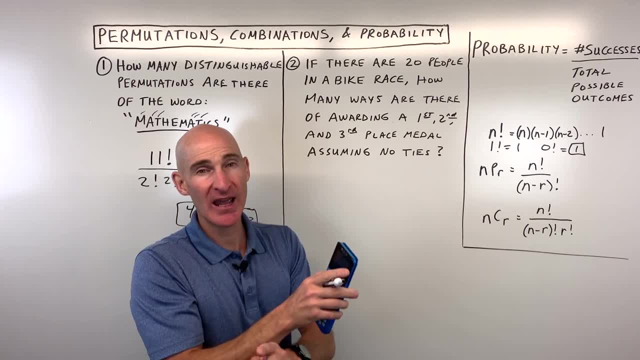 So if I change like person A, B and C, C, B and A, does that result in a different outcome? Well, yes, because in that case they would be getting different medals: Gold, silver, bronze. 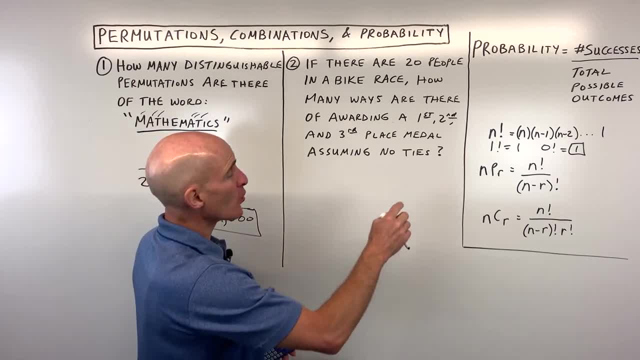 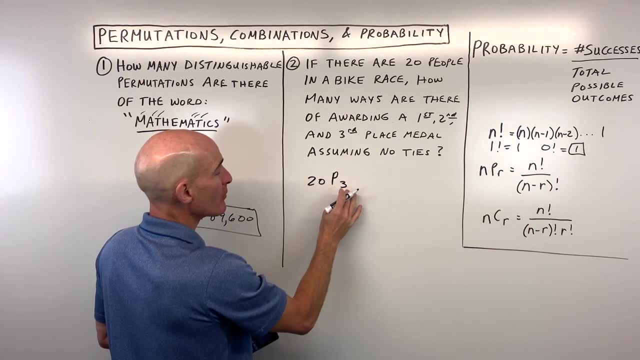 or you know it'd be a different order. So in this case, because the order is important, we want to use the permutations And we're going to say: out of 20 people, how many ways are there to pick three of them where that order is important? And so, using our formula here, 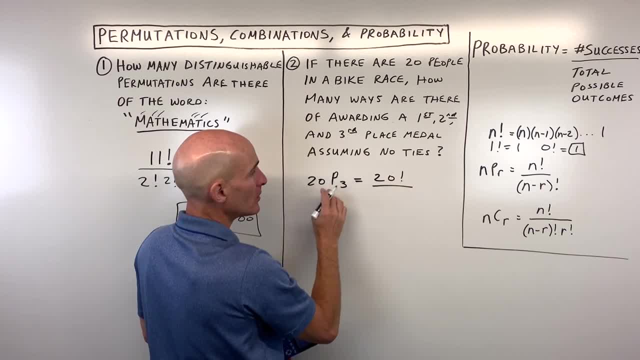 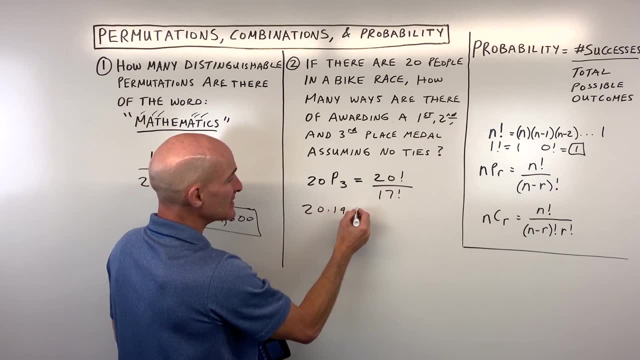 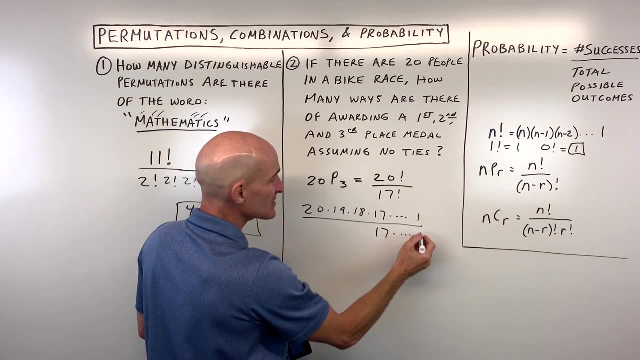 this is going to be 20 factorial over n minus r. So 20 minus 3 is 17 factorial. 20 factorial is 20 times 19 times 18 times 17, all the way down to 1.. 17 factorial is also 17 times 16 times 15. 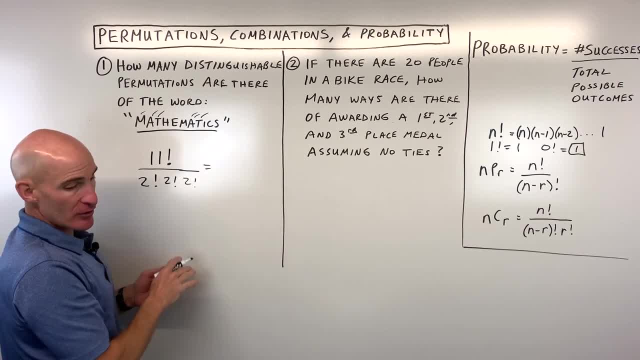 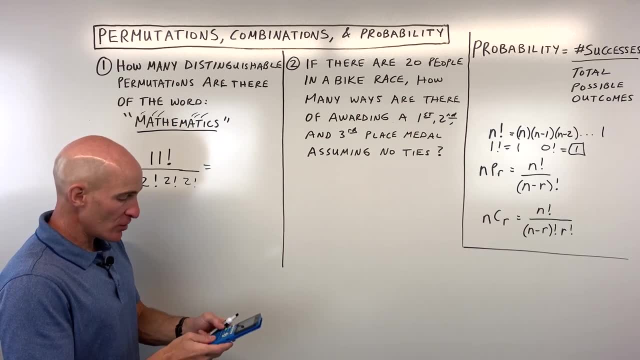 they're different. so what we're going to do now is we're going to go to the calculator. you should have a factorial button. if not, you can just do 11 times 10 times 9, all the way down to 1. the factorial is probably under a probability key that you have on your calculator. that's what. 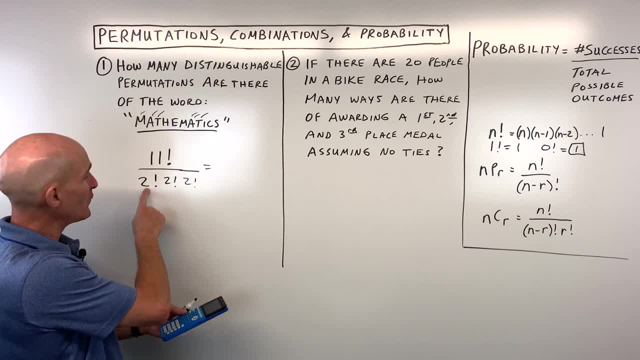 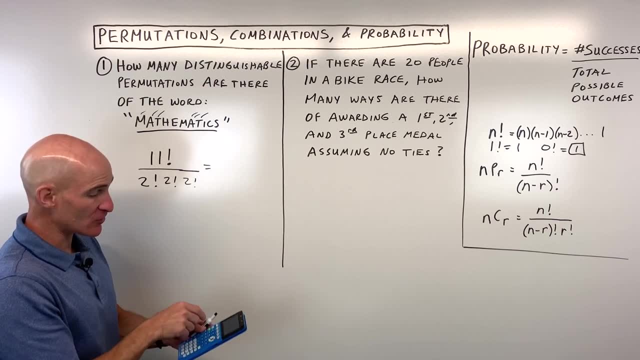 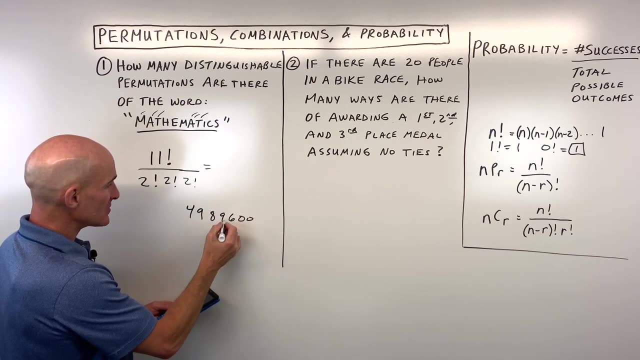 mine's under, and then i'm going to divide by two factorial, which is two times one, two times one, two times one, which is eight. so i'm going to divide 11 factorial by eight, not eight factorial, but just the number eight- and that's coming out to four, nine, eight, nine, six, zero, zero. so basically almost. 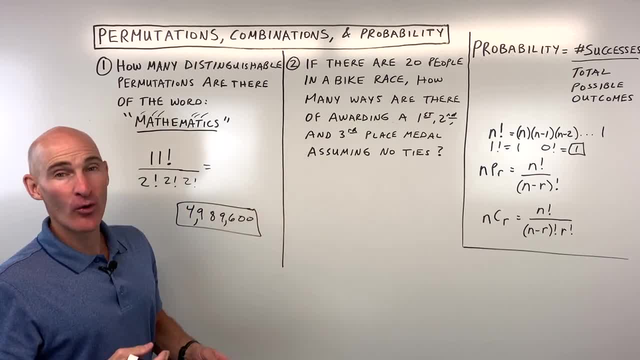 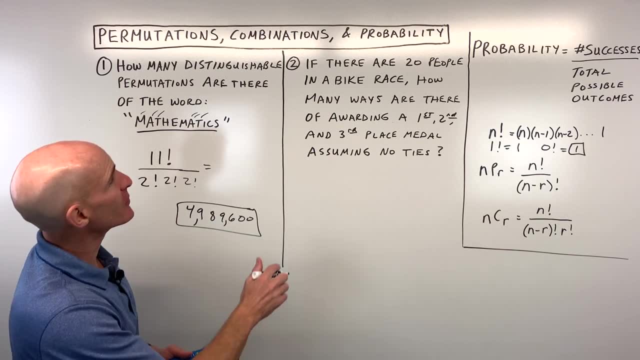 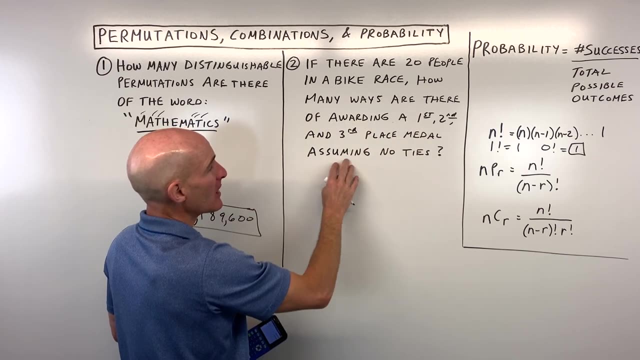 five million, five million, five million different ways of ordering these letters, such that it forms a new quote-unquote word. okay, quite a few, so number two. now let's look at this one. it says: if there are 20 people in a bike race, how many ways are there of awarding a first, second and third place medal, assuming that there? 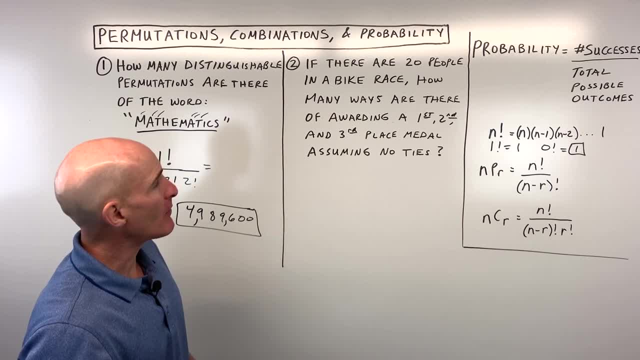 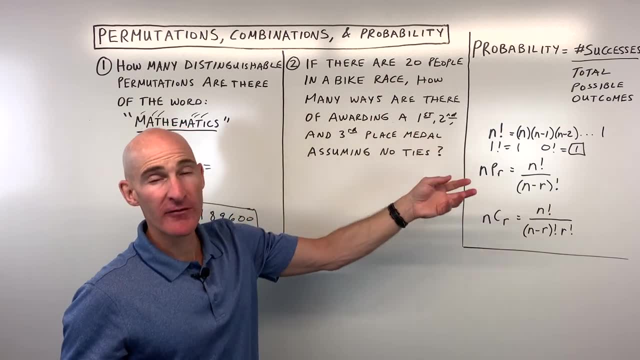 are no ties. okay, a little bit different problem here. so now what we're trying to do is figure out: out of 20 people, we want to know how many ways there are of picking three of those people to be the first, second and third place finisher. and oftentimes what you want to ask yourself is the. 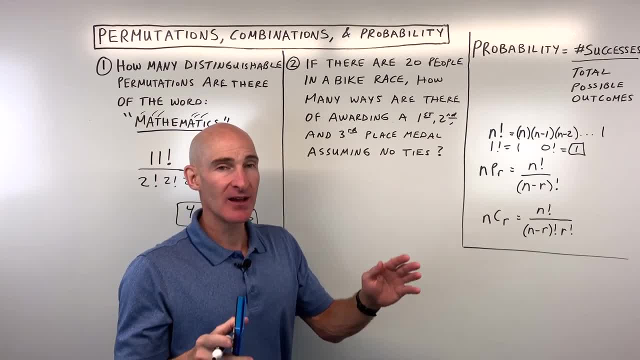 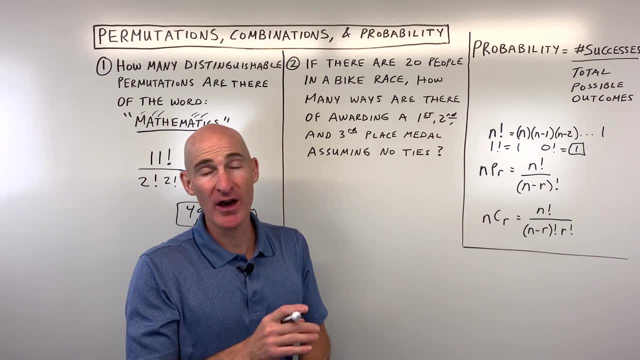 order important or is it not important? so if i change like person a, b and c, c, b and a, does that result in a different outcome? well, yes, because in that case they would be getting different medals: gold, silver, bronze, or you know. it'd be a different order. so in this case, because the order is 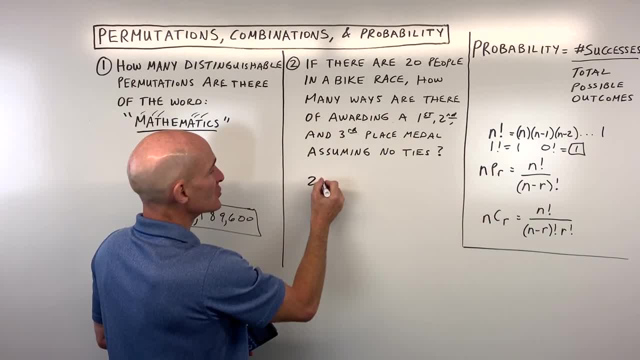 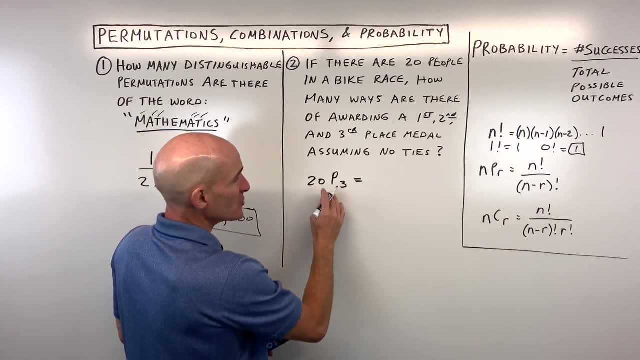 important. we want to use the permutations and we're going to say: out of 20 people, how many ways are there to pick three of them, where that order is important? and so 20 people are going to be the first two to be picked and then the other two are going to be picked. and so what we're going to do, 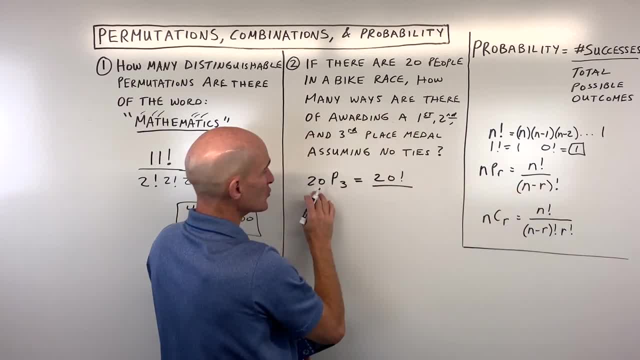 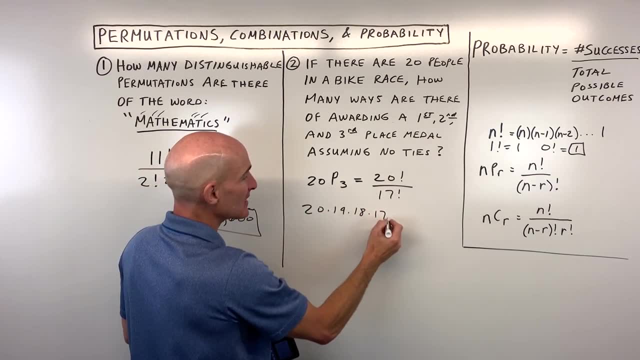 is. we're going to take our formula and we're going to take our formula here. this is going to be 20 factorial over n minus r. so 20 minus 3 is 17 factorial. 20 factorial is 20 times 19 times 18. 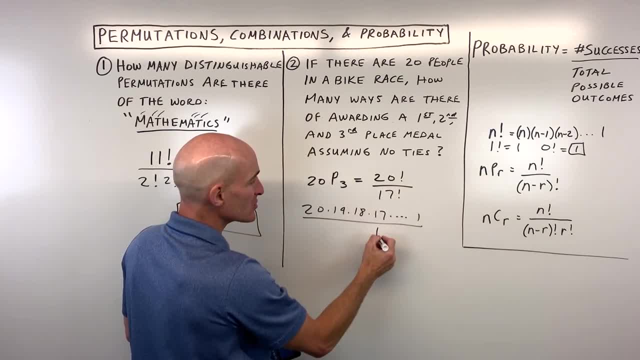 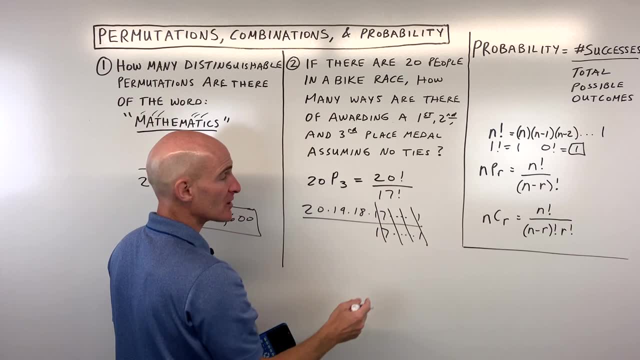 times 17 all the way down to 1. 17 factorial is also 17 times 16 times 15 all the way down to 1. so you can see that the 17, 16 all the way down to 1 are going to cancel and we're just left with 20. 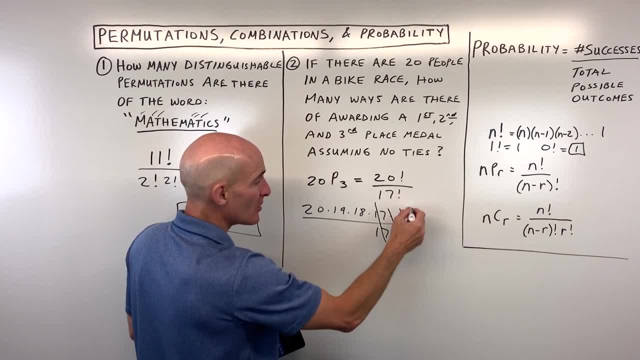 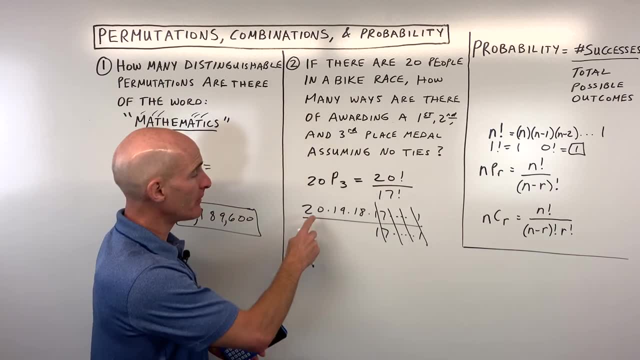 all the way down to 1.. So you can see that the 17,, 16,, all the way down to 1 are going to cancel, And we're just left with 20 times 19 times 18.. Now there's something called the multiplication. 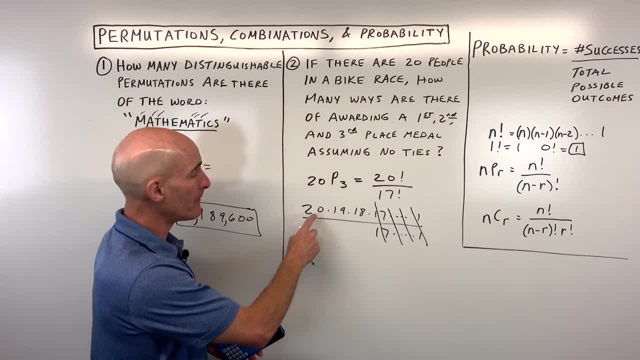 times 19 times 18.. now there's something called the number of people that we want to pick, and more called the multiplication counting principle or the fundamental counting principle, And what you do is you say how many choices are there for, like a first place finisher. There's 20 ways that. 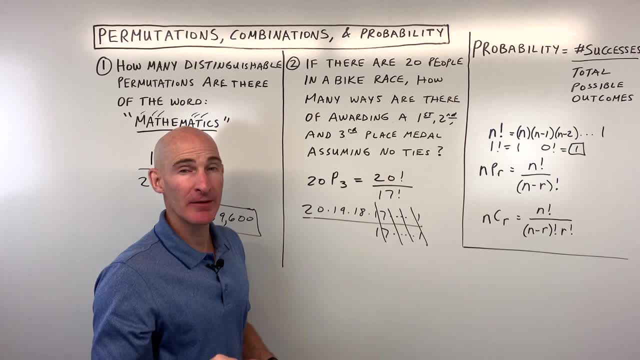 somebody could finish first. Once that person finishes first, how many different people could finish for the second medal? That would be 19.. And once those two people finish, how many ways are there for a third place finisher, 18.. So you can use this fundamental counting principle or you can 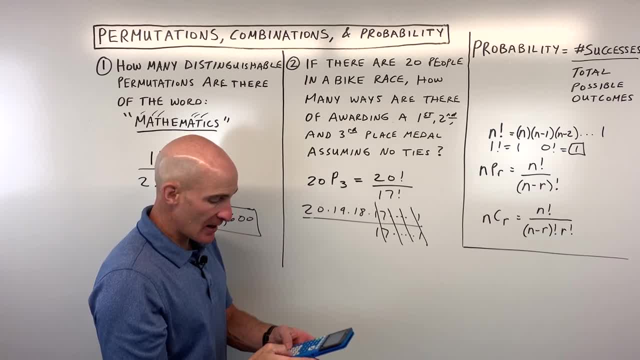 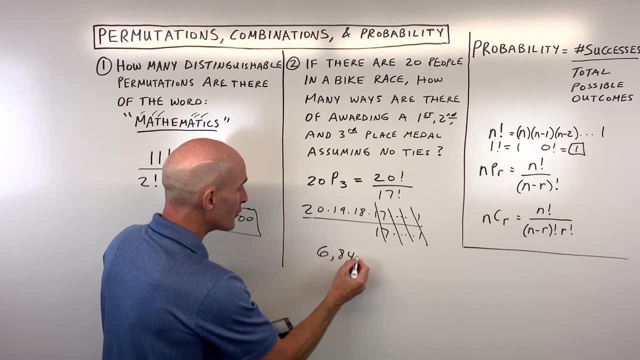 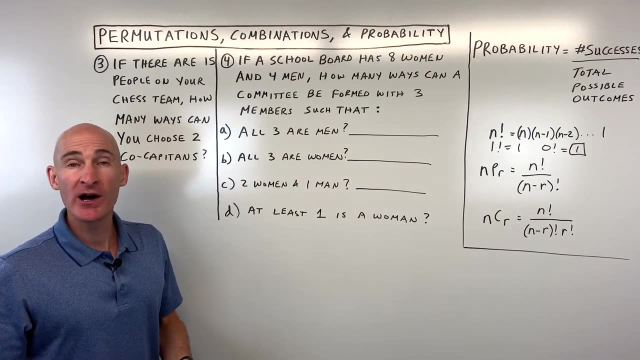 use this NPR formula for this example. So let's multiply that out and see what that comes out to. Okay, this is coming out to 6,840 different ways to award those three medals. Okay, if you want to test yourself on some of these problems, go ahead and pause the video and see if you can do them on. 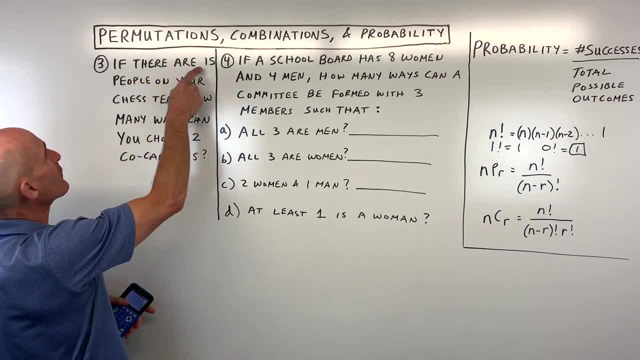 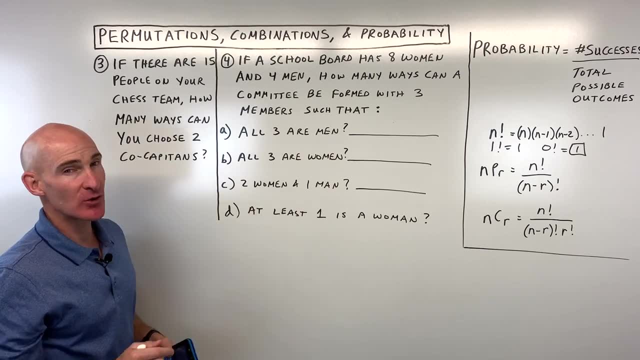 your own. But let's dive into number three. It says: if there are 15 people on your chess team, how many ways can you choose two co-captains? So what do you think about that? Well, what's interesting is: do you think that the order is important, Like if they pick? 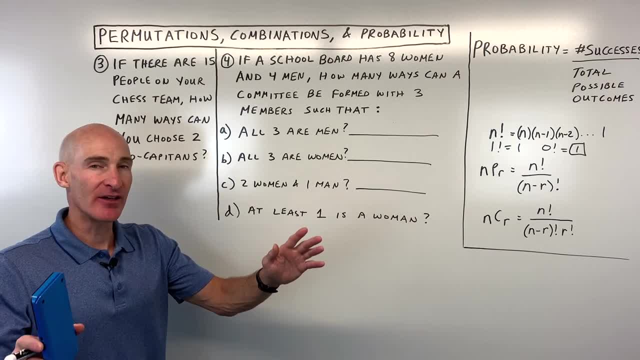 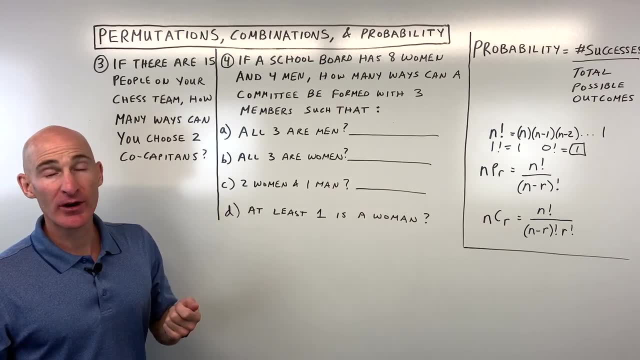 Joe first and Sally second, or Sally first and Joe second. like does the order matter? Well, in this case, because they're co-captains. it's not like the bike race one where, like gold, silver, bronze, like you would get a different medal. In this case they're co-captains, So it. 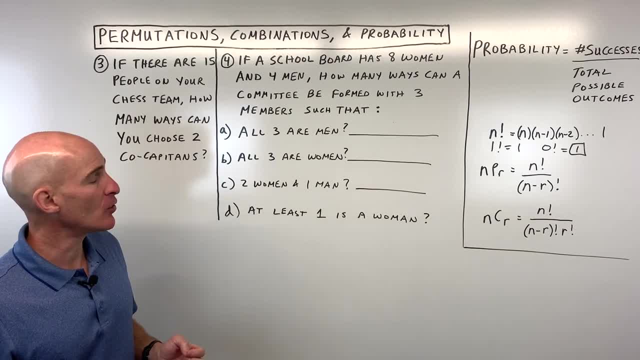 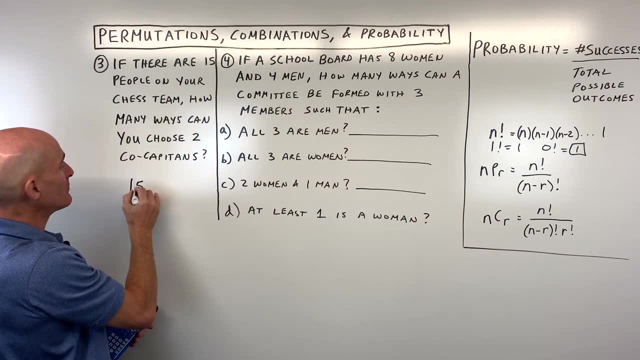 doesn't matter. A and B, B and A, they both made it into being co-captains. The order doesn't matter, You want to use combinations. So here we're saying: out of 15 people, how many ways can 15 chess members, how many ways of choosing two where the order doesn't matter? So using our 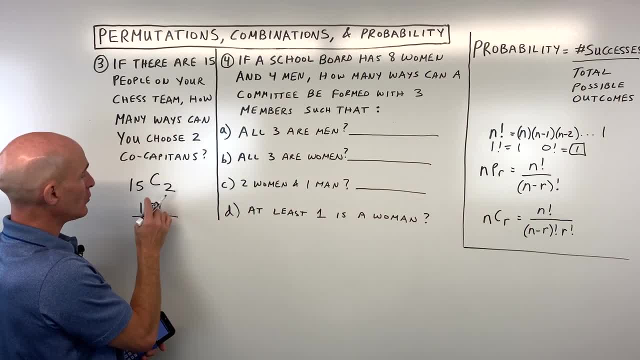 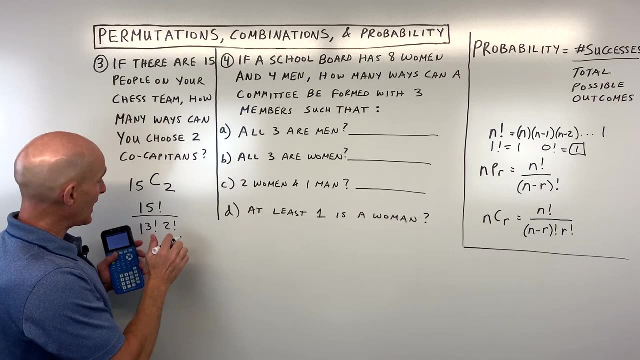 formula: here we've got 15 factorial over N minus R. So 15 minus two is 13 factorial, two factorial. Now again, remember, the two factorial is dividing out A and B, B and A. Those are the same two people. So if we simplify this down, you can do this by hand: 15 factorial. 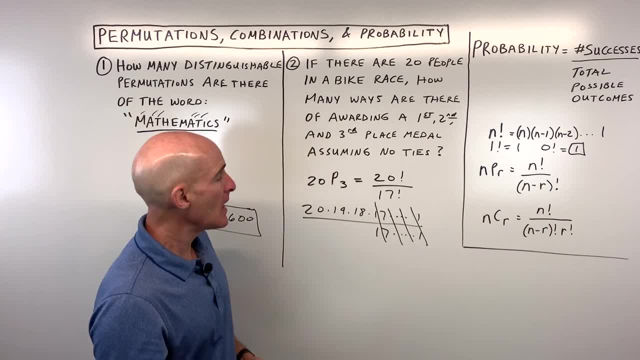 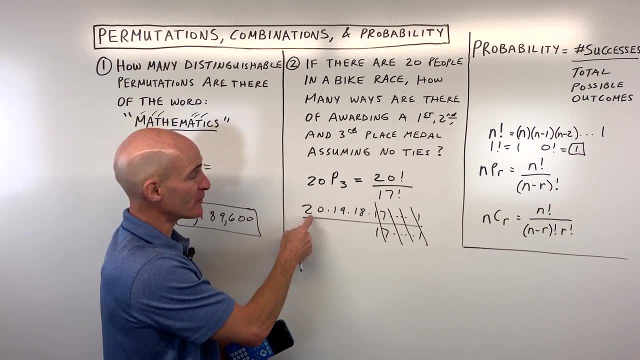 counting principle or the fundamental counting principle, And what you do is you say: how many choices are there for, like, a first place finisher? There's 20 ways that somebody could finish first. Once that person finishes first, how many different people could finish for the second medal? 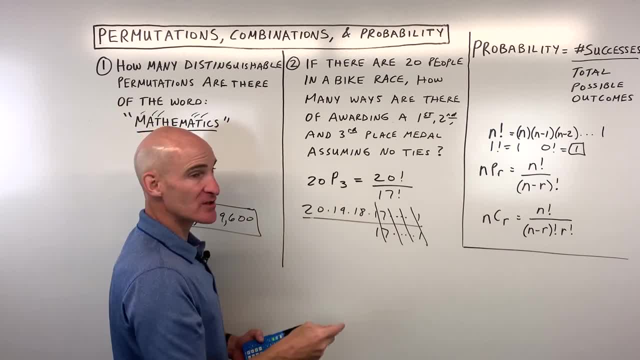 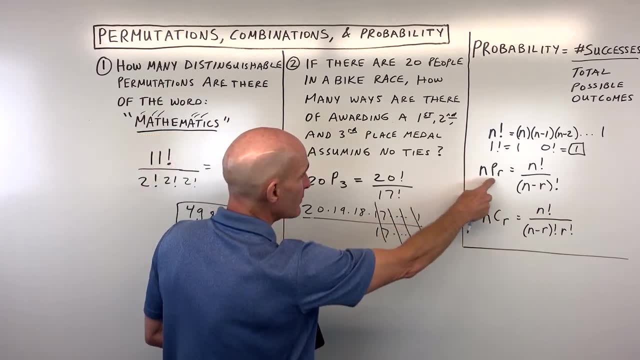 That would be 19.. And once those two people finish, how many ways are there for a third place, finisher 18.. So you can use this fundamental counting principle or you can use this NPR formula for this example. So let's multiply that out and see. 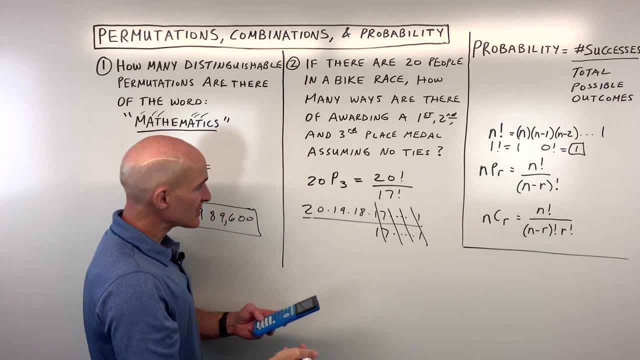 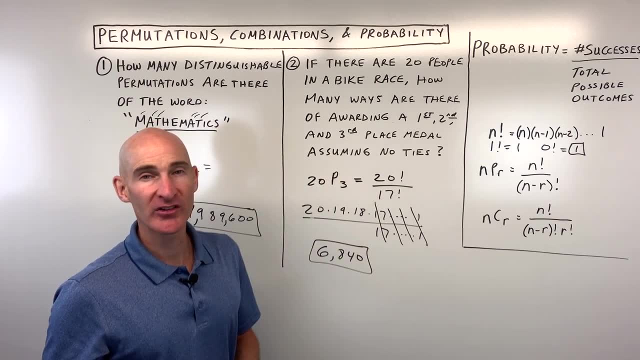 what we get. So you can use this NPR formula for this example. So let's multiply that out and see what that comes out to. Okay, this is coming out to 6,840 different ways to award those three medals. Okay, if you want to test yourself on some of these problems, go ahead and pause the video. 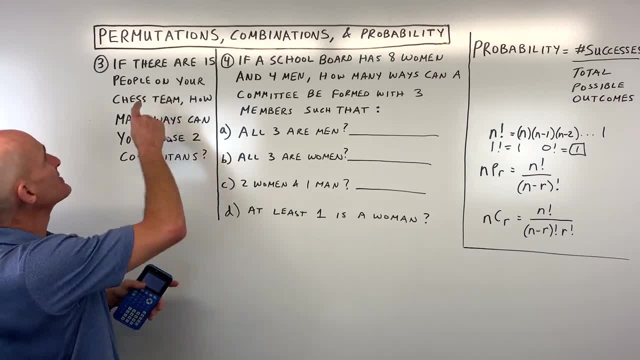 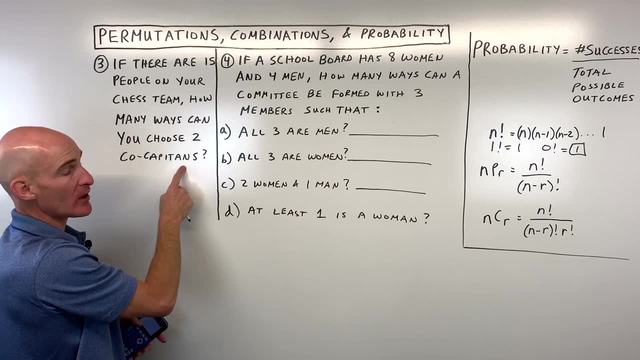 and see if you can do them on your own. But let's dive into number three. It says: if there are 15 people on your chess team, how many ways can you choose two co-captains? So what do you think about that one? Well, what's interesting is, do you think? 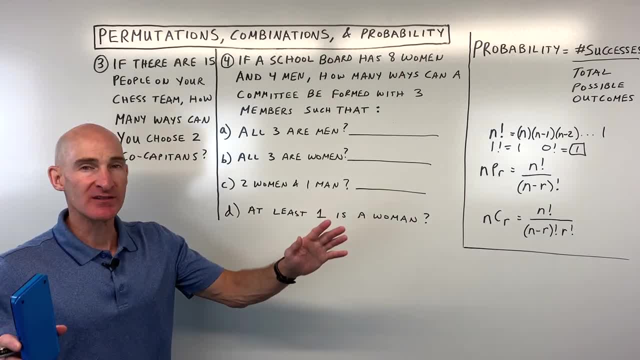 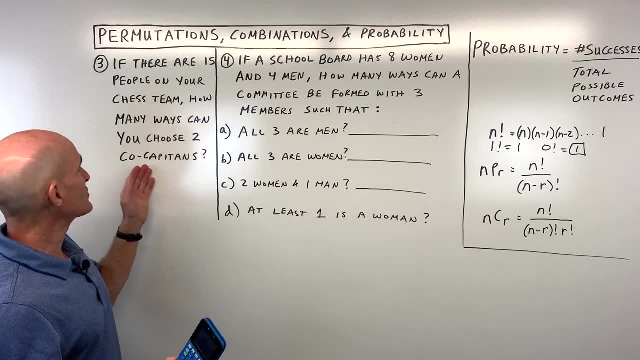 that the order is important. Like if they pick Joe first and Sally second, or Sally first and Joe second, Like does the order matter? Well, in this case, because they're co-captains. it's not like the bike race, one where, like gold, silver, bronze, like you, would get a different medal. 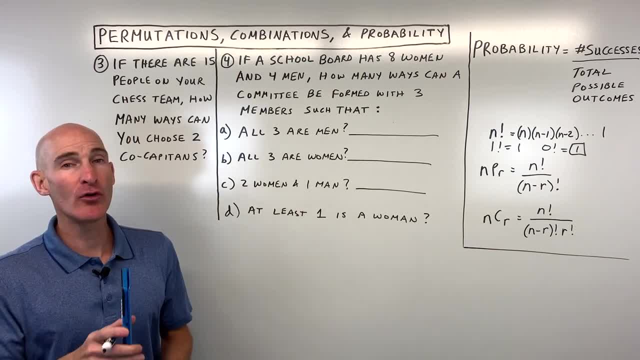 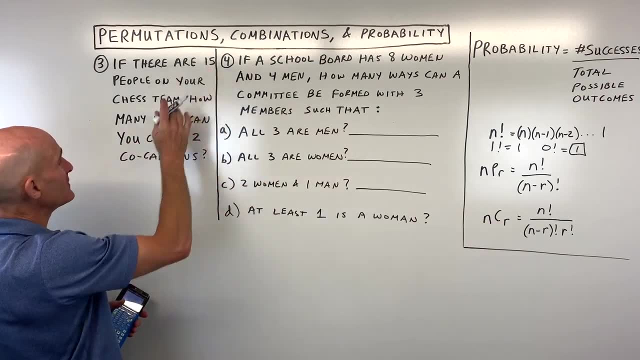 In this case they're co-captains, So it doesn't matter. A and B, B and A, they both made it into being co-captains. The order doesn't matter, You want to use combinations. So here we're saying: out of 15 chess members, how many ways are there? 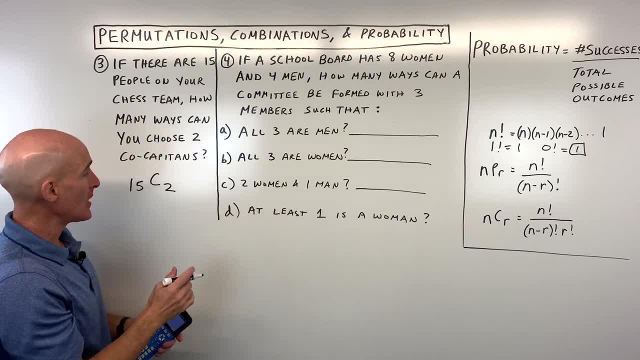 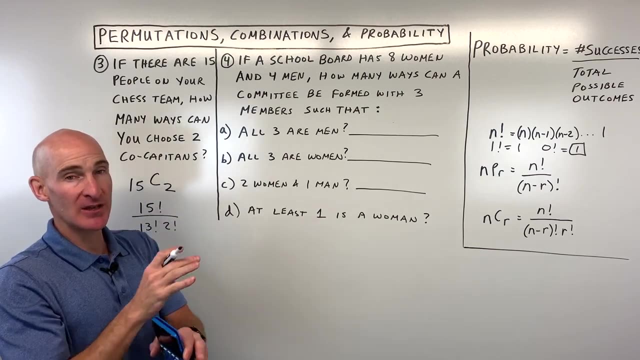 of choosing two, where the order doesn't matter. So using our formula here we've got a 15 factorial over n minus r. So 15 minus 2 is 13 factorial, 2 factorial. Now again, remember, the 2 factorial is dividing out a and b. b and a, Those are the same two people. 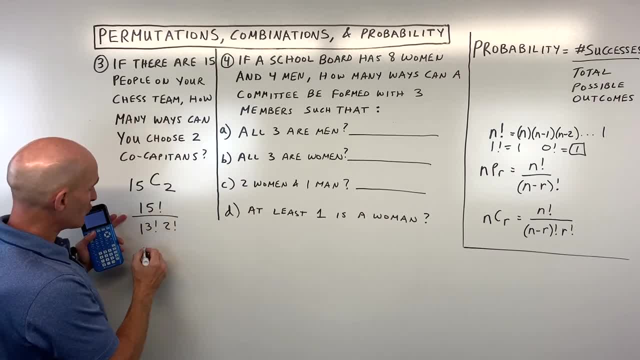 So if we simplify this down, you can do this by hand: 15 factorial is 15 times 14 times 13,, all the way down to 1.. Okay, which you could just write this as 13 factorial. That's going to cancel with this 13 factorial: 13,, 12,, 11,, all the way down to 1.. And then 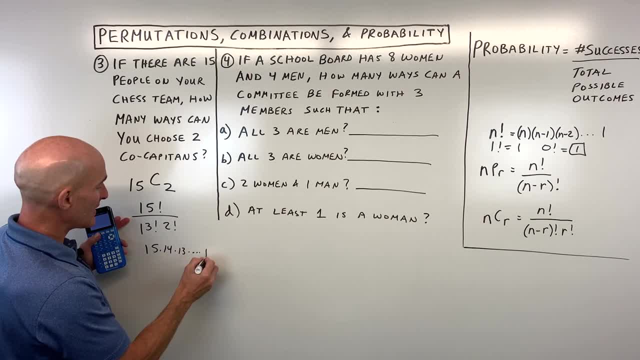 is 15 times 14 times 13.. All the way down to one, Okay, which you could just write this as 13 factorial. That's going to cancel with this 13 factorial, 13,, 12,, 11,, all the way down to one And then two. factorial is just. 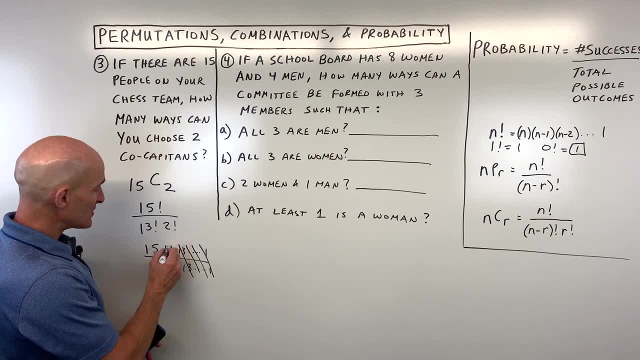 two times one, 14 divided by two, we can reduce that to seven. And 15 times seven is 105. divided by one is just 105.. So there's 105 different ways to choose those two co-captains out of the 15. 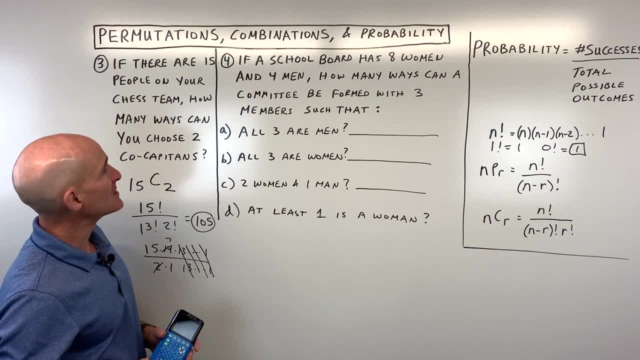 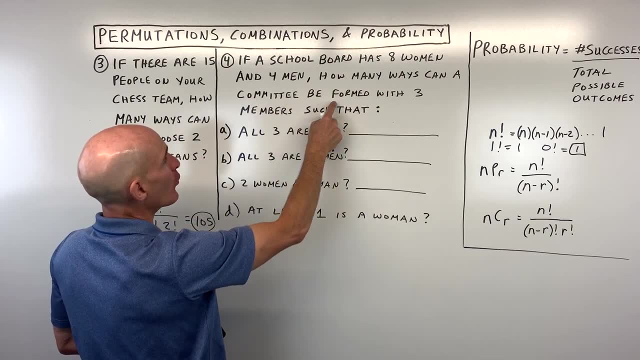 chess members. Okay, so for number four, see if you can do this one. It says: if a school board has eight women and four men, how many ways can a committee be formed with three members such that all three are men or all three are women or 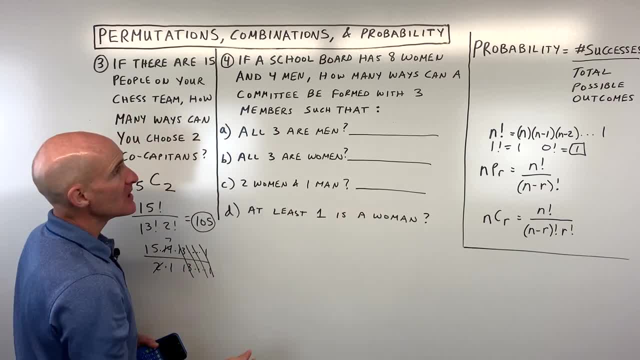 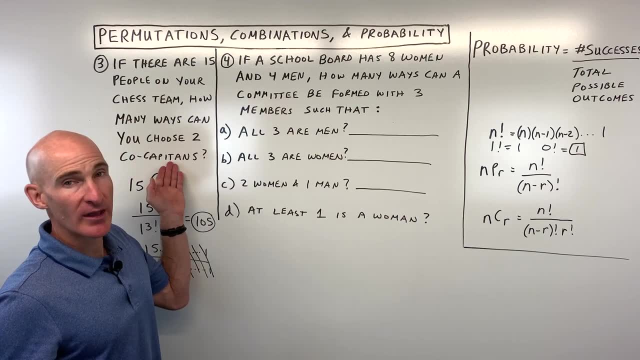 two are women and one's a man and at least one is a woman, So we've got a multi-part question here. Now, when you see the word committee, it's very similar to what we did with the co-captain. So the order it's not important, right? Because it's not like there's a president, vice president. 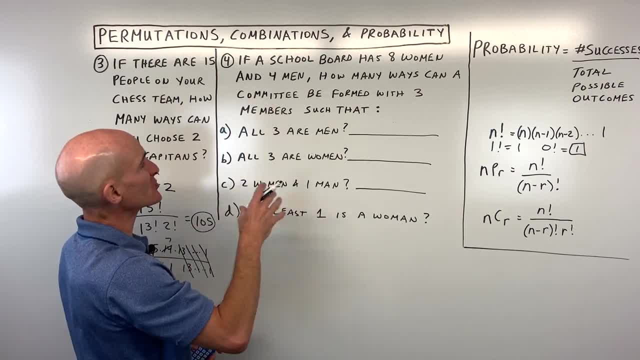 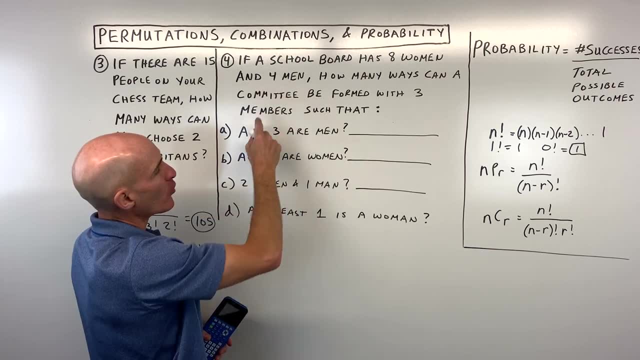 secretary, treasurer, like that, Order is not important. when it's a committee They're just all together. So it says: all three are men. So we know that there's four men and the order doesn't matter. So we're saying out of 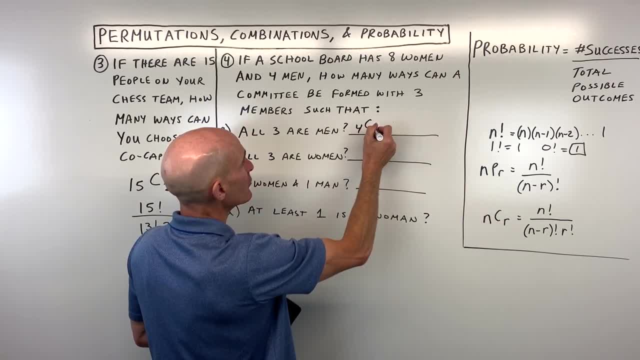 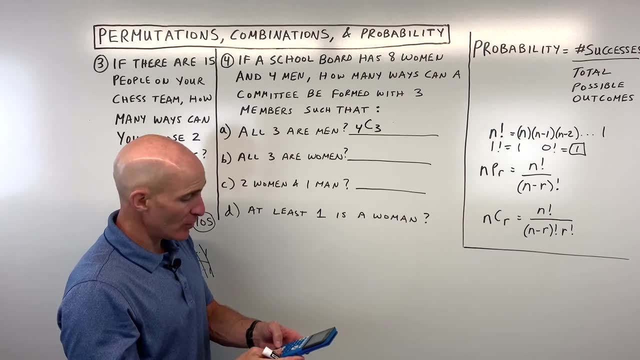 four, how many ways are there of choosing three? So we would say 4C3.. Now on your calculator there should be a combination button also underneath that probability menu. So I'm going to do that on the calculator. I'm also going to show you how to do it by hand, in case you can't. 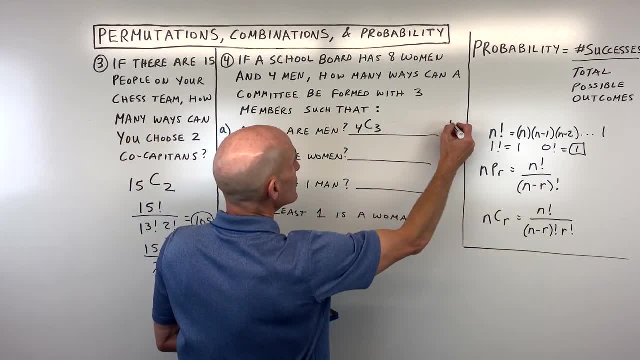 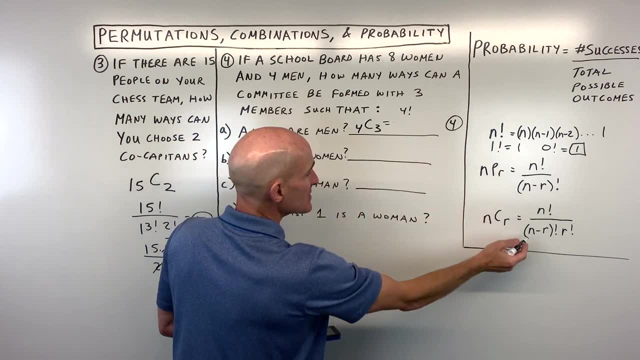 use a calculator, This is coming out to four. So let's just write that down, And then we're going to do that here Now. 4C3, using our formula, this is going to be 4 factorial over 4 minus 3, see n minus. 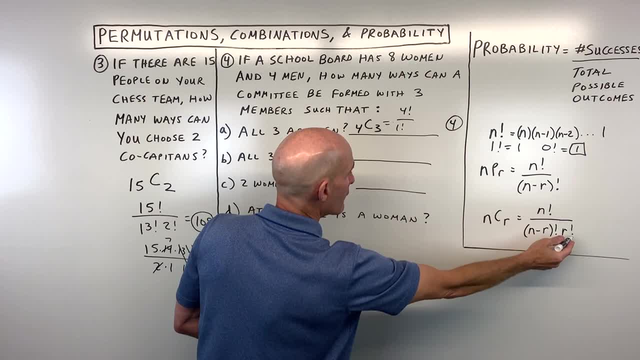 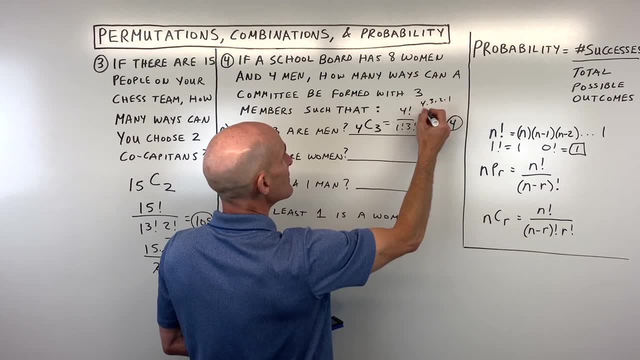 r, which is 1 factorial, and r factorial, which is 3 factorial. Now 4 factorial is 4 times 3 times 2 times 1.. 1 times 3 factorial is just 3 factorial, So that's 3 times 2 times 1.. And you can see. 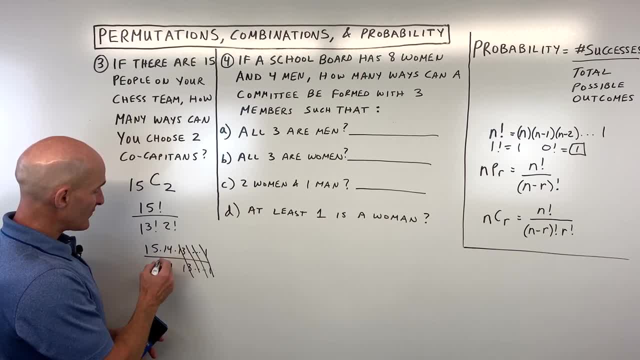 2 factorial is just 2 times 1.. 14 divided by 2, we can reduce that to 7.. And 15 times 7 is 105, divided by 1 is just 105.. So there's 105 different ways to choose those two co-captains. 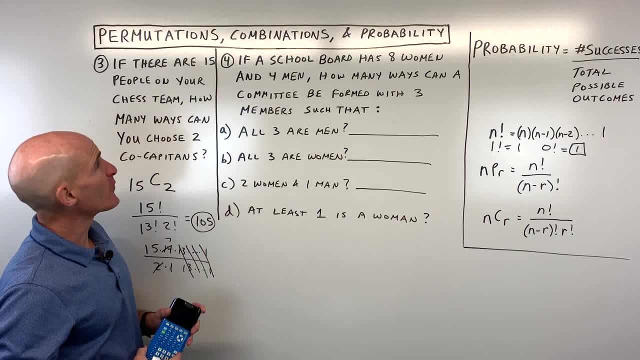 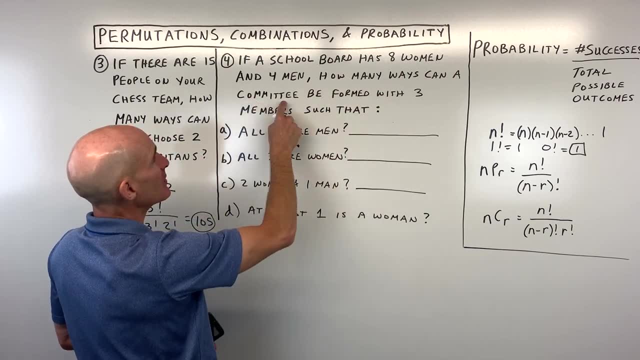 out of the 15 chess members. Okay, so for number 4, see if you can do this one. It says: if a school board has 8 women and 4 men, how many ways can a committee be formed with 3 members such that all 3 are men or all 3 are women? 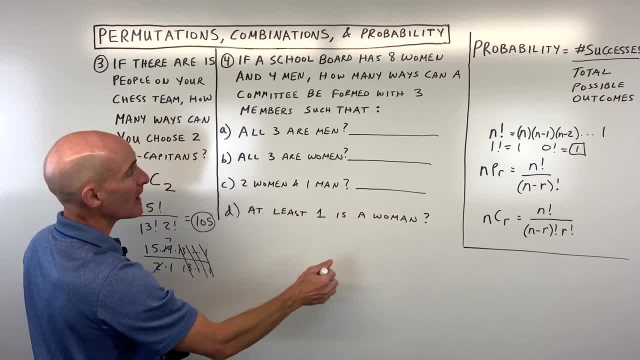 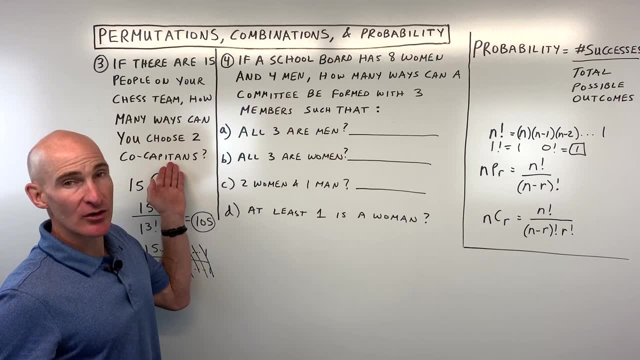 or 2 are women and 1 is a man and at least 1 is a woman. So we've got a multi-part question here Now. when you see the word committee, it's very similar to what we did with the co-captain. So 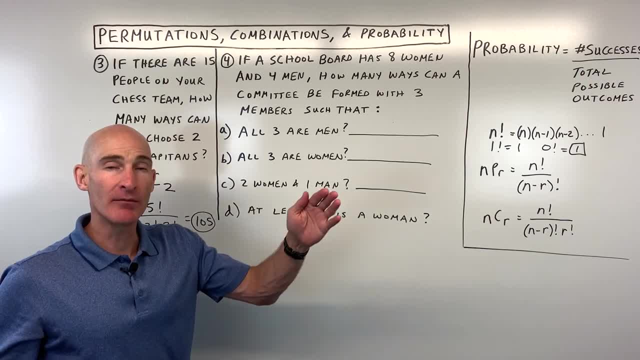 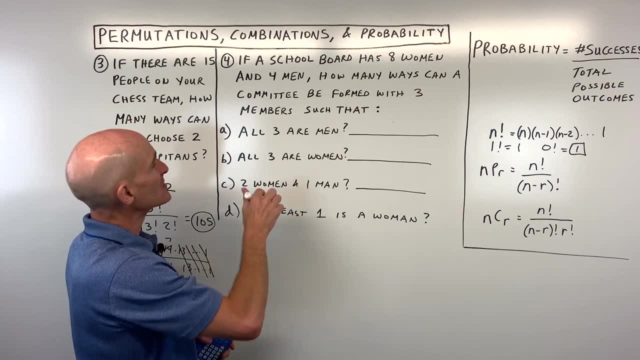 the order. it's not important, right? Because it's not like there's a president, vice president, secretary, treasurer, like that. The order is not important. when it's a committee, They're just all together. So it says. 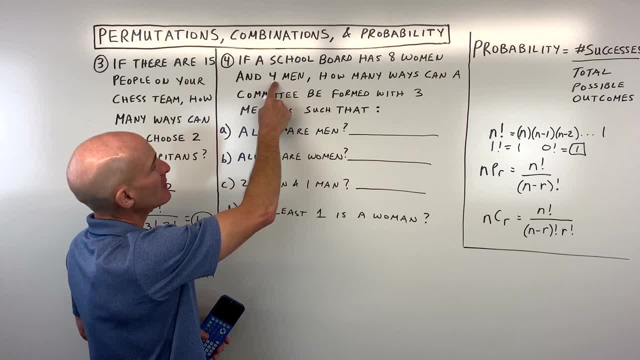 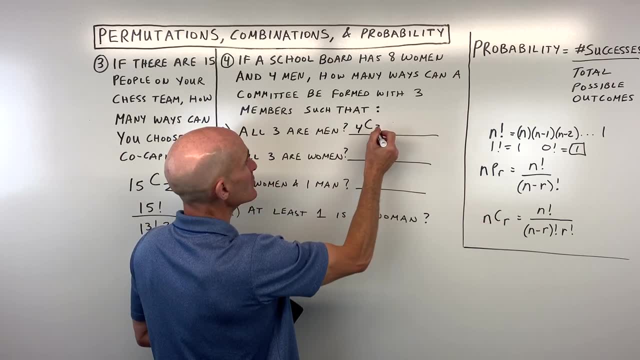 all 3 are men. So we know that there's 4 men and the order doesn't matter. So we're saying: out of 4, how many ways are there of choosing 3?? So we would say 4c3.. Now on your calculator. 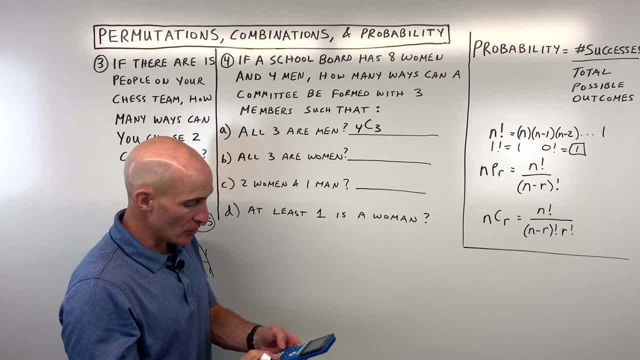 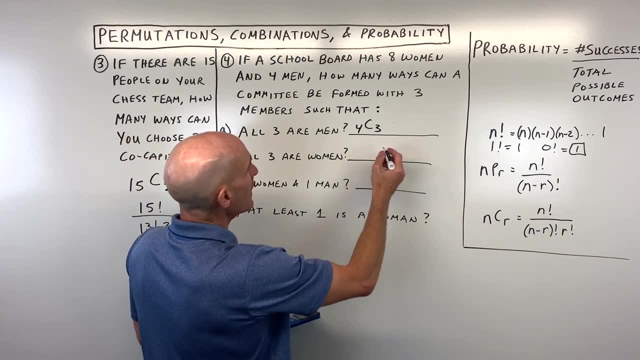 there should be a combination button also underneath that probability menu. So I'm going to do that on the calculator. I'm also going to show you how to do it by hand, in case you can't use a calculator. This is coming out to 4.. So let's just write that here Now: 4c3, using our formula, this is going to be 4 factorial. 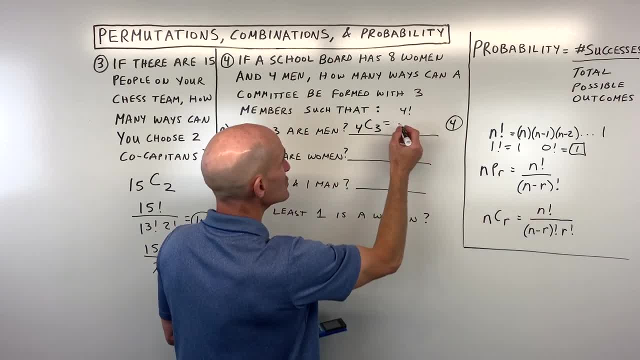 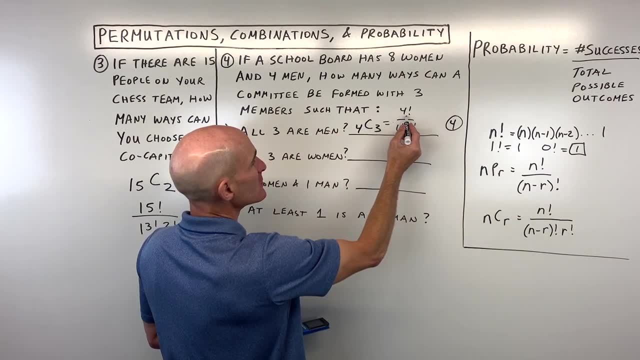 Over 4 minus 3, see n minus r, which is 1 factorial, And r factorial, which is 3 factorial. Now 4 factorial is 4 times 3 times 2 times 1.. 1 times 3 factorial is just 3 factorial. So 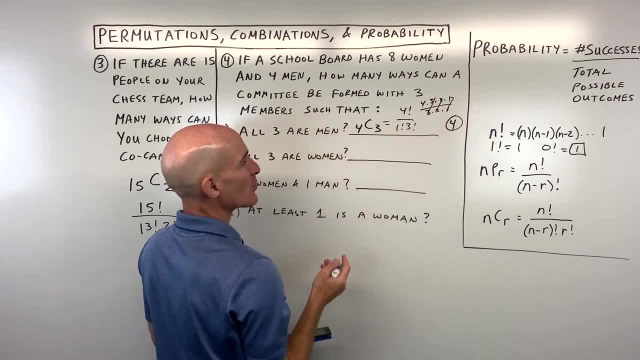 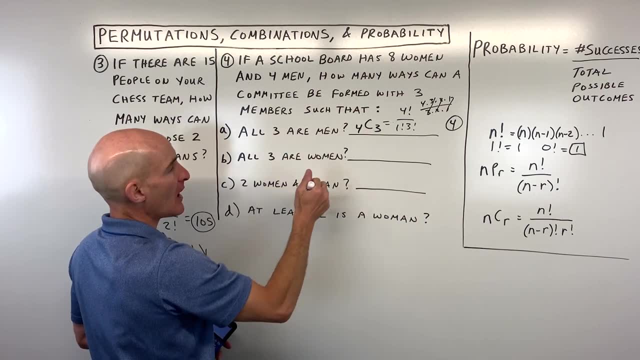 that's 3 times 2 times 1. And you can see that's how we're getting 4.. So let's go to number uh, letter b: here All 3 are women. Well, we know there's 8 women and we want to find out how many ways of choosing 3?. 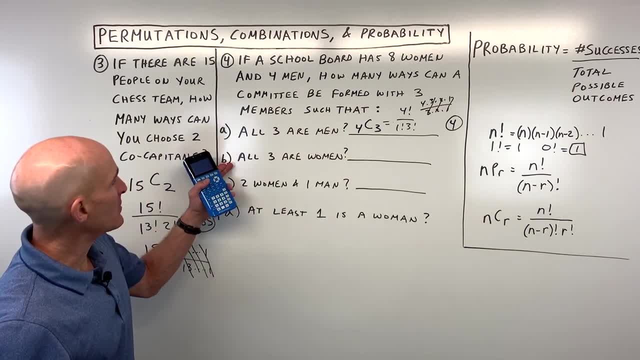 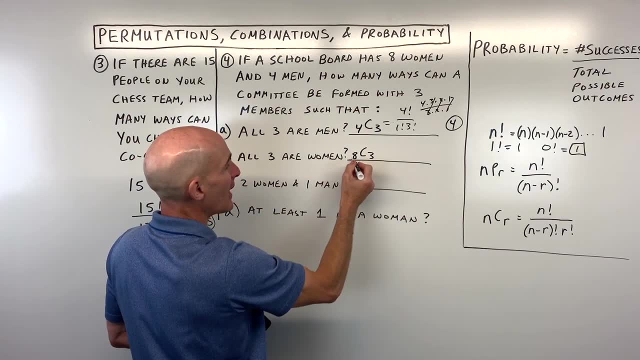 that's how we're getting 4.. So let's go to letter B. here All three are women. Well, there's eight women And we want to find out how many ways of choosing three women out of those eight where the order is not important. So it's a combination, So same idea. We're going to do. 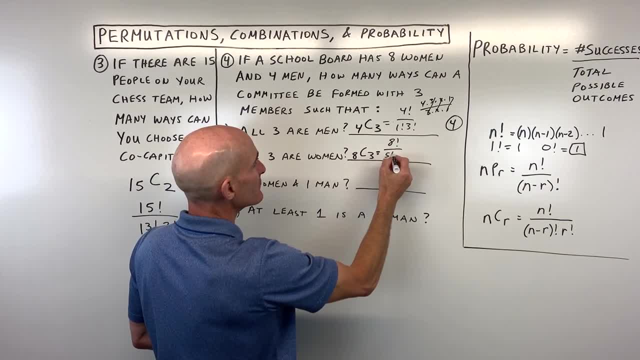 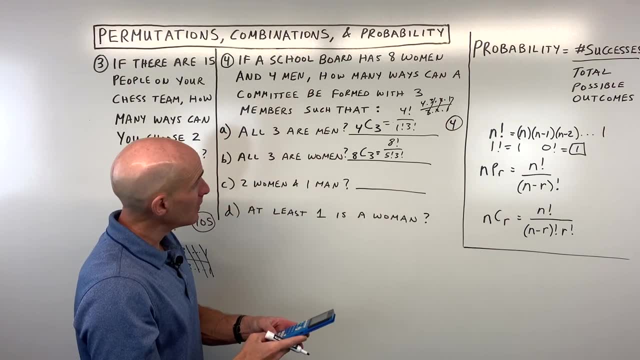 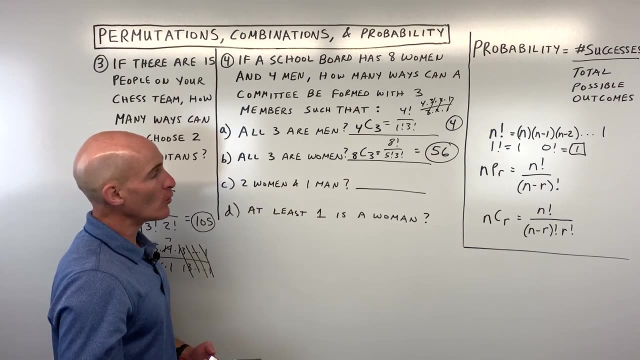 8 factorial. over 8 minus 3 is 5 factorial, 3 factorial. If you simplify that down, let's see what we get: 56.. And for letter C, two are women and one's a man, So this one's a little. 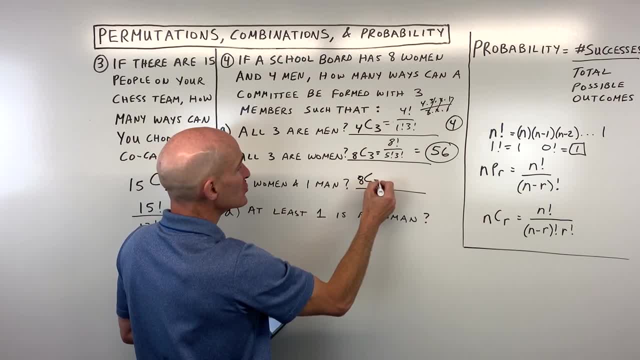 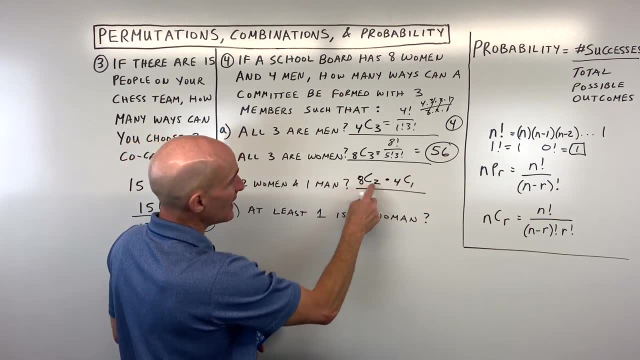 different because out of the eight women we're saying, how many ways are there to choose two times? out of the four men, how many ways are there of choosing one? Now you'll notice, the eight and the four add up to 12, the 12 people on the board, and the two and the one add up to. 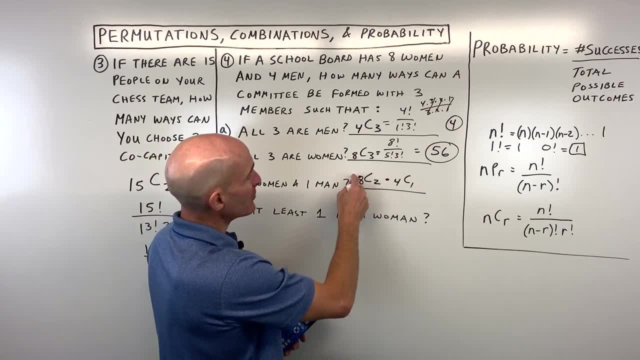 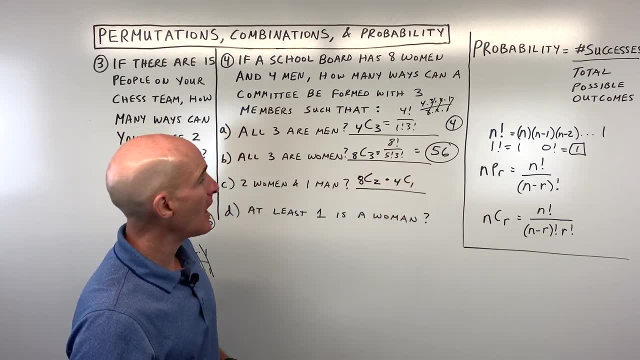 three members on the committee And we're making use of that fundamental counting principle. We're saying, how many ways are there to choose the women, how many ways are there to choose the one man, and we're multiplying them together to get the total possible outcomes. So let's see what this 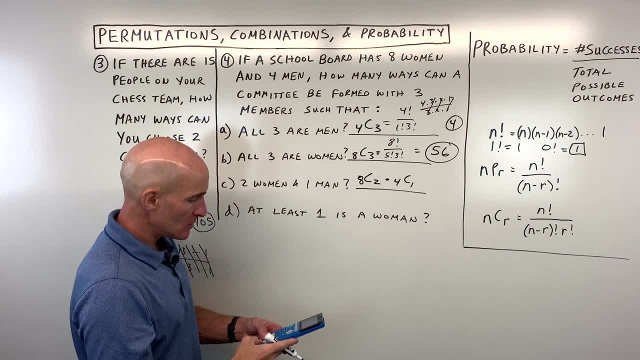 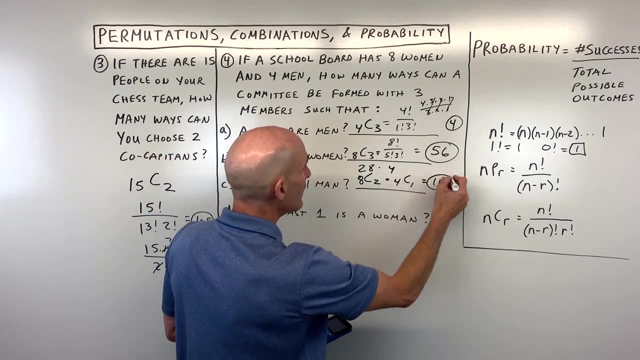 comes out to So eight. combination two is 28, and four. combination one is four, And if we multiply those together we get 112.. So 112 outcomes there, And for the last one, this one's a little bit different At. 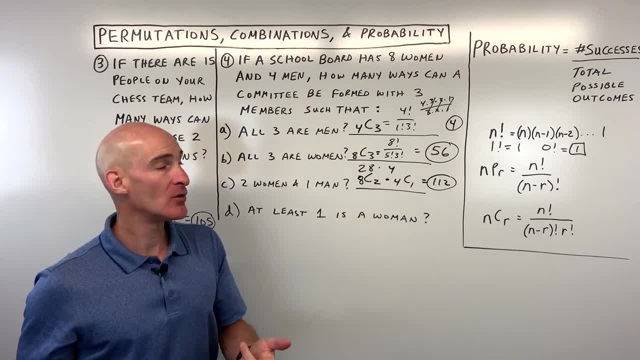 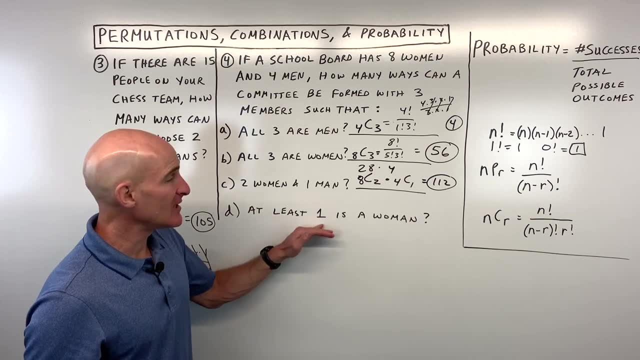 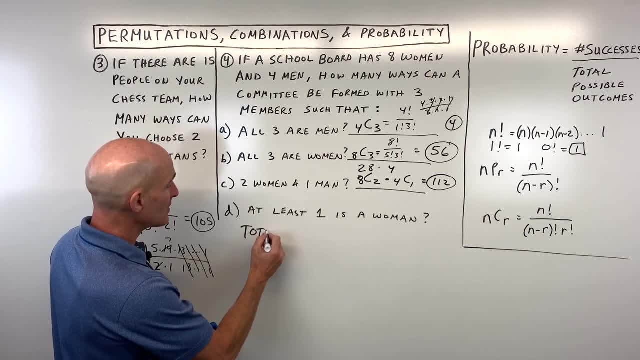 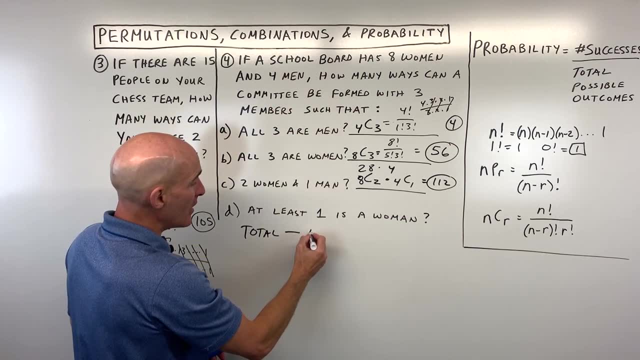 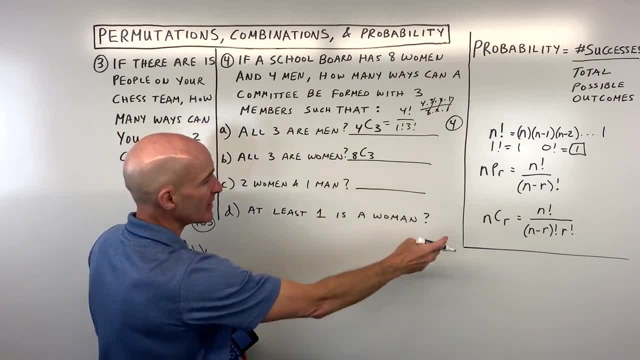 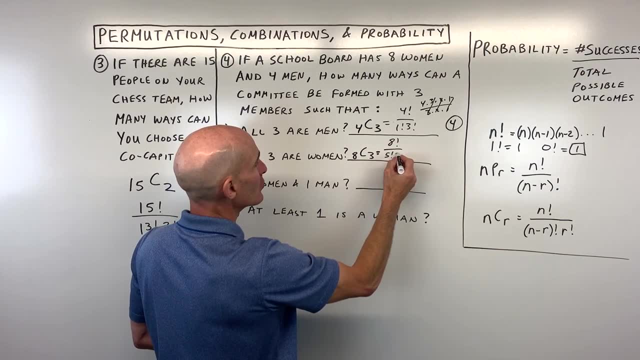 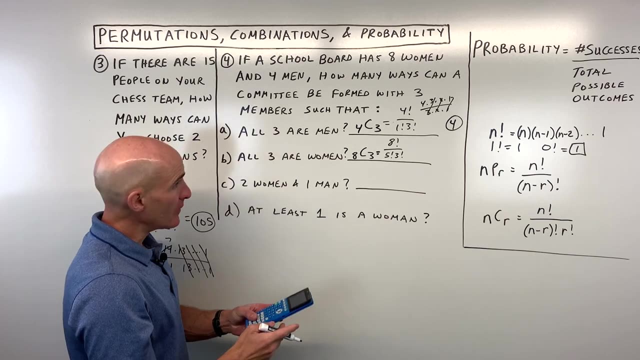 women out of those eight where the order is not important. so it's a combination. So same idea. we're going to do 8 factorial over 8 minus 3 is 5 factorial, 3 factorial. If you simplify that down, let's see what we get. 56 and for letter: 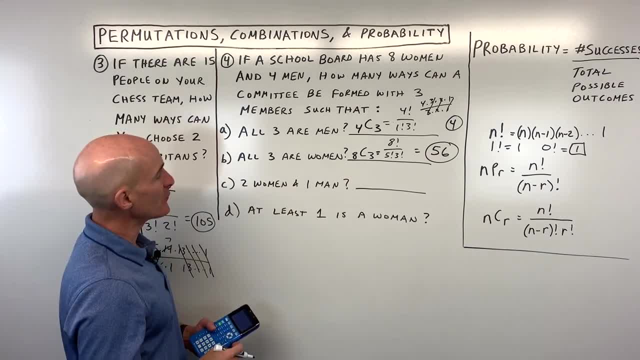 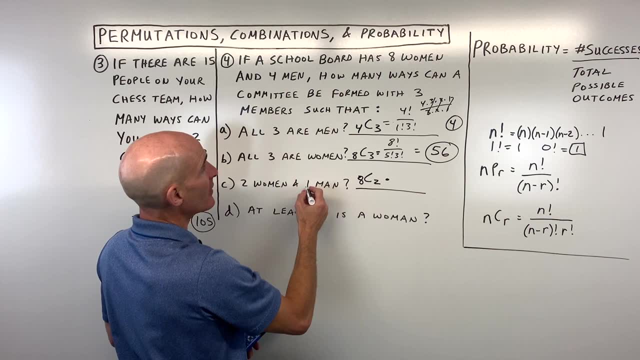 C, two are women and one's a man. So this one's a little bit different, because out of the eight women we're saying, how many ways are there to choose two times? out of the four men, how many ways are there of choosing one? Now you'll notice. 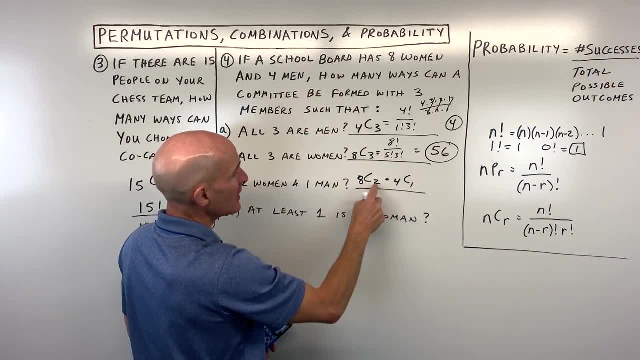 the eight and the four add up to 12- the 12 people on the board, and the two and the one add up to three members on the committee. and we're making use of that fundamental counting principle. We're saying how many ways are there to choose? 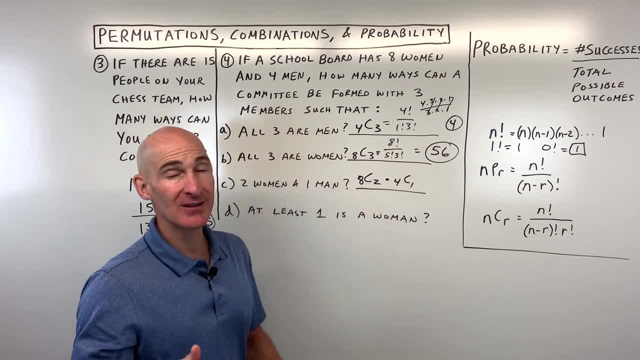 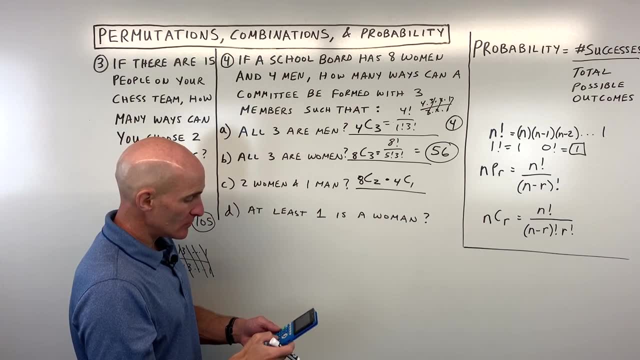 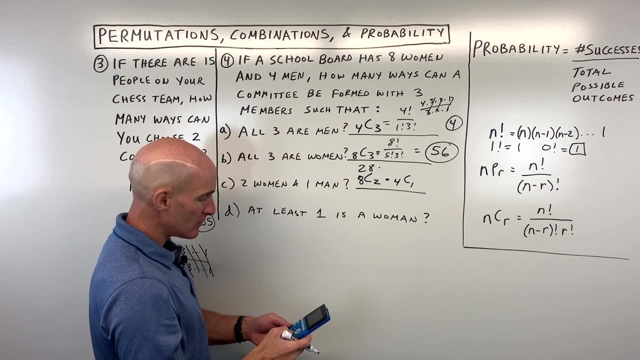 the women. how many ways are there to choose the one man? and we're multiplying together to get the total possible outcomes. So let's see what this comes out to. So eight combination two is 28 and four combination one is four, and if we multiply those together we get 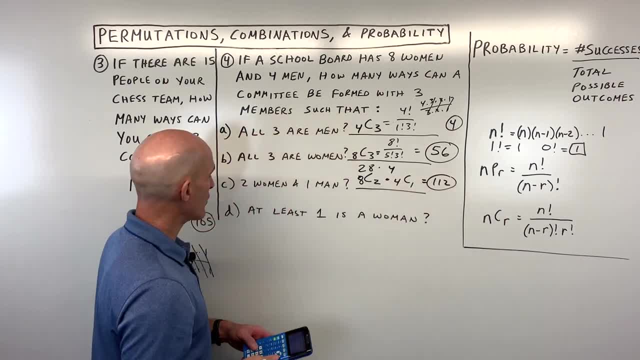 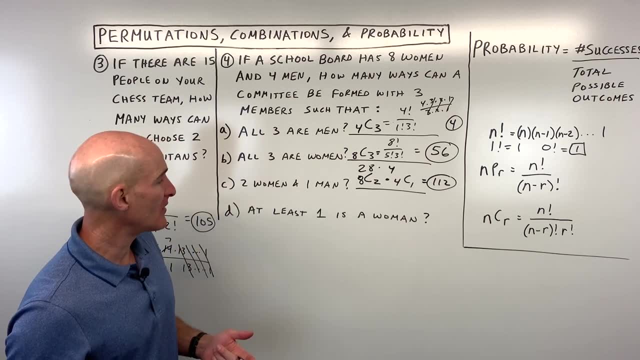 a hundred and twelve, So 112 outcomes there. and for the last one- this one's a little bit different. at least one is a woman, So that means one could be a woman, two could be two women on the committee, or all three women could be on the. 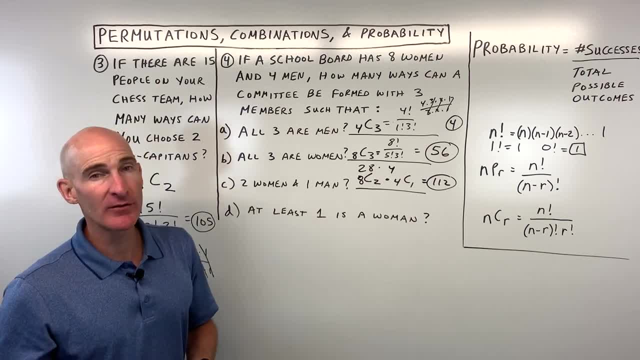 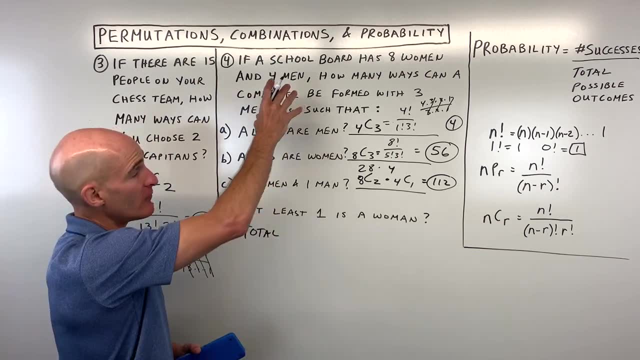 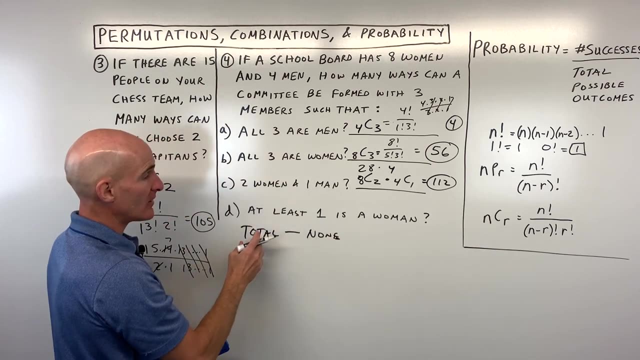 committee. So when you see at least one, there's a little bit of a trick here that you can do. you can take the total number of ways of choosing three members. okay, out of the 12 members minus that, none are women. okay, so at least one is the total minus none, and that'll give you. 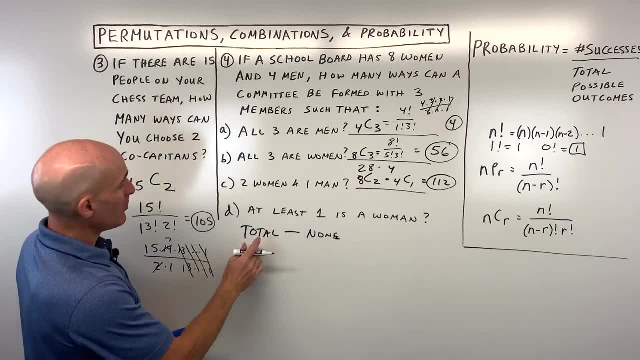 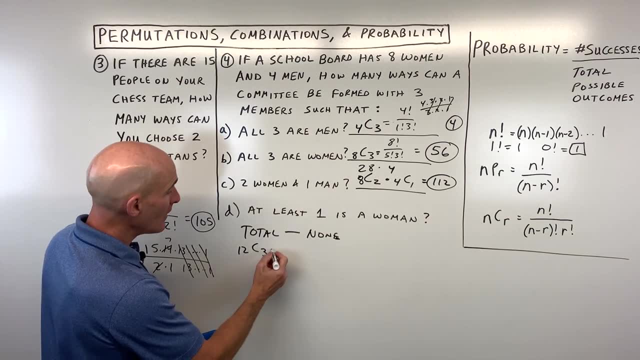 one or two or three women on the committee, so the total would be 12 c3 out of 12 members. how many ways are there to choose a committee of three members minus none are women? now, none are women. that was like saying that all three of them were men, which there was four ways there. and so let's. 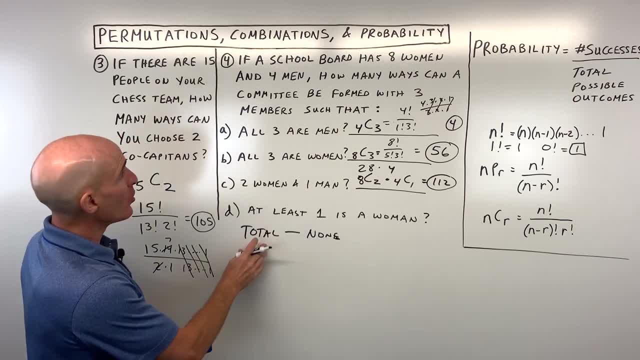 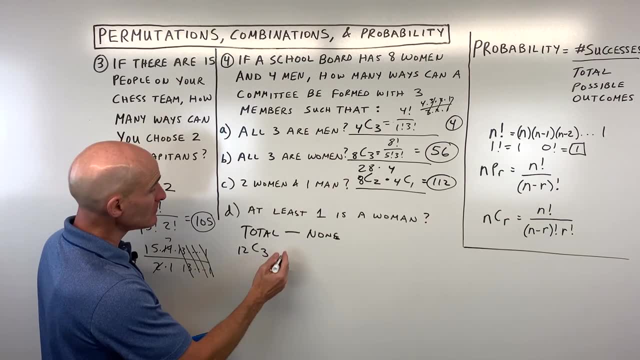 will give you one or two or three women on the committee, so the total would be 12 c3 out of 12 members. how many ways are there to choose a committee of three members minus none are women? now, none are women. that was like saying that all three of them were men, which there was four ways. 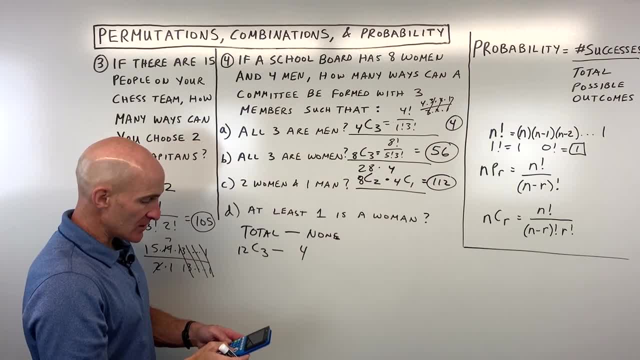 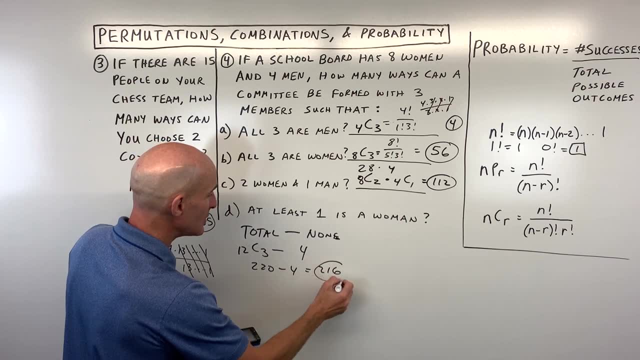 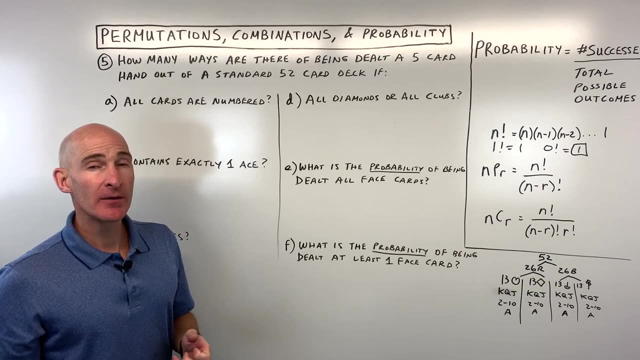 there. and so let's see what 12 combination 3 is, that's 220 minus 4 is 216, ways that there could be at least one woman, one woman, on this committee. okay, for number five. we're going to be dealing with some standard deck of playing cards, and you might be saying, Mario, I'm not a card player. 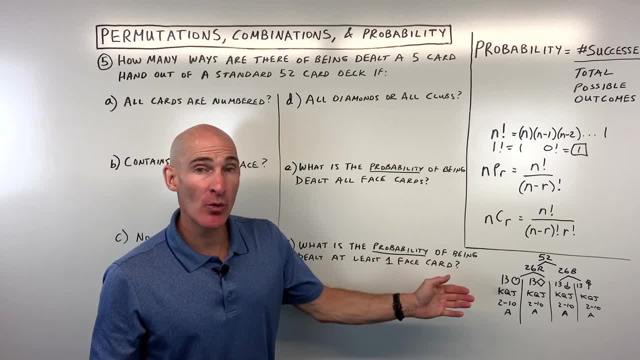 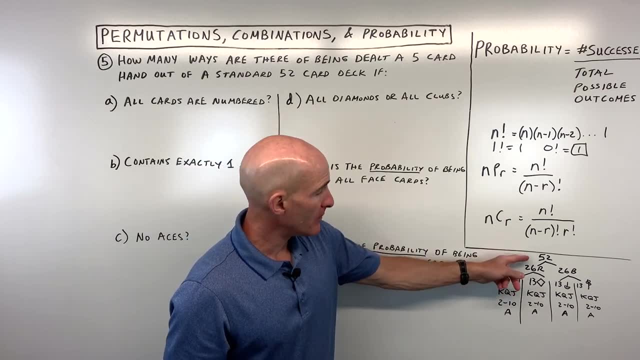 don't worry, I'm not a card player either. but the thing you want to do is you want to remember and you might want to write this down- is what is the breakdown of a standard 52 card deck? well, of the 52 cards, half are red and half are black. so 26 red, 26 black. of the red cards, they're. 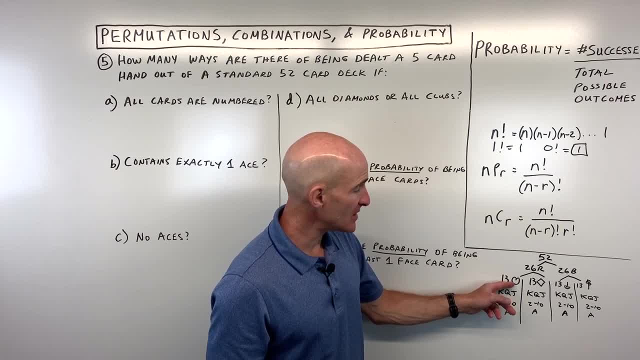 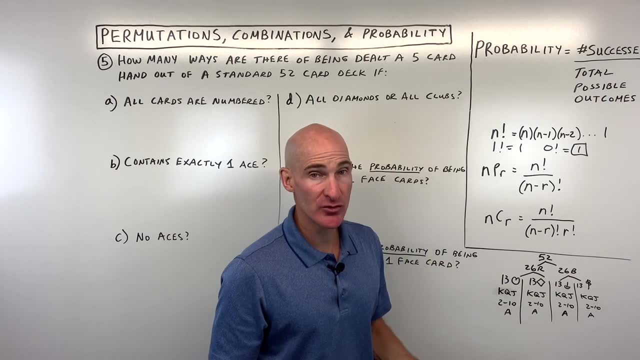 divided up into what we call suits. so there's 13 hearts and 13 diamonds. those are red, okay, whereas over here there's 13 spades and 13 clubs. those are black. so half red, half black. four suits, and then, underneath each suit, you've got a card deck and a card deck and a card deck and a card deck. 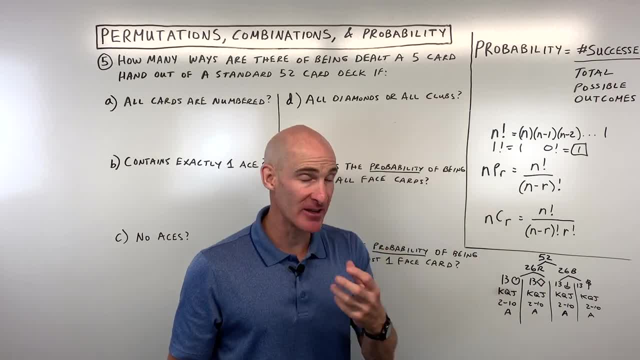 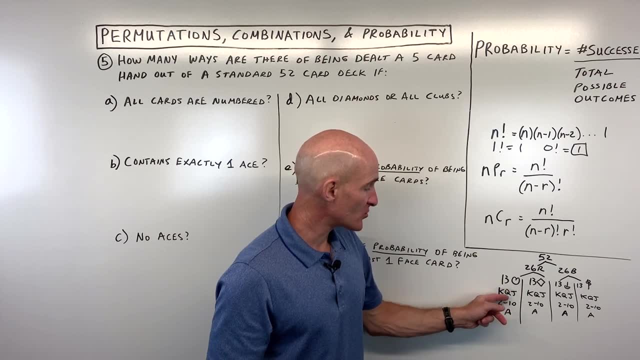 you've got a face card of a king queen and jake jack. they have a face on it, king queen jack, and that's in each of the suits. and then there's a numbered cards in each suit, so there's a two of hearts, three of hearts, all the way through 10 of hearts. same thing with the diamonds, two through. 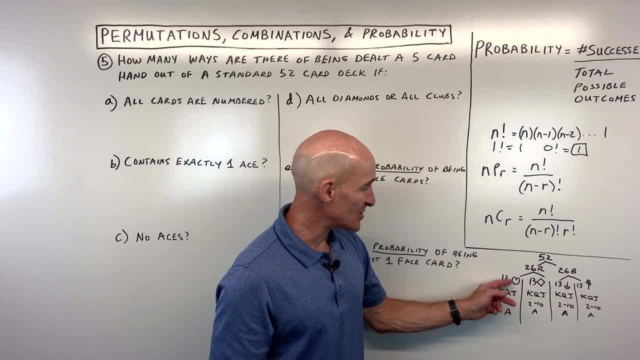 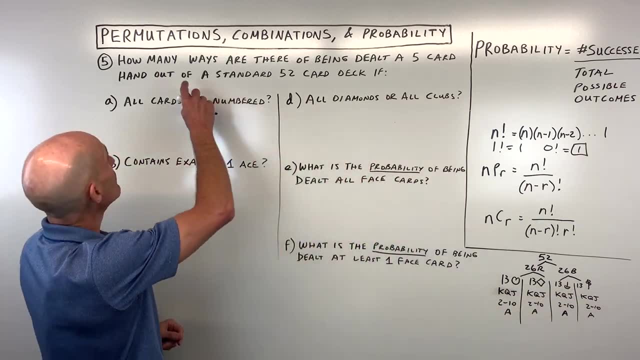 10. those are the numbered cards, and then you've got an ace in each suit. so an ace of hearts, ace of diamonds, ace of spades, ace of clubs. so that's the breakdown. so let's see if we can do some problems here. so it says how many ways are there of being dealt a five card hand. 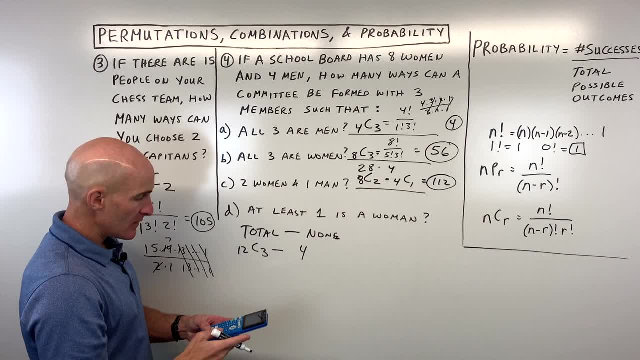 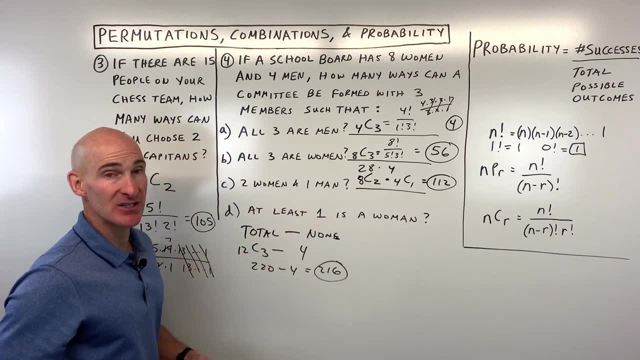 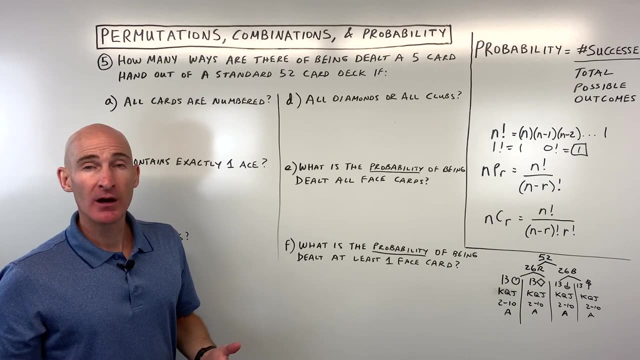 see what 12 combination three is, that's 220 minus 4 is 216, ways that there could be at least one woman, one woman, on this committee. okay, for number five. we're going to be dealing with some standard deck of playing cards and you might be saying, Mario, I'm not a card player, I don't worry, I'm. 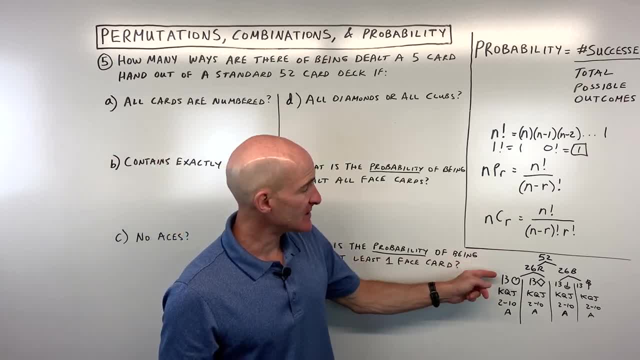 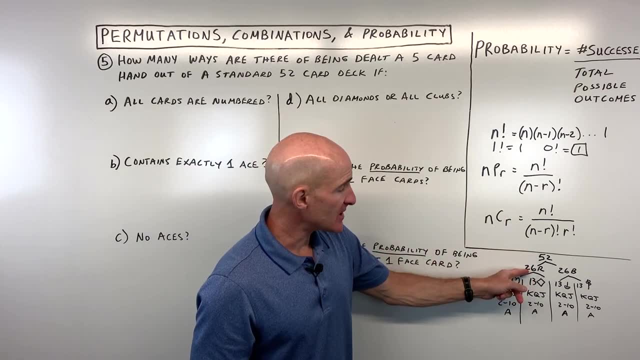 not a card player either, but the thing you want to remember, and you might want to remember, is that you're not a card player. you're not a card player. you're not a card player. want to write this down is: what is the breakdown of a standard 52 card deck? Well, of the 52 cards, 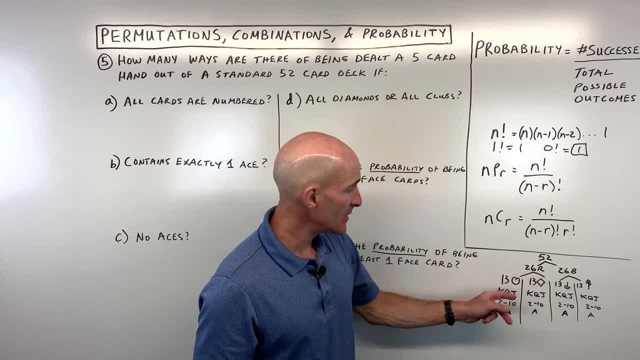 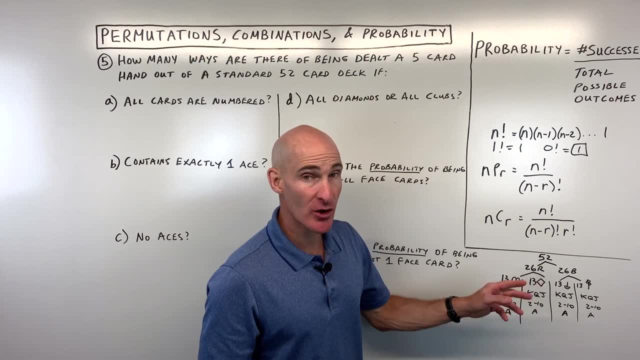 half are red and half are black, So 26 red, 26 black. Of the red cards. they're divided up into what we call suits, So there's 13 hearts and 13 diamonds. Those are red, Okay, Whereas over here, 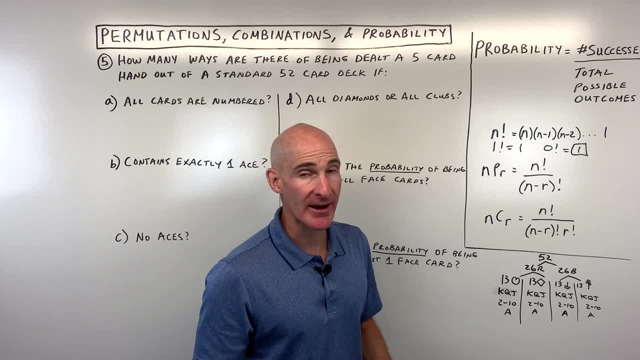 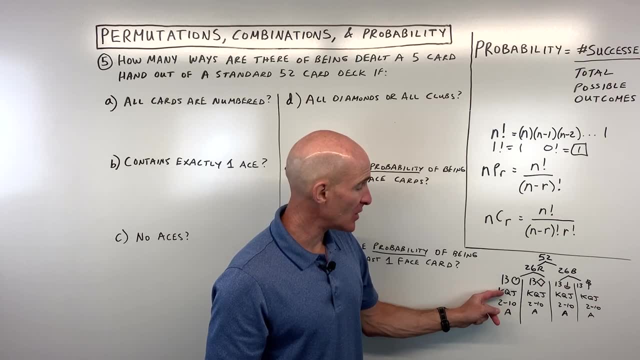 there's 13 spades and 13 clubs. Those are black. So half red, half black. four suits And then underneath each suit you've got a face card of a king, queen and jack. They have a face on it. 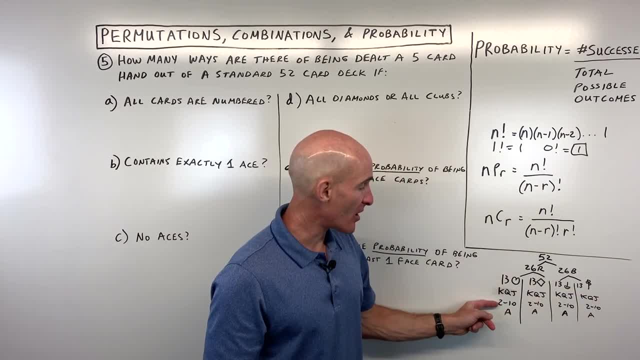 king, queen jack, and that's in each of the suits. And then there's a numbered cards in each suit, So there's a, two of hearts, three of hearts, all the way through 10 of hearts. Same thing with the. 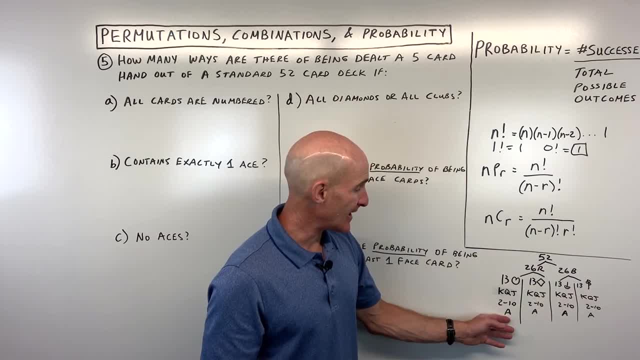 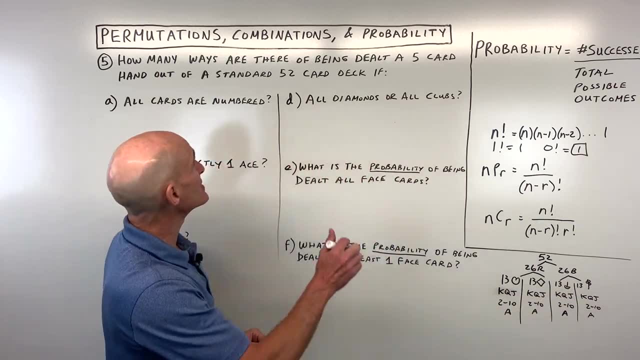 diamonds, two through 10.. Those are the numbered cards, And then you've got an ace in each suit. So an ace of hearts, ace of diamonds, ace of spades, ace of clubs. So that's the breakdown. So let's see if we can do some problems here. So it says how many ways are there of being dealt a. 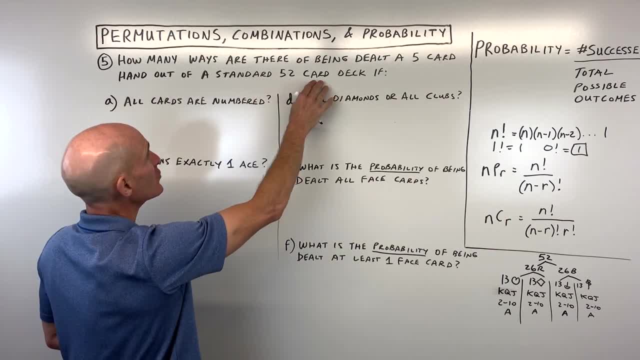 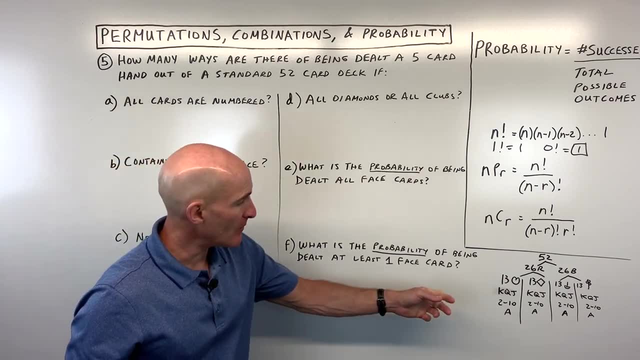 five card deck. How many ways are there of being dealt a five card hand out of a standard 52 card deck if all cards are numbered? So what you would do is you'd say, well, hmm, how many numbered cards are there? Well, it looks like. 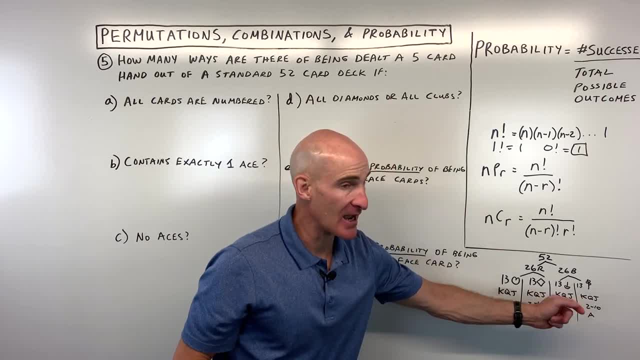 there's two through 10.. That's nine, nine, nine. nine Nine times four is 36.. So there's 36 cards in the deck that have a number on it And we want to know how many ways there are being dealt. 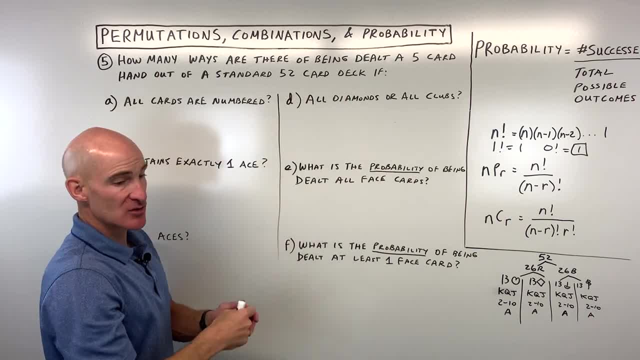 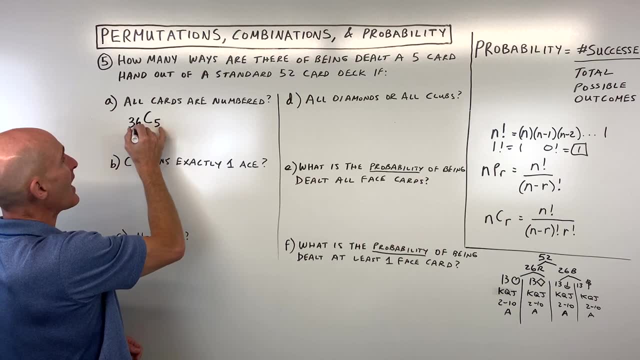 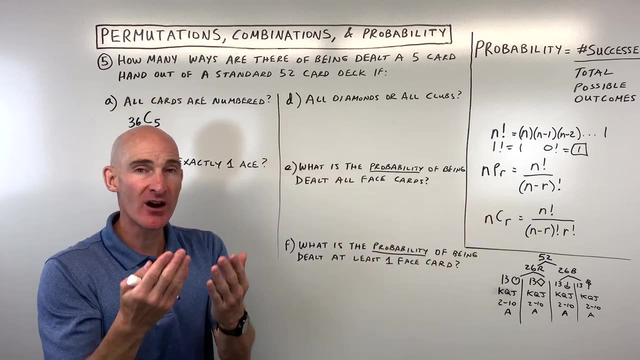 five of those cards. Okay, So you're dealt a hand And so that would be out of 36, how many ways are there of choosing five out of that 36?? Okay, The numbered cards. Now we're using combinations because the order doesn't matter: When you're dealt those cards, when you're in your 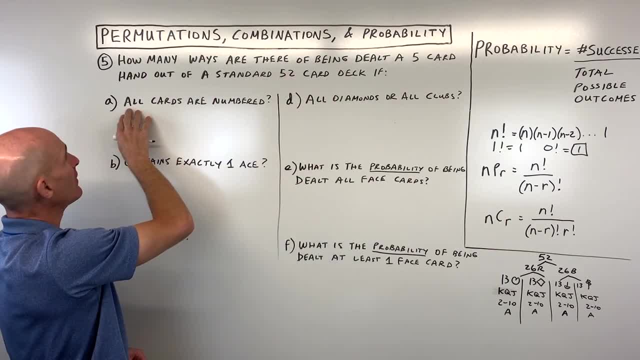 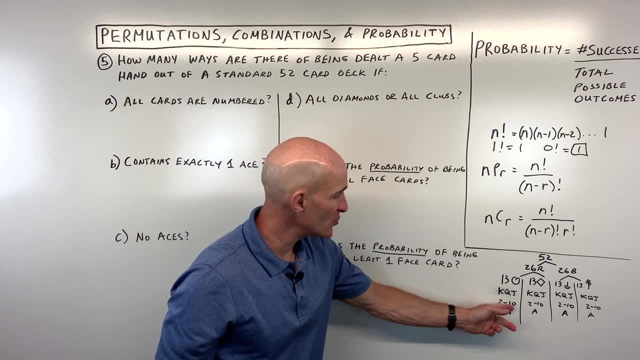 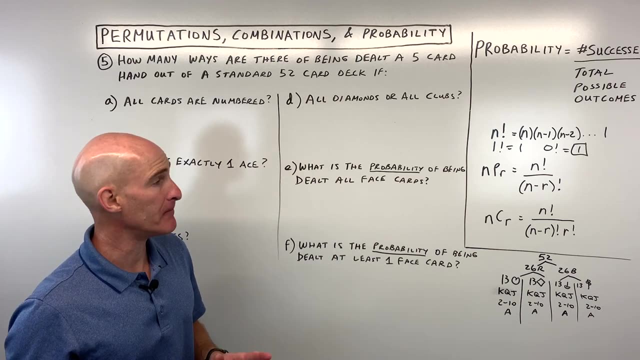 out of a standard 52 card deck if all cards are numbered. so what you would do is you'd say: well, hmm, how many numbered cards are there? well, it looks like there's two through ten, that's nine, nine, nine, nine nine times four is 36. so there's 36 cards in the deck that have a number on it. 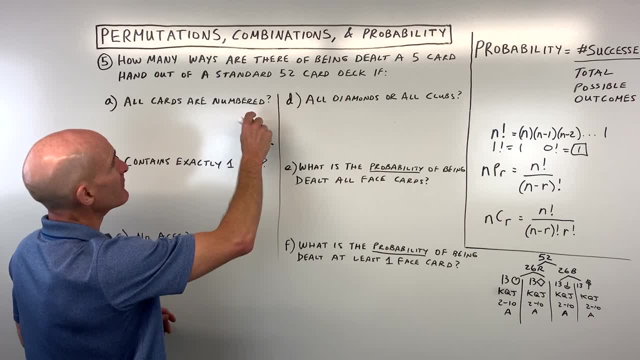 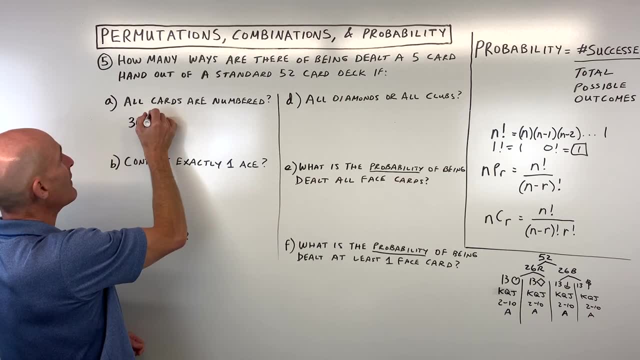 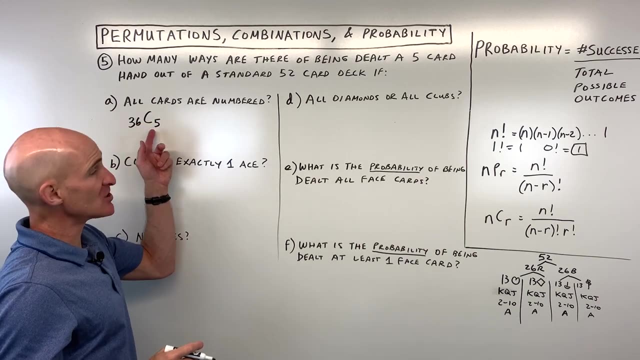 and we want to know how many ways there are being dealt um five of those cards. okay, so you're dealt a hand, and so that would be out of 36. how many ways are there of choosing five out of that 36? okay, the numbered cards. now we're using combinations because the order 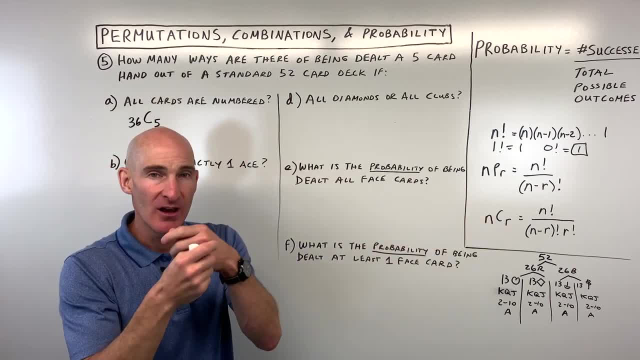 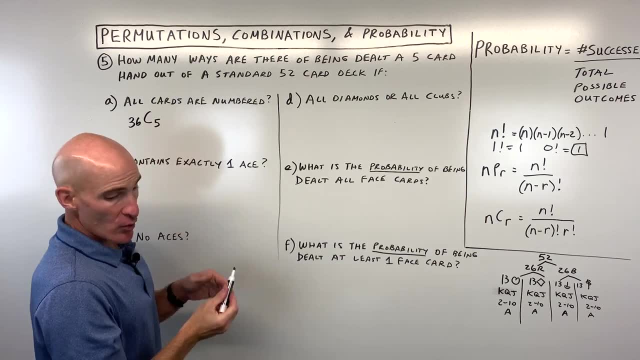 doesn't matter when you're dealt those cards, when you're in your hand, you can rearrange them. so it doesn't matter which card you're given first, second, third, because you can rearrange them. so it's the same five cards. so let's go ahead and figure out what that is: 36 combination five. let's. 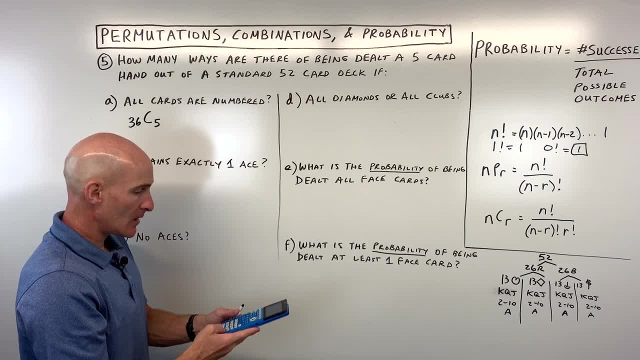 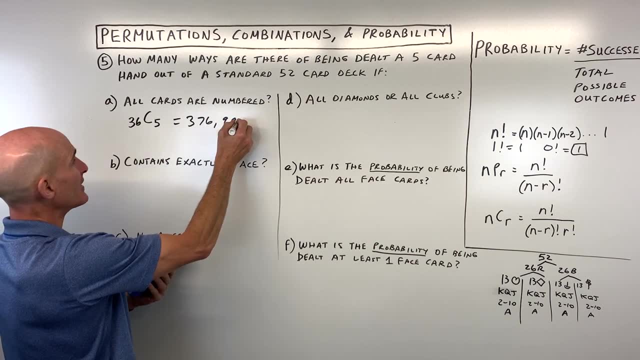 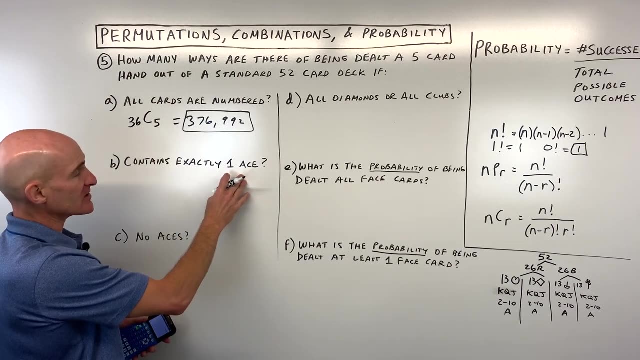 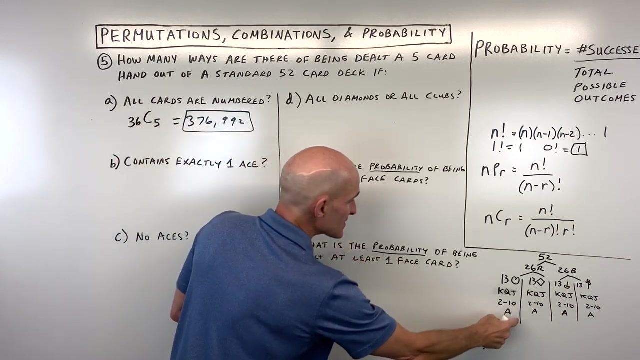 see what that is. it looks like we're about: okay, three hundred and seventy six thousand, uh, nine hundred ninety two different ways to be dealt. all numbered cards: okay, for letter b: it contains exactly one ace, so five. card hand: okay, and it contains exactly one ace. well, let's see, there's four aces, so out of the 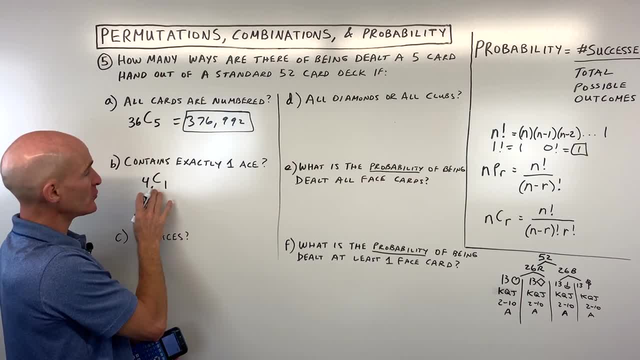 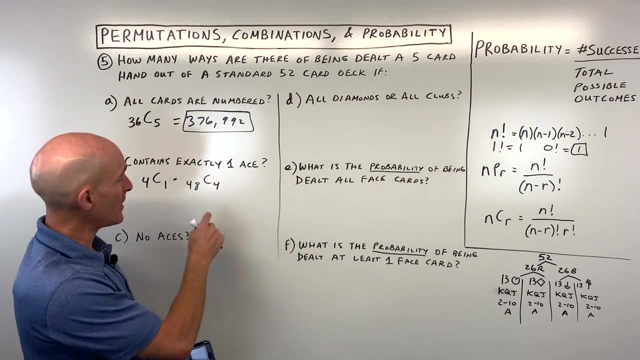 four aces. how many ways are there of being adult one of those four times out of the 48 remaining cards that are not aces, see 48, and 4 adds up to 52. how many ways are there of being dealt four of those cards out of the 48? so just remember, the first number is like how many you're dealing with. 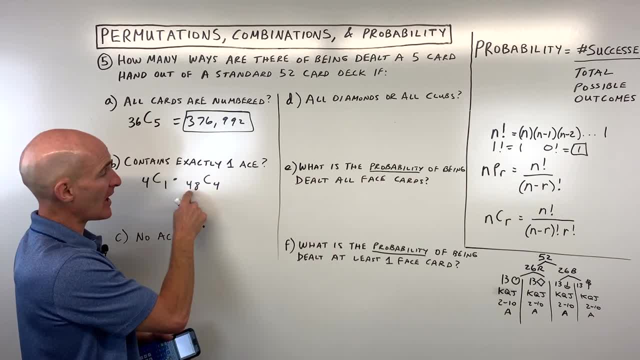 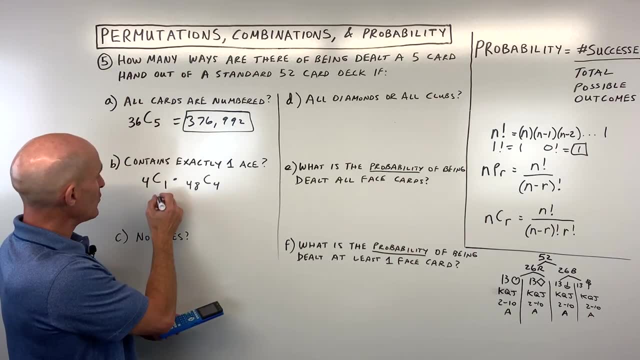 in that group, 48 non-aces, and the second number is how many we want out of that. 48, okay, and we're using combination c because the order doesn't matter, so let's go ahead and do this on the calculator. four c one is just four. four forty eight c four is one hundred ninety four thousand. 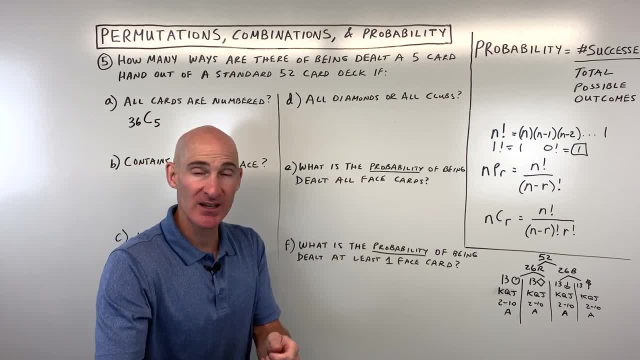 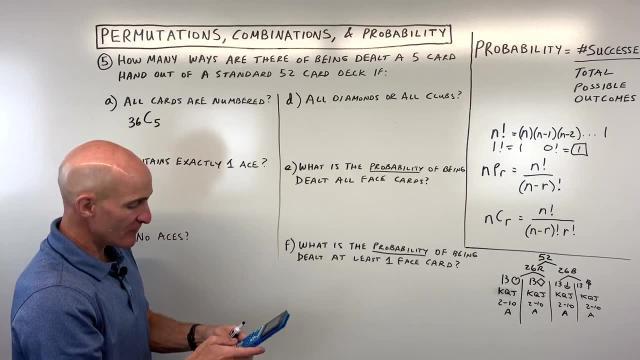 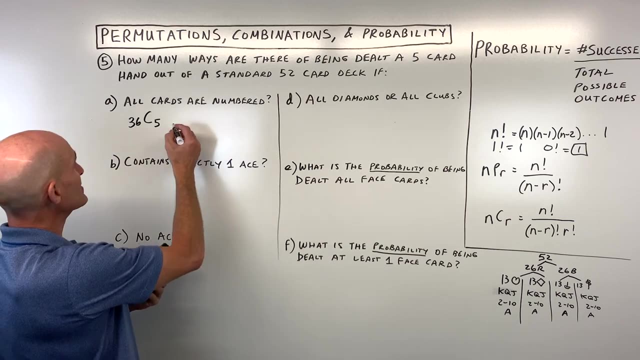 hand. you can rearrange them, So it doesn't matter which card you're given first, second, third, because you can rearrange them, So it's the same five cards. So let's go ahead and figure out what that is: 36 combination five. Let's see what that is. It looks like we're about, okay, 376,000. 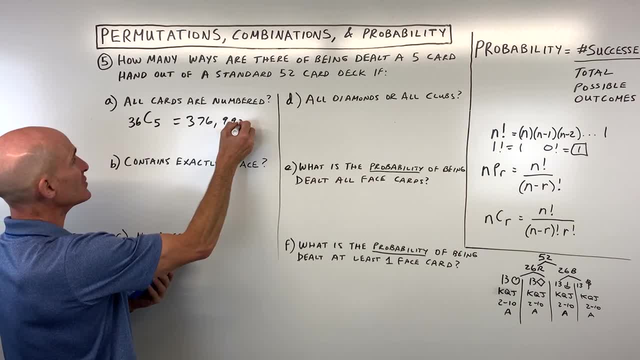 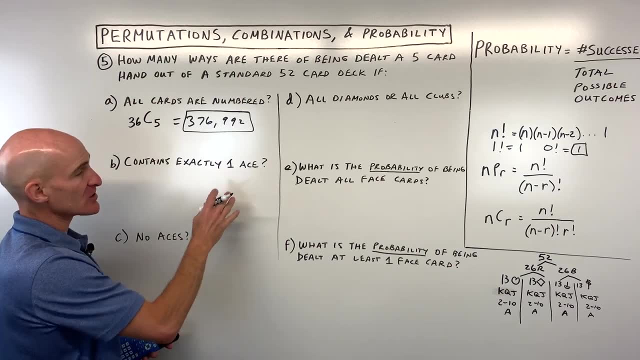 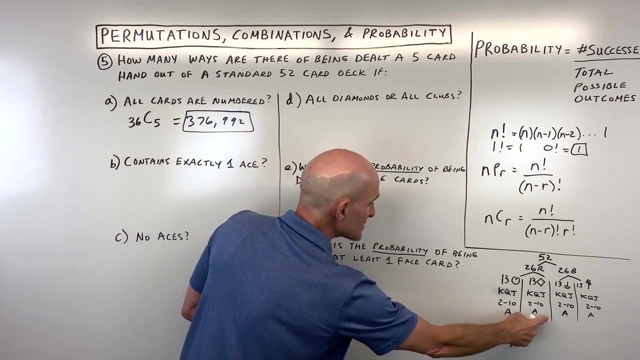 992 different ways to be dealt. all numbered cards: Okay. For letter B: it contains exactly one ace. So five card hand: Okay, And it contains exactly one ace. Well, let's see There's four aces. So, out of the four aces, how many ways are there of being dealt one of those four? 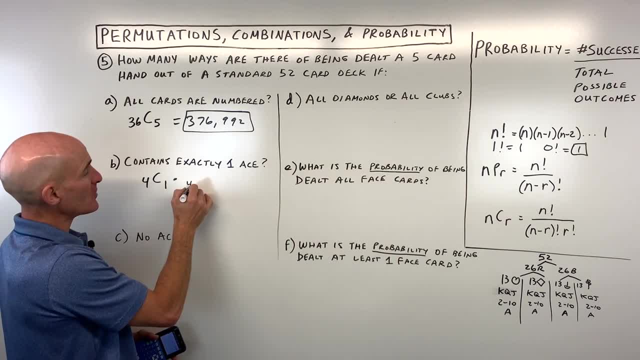 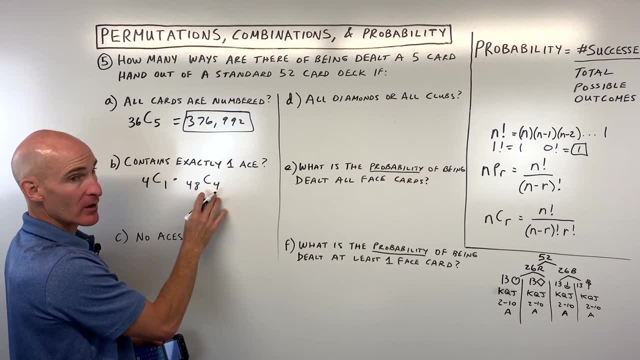 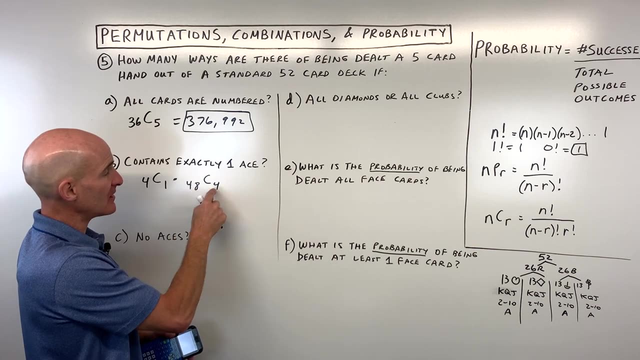 times out of the 48 remaining cards that are not aces, see 48, and four adds up to 52. How many ways are there of being dealt four of those cards out of the 48?? So just remember, the first number is like how many you're dealing with in that group: 48 non-aces. And the second number 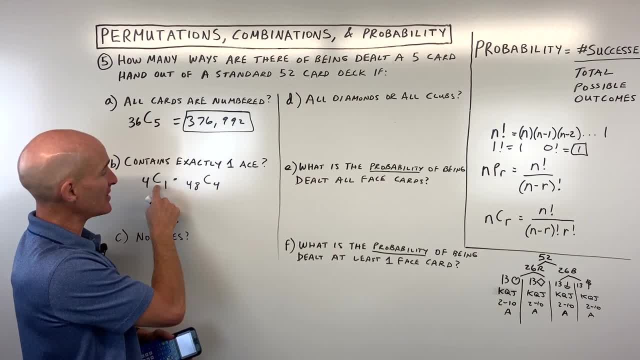 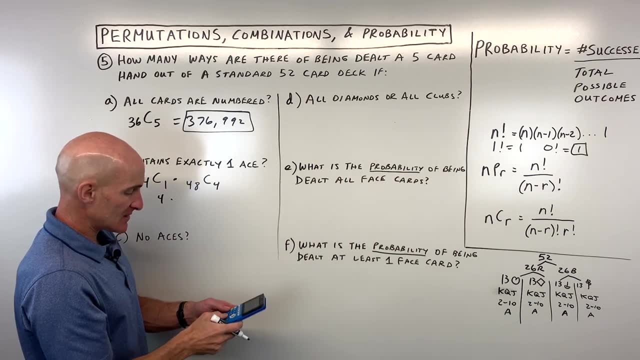 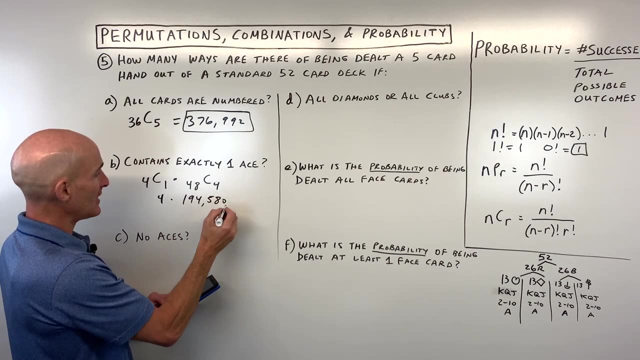 is how many we want out of that? 48.. Okay, And we're using combination C because the order doesn't matter, So let's go ahead and do this on the calculator. 4C1 is just four, 48C4 is 194,580. 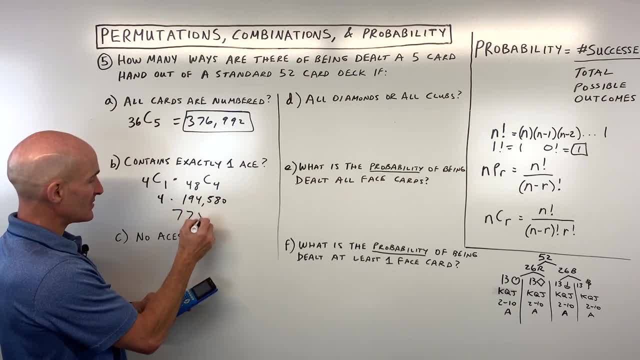 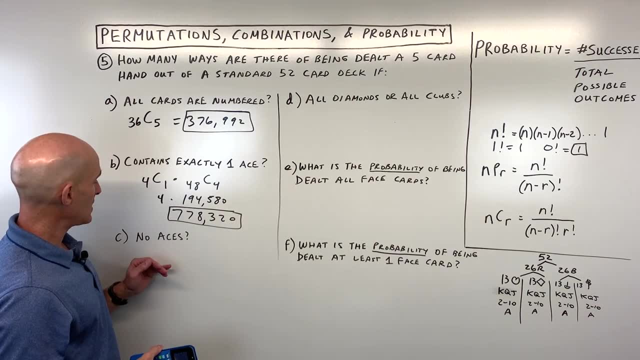 And if we multiply that by four, okay, we're getting 778,320.. So 778,320 different ways of getting a five card hand that contains exactly one ace. Now, what happens if you want no aces? How many ways are there to be dealt? 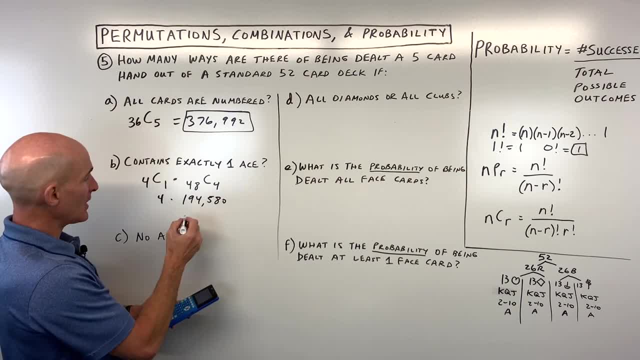 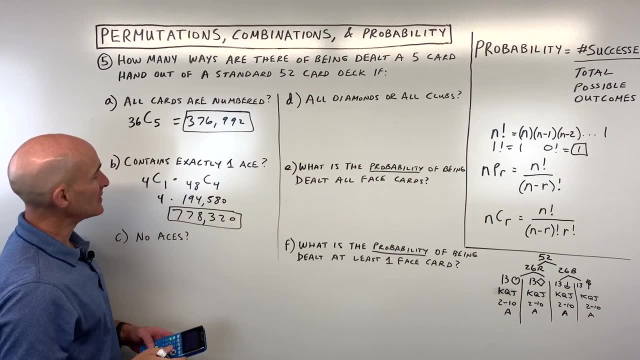 five hundred and eighty, and if we multiply that by four, okay, we're getting seven, seven, eight, three, two, zero. so seven hundred seventy, eight thousand, three hundred, twenty. uh, different ways, uh, of getting a five card hand that contains exactly one ace. now what happens if you want no? 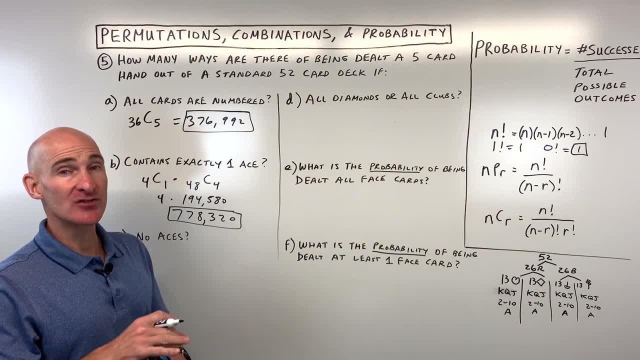 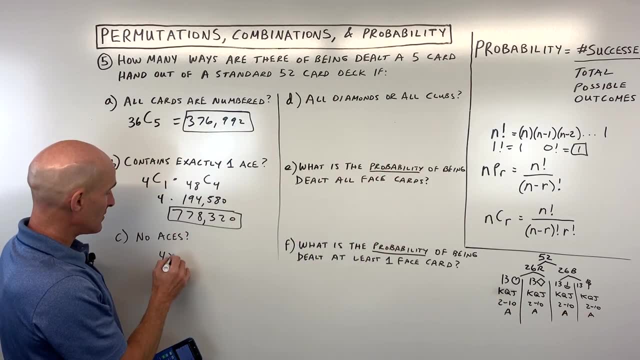 aces. how many ways are there to be dealt a five card hand and there's no aces in that five card hand? well, because we said there's four aces, that means there's 48 cards that are not aces and we want to see how many ways are getting five out of that 48. so 48 combination, five. 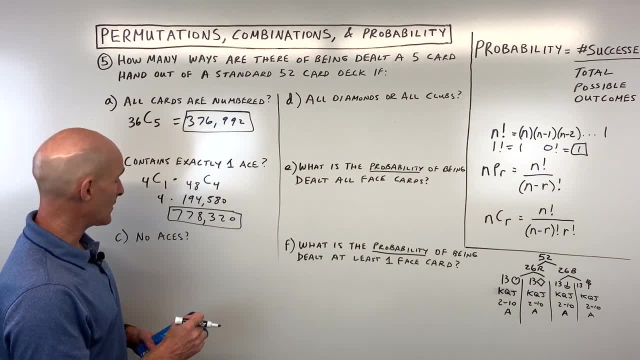 a five card hand and there's no aces in that five card hand. Well, because we said there's four aces, that means there's 48 cards that are not aces And we want to see how many ways are getting five out of that 48.. So 48,. 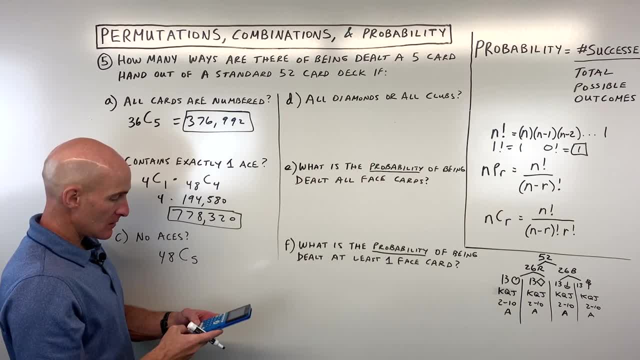 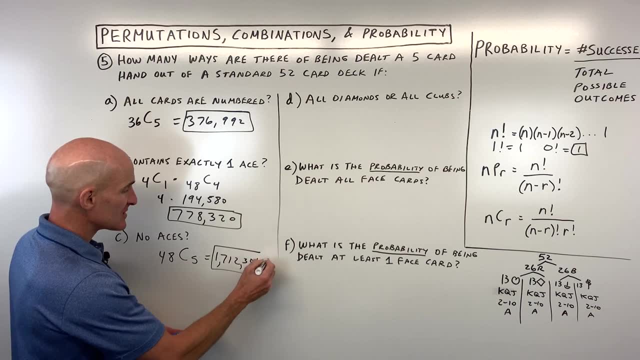 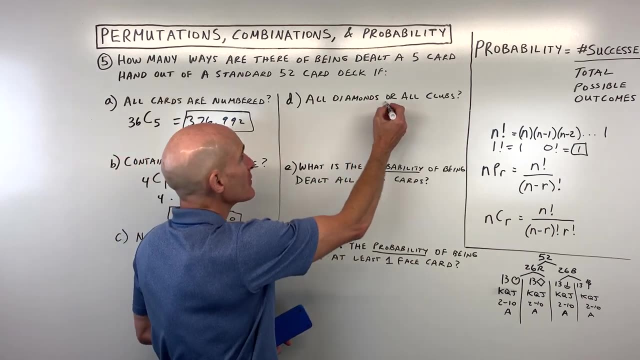 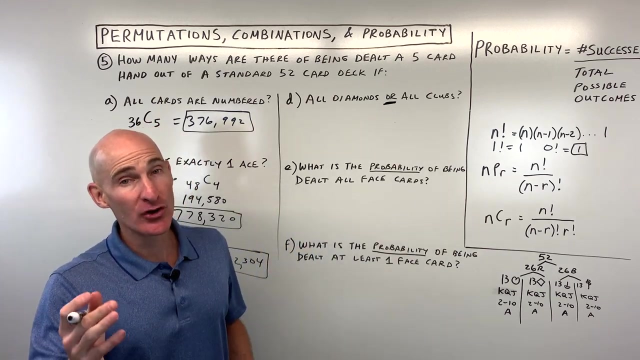 combination five, Okay, And that comes out to 1,700,000.. Okay, And then for letter D: all our diamonds or all our clubs. Now, in math, let's talk about this for a second. Or means union, It means like combined, It means both, but you don't want to double count, So 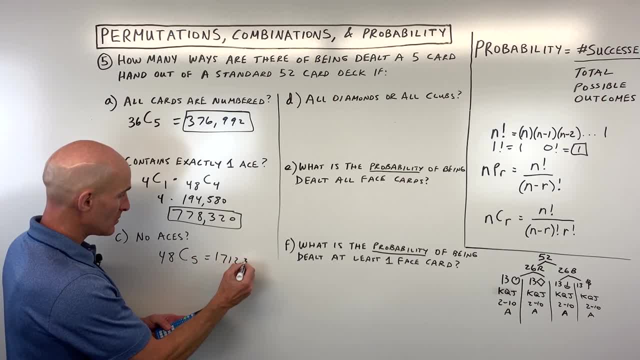 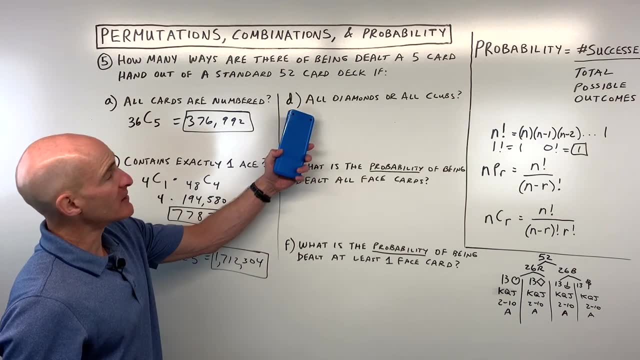 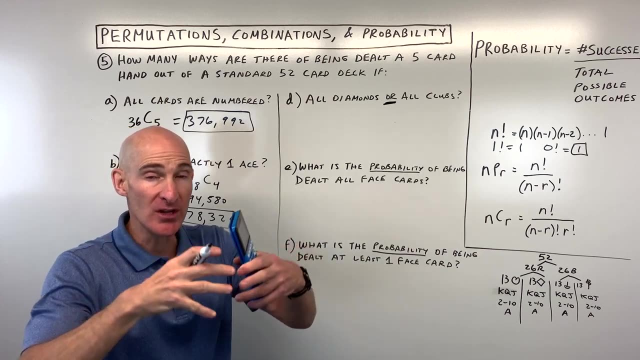 okay, and that comes out to one million seven hundred thousand. okay, and then for letter d, all our diamonds or all our clubs. now, in math, let's talk about this for a second. or means union. it means like combined, it means both, but you don't want to double count. so if you're familiar with venn diagrams, 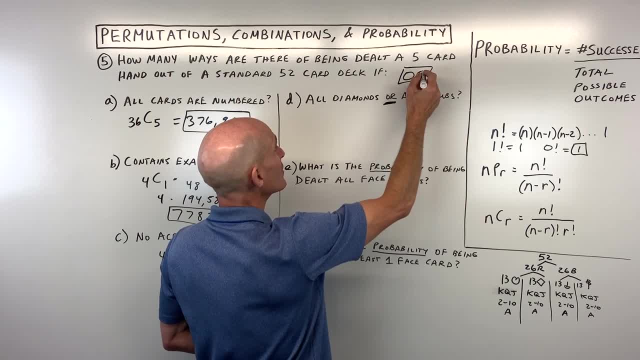 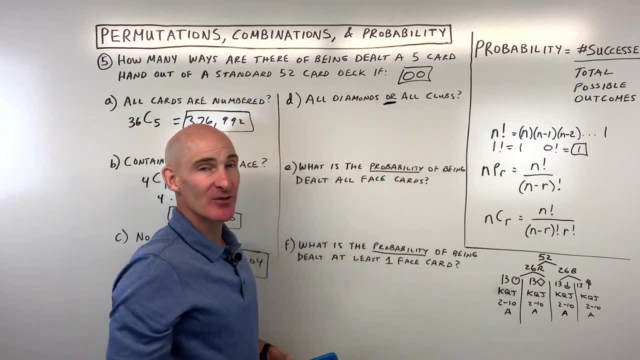 remember your venn diagrams? see, here's the diamonds, here's the clubs, or means both combined together. now, if they were overlapping, like if there was some diamonds that were clubs and some clubs that were also diamonds, we'd have to double count the ones we'd have to subtract off. 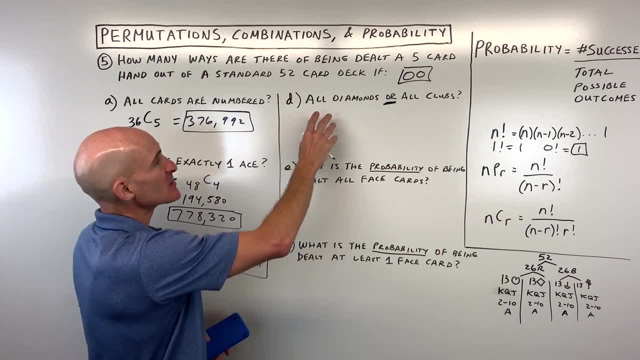 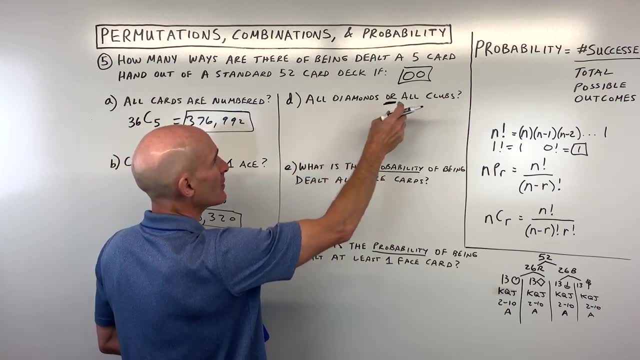 the double counted ones. we don't want to double count, but in this case these are what they call mutually exclusive or non-overlapping, and so what we can do is we can just add the number of diamonds, or the number of ways to get five diamonds, the number ways to get five clubs. so how many diamonds? 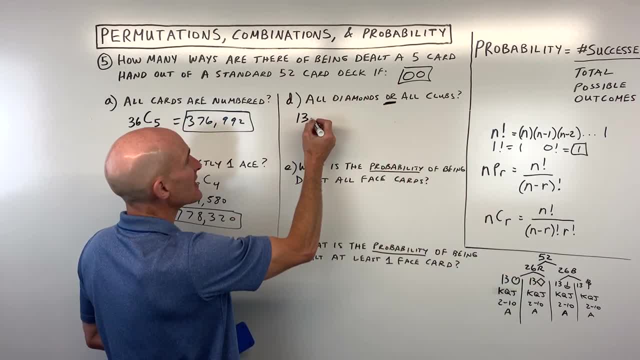 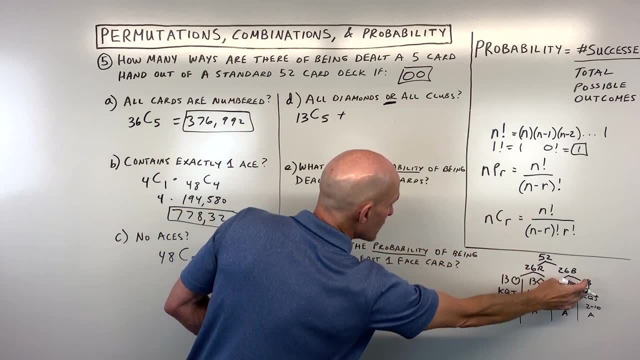 are there, there's thirteen diamonds. so, out of the thirteen diamond cards, how many ways are there of Choosing five of those where the order doesn't matter? Plus, out of the 13 clubs, how many ways are there of choosing five of those? So let's see what that comes out to. 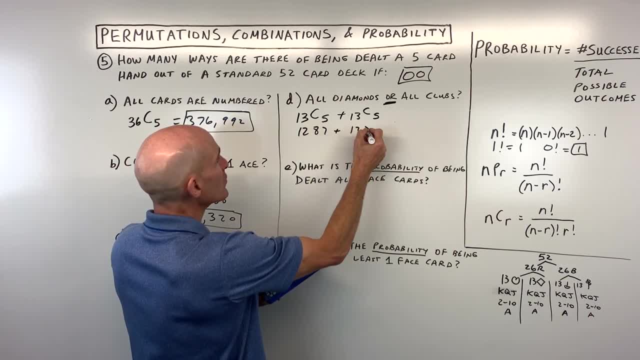 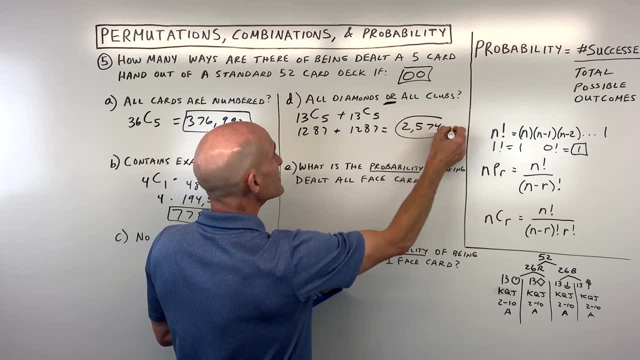 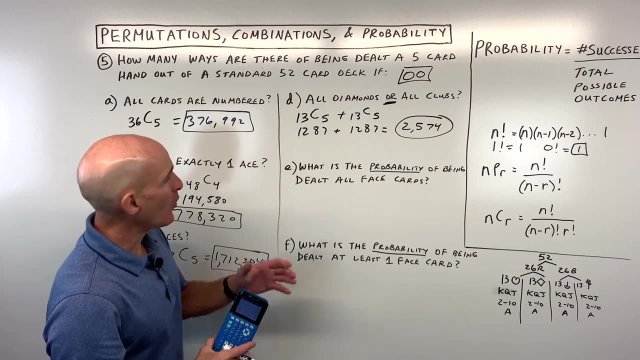 This is 1,287 plus 1,287, which is 2,574 ways of being dealt five diamonds or five clubs. Okay, so for letter E. now what is the probability of being dealt? all face cards? Okay, now notice, we're dealing with probability. 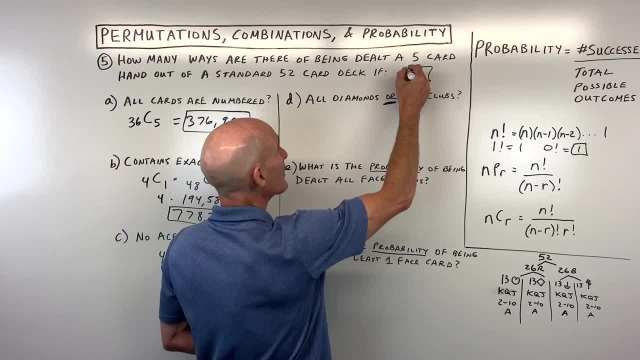 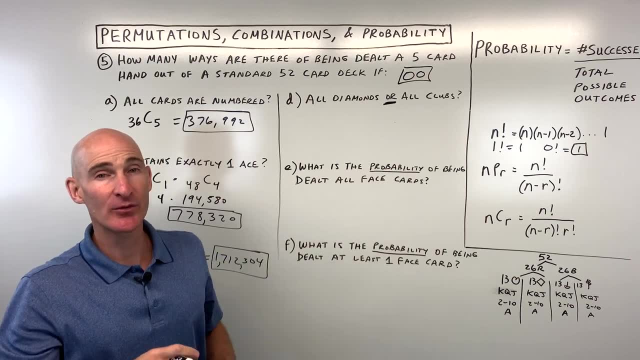 if you're familiar with Venn diagrams, remember your Venn diagrams. See, here's the diamonds, here's the clubs. Or means both combined together. Now, if there were overlapping, like if there was some diamonds that were clubs and some clubs that were also. 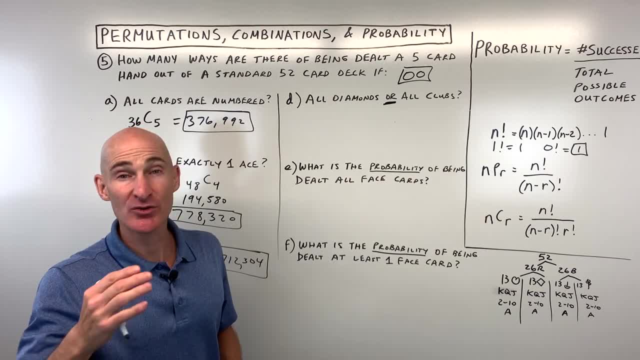 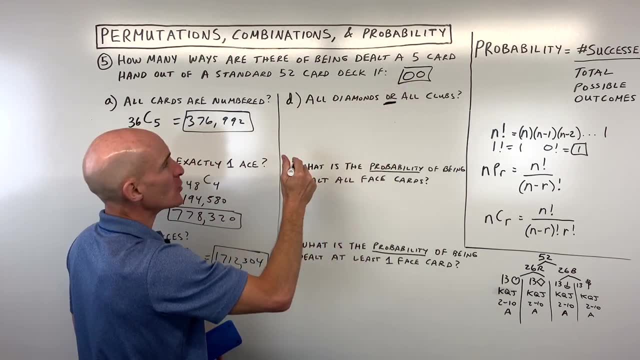 diamonds, we'd have to double count, the ones We'd have to subtract off the double counted ones. We don't want to double count, But in this case these are what they call mutually exclusive or non-overlapping, And so what we can do is we can just add the number of diamonds or the number of. 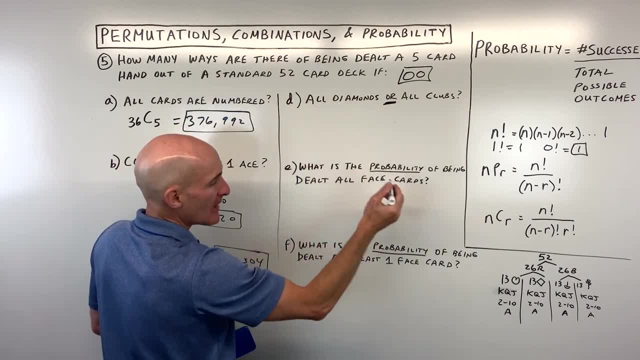 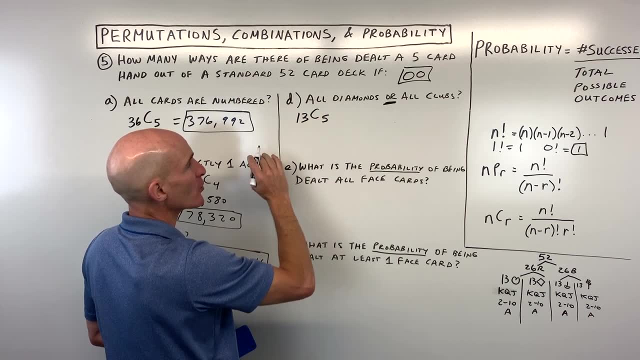 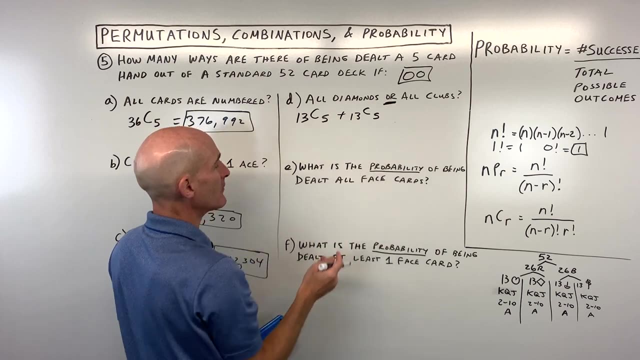 ways to get five diamonds, the number of ways to get five clubs. So how many diamonds are there? There's 13 diamonds Out of the 13 diamond cards. how many ways are there of choosing five of those where the order doesn't matter Plus out of the 13 clubs? how many ways are there of choosing five of those? 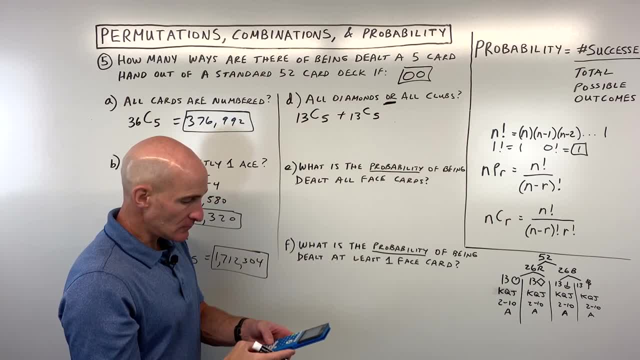 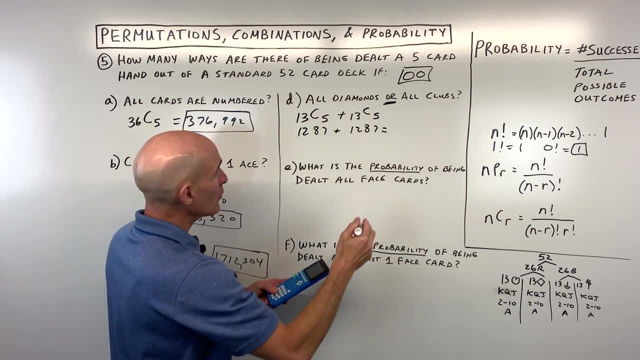 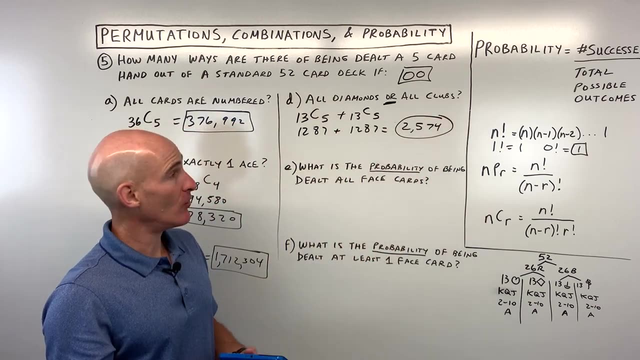 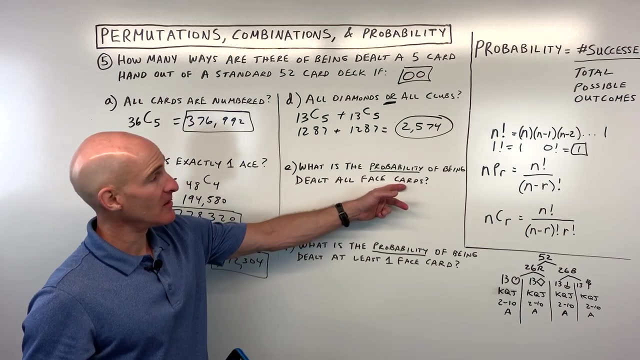 So let's see what that comes out to. This is 1,287 plus 1,287, which is 2,574 ways of being dealt five diamonds or five clubs. So for letter E now what is the probability of being dealt? all face cards. 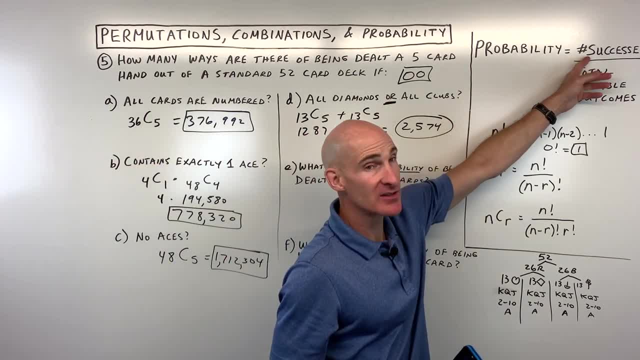 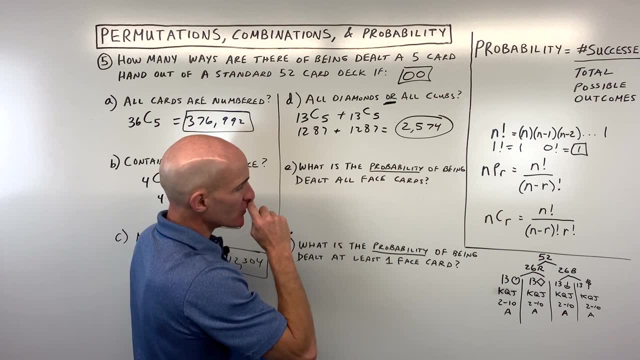 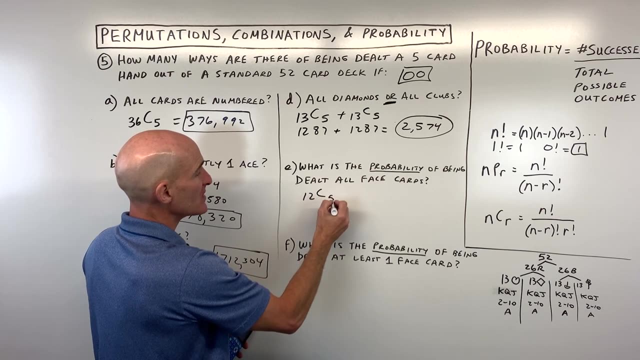 Now notice we're dealing with probability. Probability is the number of successful outcomes, or what we want, divided by the total possible outcomes. So being dealt: all face cards, So face cards. we can see that there's 12 face cards. So, out of 12 face cards, how many ways are there of getting five out of that 12, where the order doesn't matter? 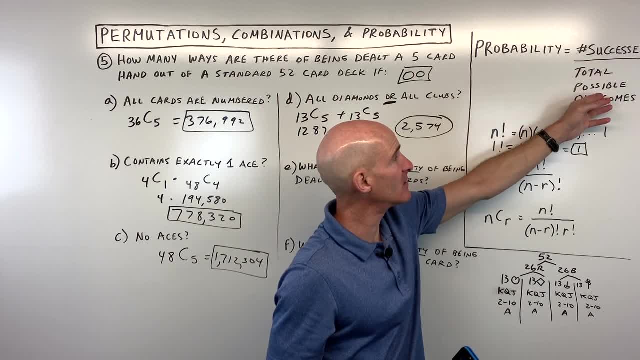 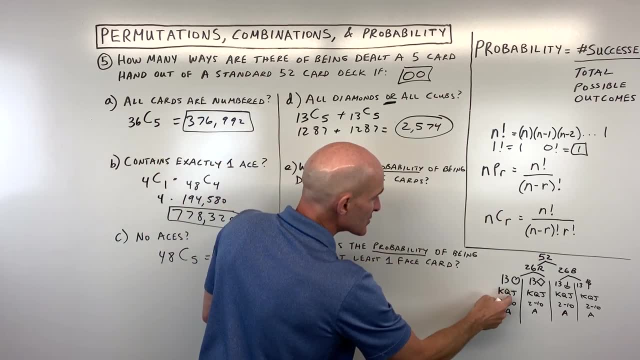 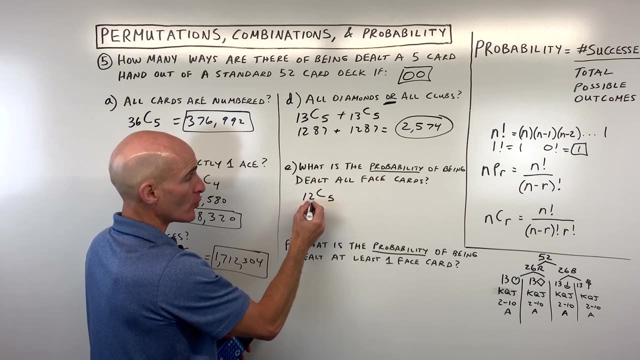 Probability is the number of successful outcomes, or what we want, divided by the total possible outcomes. So being dealt: all face cards, So face cards. we can see that there's 12 face cards. So, out of 12 face cards, how many ways are there of getting five out of that 12, where the order doesn't matter? 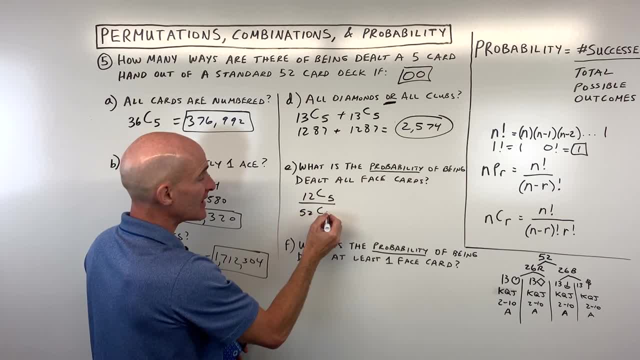 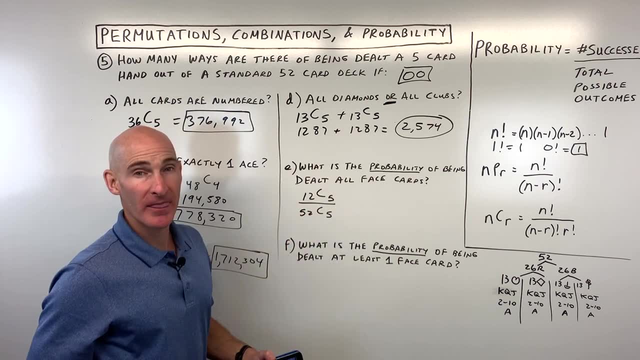 divided by the total ways of being dealt, Five cards out of the 52 card deck: See probability. again, it's what you want out of the total. Okay, so in this case, let's see what this comes out to. 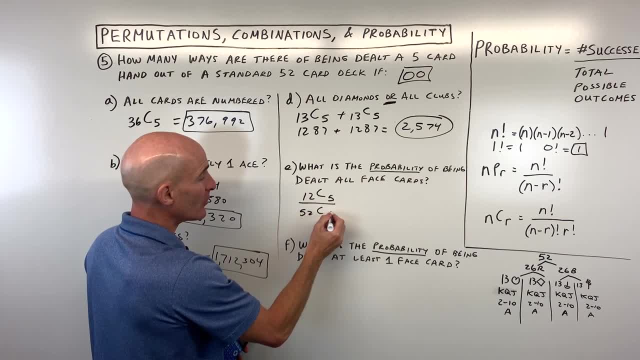 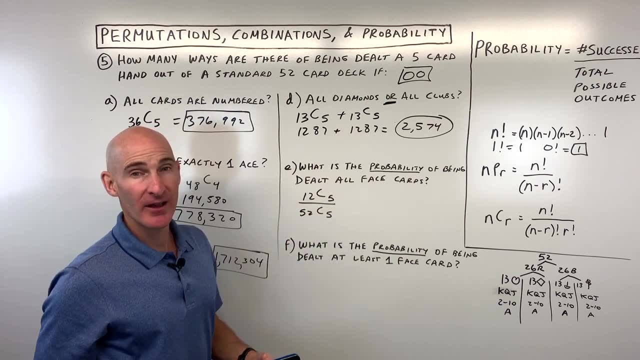 divided by the total ways of being dealt. five cards out of the 52 card deck: See probability. again, it's what you want out of the total. Okay, So in this case, let's see what this comes out to. So 12 combination: 5. 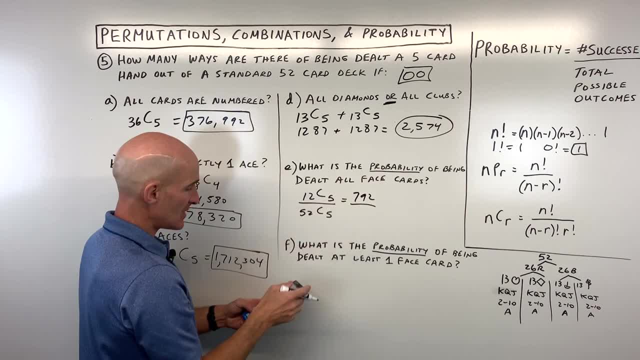 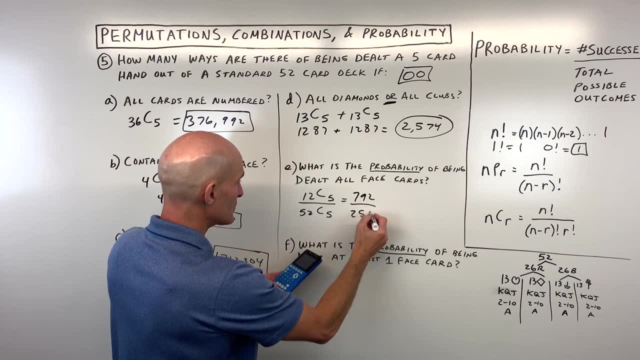 is 792 ways of being dealt. all face cards. and 52 combination 5 is a big number: 25.oops 2598960.. and 52 combination 5 is a big number: 25.oops 2598960.. 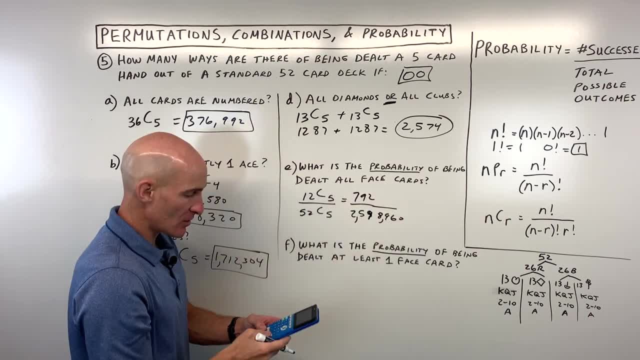 and 52 combination. 5 is a big number: 25.oops, 2598960.. And you might be able to reduce this down Here. I'll see if it reduces down a little bit. Let's see, does that reduce? 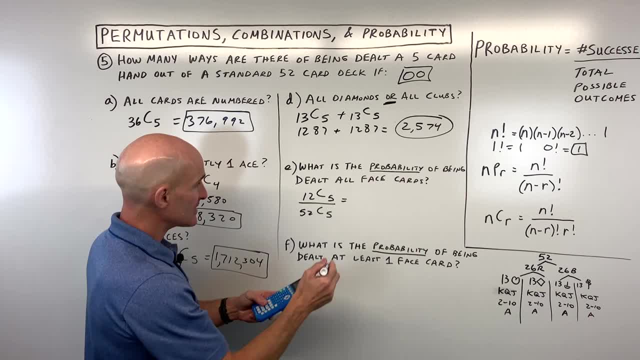 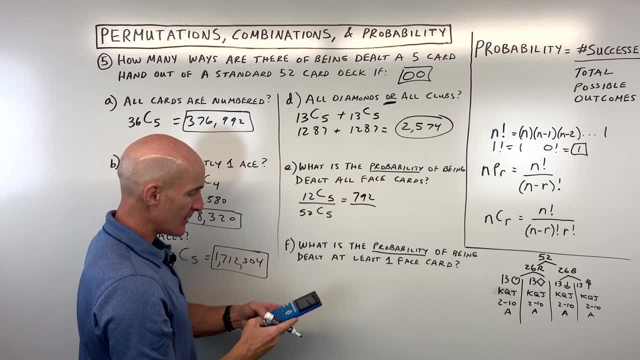 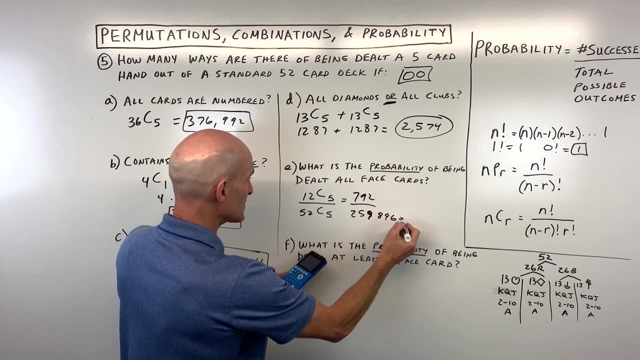 So 12 combination 5 is 792 ways of being dealt all face cards And 52 combination 5 is a big number. 2, 5, oops 2, 5, 9, 8, 9, 6, 0.. 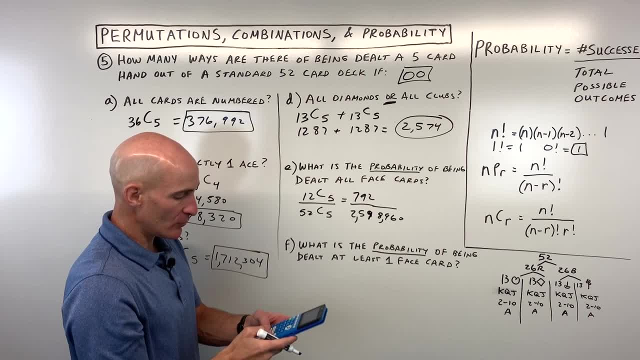 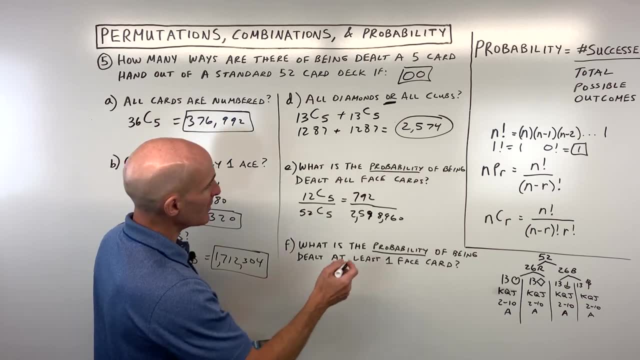 And you might be able to read: Let's see if I can reduce this down Here. I'll see if it reduces down a little bit. Let's see. does that reduce? My calculator's not reducing it, but you can reduce it to see how they're both even. 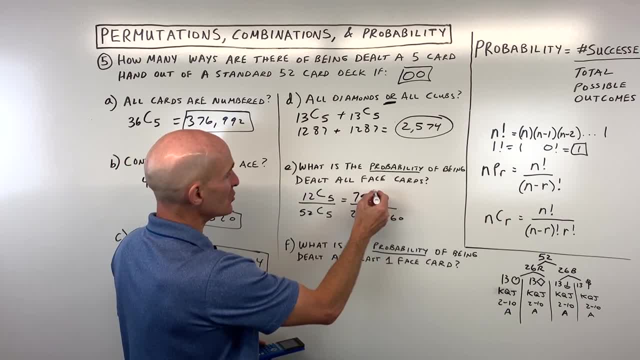 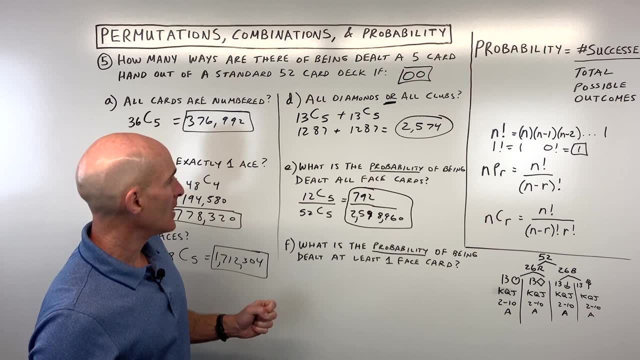 You can divide by 2.. You can also write it as a decimal approximation, You can even convert it to a percent, but that's really the percent. chance Probability is more like a fraction or a decimal, not a percent. Okay, and then the last one, letter F. 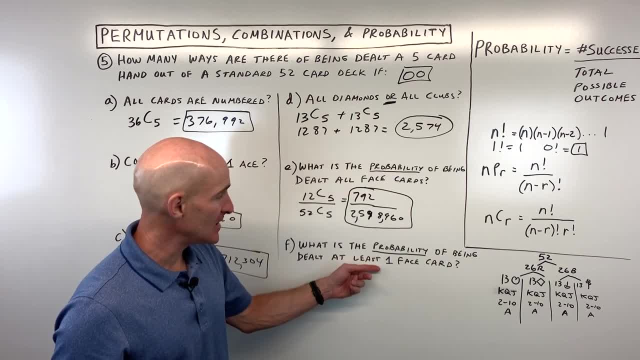 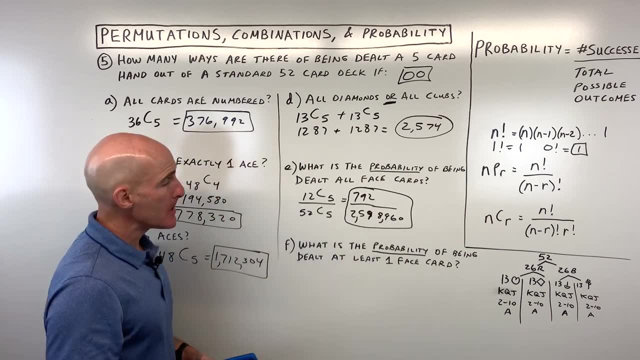 What is the probability of being dealt at least one face card? So at least Now again we're dealing with probability And we did a similar problem where we said- at least one woman remember in that committee- But with probability the total is 100% right. 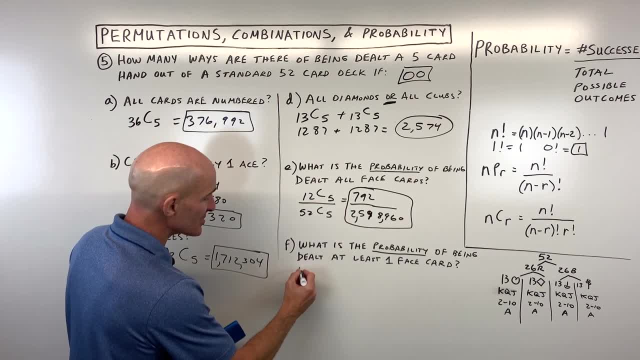 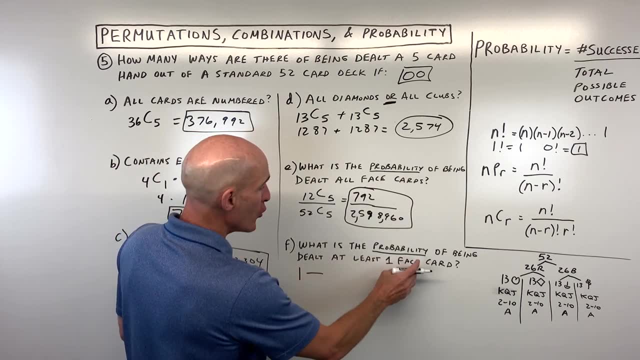 That's everything that could happen, And 100% written just as a number is the number 1.. 1 is, like you know, 100%, So 1 minus okay, no face cards. So we're going to do the probability that you get no face cards. 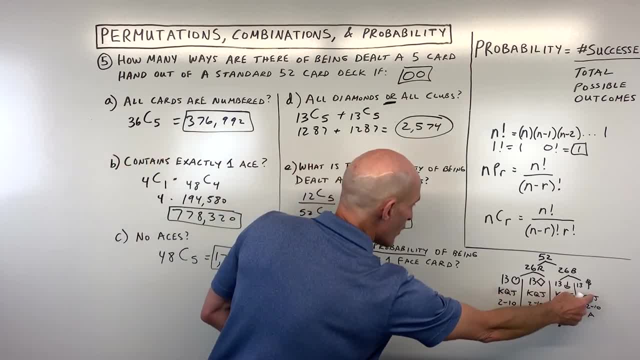 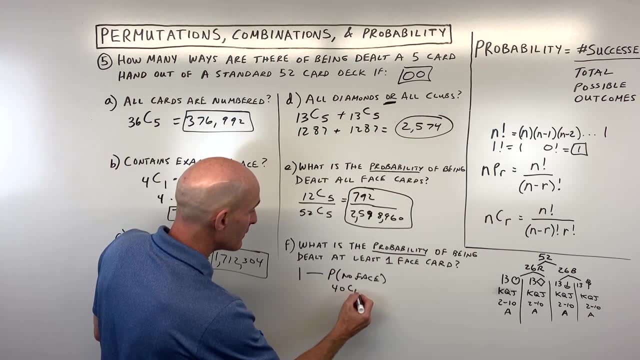 And let's see So no face cards would be. There's 12 face cards, which means that there's 52 minus 12, 40 non-face cards, So that would be 40C5.. So, out of 40 non-face cards, how many ways are there of choosing 5?? 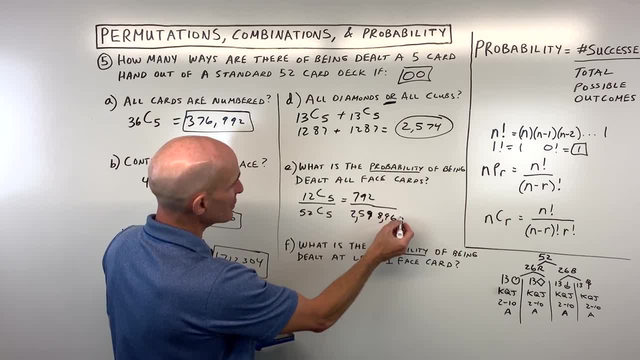 My calculator's not reducing it, but you can reduce it to see how they're both even. You can divide by two. You can also write it as a decimal approximation. You can even convert it to a percent, but that's really the percent chance. 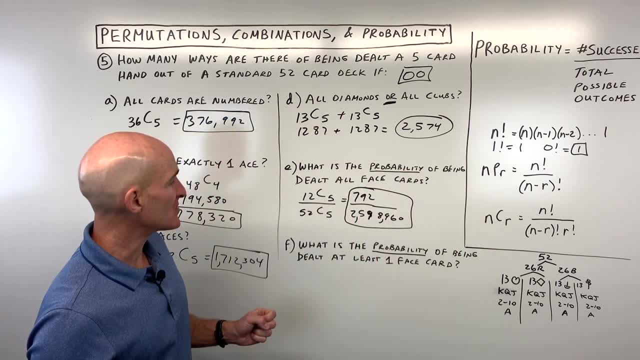 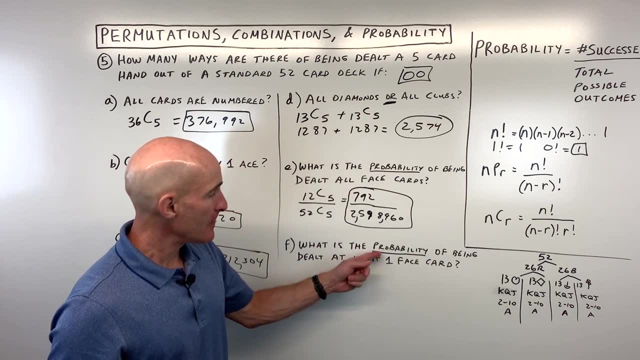 Probability is more like a fraction or a decimal, not a percent. Okay, and then the last one, letter F. What is the probability of being dealt at least one face card? So at least Now again we're dealing with probability. 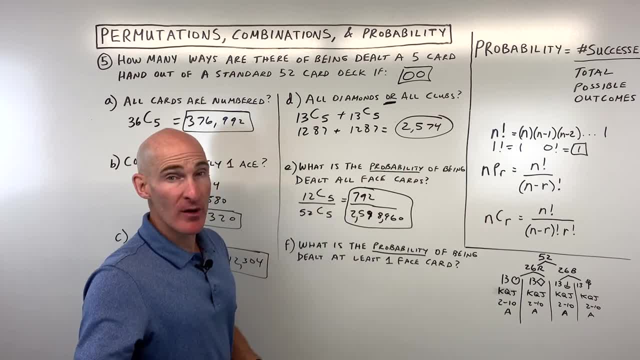 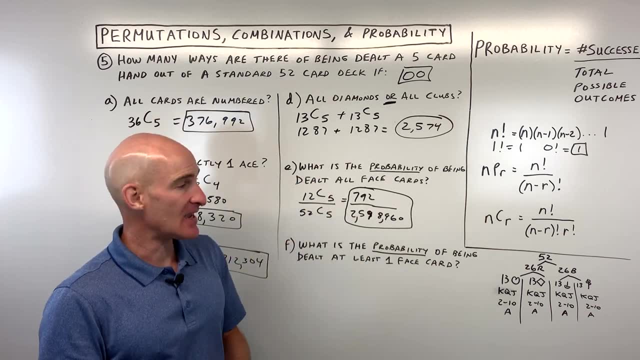 And we did a similar problem where we said at least one woman remember in that committee, But with probability the total is 100%. right, That's everything that could happen, And 100% written, just as a number, is the number one. 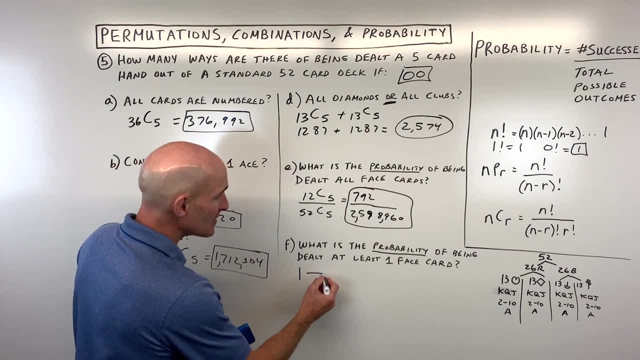 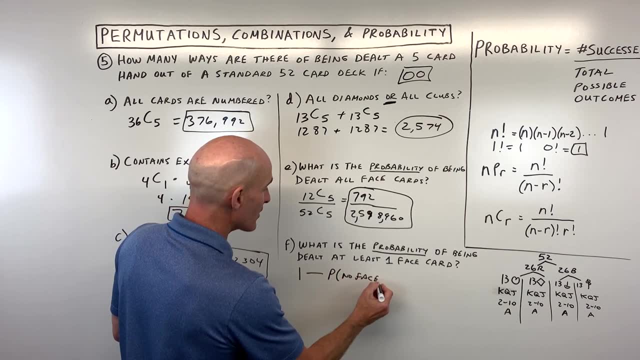 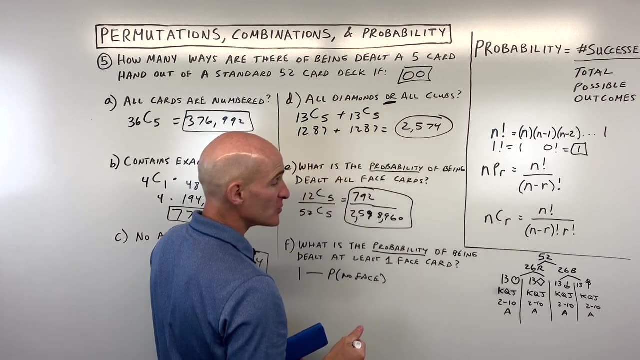 One is like 100%, So one minus. okay, no face cards. So we're going to do the probability that you get no face cards And let's see. so no face cards would be. there's 12 face cards, which means that there's 52 minus 12, 40 non-face cards. 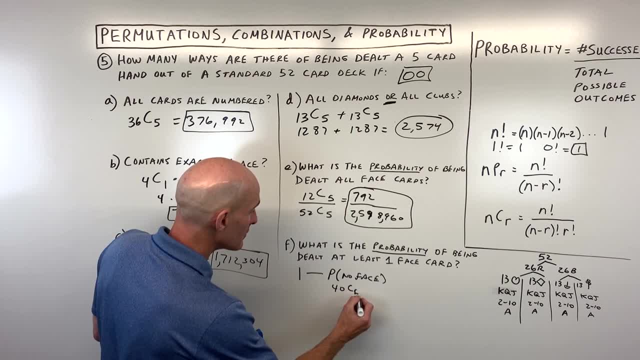 So that would be 40C5.. So, out of 40 non-face cards, how many ways are choosing five Divided by how many ways are there of getting five face cards out of the 52 standard deck here? And we're going to take that away from one? 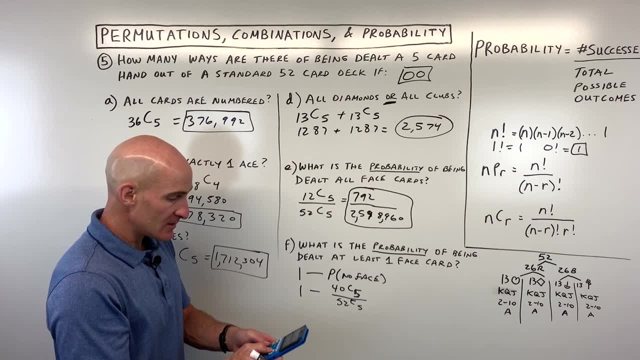 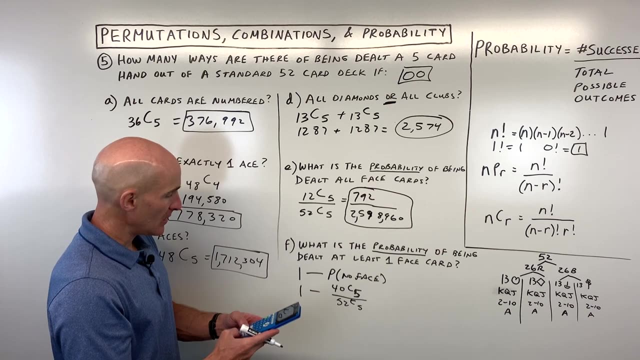 So let's see what that comes out to. So 40C5.. 40C5, okay, divided by 52C5.. Okay, so this is basically. I'm going to round a little bit. So this comes out to about 0.25. 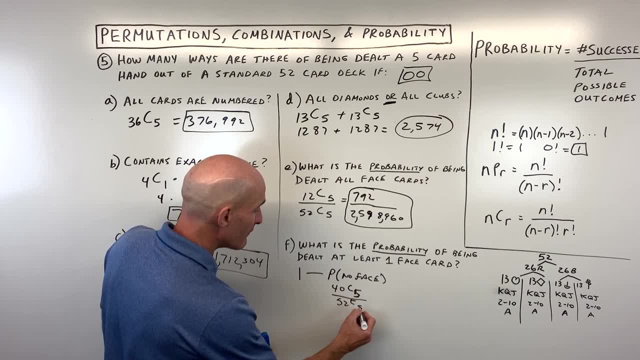 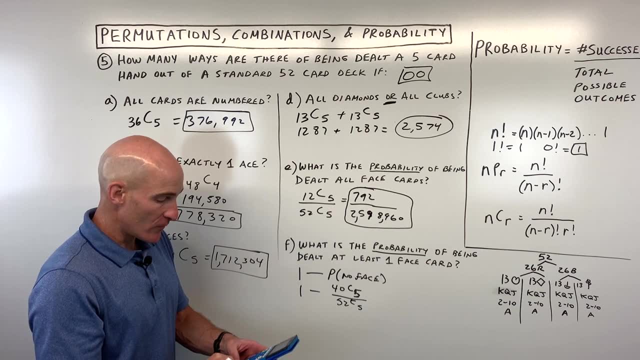 Divided by how many ways are there of getting 5 face cards out of the 52 standard deck here? And we're going to take that away from 1.. So let's see what that comes out to. So 40C5.. 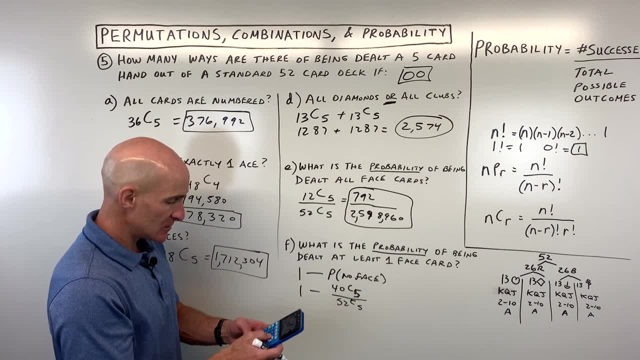 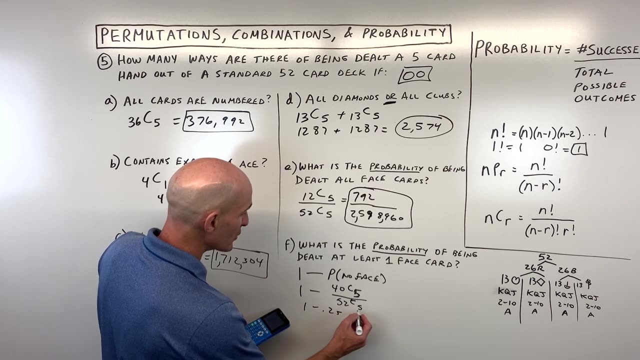 Okay, Divided by 52C5.. Okay, So this is basically. I'm going to round a little bit. So this comes out to about 0.25.. So 1 minus 0.25 is going to be 0.75.. 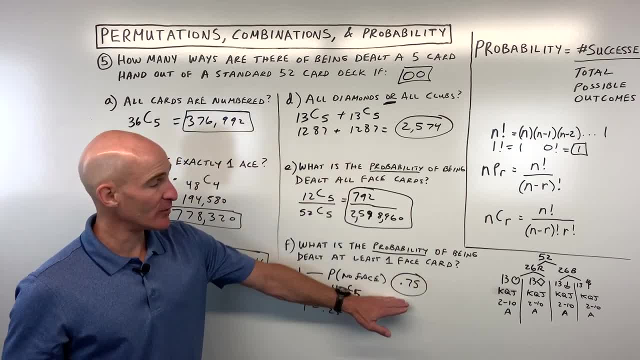 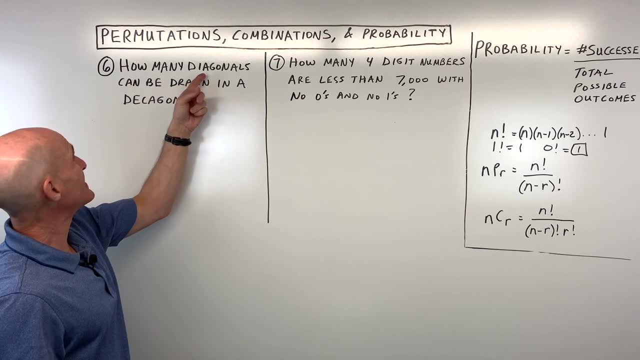 So it's about a 75% chance, but the probability is 0.75 or 3 fourths approximately. And you got it Okay. let's take a look at number 6 now. It says How many diagonals can be drawn in a decagon. 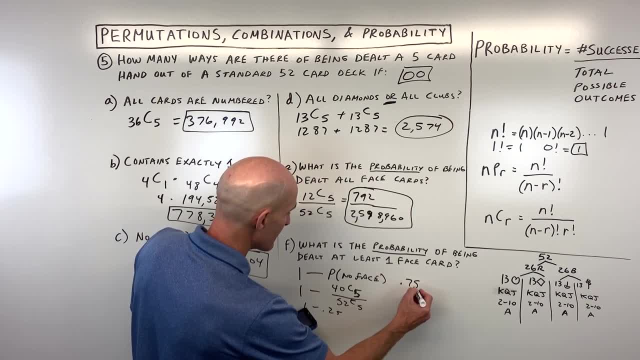 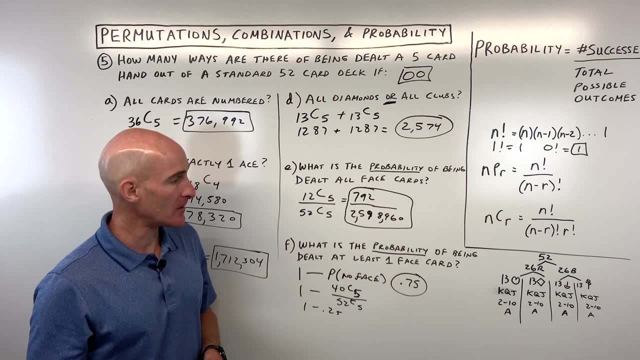 So one minus 0.25 is going to be 0.75.. So it's about a 75% chance, but the probability is 0.75 or three-fourths approximately. And you got it Okay. So let's take a look at number six now. 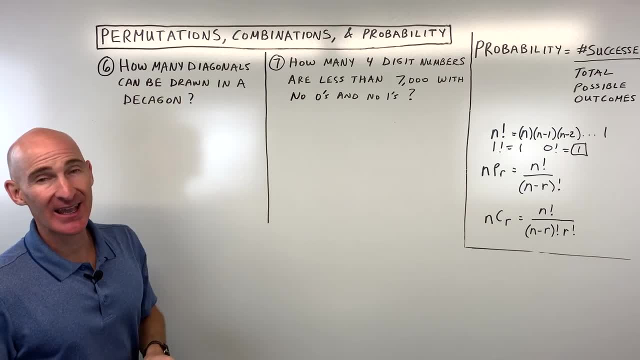 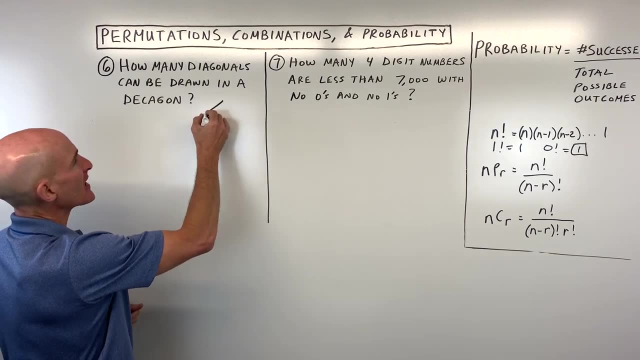 It says how many diagonals can be drawn in a decagon. So remember: a decagon, it's a polygon with 10 sides. And what exactly is a diagonal? Well, let's do a simpler example, And this is a good technique sometimes. 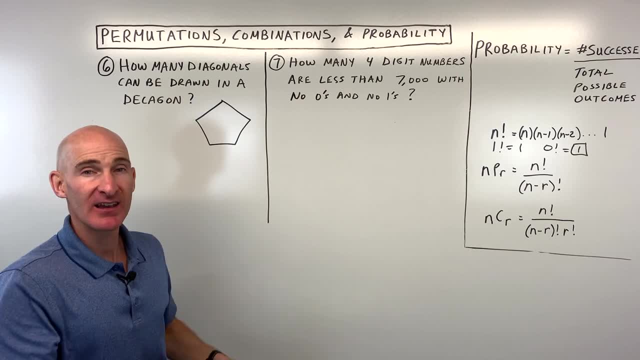 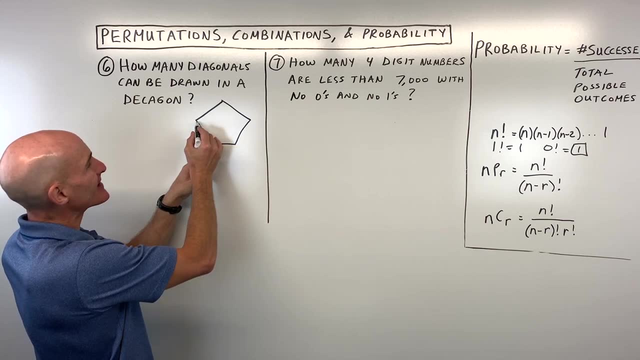 If you ever have a difficult problem, try to do a simpler one and then kind of extrapolate out and you can solve more challenging ones that way. A diagonal: it connects two non-consecutive vertices. The vertices are the points here on our polygon. 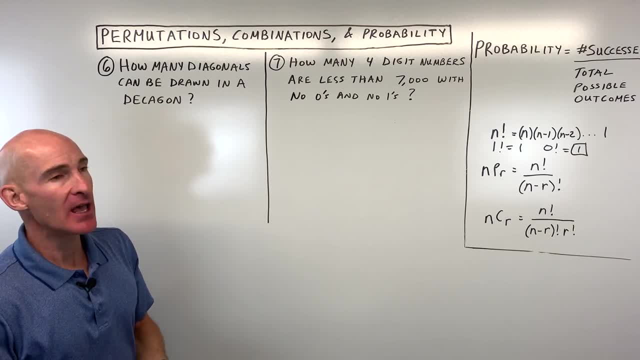 So remember a decagon. it's a polygon with 10 sides, And what exactly is a diagonal? Well, let's do a simpler example, And this is a good technique sometimes: If you ever have a difficult problem, try to do a simpler one and then kind of extrapolate out. 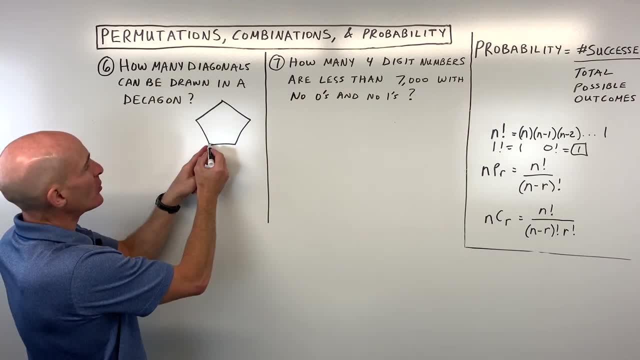 And you can solve more challenging ones that way. A diagonal: it connects two non-consecutive vertices. The vertices are the points here on our polygon. So, for example, this would not be a diagonal, but this would be a diagonal. This would be a diagonal. 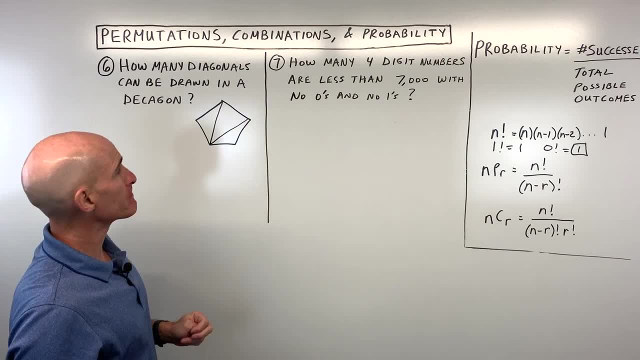 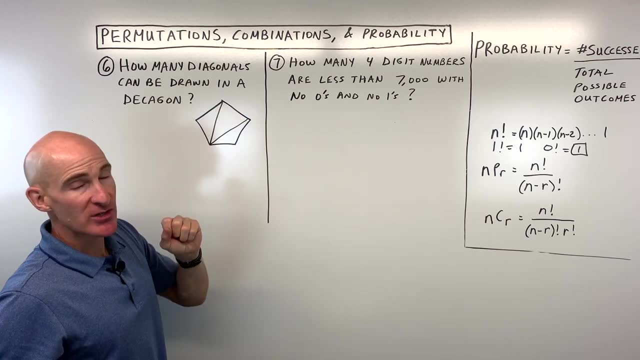 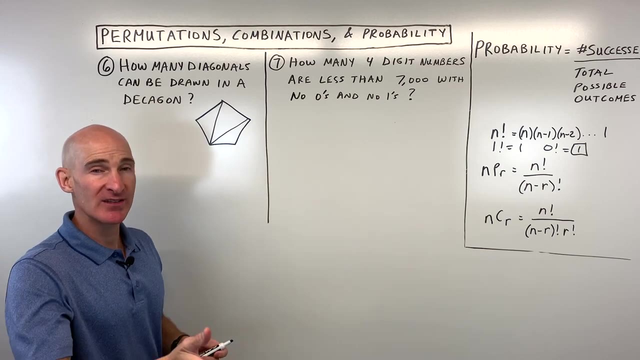 This would not be a diagonal. So what's interesting here is you can see you're connecting up two points in the polygon right And there's- in this case there's five points total. And there's a similar problem that I think I've done before in another video, where it's like you're at a party and it's like how many different ways can you know everyone shake hands with every other person, right? 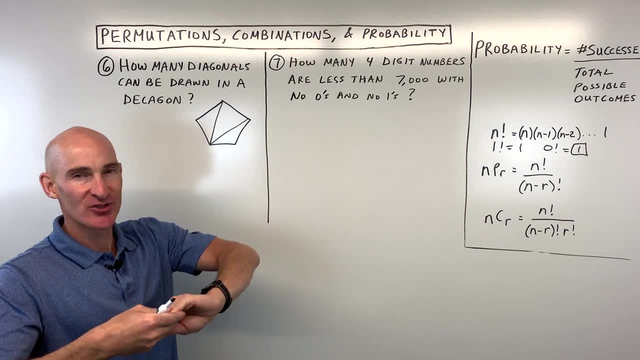 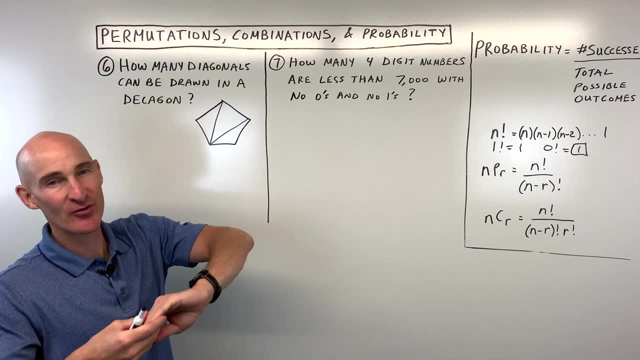 So when you're shaking hands, like there's two people are involved in that handshake right, And the order doesn't matter. If A shakes person B's hand or B shakes person's A hand, right, that's the same one handshake. 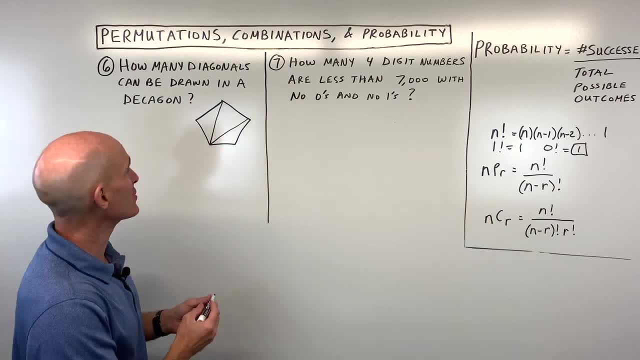 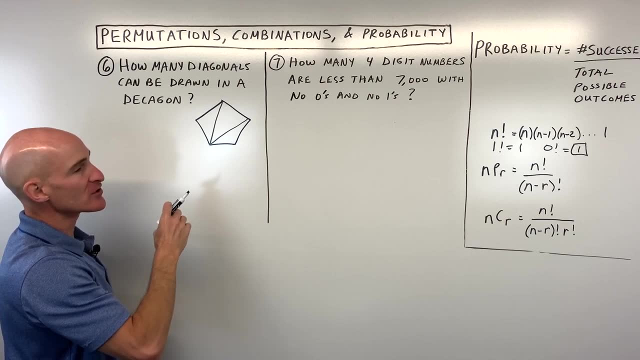 You don't want to double count it, So you're going to want to use combinations, because the order doesn't matter: This vertice and this vertice, or this one and this one, the order doesn't matter. But you're pairing up two vertices out of the okay. in this case it's a decagon, so 10.. 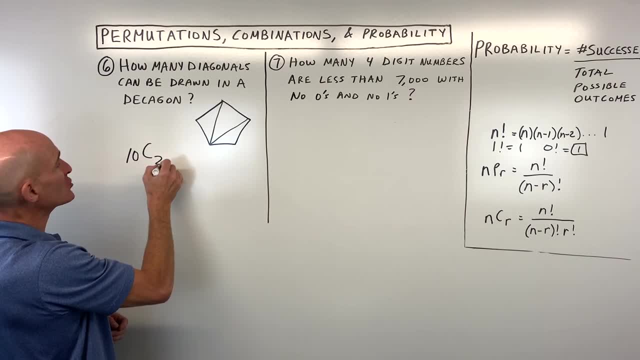 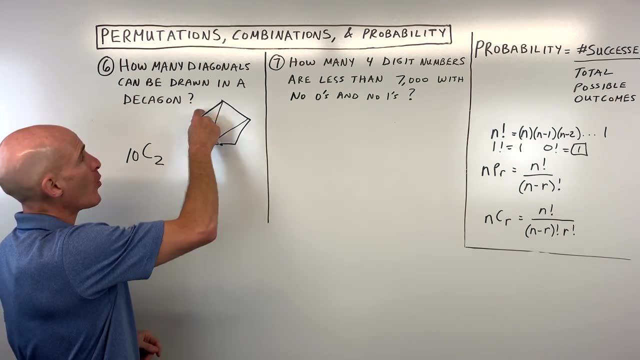 So we're saying: out of 10 vertices, how many ways are there to choose two, to make a line segment between the two of them? That's a diagonal. But what's interesting about this is we don't want to count the sides of the polygon because those are not diagonal. 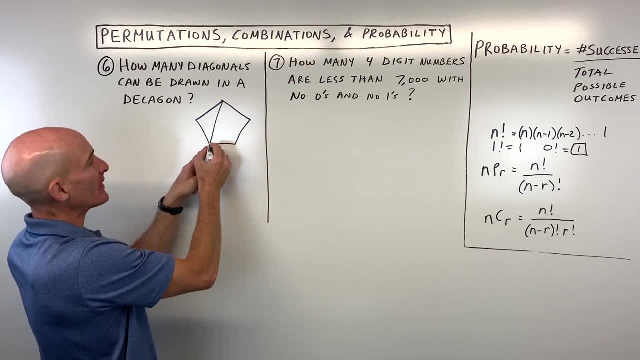 So, for example, this would not be a diagonal, But this would be a diagonal. this would be a diagonal, this would not be a diagonal. So what's interesting here is you can see you're connecting up two points in the polygon right. 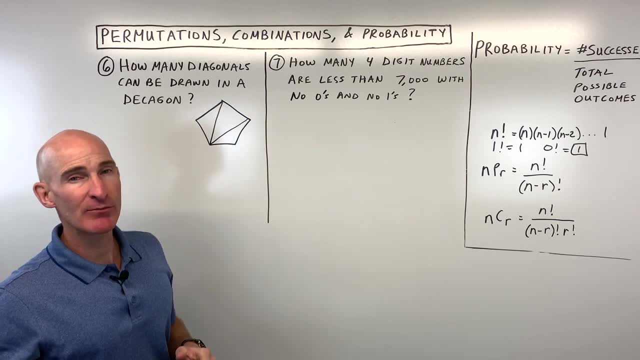 And there's- in this case there's five points total. And there's a similar problem that I think I've done before in another video, where it's like you're at a party and it's like: how many different ways can you know? 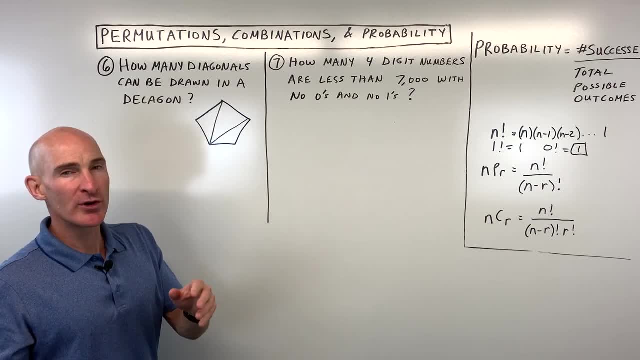 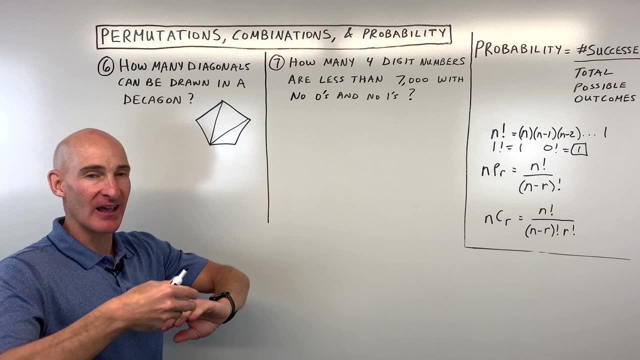 everyone shake hands with every other person, right. So when you're shaking hands, like there's two people are involved in that handshake, right. And the order doesn't matter if A shakes person B's hand or B shakes person's A hand, right. 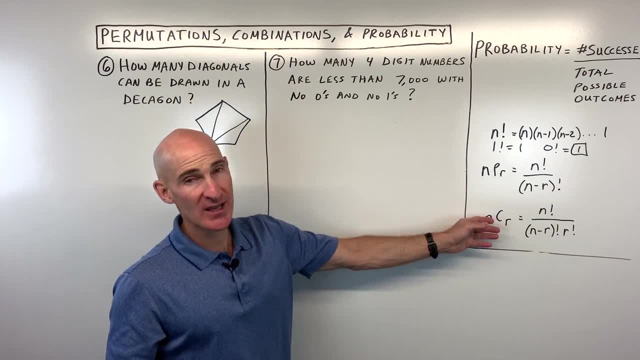 That's the same one handshake. You don't want to double count it, So you're going to want to use combinations, because the order doesn't matter: This vertice and this vertice, or this one and this one- the order doesn't matter. 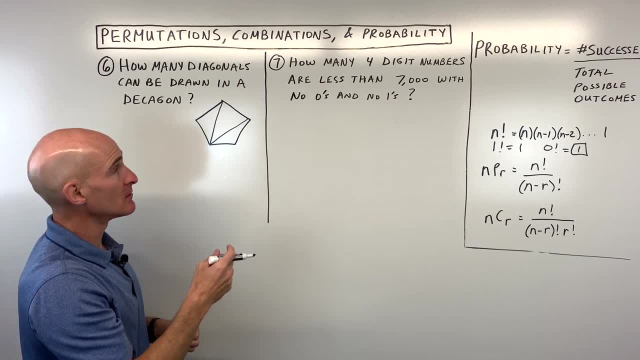 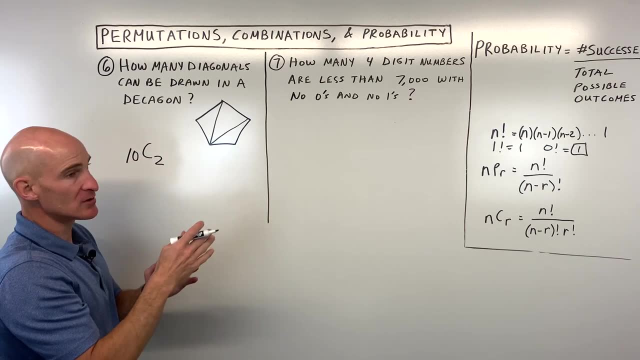 But you're pairing up two vertices out of the okay, in this case it's a decagon, so 10.. So we're saying: out of 10 vertices, how many ways are there to choose two, to make a line segment between the two of them? 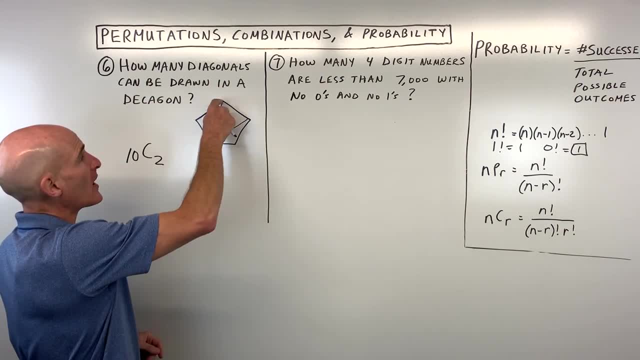 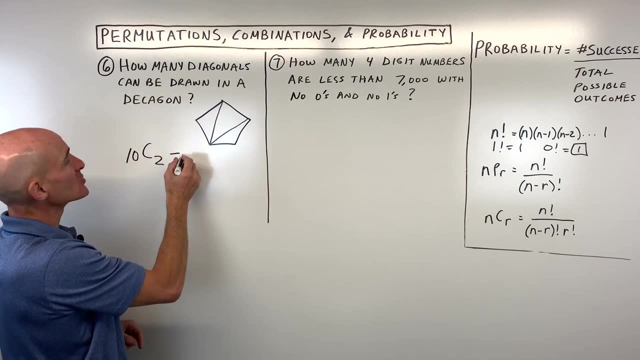 That's a diagonal. But what's interesting about this is we don't want to count the sides of the polygon because those are not diagonal. So this is a segment, but we want to subtract that off. So in a decagon there's 10 sides. We're going to subtract off the 10 sides. 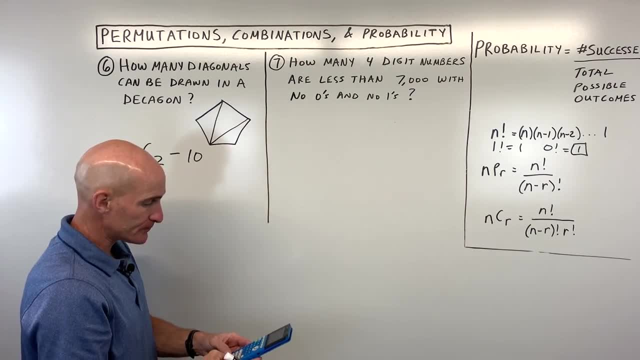 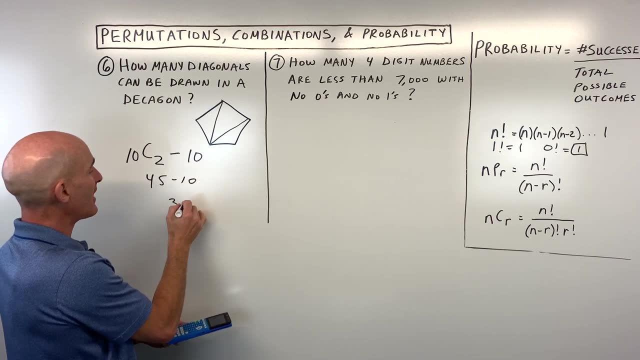 So let's see what that comes out to. So 10C2 is 45 minus 10 would be 35 diagonals. Now you could try to draw them, but again that takes a little bit more time, So that's why I start with a simple. 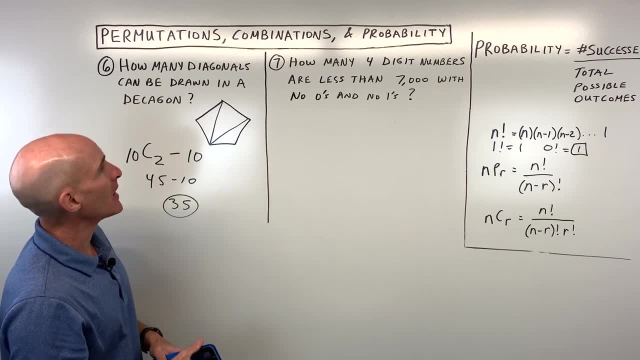 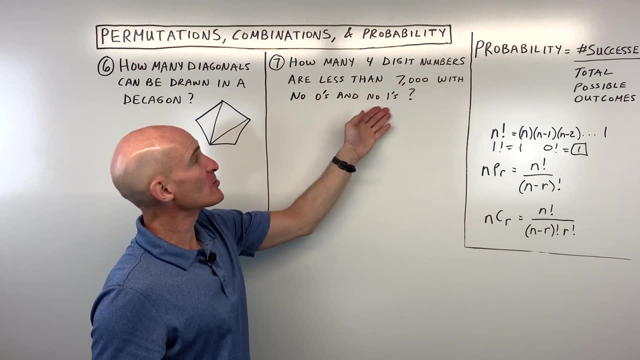 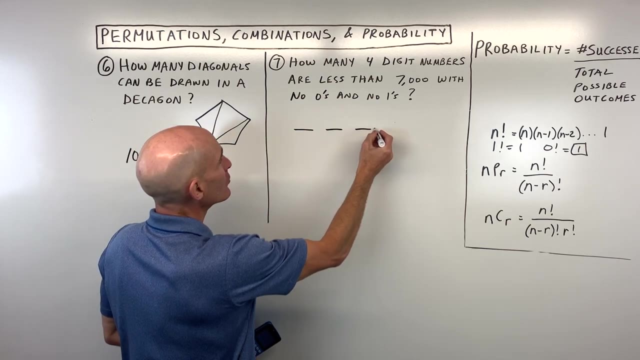 example, and then you can apply that to a more challenging problem. Let's look at number seven now. It says how many four digit numbers are less than 7,000, with no zeros and no ones. Okay, that's an interesting question. So a four digit number. let's diagram this out: One, two, three, four digits, right? 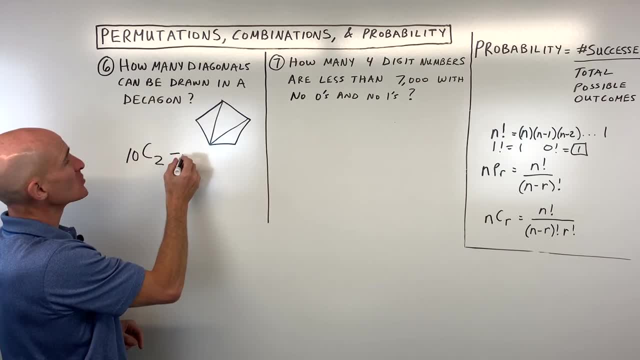 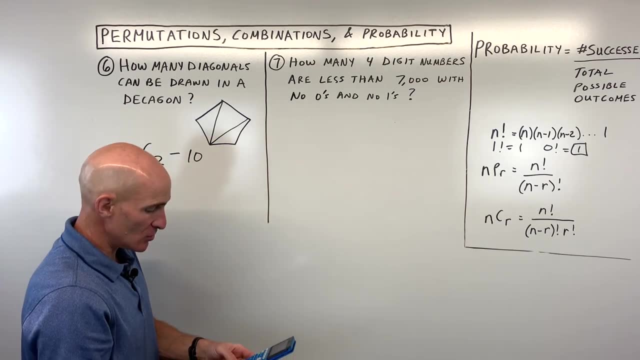 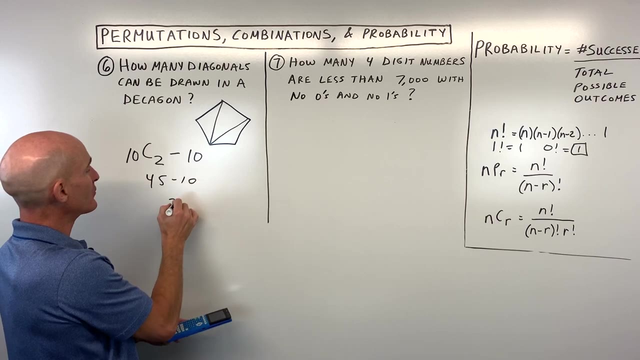 So this is a segment, but we want to subtract that off. So in a decagon there's 10 sides. We're going to subtract off the 10 sides, So let's see what that comes out to. So 10C2 is 45 minus 10 would be 35 diagonals. 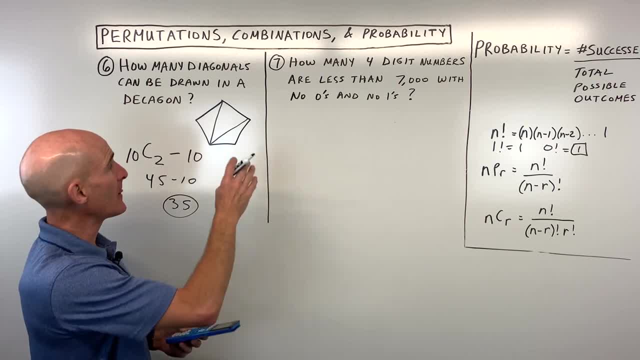 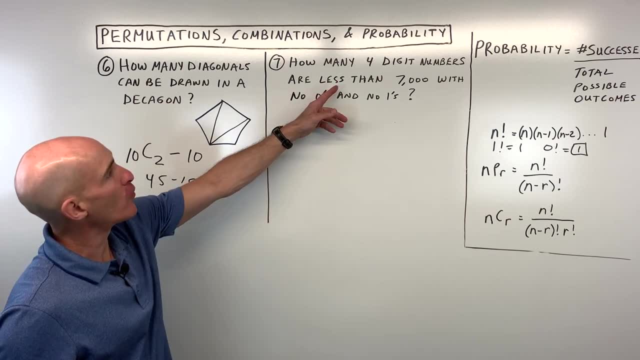 Now you could try to draw, but again that takes a little bit more time. So that's why I start with a simple example, And then you can apply that to a more challenging problem. Let's look at number seven now. It says how many four-digit numbers are less than 7,000, with no zeros and no ones. 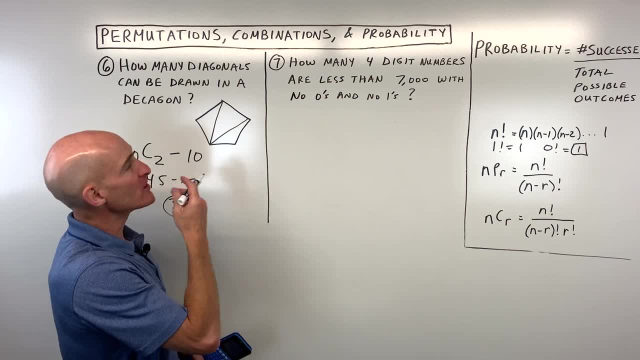 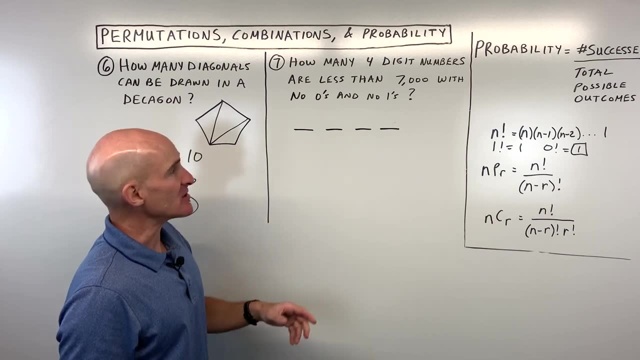 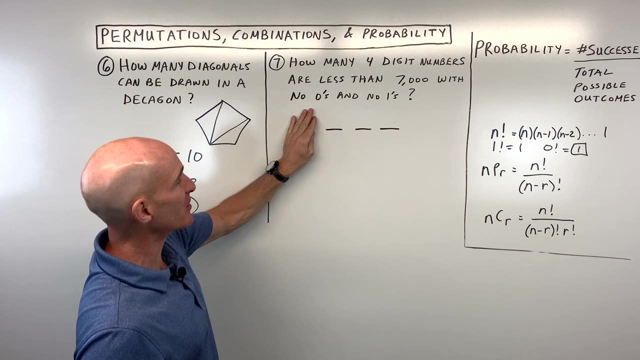 Okay, that's an interesting question. So a four-digit number. let's diagram this out: One, two, three, four digits, right? And you want it to be less than 7,000.. So less than 7,000 means that this has to be well, it can't be zero, because if the first digit was zero, then it's only a three-digit number, right? 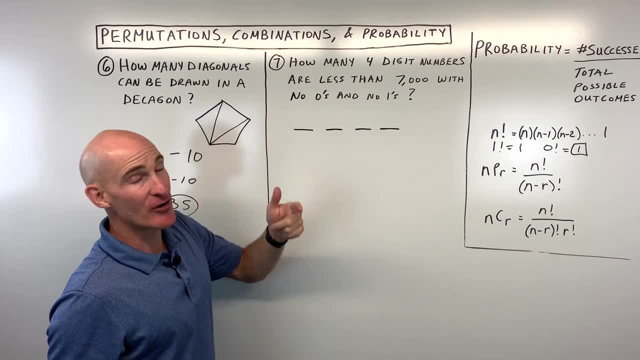 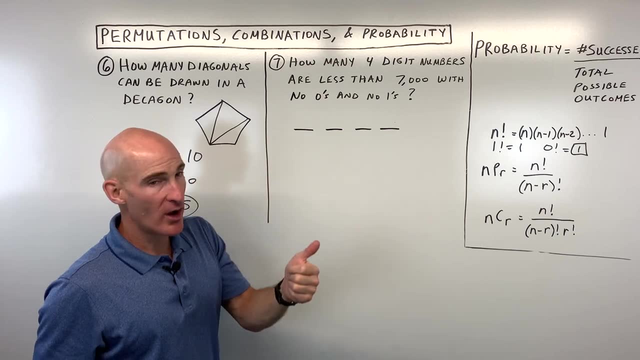 Can't be zero, Can't be eight or nine, because then that would be like 8,000, 9,000.. Can't even be seven, because we want it to be less than 7,000.. So basically, that leaves us with one, two, three, four, five or six. 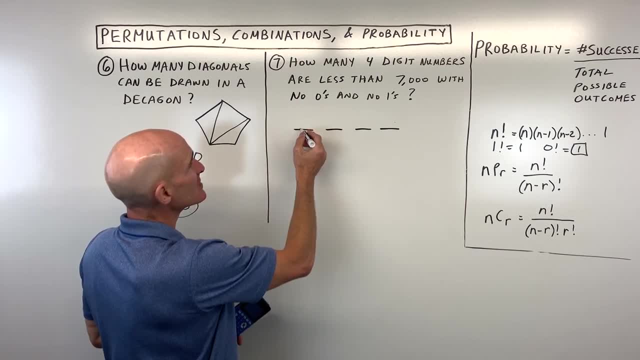 So there's basically six choices for this number, but we don't want any zeros and ones, So one is out. So that means there's only five possibilities for this first digit. Okay times, How many possibilities are there for the second digit? 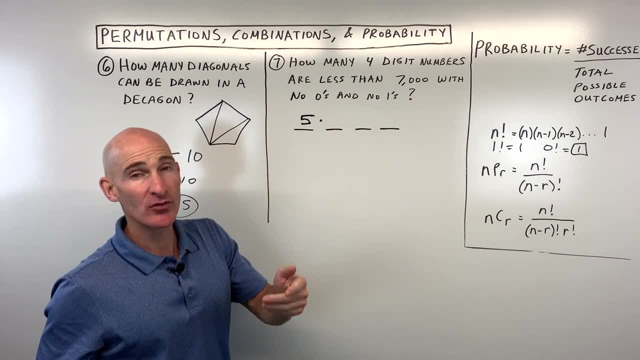 Well, normally there would be ten possibilities: Zero one, two, three, four, five, six, seven, eight, nine. right Zero through nine is ten digits, but we don't want any zeros and we don't want any ones. 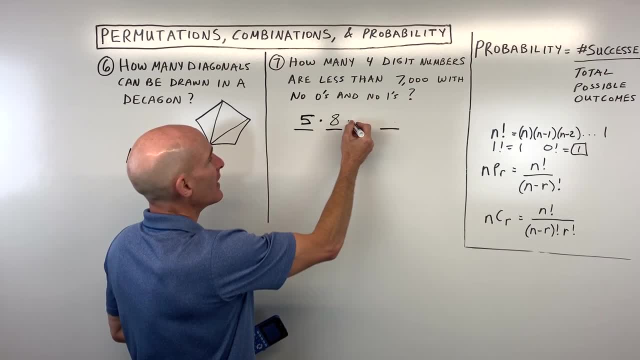 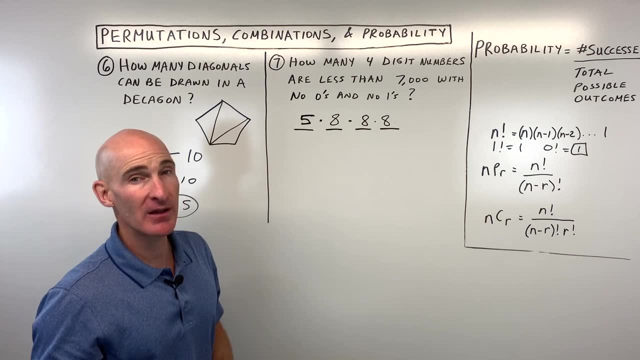 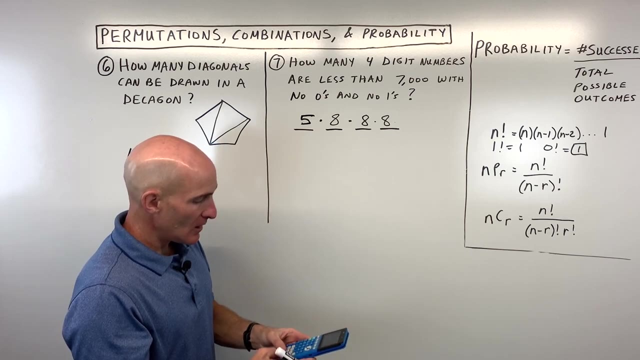 So ten minus two would be eight. Eight possibilities for the third digit and eight possibilities for the fourth digit. And if we multiply those together using that fundamental counting principle or that multiplication counting principle, what does that come out to? Let's see 2,500. 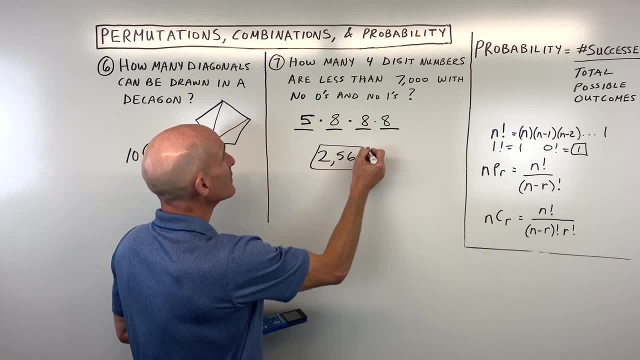 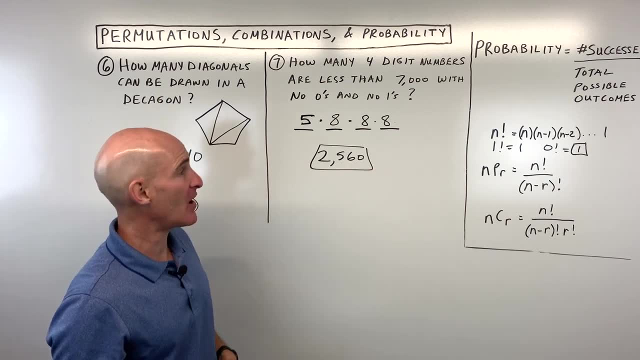 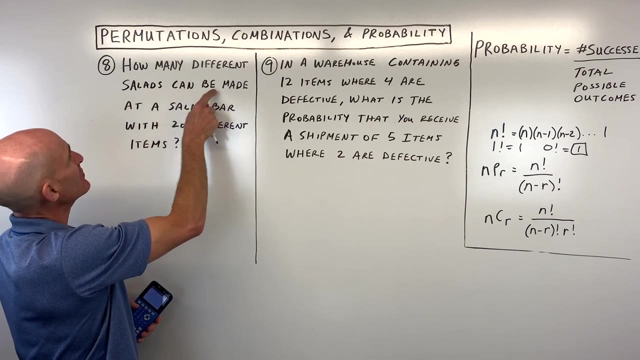 560 numbers are less than 7,000, with no zeros and no ones, So a lot faster than having to actually try to write them down and count all the possibilities. Okay, let's try number eight now. So it says how many different salads can be made at a salad bar with 20 different items. 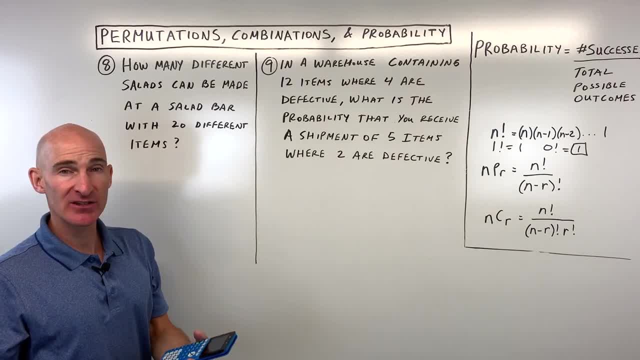 Okay, this is an interesting question. So it's just asking how many different? you walk up to the salad bar, you say how many different salads are possible. Well, it doesn't say that. It doesn't say like you're making a salad with five ingredients, or seven ingredients, or three ingredients. 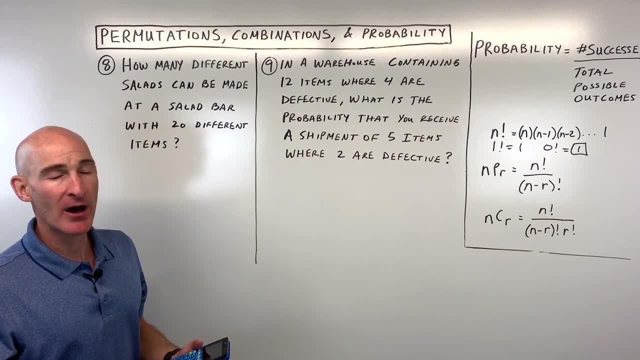 It just says how many different salads can be made. So one way to think about it is: it's kind of like a yes or no question. You walk up to the olives, yes or no, right? So basically there's two choices. 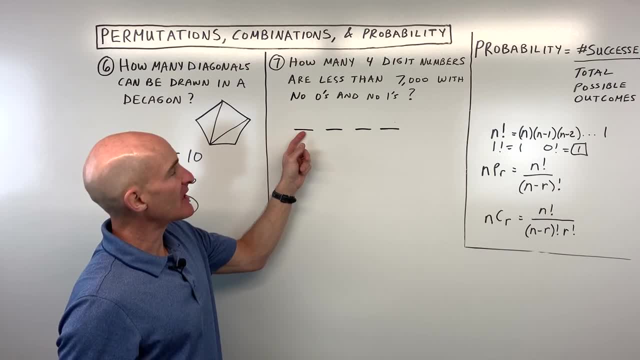 And you want it to be less than 7,000.. So less than 7,000 means that this has to be well, it can't be zero, because if the first digit was zero, then it's only a three digit number. 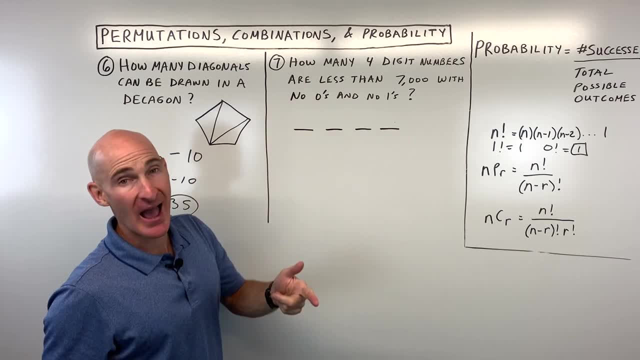 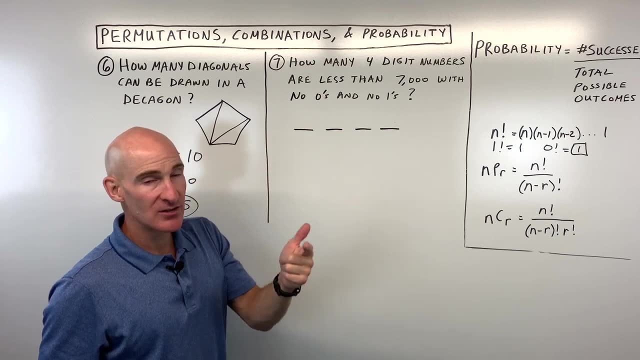 Right, Can't be zero, can't be eight or nine, because then that would be like 8,000, 9,000.. Can't even be seven, because we want it to be less than 7,000.. So basically that leaves us with one, two, three, four, five or six. 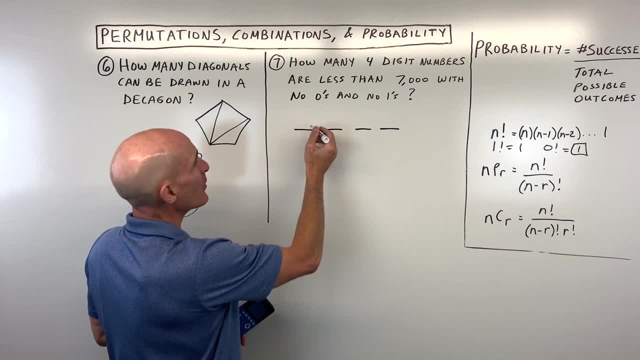 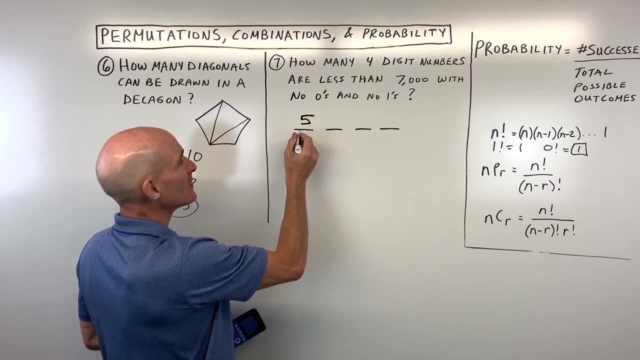 So there's basically six choices for this number, but we don't want any zeros and ones, So that so one is out. So that means there's only five possibilities for this first digit. Okay times, how many possibilities are there for this? 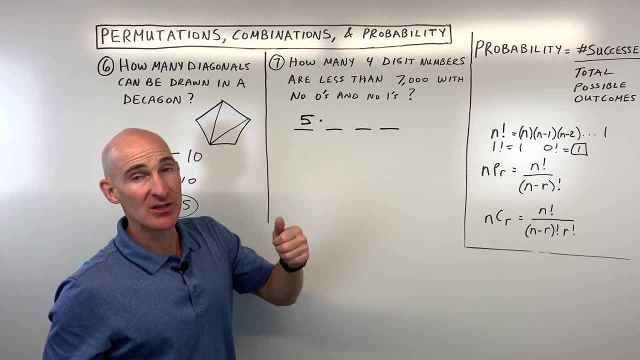 For the second digit. Well, normally there would be 10 possibilities: zero, one, two, three, four, five, six, seven, eight, nine. right Zero through nine is 10 digits. but we don't want any zeros and we don't want any ones. 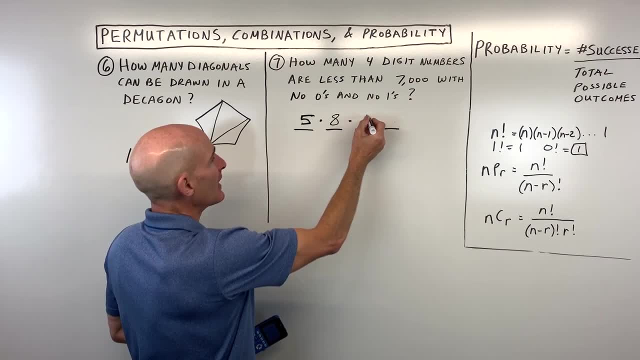 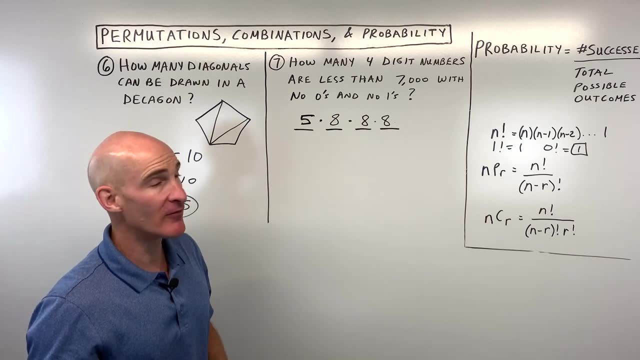 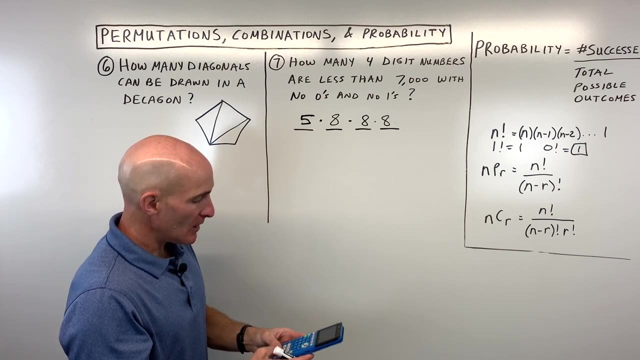 So 10 minus two would be eight. Eight possibilities for the third digit and eight possibilities for the fourth digit. And if we multiply those together using that fundamental counting principle or that multiplication counting principle, what does that come out to? Let's see. 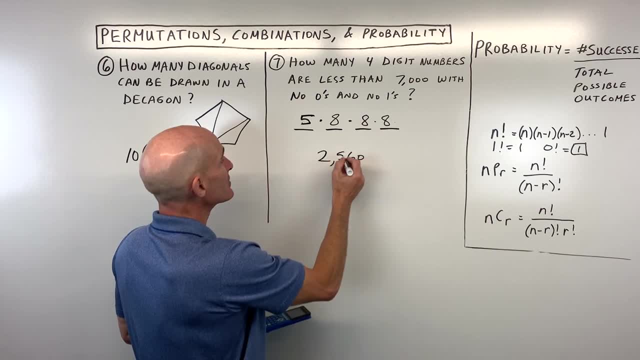 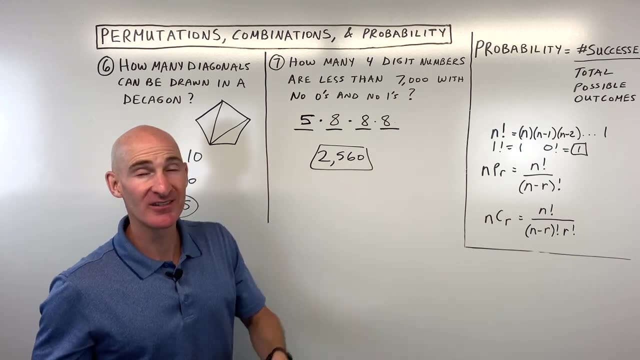 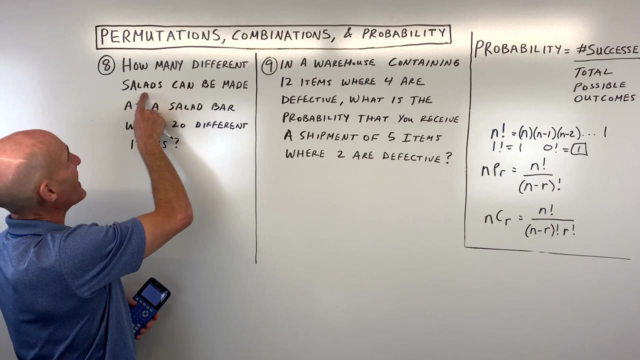 2,560.. Numbers are less than 7,000 with no zeros and no ones, So a lot faster than having to actually try to write them down and count all the possibilities. Okay, let's try number eight now. So it says how many different salads can be made at a salad bar with 20 different items. 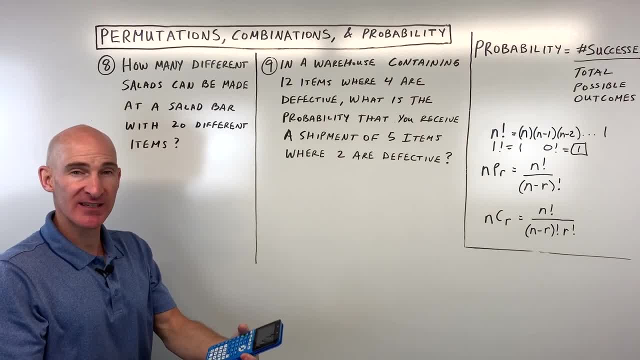 Okay, this is an interesting question. So it's just asking how many different? you walk up to the salad bar, you say how many different salads are possible. Well, it doesn't say like you're making a salad, but it does say how many different salads are possible. 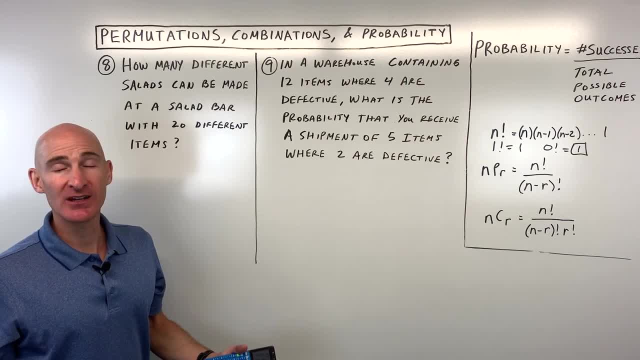 Well, it doesn't say like you're making a salad, but it does say how many different salads are possible. So a salad with five ingredients or seven ingredients, or three ingredients. So a salad with five ingredients or seven ingredients, or three ingredients. 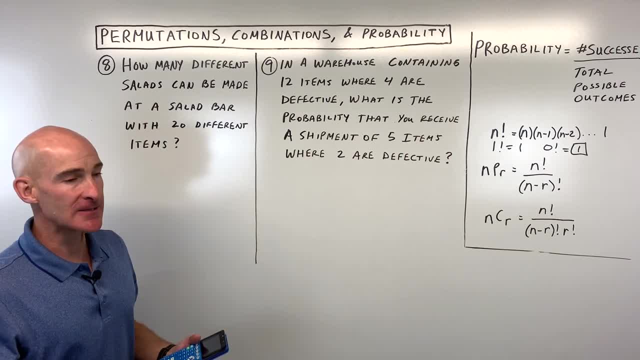 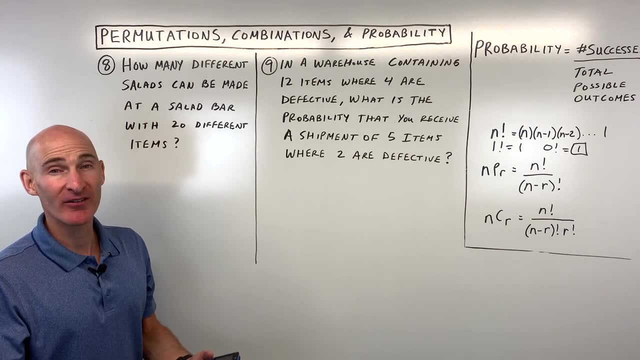 It just says how many different salads can be made. So one way to think about it is: it's kind of like a yes or no question. you walk up to the uh olives, yes or no, right? So basically there's there's two choices. 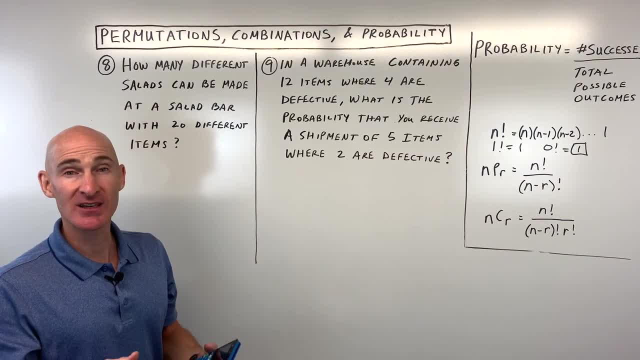 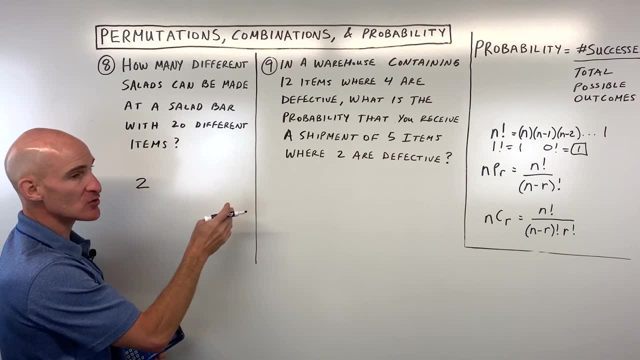 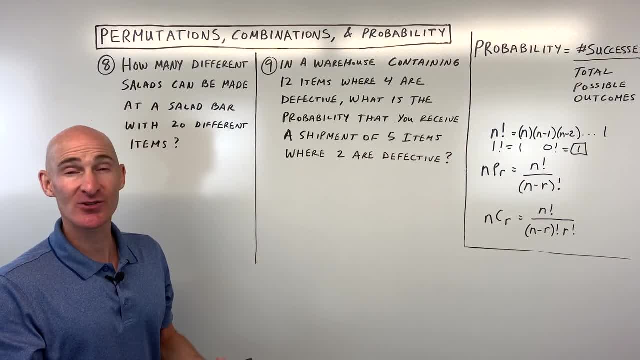 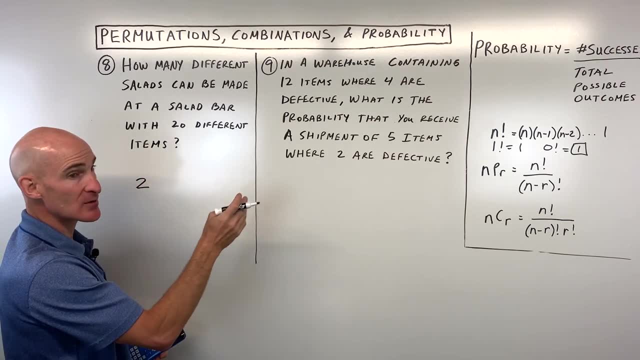 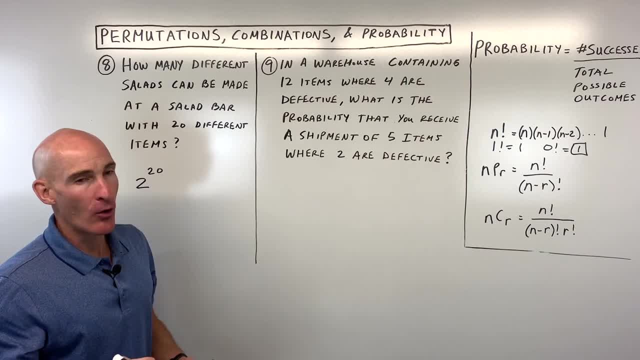 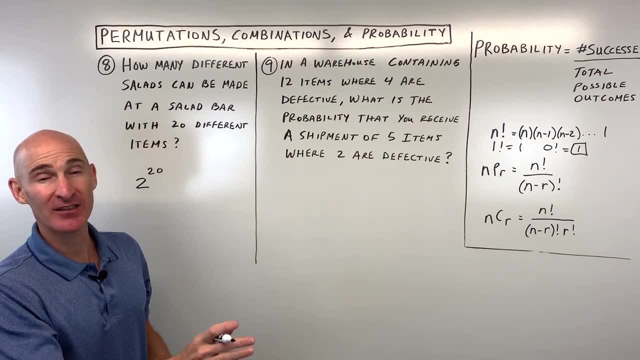 That's two to the 20th power. Now what happens if you said, no, I don't want tomatoes. No, I don't want lettuce. No, I don't want this. Okay, You say no to everything? Well then, you really wouldn't have a salad at all. 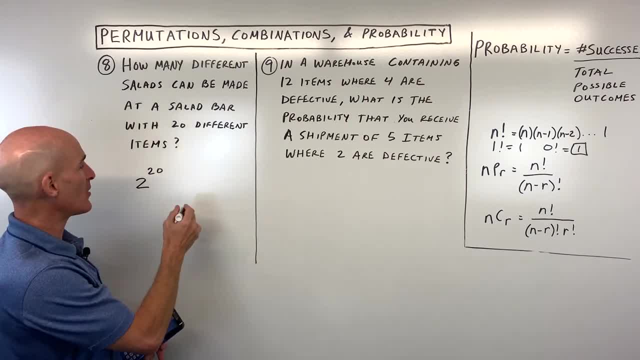 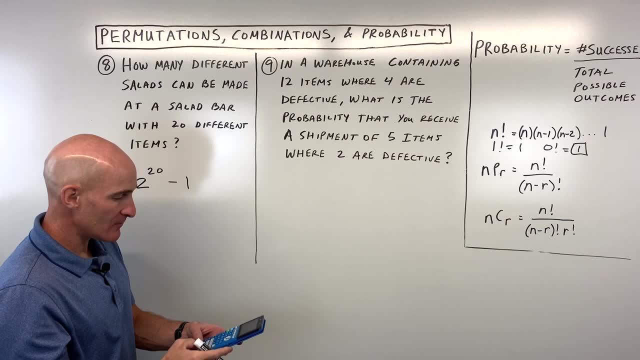 So that particular outcome: we're going to say that's no salad, We're going to subtract that one off. Okay, So we could argue that that's technically not a salad at all. So let's see what this comes out to. So two to the 20th. 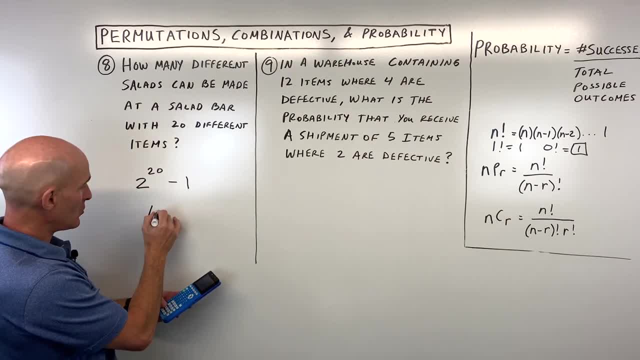 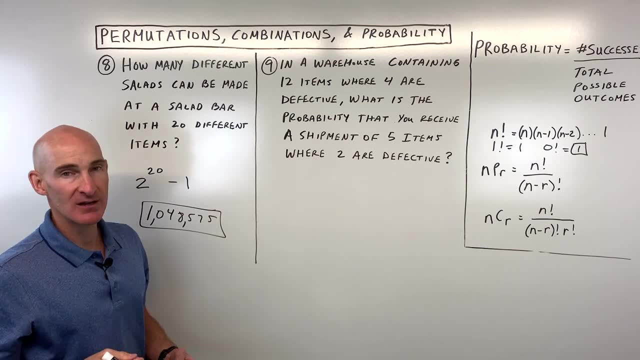 Okay, Minus one, So this is 1, 0,, 4,, 8,, 5,, 7, 8.. 5, 7, 5.. So about a million different salads that you could create. Now again, you know, sometimes I know students struggle with this- permutations, combinations, probability. 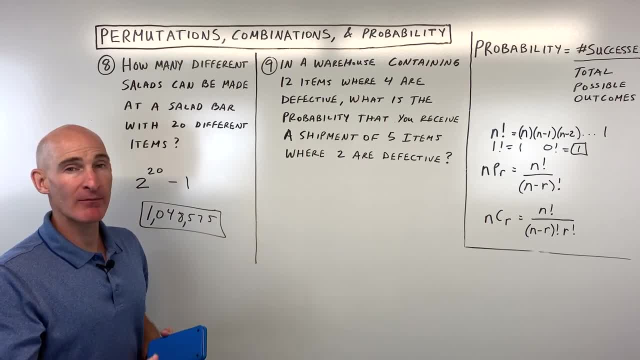 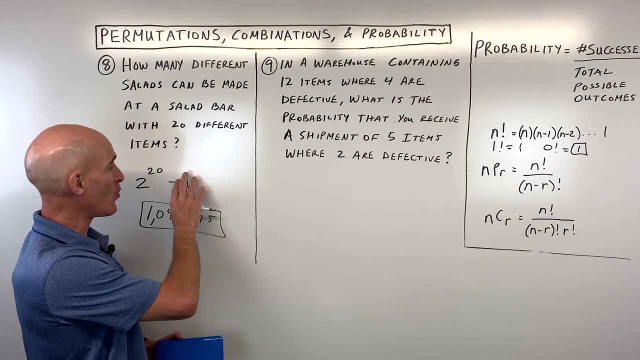 But if you can understand these basic problems that we're going through, you can apply them to other problems, Like say, for example, it was like a true and false test. How many ways could you answer this true and false test? You wouldn't subtract one, but you would say: oh, there's 20 questions. 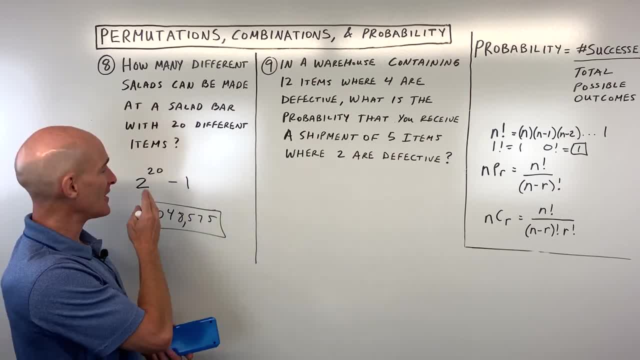 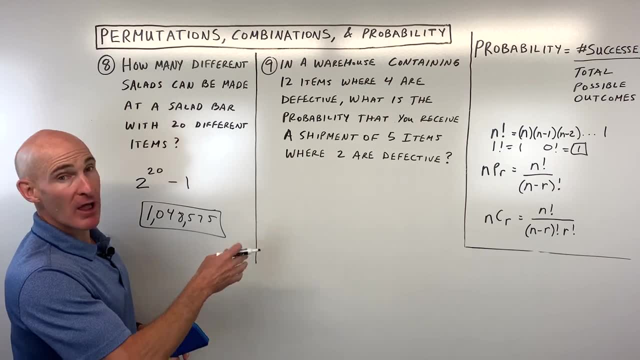 I could pick true or false for the first question, true or false for the second question. That's two times Two times two, two to the 20th. So I hope this is encouraging to you to try to apply this to other problems. 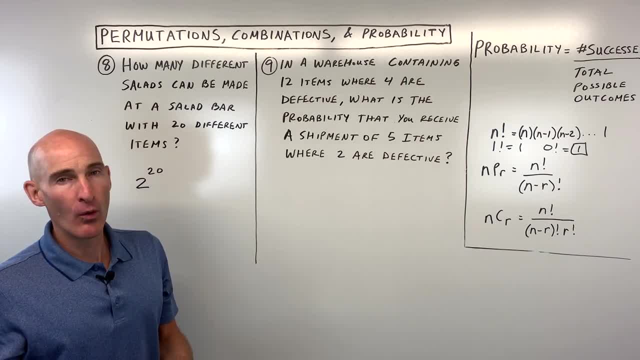 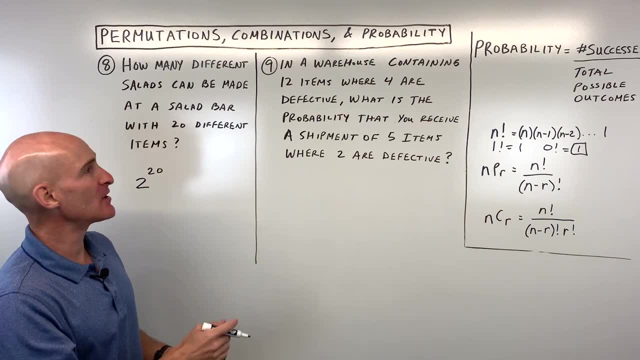 Okay, power. Now what happens if you said, no, I don't want tomatoes, no, I don't want lettuce, no, I don't want this. Okay, you say no to everything. Well then, you really wouldn't have a salad at all. So that particular outcome, we're gonna say: 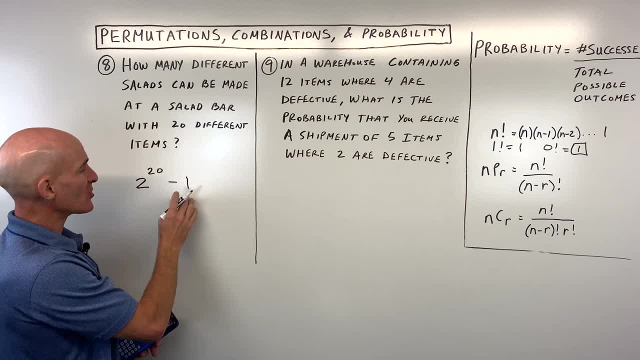 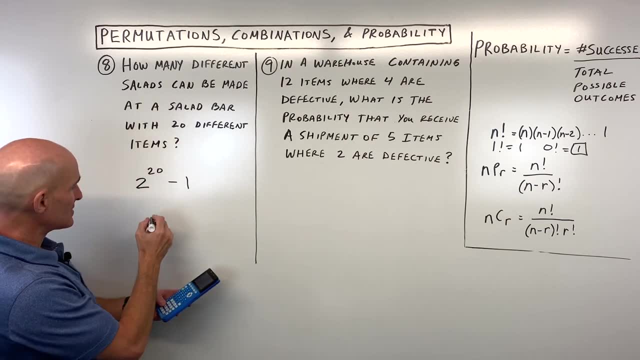 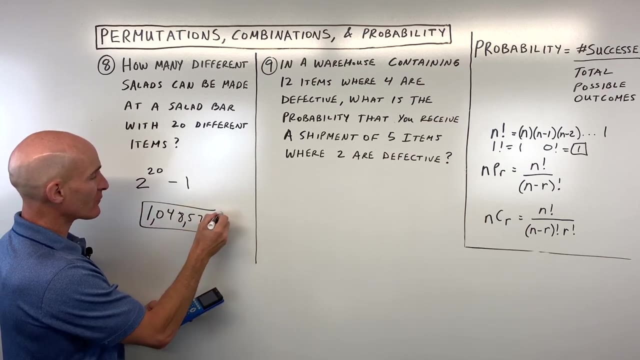 that's no salad. We're gonna subtract that one off, Okay. so we could argue that that's technically not a salad at all. So let's see what this comes out to. So 2 to the 20th, Okay, minus 1.. So this is 1, 0,, 4, 8, 5, 7, 5.. So about a million different. 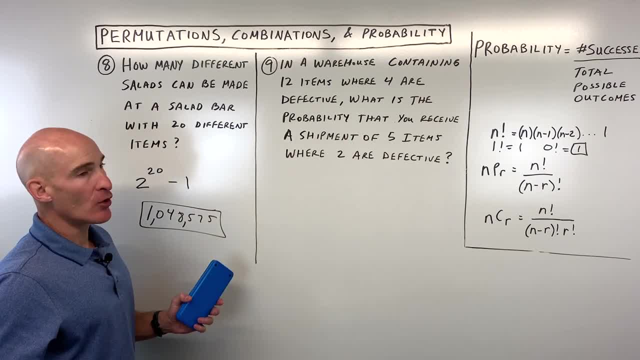 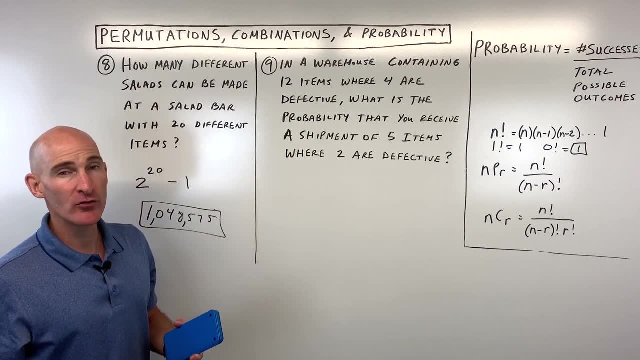 salads that you could create. Now again, you know, sometimes I know students struggle with this- permutations, combinations, probability- But if you can understand these basic problems that we're going through, you can apply them to other problems Like say, for example, it was like a true and false test- How. 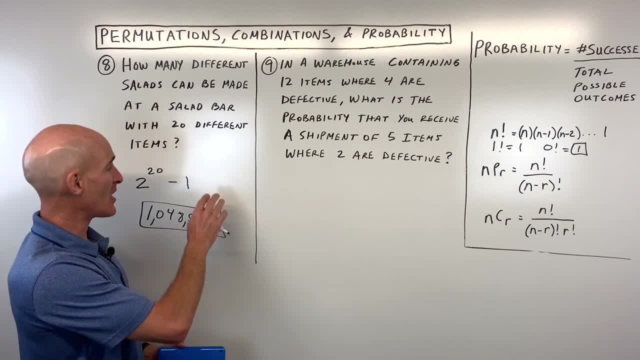 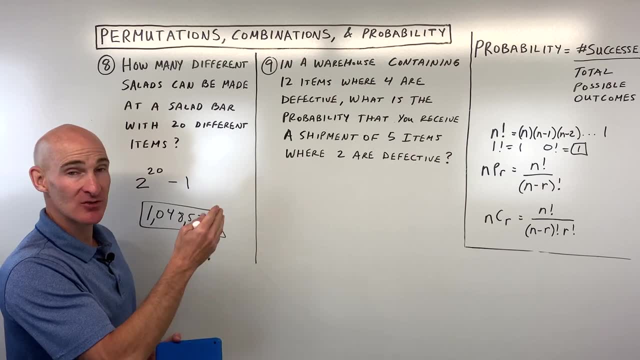 many ways could you answer this true and false test? You wouldn't subtract one, but you would say: oh, there's 20 questions, I could pick. true or false for the first question, true or false for the second question. That's 2 times 2 times. 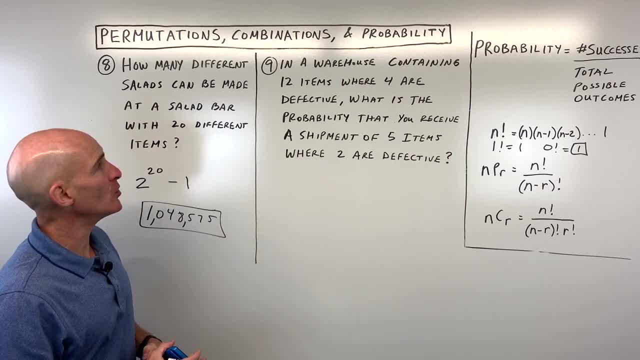 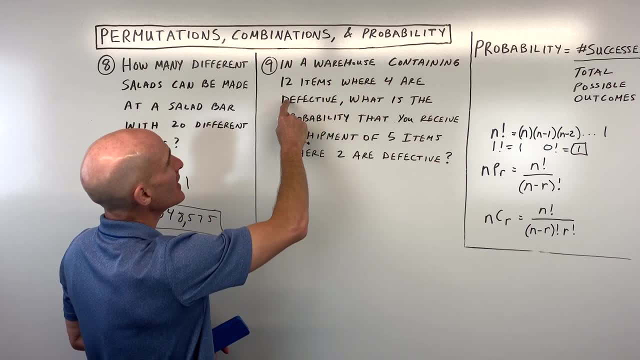 2, 2 to the 20th. So I hope this is encouraging to you to try to apply this to other problems. So for number nine, it says: in a warehouse containing 12 items where four are defective like broken right. Okay, they're bad. What is the? 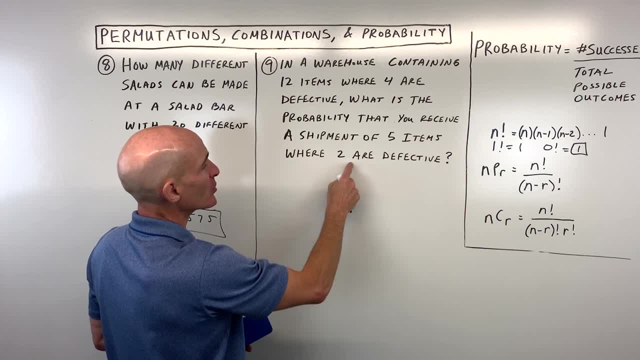 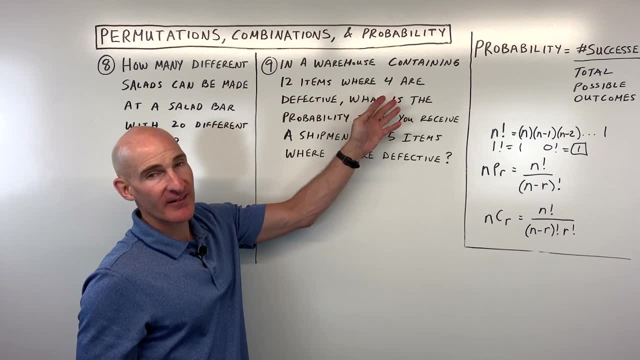 probability that you receive a shipment of five items, where two are defective or bad. So if there are nine items that are defective and if there are 10 items that are, there's 12 items total. that means there's eight good and four bad. right, and you're receiving a. 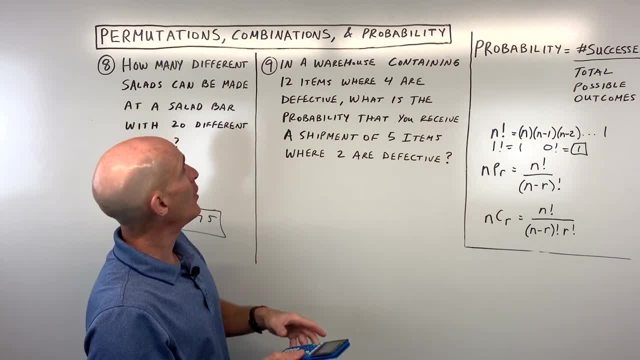 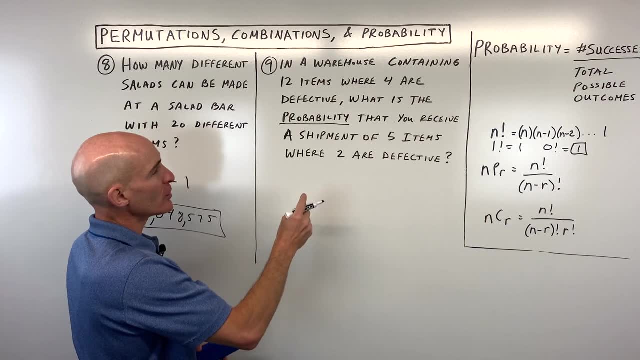 shipment, okay, of five items and it wants to know what is the probability. okay, remember, that's the number of successes over the total possible, and what we're looking for is that two are defective. okay, so let's think about it. so two are defective. so, out of the four defective items at this, 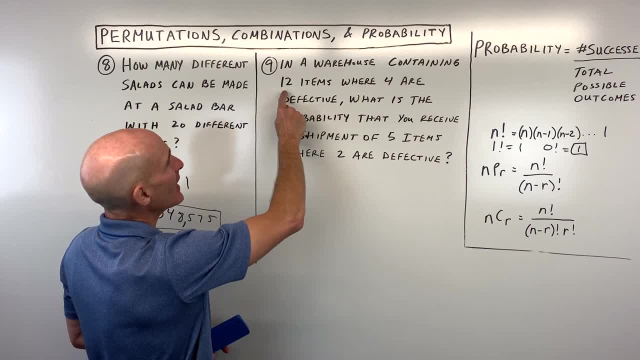 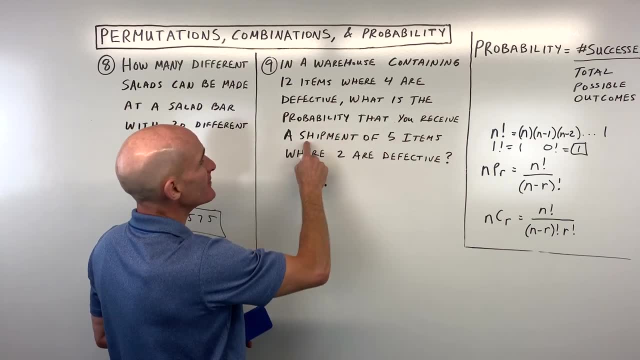 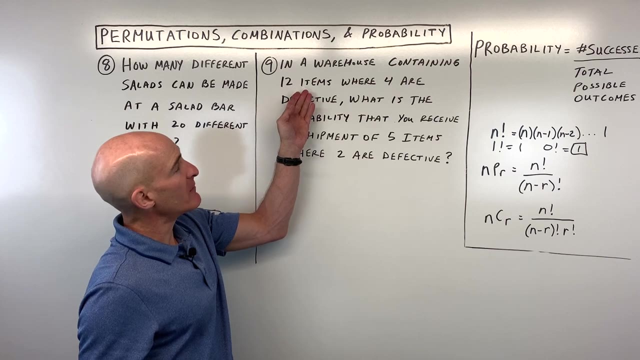 So for number nine, it says: in a warehouse containing 12 items where four are defective, like broken right, Okay, they're bad. What is the probability that you receive a shipment of five items where two are defective or bad? So if there's 12 items total, that means there's eight good and four bad, right. 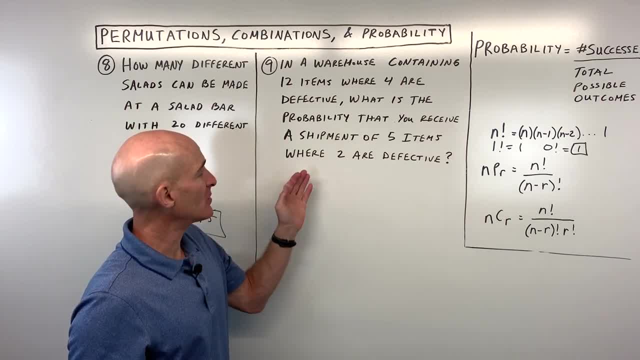 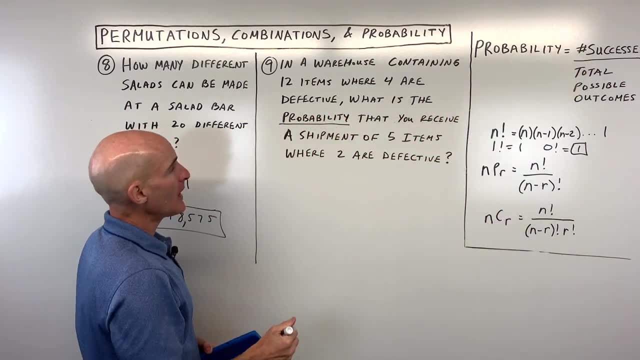 And you're receiving a shipment, okay, of five items and it wants to know what is the probability. Okay, remember, that's the number of successes over the total possible, And what we're looking for is that two are defective. Okay, so let's think about it. 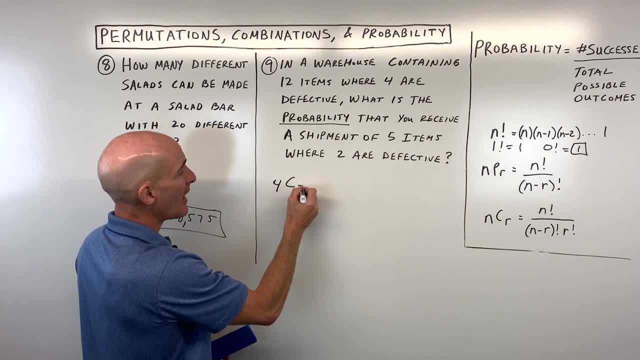 So two are defective. So out of the four defective items at this warehouse, how many ways are there to get two? Now we're using combinations because it doesn't matter the order. We're assuming these are all the same kind of widget. whatever, that is okay. 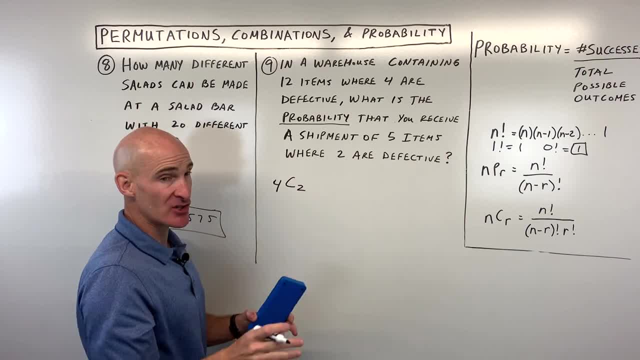 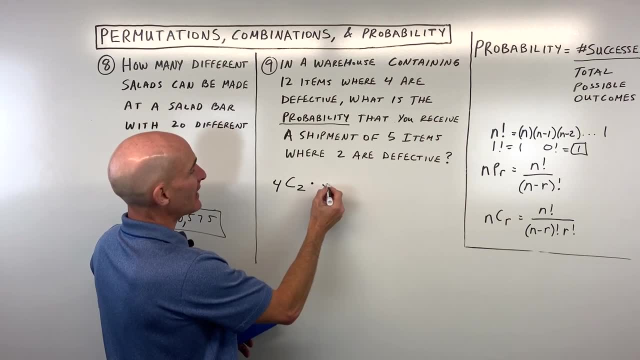 warehouse. how many ways are there to get two? now we're using combinations because it doesn't matter the order. we're assuming these are all the same kind of widget, whatever, that is okay. and then out of the eight good ones, how many ways are the to receive three of the good ones out of the eight? 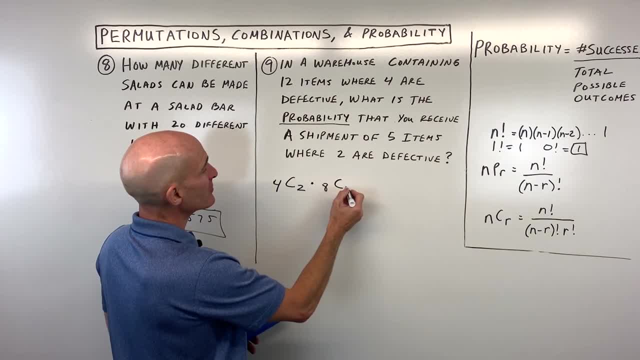 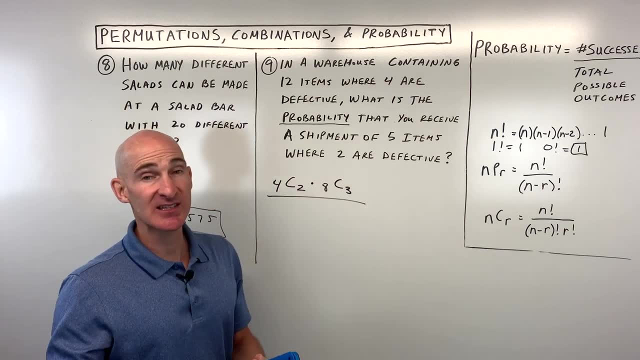 And then out of the eight good ones. how many ways are there to receive three of the good ones out of the eight good ones? That's going to give us the total number of successes. When I say success, it's like what you're looking for, what you want. 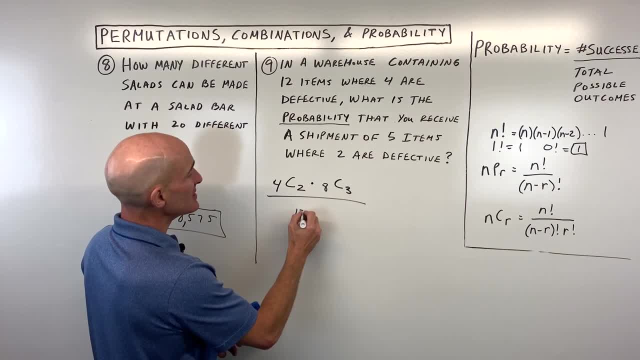 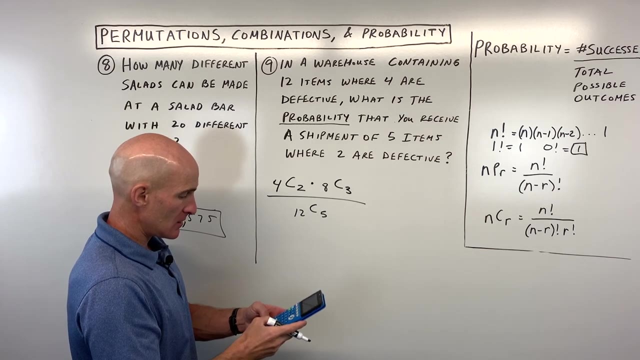 Divided by the total possible ways of receiving five items from this warehouse, that has 12 of these items, Okay. so this is the total possible, So let's see what that comes out to. So we have four, Okay, Uh-huh. 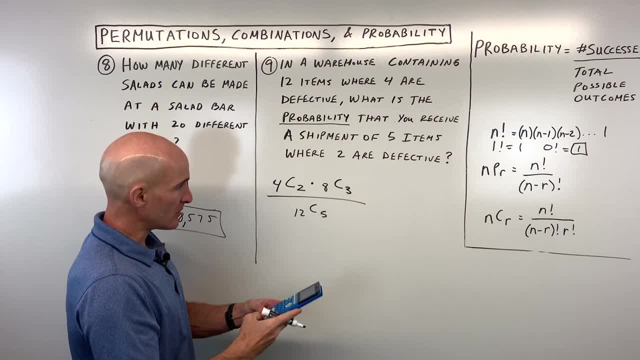 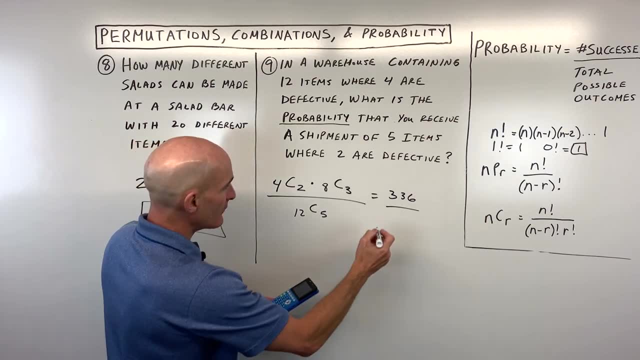 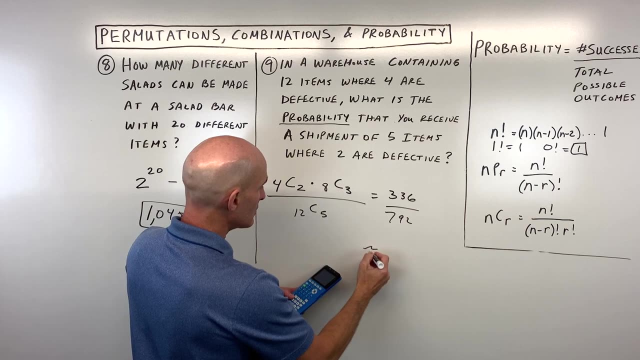 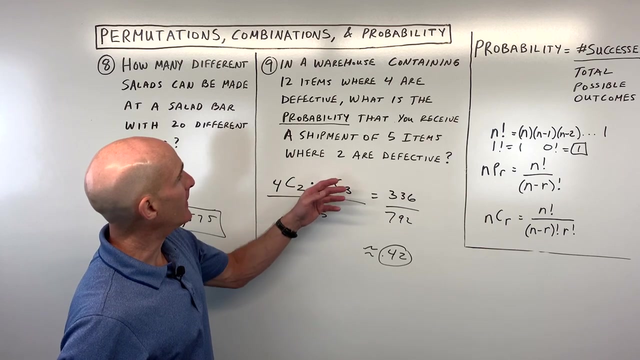 Put this on the calculator, Okay. so this is coming out to 336 divided by 792, which is about 0.42.. So it's about a 42% chance that you would receive two defective and three good For number 10,. 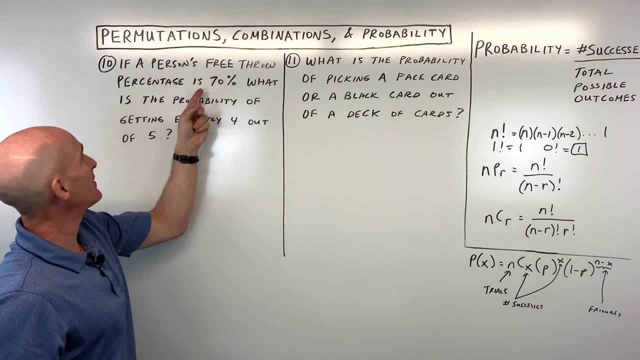 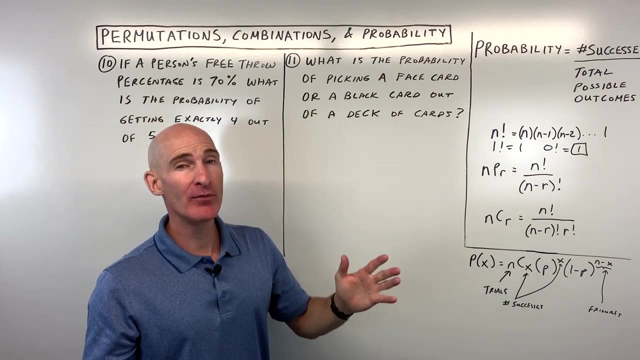 we have. if a person's free throw percentage is 70%, what is the probability of getting exactly four out of five free throws? So the percentage of scoring is 70%, That's a 0.70.. And what we're going to do is let's talk about this binomial probability. 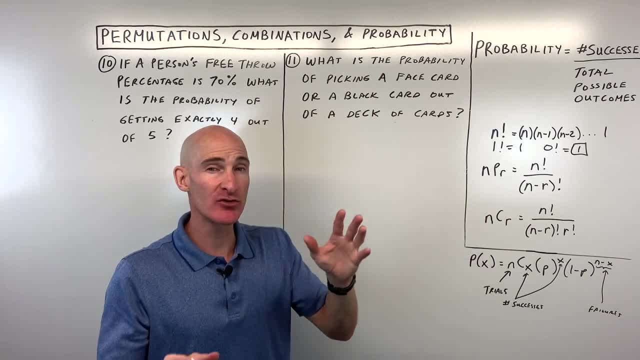 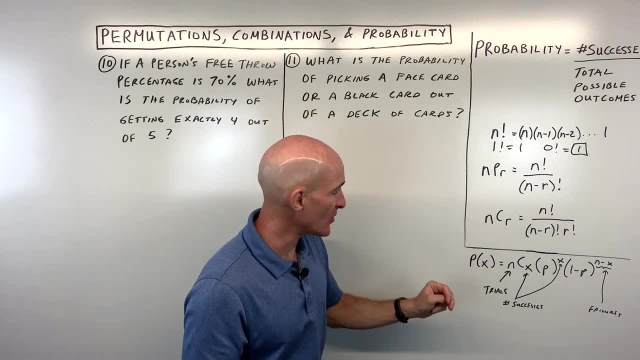 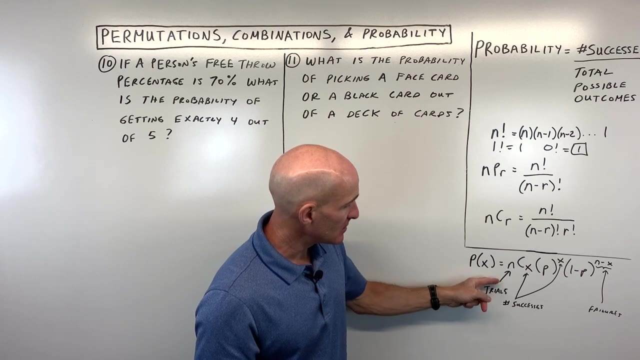 So binomial means like a bias two, There's two possibilities: Either you make the free throw or you miss the free throw. So it's like win or lose, succeed or fail. There's only two options. right, And so the probability okay. when it's a binomial like this, you take the number of trials, okay. 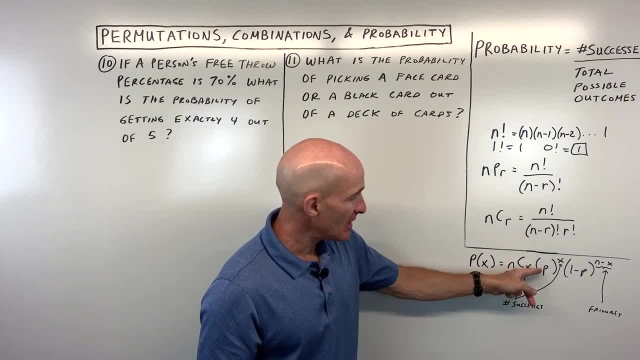 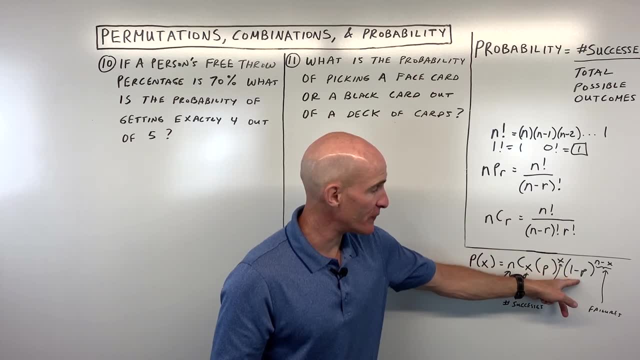 and the number of successes out of that number of trials, the probability of success, the number of those successes, one minus the probability of success, which gives us our probability of failure and the number of those failures. So the way we would set this one up is we'd say: there's five shots that you're taking. 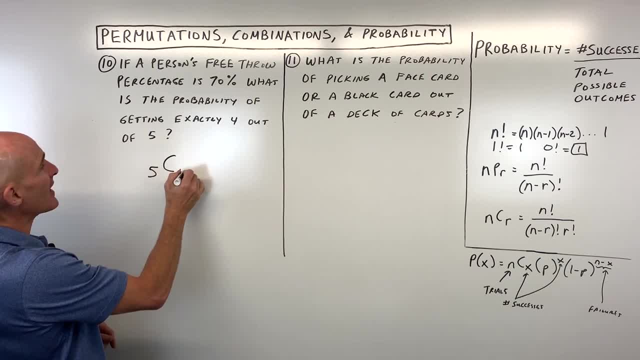 That's the five trials And we're looking to get exactly four free throws, four successes. The probability of making the free throw is 70%, or 0.7, 0.70.. We want four of those And the probability of missing is 30%. 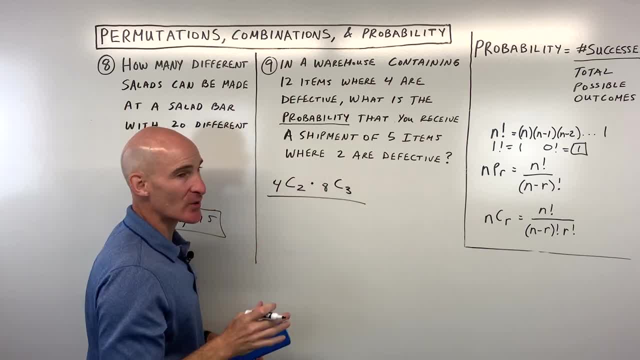 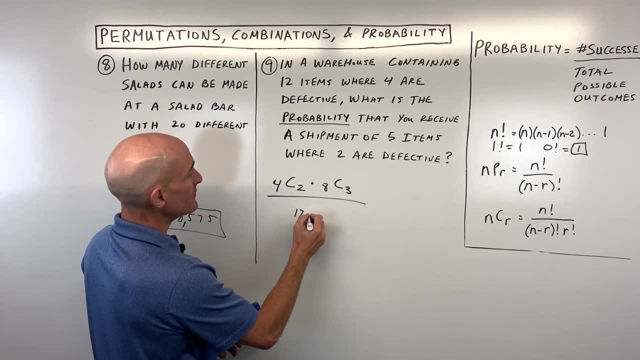 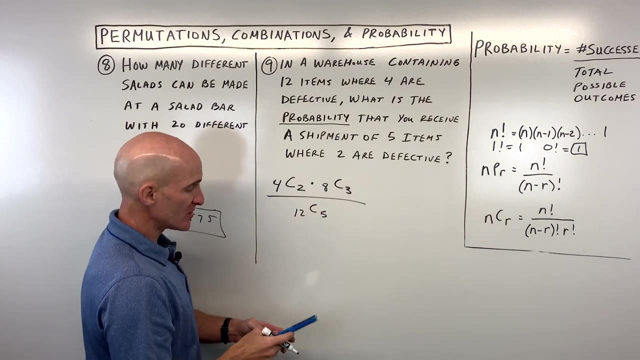 good ones. that's going to give us the total number of successes. when i say success, it's like what you, what you're looking for, what you want, divided by the total possible ways of receiving five items from this warehouse that has 12 of these items. okay, so this is the total possible. so let's see. 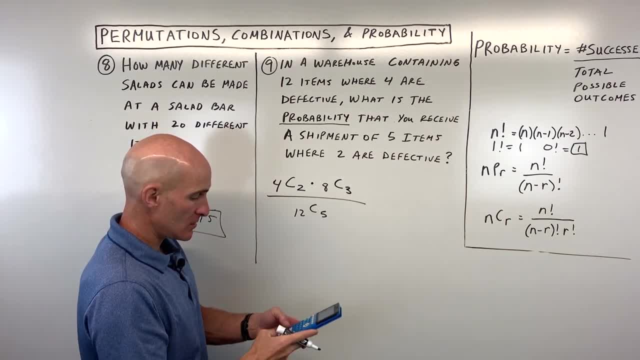 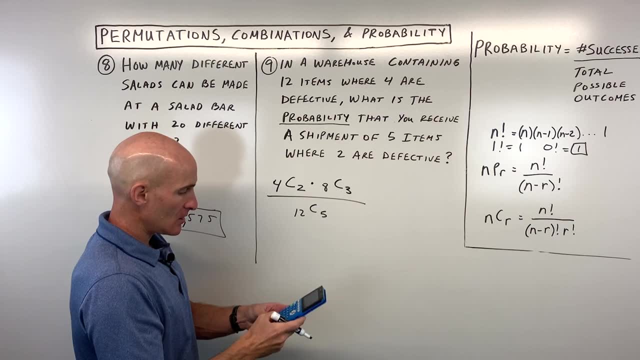 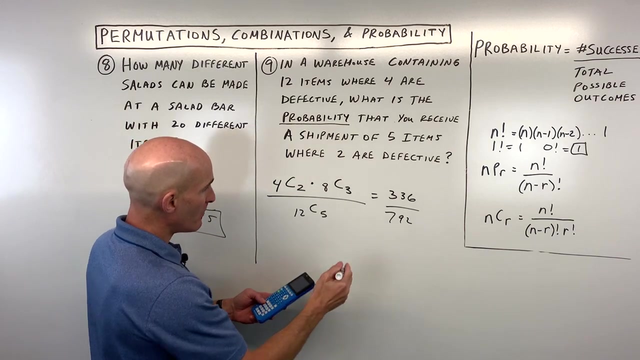 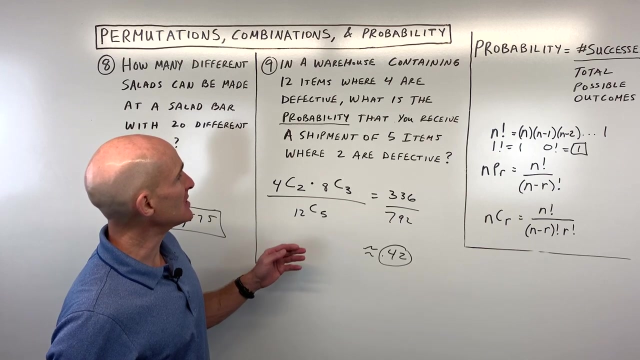 what that comes out to. so we have four ули k case. this is coming out: two, three hundred and thirty six divided by seven hundred and ninety two, which is about 0.4 to. it's about a forty two percent chance that you would receive 2 defective and 3 good For number 10 we have. if a person's free. 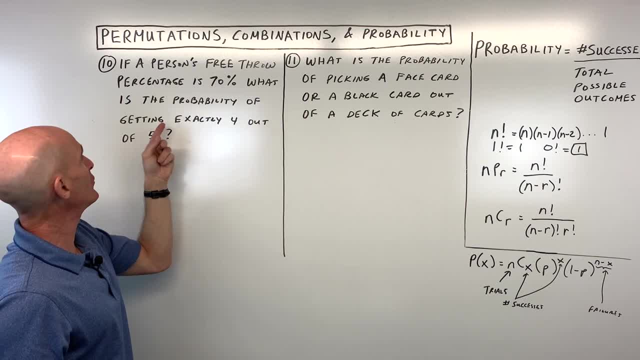 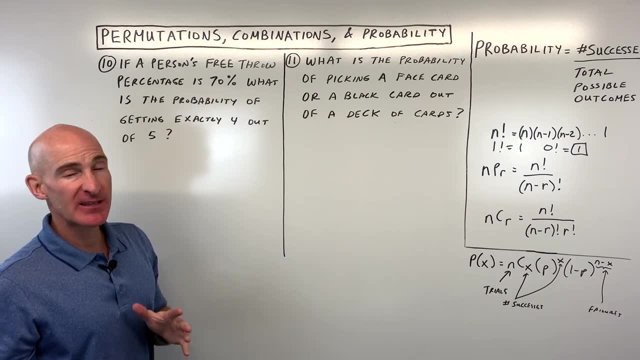 throw percentage is 70%, what is the probability of getting exactly 4 out of 5 free throws? So the percentage of scoring is 70%. that's a point seven zero, and what we're going to do is let's talk about this binomial probability. So 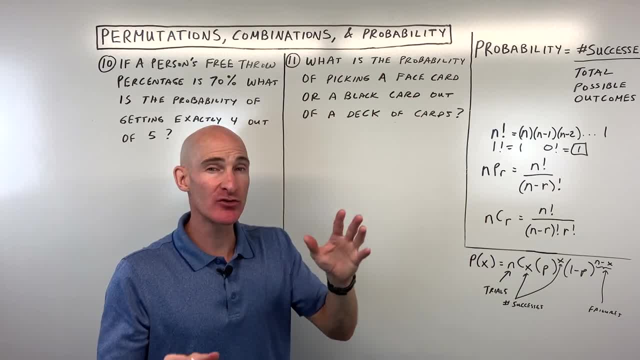 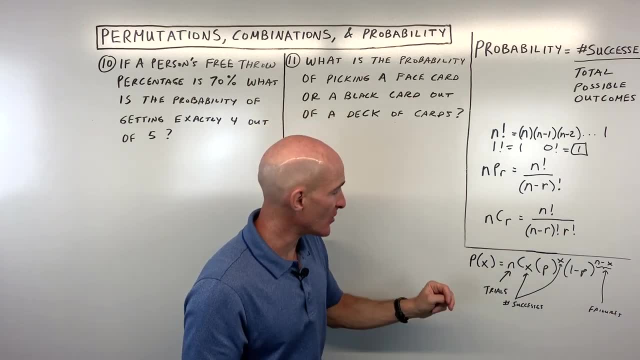 binomial means like a bias two. There's two possibilities: either you make the free throw or you miss their free throw. So it's like win or lose, succeed or fail. There's only two options, right, and so the probability okay when it's a. 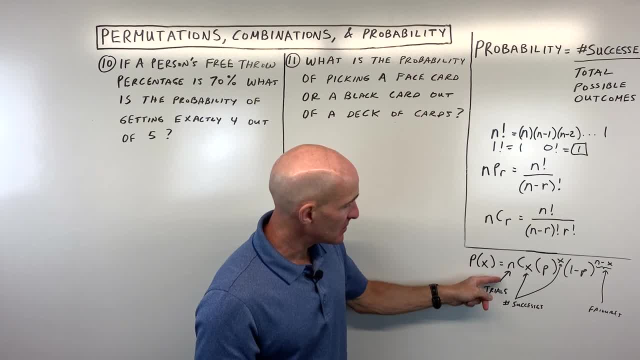 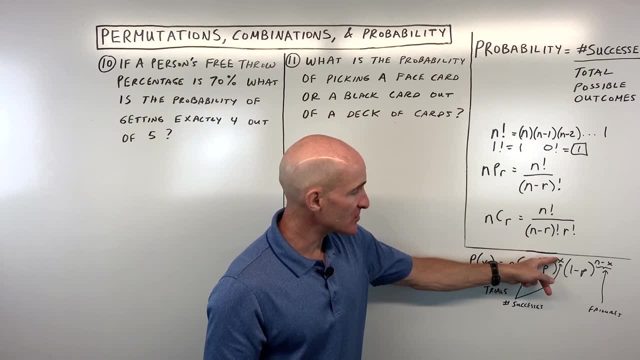 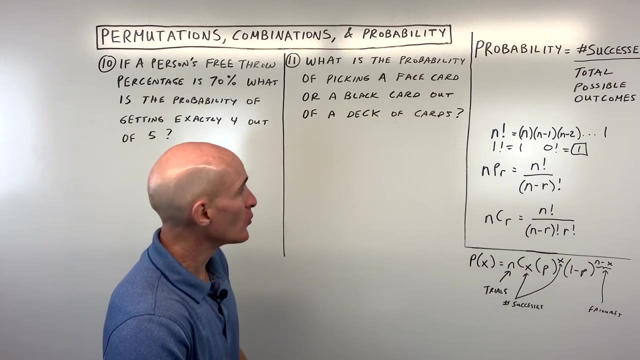 binomial like this: you take the number of trials, okay, and the number of successes out of that number of trials, the probability of success, the number of those successes, 1 minus the probability of success, which gives us our probability of failure and the number of those failures. So the way we would set this, 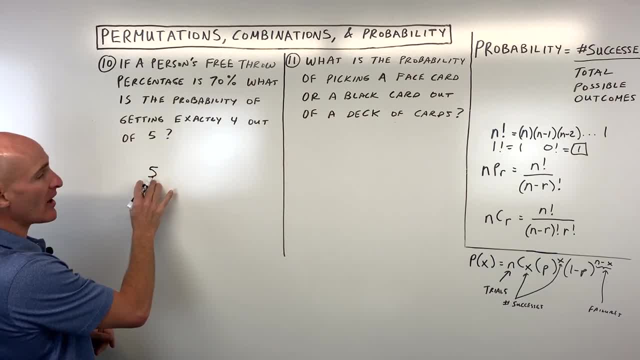 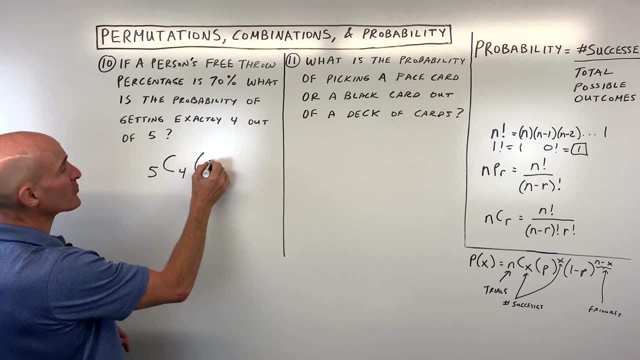 one up is: we'd say there's a five shots that you're taking, that's the five trials, and we're looking to get exactly four free throws, four successes. The probability of making the free throw is 70%, or point seven, point seven, zero. We want four of those and the probability 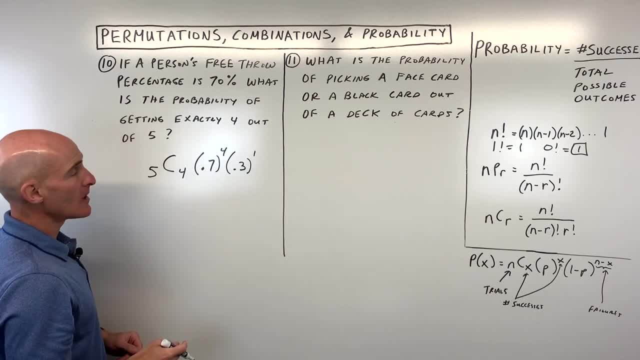 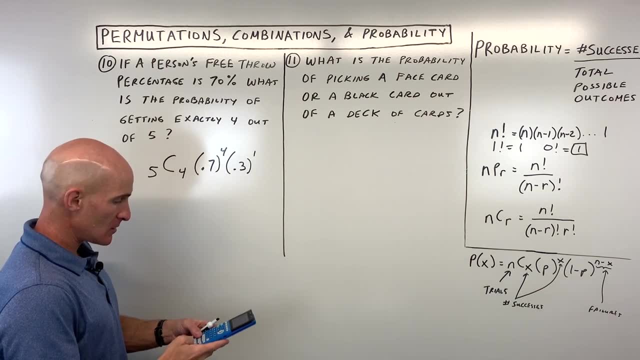 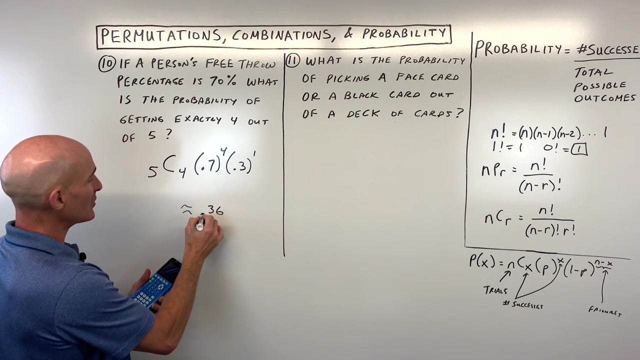 of missing is 30% and we want one of those. So let's see what that comes out to: 5c4, okay, times point seven to the fourth times, point three to the firstokay. so this is coming out to 0.3, approximately 36%, or we just say, as a probability, approximately 0.36. so 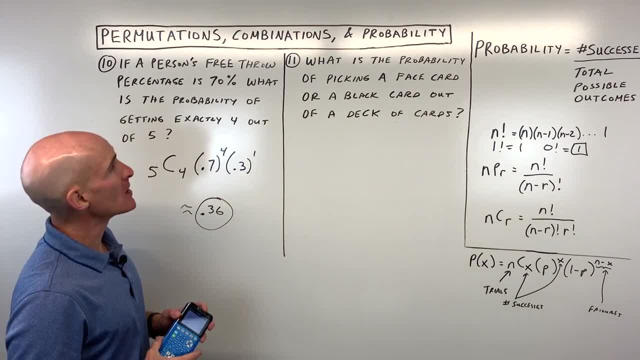 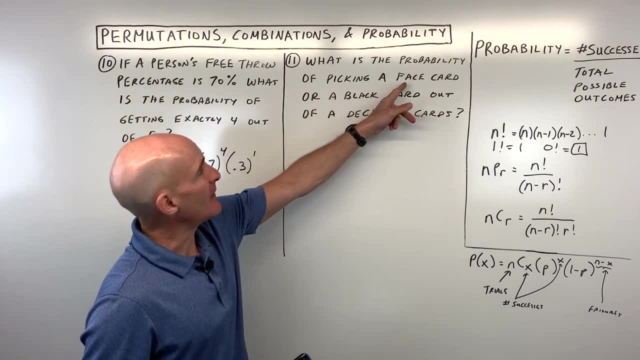 that's binomial probability when there's only two possible outcomes. Okay, now for number 11 of the success or failure right winner lose. For number 11: what is the probability of picking a face card or a black card out of a deck of cards? 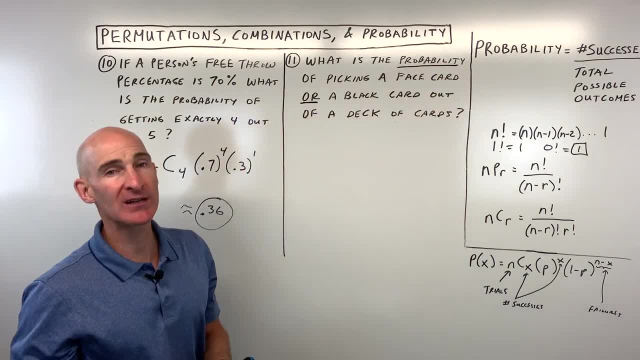 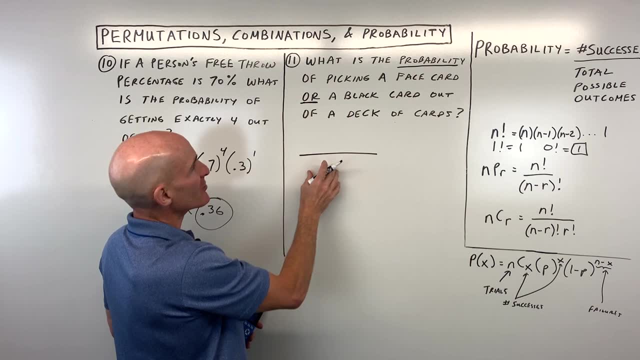 Now here we are talking about a block out of a deck of cards. Now here we're brought about probability and we talked about the breakdown of face cards- or not face cards but a deck of cards- earlier. Remember, when it's probability, it's going to be a fraction out of. 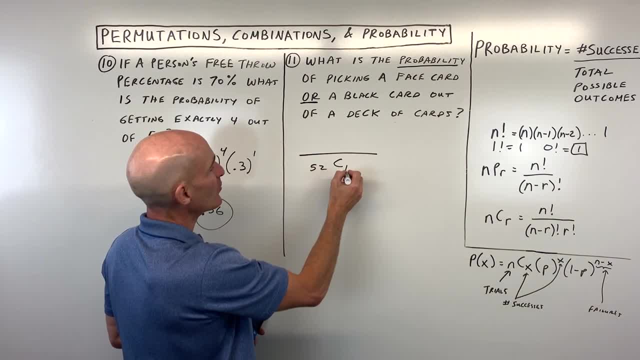 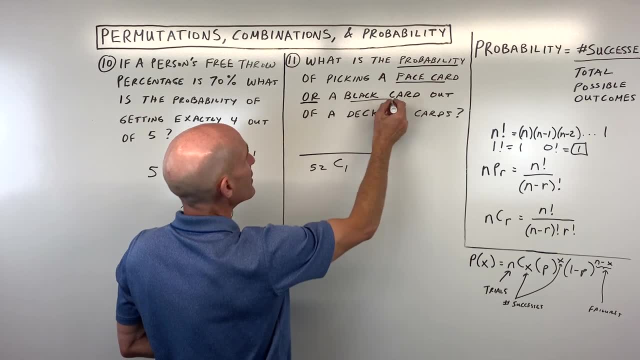 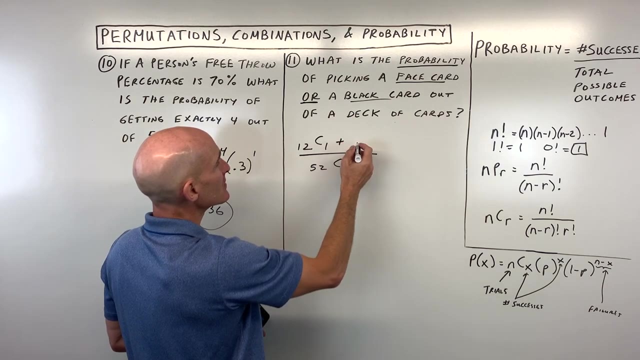 the total. So, out of the 52 cards total, we're saying: how many ways are there to choose one? Okay, but we're saying that it's a face card or a black card. Now there's 12 face cards. We say: how many ways are there to choose one face card plus how many black cards are there? 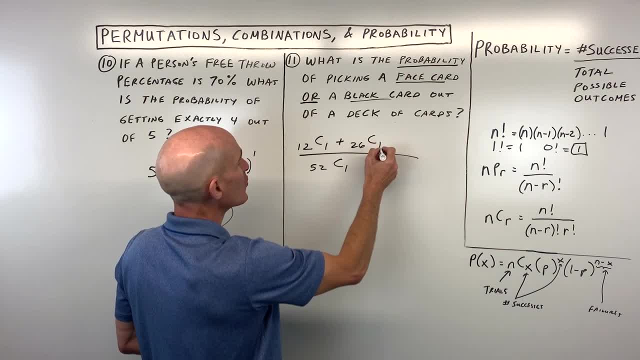 There's 26 black cards, because half are black, half are red. Choose one of those. but you see there's an overlap here. Some of the face cards are black, which means that we're going to have to subtract off the ones that were double counting, that we counted in this group and this 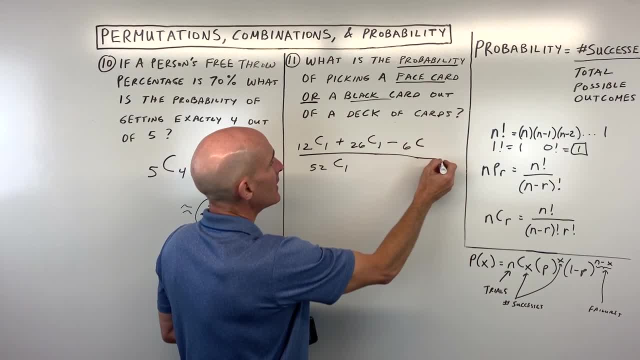 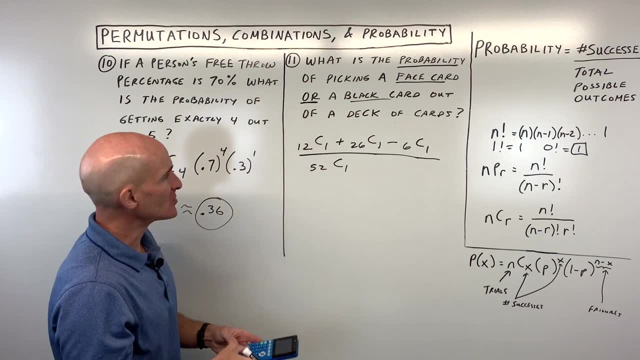 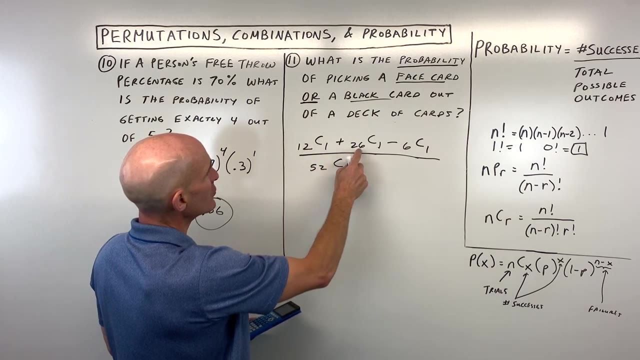 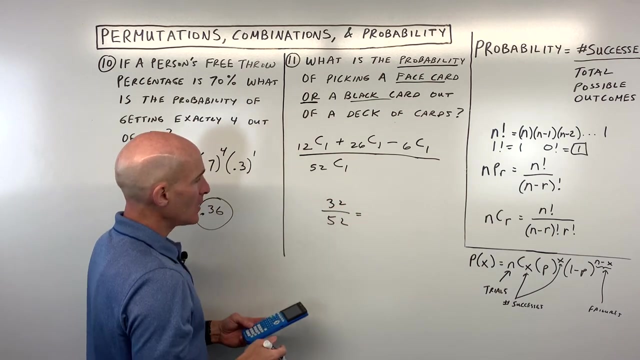 group, So that's going to be minus the six clubs and spades, face cards- Choose one. Okay, so let's see what this comes out to. So this would be: let's see: this is 12: choose one, which is 12, 26. choose 1 is 26,, so that's 38, minus 6. choose 1 is 6, so that's 32 over 52, which is. 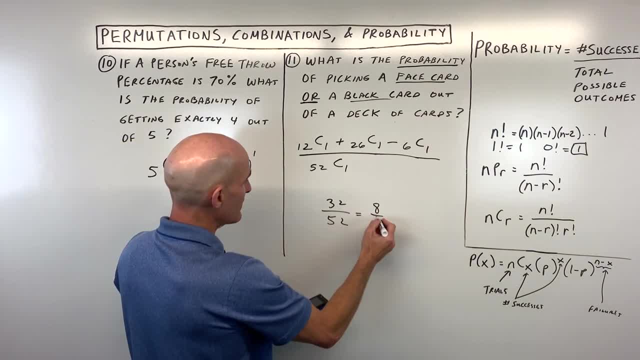 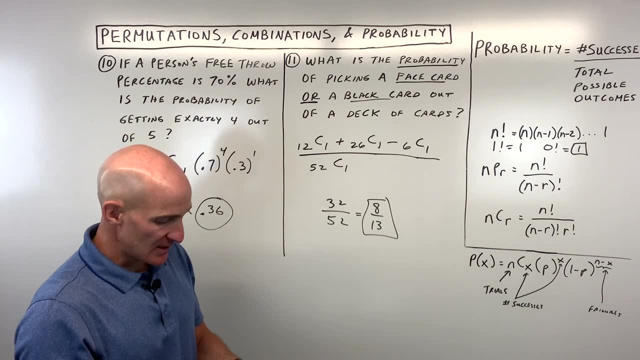 let's see if we reduce that down. 4 goes in here 8 times and 4 goes in here 13 times, So it'd be an 8 out of 13 probability which we can get. that as a decimal It's approximately 0.62.. 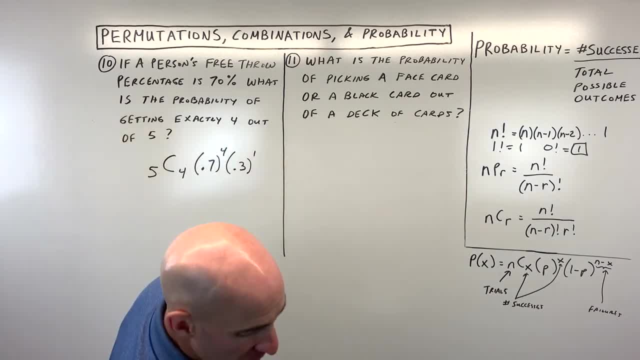 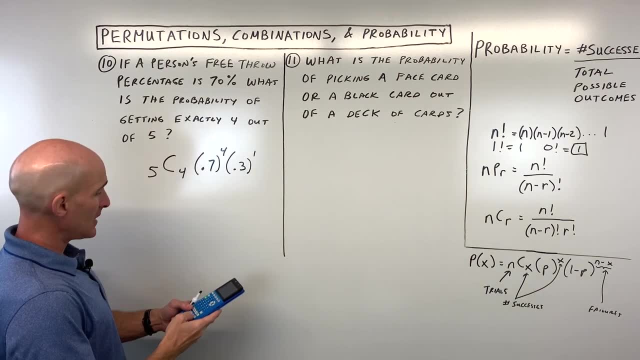 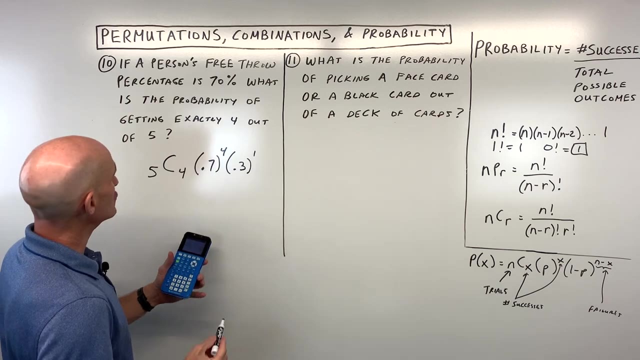 And we want one of those. So let's see what that comes out to. 5C4, okay times 0.7 to the fourth, times 0.3 to the first. Okay, so this is coming out to 0.3.. 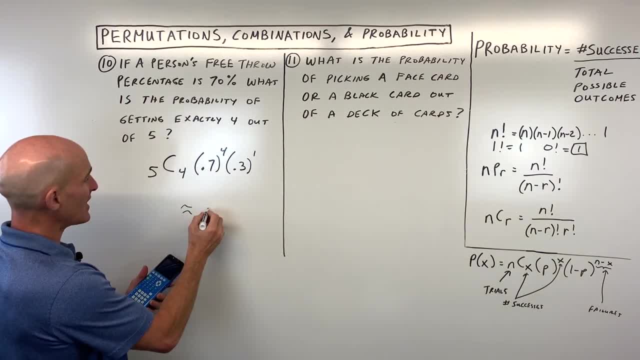 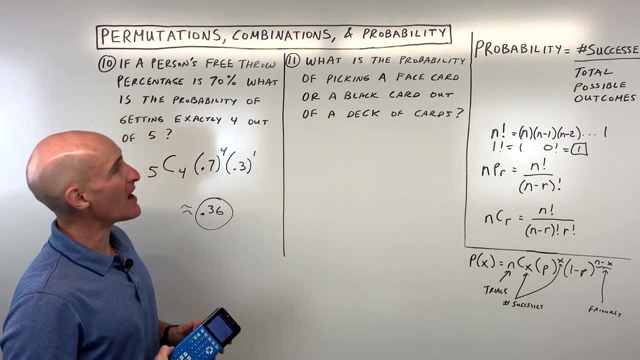 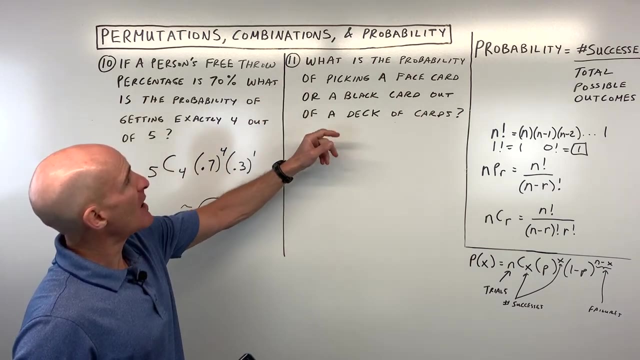 Approximately 36%, or we just say, as a probability, approximately 0.36.. So that's binomial probability when there's only two possible outcomes. Okay, now for number 11,. success or failure, right win or lose. For number 11,: what is the probability of picking a face card or a black card out of a deck of cards? 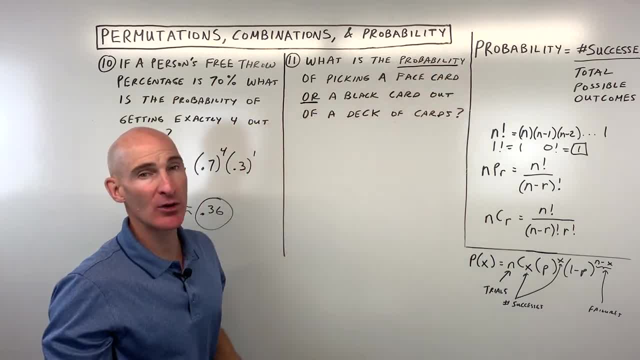 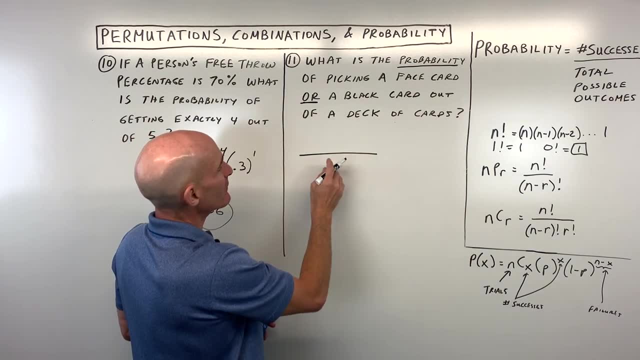 Now here we're talking about probability and we talked about the breakdown of face cards or not face cards, but a black card, A deck of cards, earlier. Remember, when it's probability, it's going to be a fraction out of the total. 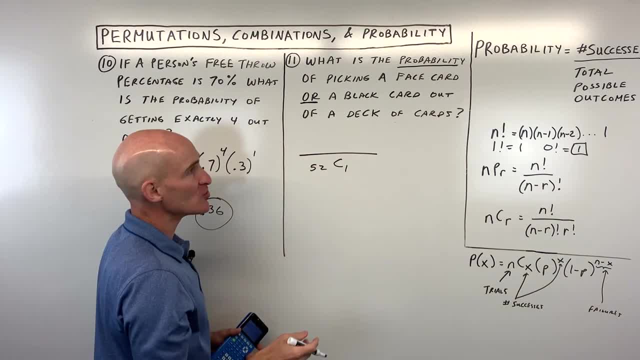 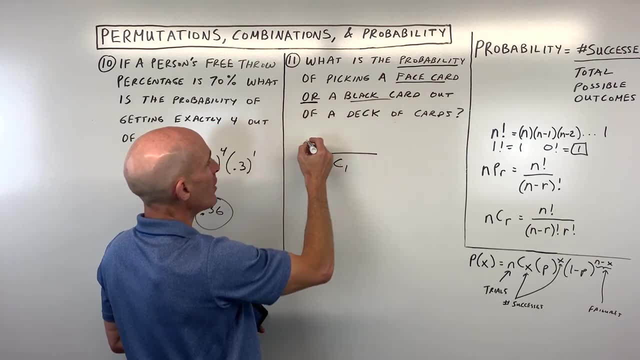 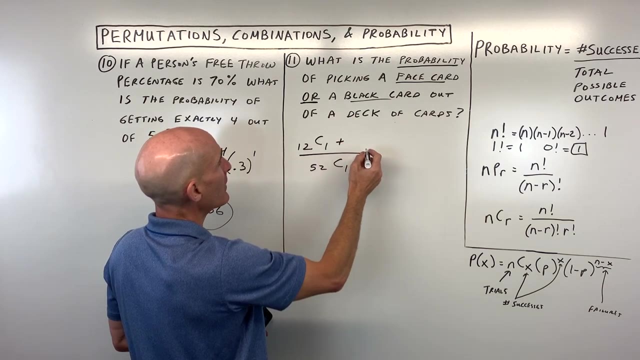 So, out of the 52 cards total, we're saying: how many ways are there to choose one? Okay, but we're saying that it's a face card or a black card. Now there's 12 face cards. We say: how many ways are there to choose one face card plus how many black cards are there? 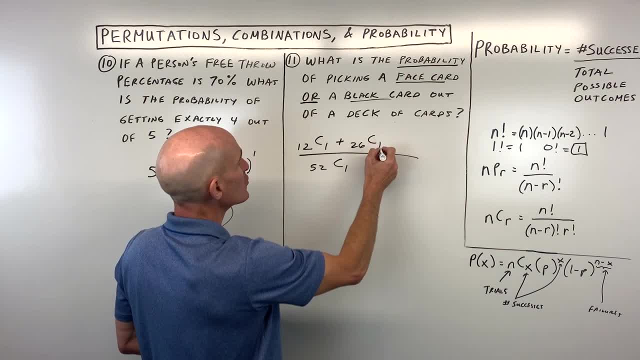 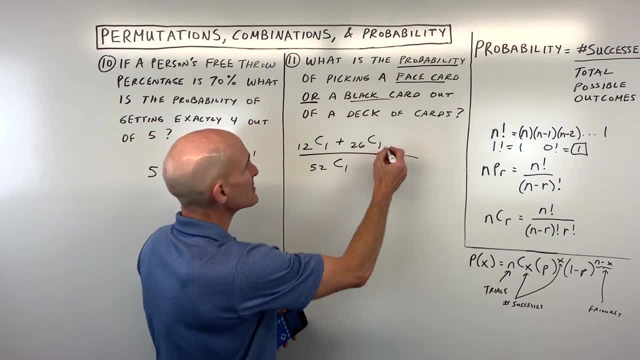 There's 26 black cards because half are black, half are red. Choose one of those. So you see there's an overlap here. Some of the face cards are black, which means that we're going to have to subtract off the ones that we're double counting. 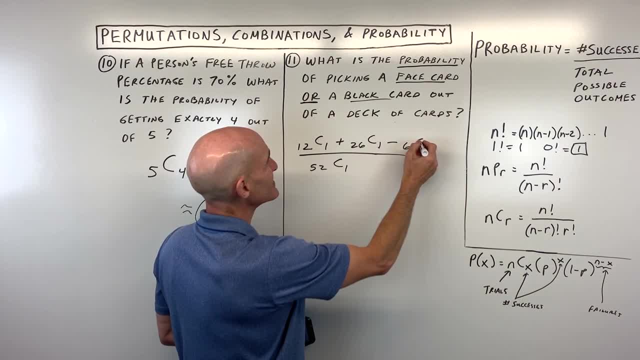 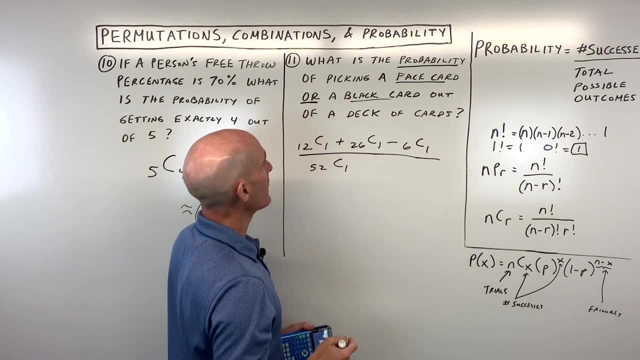 that we counted in this group and this group, So that's going to be minus the six clubs and spades. face cards: Choose one. Okay, so let's see what this comes out to. So this would be: let's see, this is 12. choose one which is a 12.. 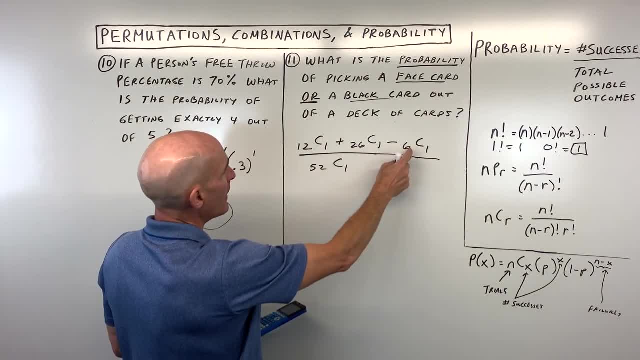 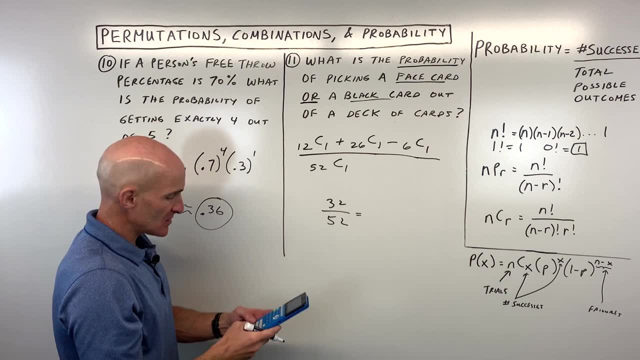 26: choose one is 26,, so that's 38.. Minus six: choose one, is six, so that's 32 over 52, which is- let's see if we reduce that down, Four goes in here eight times and four goes in here 13 times. 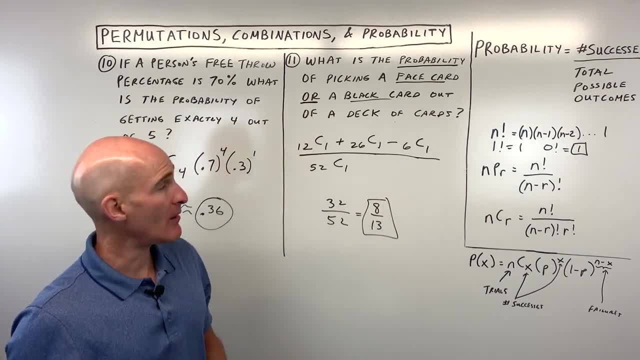 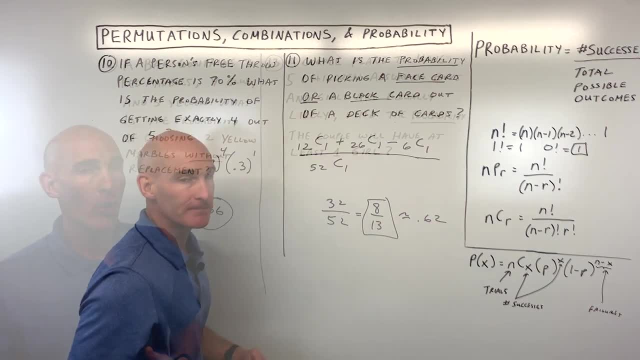 So it would be an eight out of 13 probability which we can get. that as a decimal It's approximately 0.62.. Okay, before we do these last four word problems, I wanted to let you know about an Algebra 1 and an Algebra 2.. 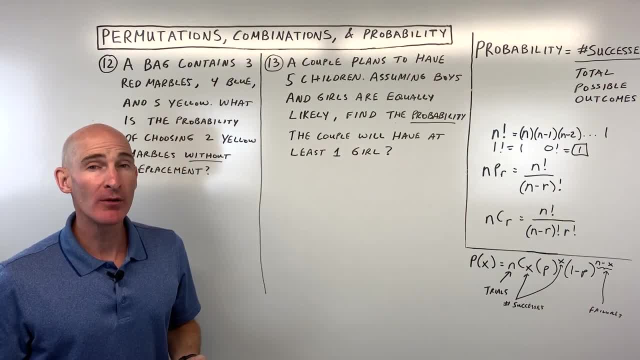 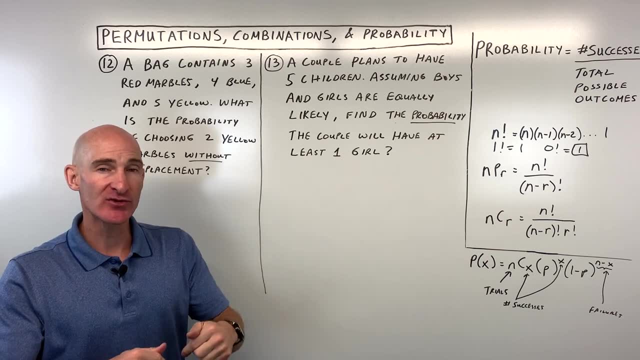 Okay, before we do these last four word problems, I wanted to let you know about an Algebra 1 and an Algebra 2 video course that I have for sale. You can check those out down in the description. Algebra 2 is also suitable for like a college algebra class, so check out those videos where 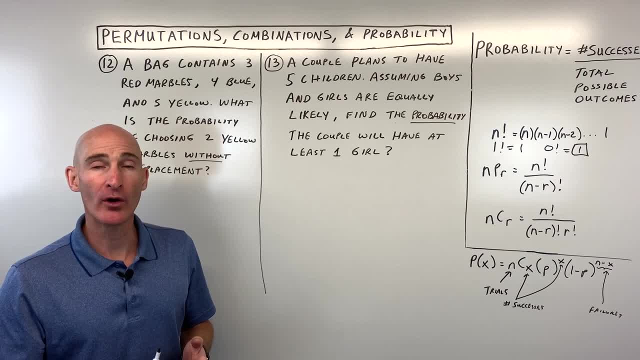 I take you step by step through a typical Algebra 1 or Algebra 2 curriculum And if you'd just like to support the videos that I'm putting up here on my Mario's Math Tutoring YouTube channel. you like the way I explain things and you want to help me to keep. 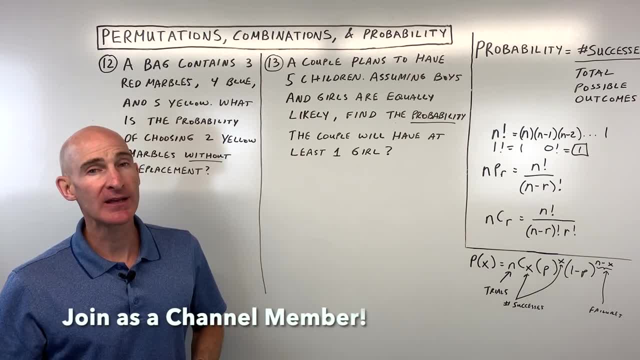 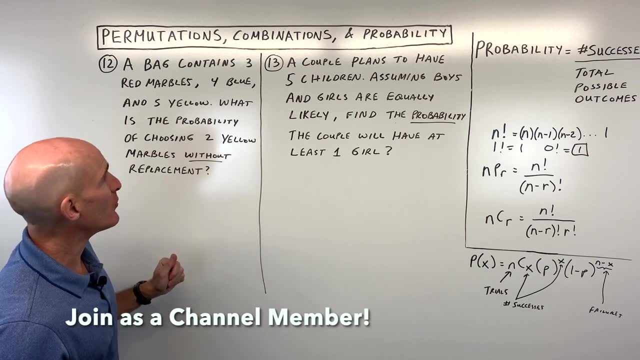 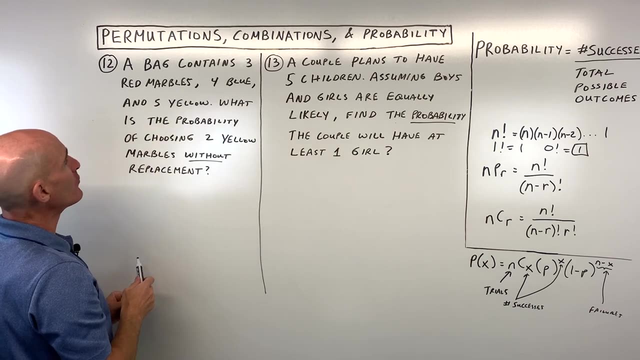 this going. consider supporting the channel as a channel member, So you can join the channel for a few dollars a month and I really appreciate that. Let's dive into the last few examples. So for number 12, it says: a bag contains three red marbles, four blue marbles and five yellow. 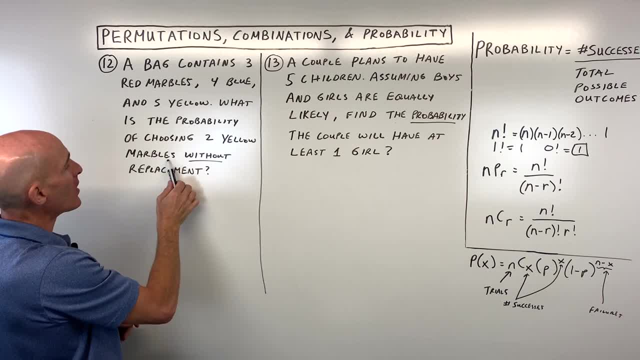 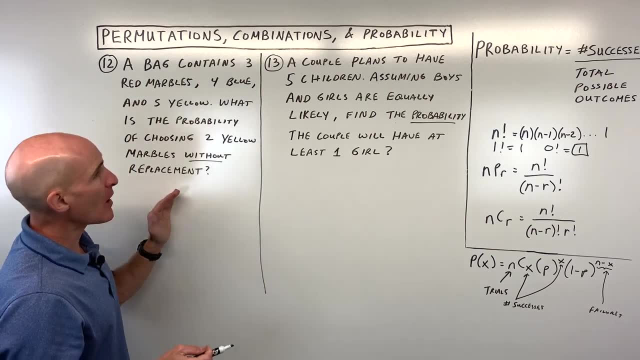 marbles. What is the probability of choosing two yellow marbles without replacement? So this is important, without replacement, And there's a couple different ways to do this problem. One way to do it: remember how we said, probability is well. 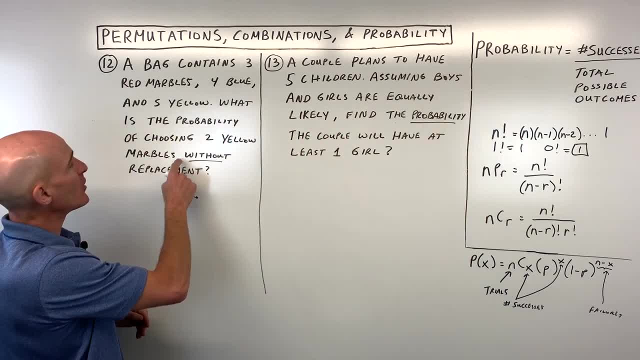 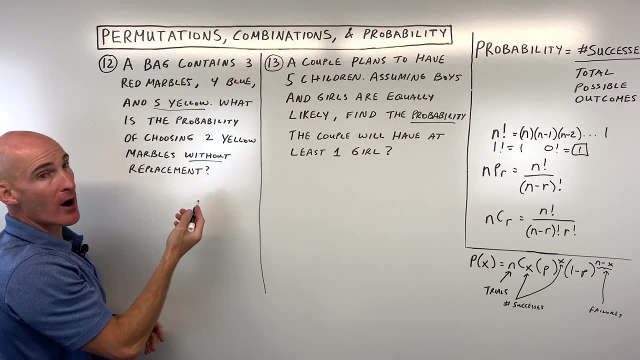 you want out of the total. In this case we want two yellow marbles. So when we reach into this bag, there's five yellow right And there's 12 total marbles. So the probability of getting a yellow would be five chances of success out of 12 possible marbles that you could pick Once you. 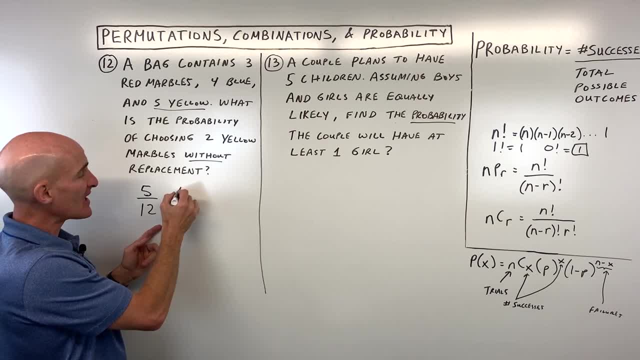 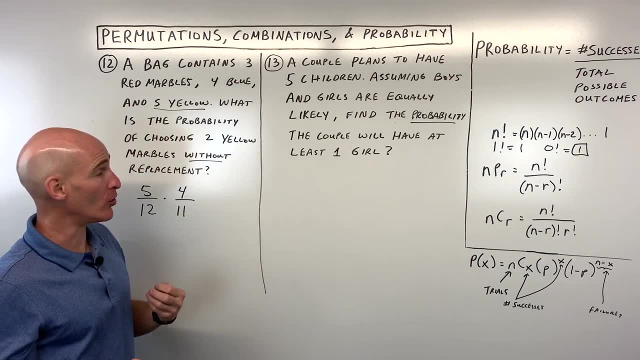 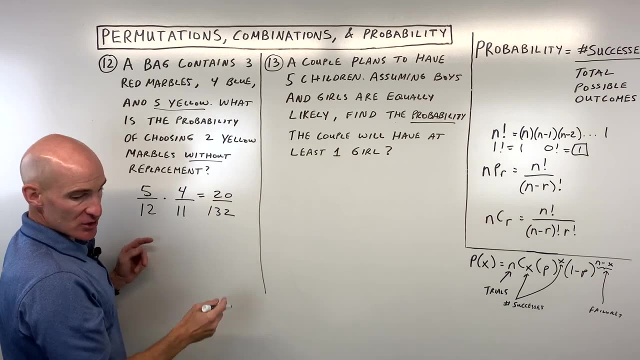 pick that first yellow marble. when you go to reach for the second yellow marble, there's only going to be four chances of success out of 11, because there's one less marble in the bag total. So when we multiply these together, you can see we're going to get 20 over 132, which we could reduce this down. Let's. 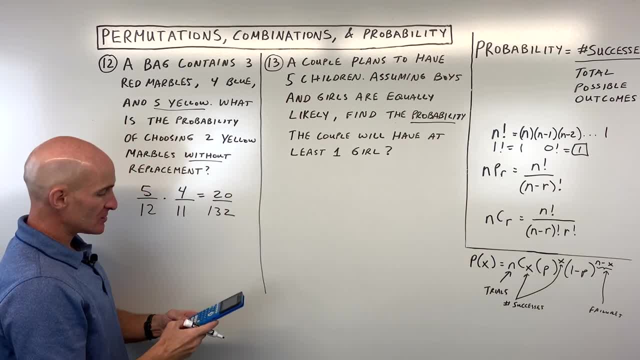 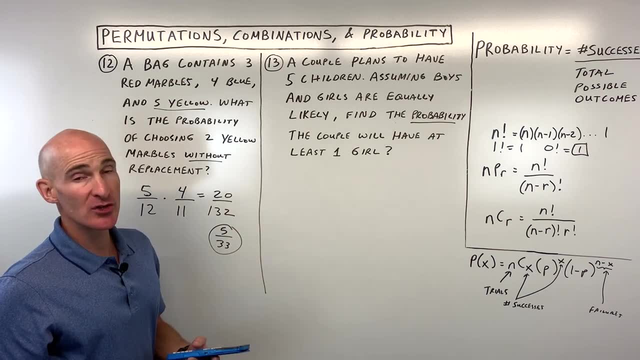 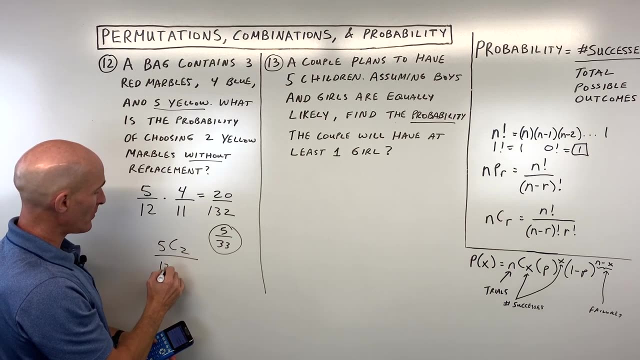 see what does that? reduce down to 530 thirds. Okay, the other way to do it is use the combinations. you could say: out of five, yellow, how many ways are there to choose two? and the total possible way of choosing two marbles out of 12, you're going to get the same answer: five out of 33.. 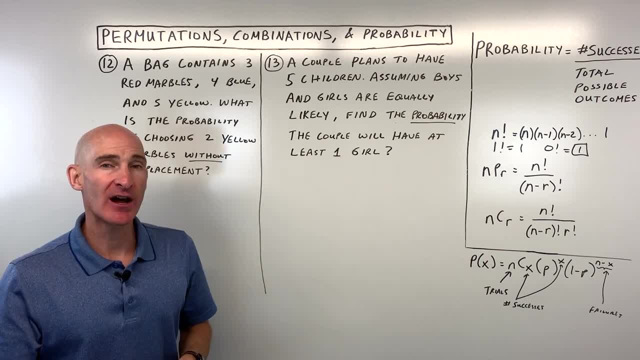 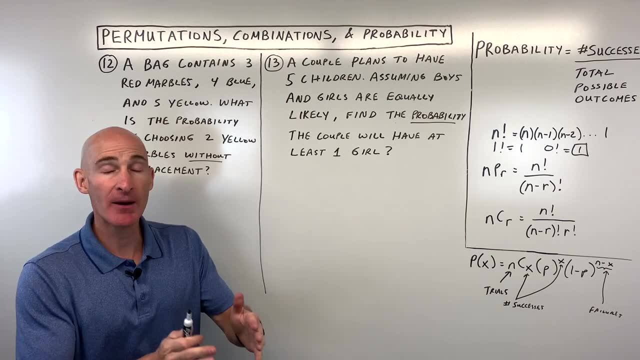 Video course that I have for sale. You can check those out down in the description. Algebra 2 is also suitable for like a college Algebra class, So check out those videos where I take you step by step through a typical Algebra 1 or Algebra 2 curriculum. 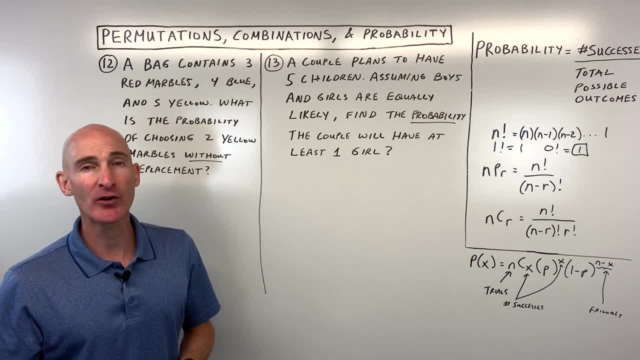 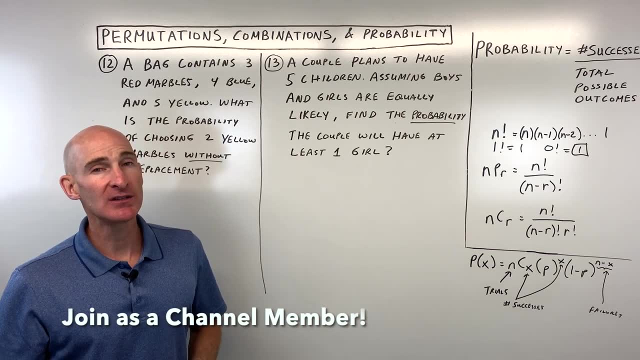 And if you'd just like to support the videos that I'm putting up here on my Myers Math Tutoring YouTube channel, you like the way I explain things and you want to help me to keep this going, consider supporting the channel as a channel member. 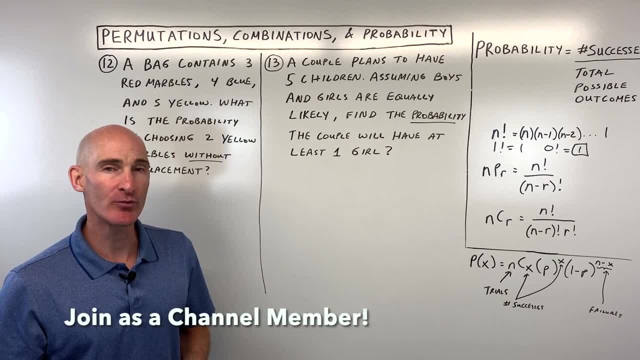 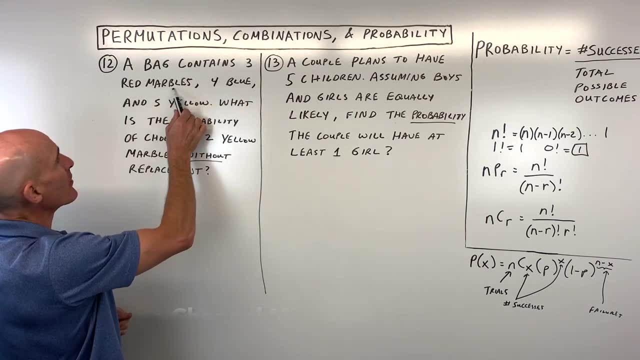 So you can join the channel for a few dollars a month and I really appreciate that. Let's dive into the last few examples. So for number 12, it says a bag contains three red marbles, four blue marbles and five yellow marbles. 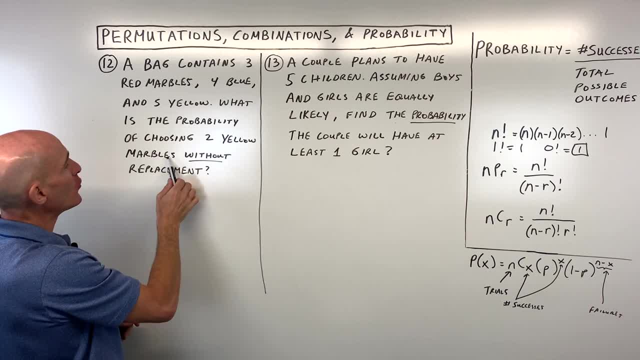 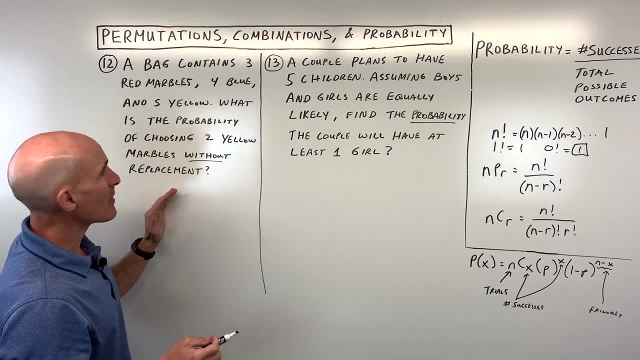 What is the probability of choosing two yellow marbles without replacement? So this is important without replacement, And there's a couple different ways to do this problem. One way to do it: remember how we said: probability is what you want out of the total. 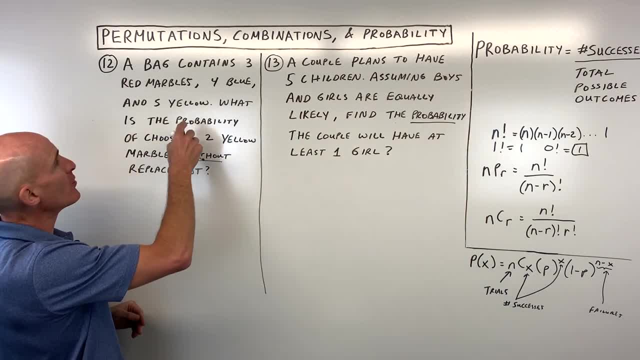 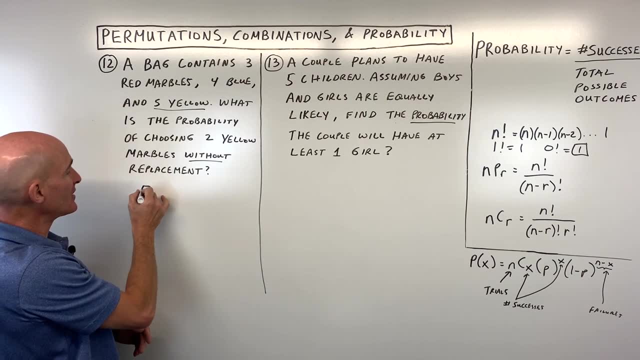 In this case we want two yellow marbles. So when we reach into this bag, there's five yellow right And there's 12 total marbles. So the probability of getting a yellow would be five chances of success out of 12 possible marbles that you could pick. 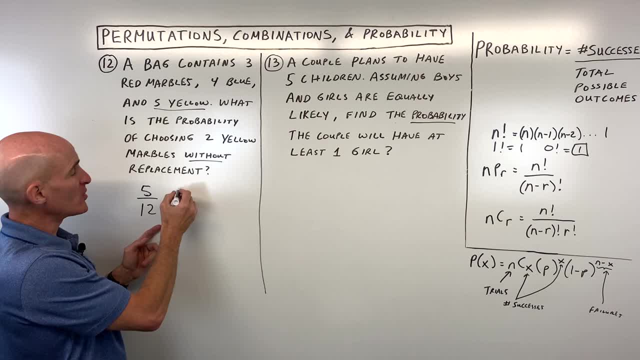 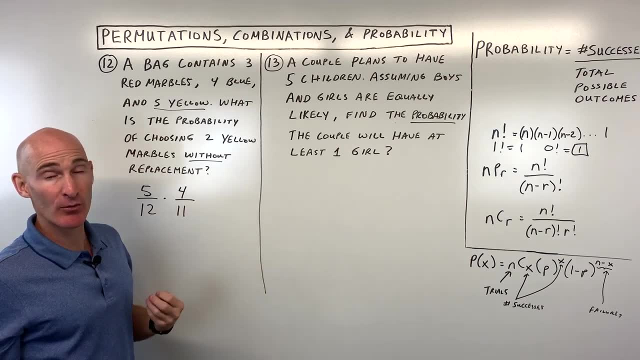 Once you pick that first yellow marble, when you go to reach for the second yellow marble, there's only going to be four chances of success out of 11, because there's one less marble in the bag total. So when we multiply these together you can see we're going to get 20 over 132,. 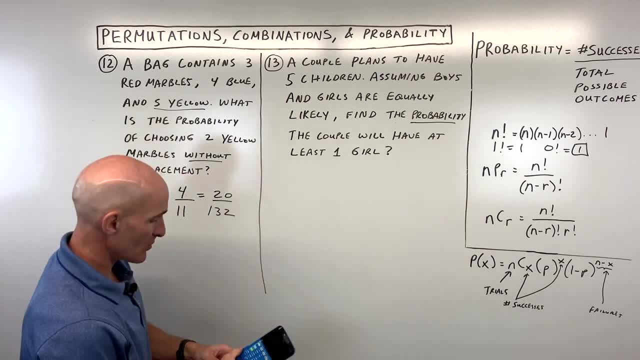 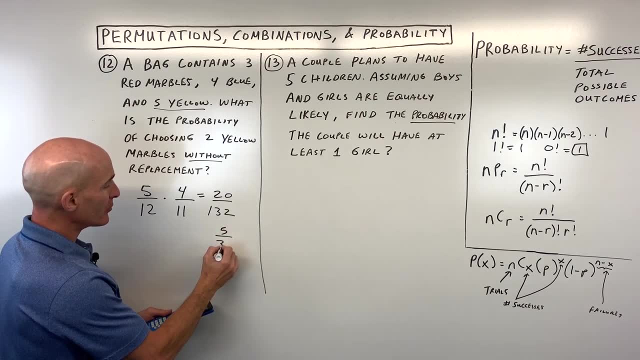 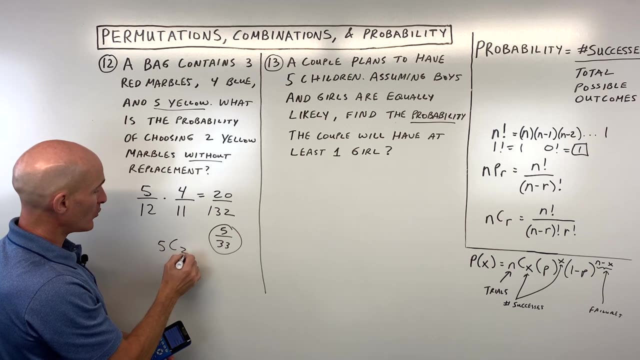 which we could reduce. Let's see, does that reduce down to five thirty-thirds? The other way to do it is to use the combinations. You could say: out of five yellow, how many ways are there to choose two? And the total possible way of choosing two marbles out of 12,? 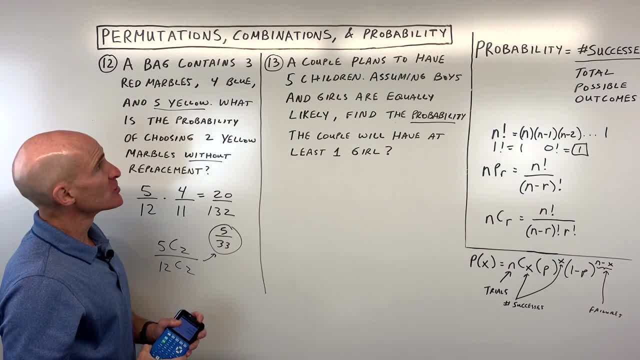 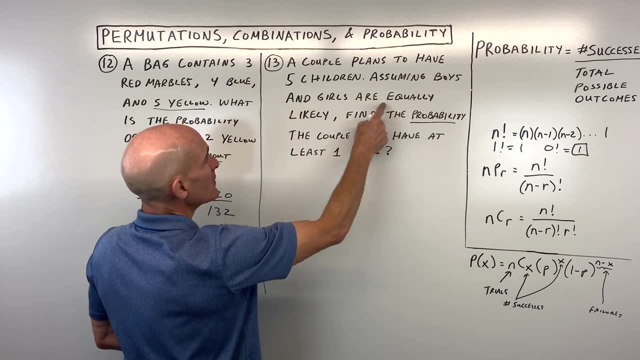 you're going to get the same answer: five out of 33.. So for number 13,, let's look at this one. A couple plans to have five children. Assuming that boys and girls are equally likely, find the probability that the couple will have at least one girl. 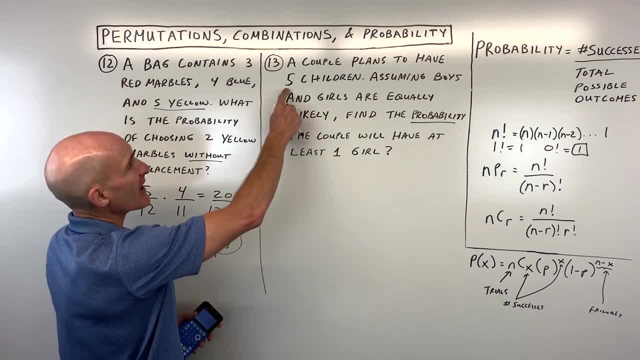 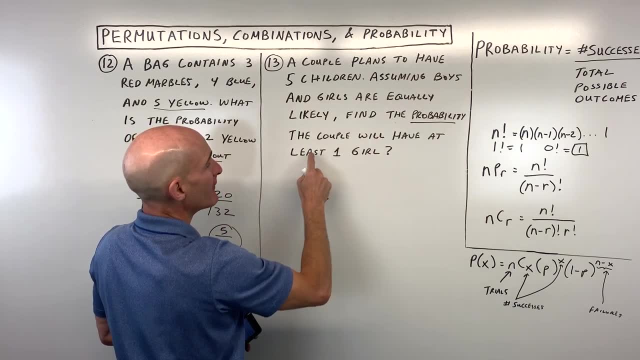 So for number 13,. let's look at this one. a couple plans to have five children, assuming that boys and girls are equally likely to get both of these marbles, Finding that probability that the couple will get at least one girl. so we've seen this a lot. 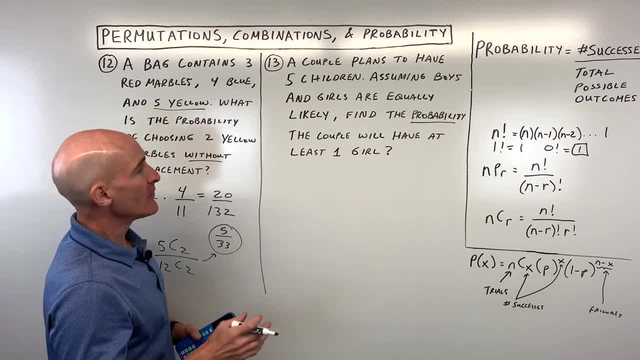 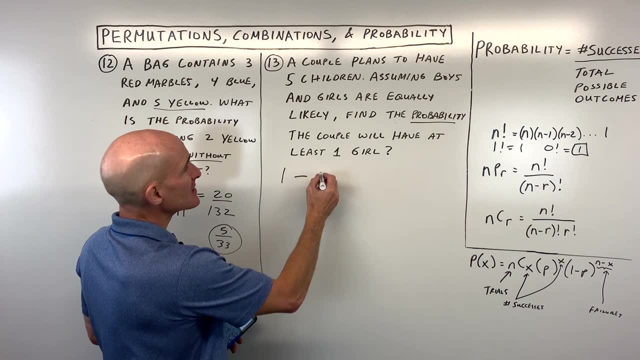 So we've seen this a lot. in this particular video at least, right. So at least when it comes out to probability. 100% is the total, which is like the number one minus the probability that they have no girls. 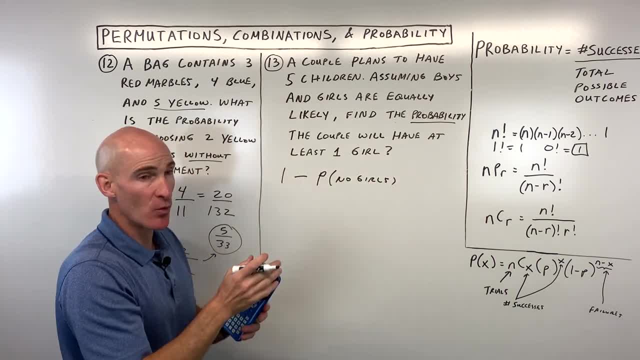 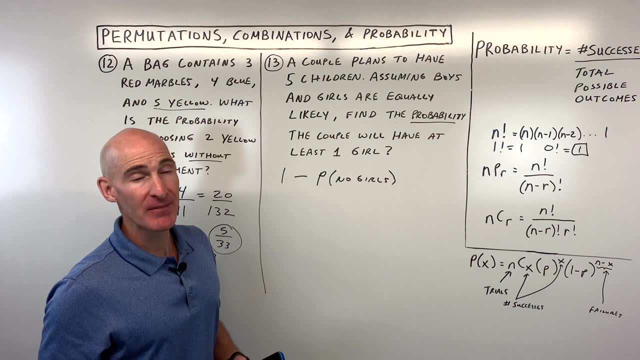 Okay, so one minus the probability of no girls means that it's one or more. So one, two, three, four or all five. Now, no girls is another way of saying. all boys, right, And what's the probability that the first one's a boy? 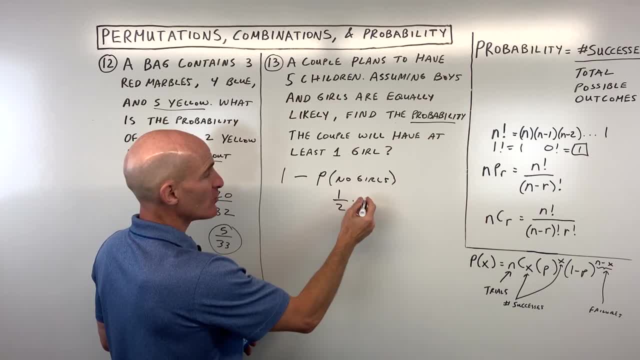 It's one chance out of two. What's the probability that the second one's a boy? One out of two, one out of two. one out of two, one half, one half, one half. So that's really one half to the fifth power, okay. 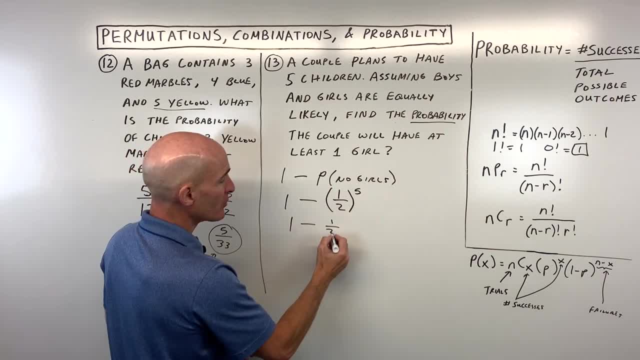 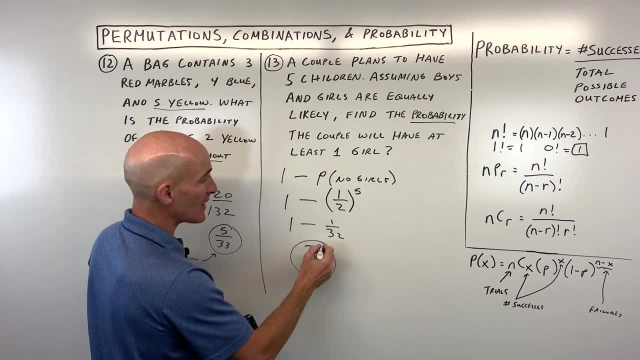 And we want one minus that. So one half to the fifth is one over 32.. One is like 32 over 32, minus one would be 31 over 32.. So that would be your probability of having at least one girl. 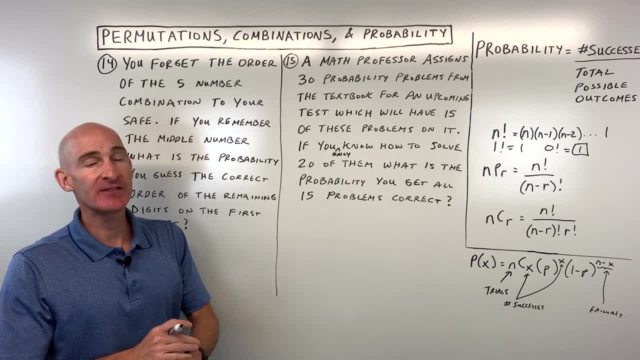 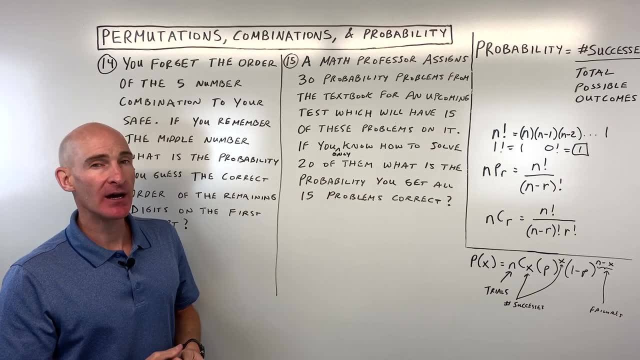 Okay, before we do these last two problems, I'll indicate at the end of this video another video that you can click on if you want more practice and more problems, to kind of work on a video that I did similar to this, different problems, obviously for more practice. 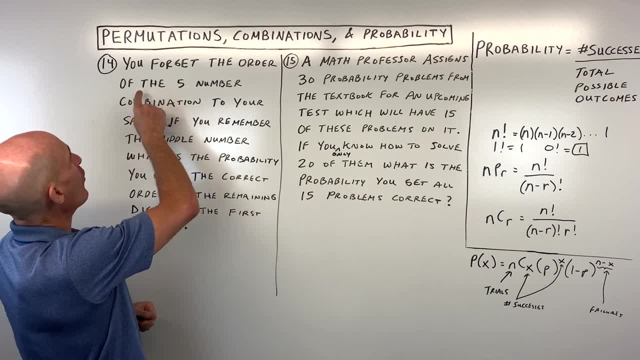 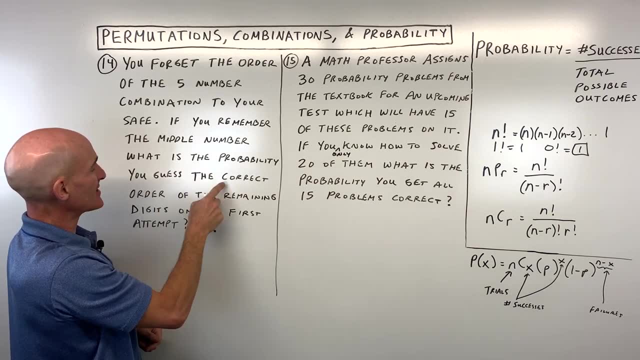 But let's do these last two problems. It says you forget the order of the five-number combination. to your safe, If you remember the middle number, what is the probability that you guessed the correct order of the remaining digits on the first attempt? Okay, that's interesting. 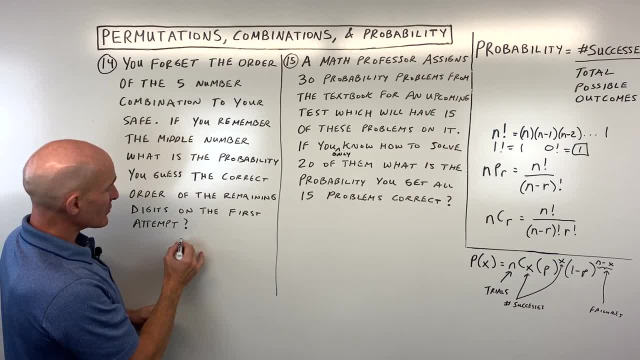 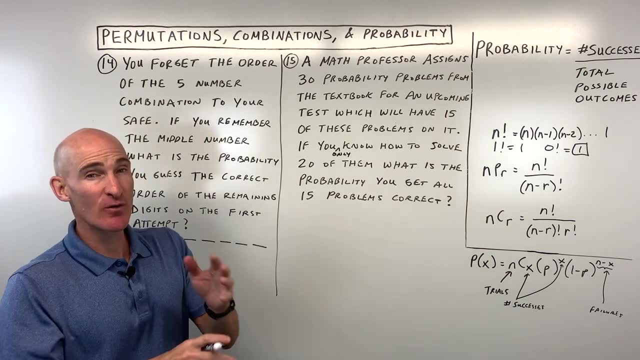 So what do you think for that one? Well, let's kind of diagram this out. So you've got one, two, three, four, five numbers. Now you know all five of the numbers, okay, It's just that you forgot the order of those five numbers. 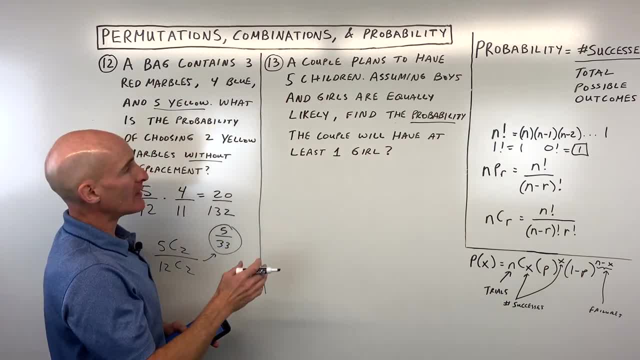 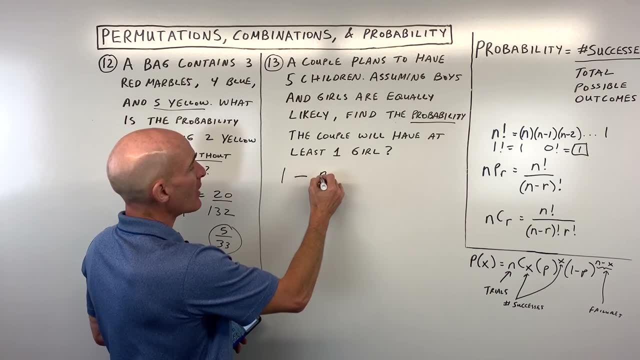 in this particular video at least right. So at least that this scale is equal. when it comes out to probability, 100% is the total, which is like the number one minus the probability that they have no girls available. okay, So one minus probably of no girls means it's one. 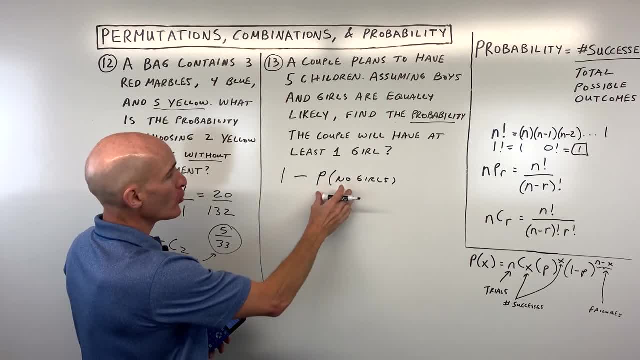 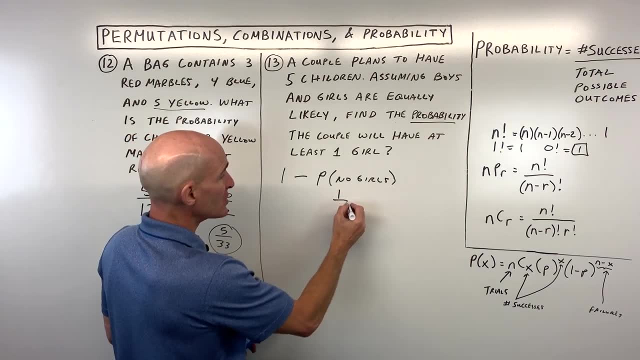 or more. So one, two, three, four or all five. Now, no girls is another way of saying. all boys right. And what's the probability? the first one's a boy, It's one chance out of two. And what's the? 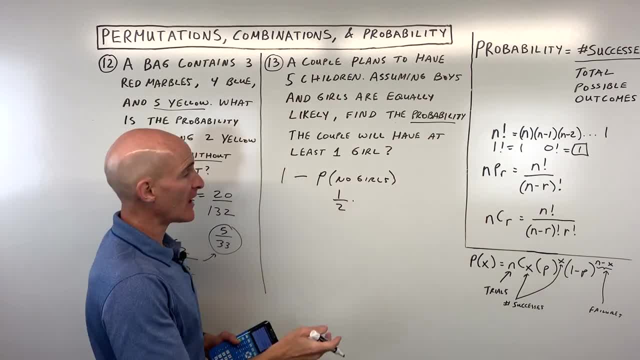 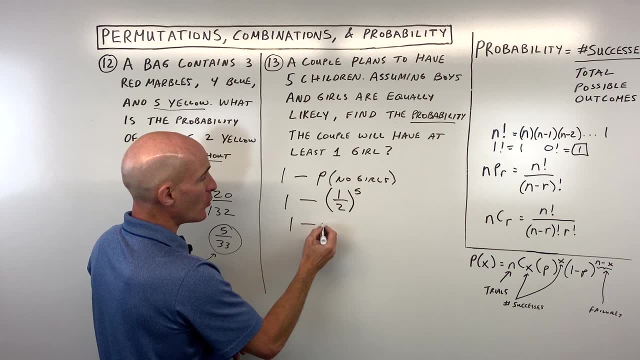 probability. the second one's a boy. One out of two. one out of two. one out of two, one half, one half, one half, So that's really one half to the fifth power. okay, And we want one minus that, So one. 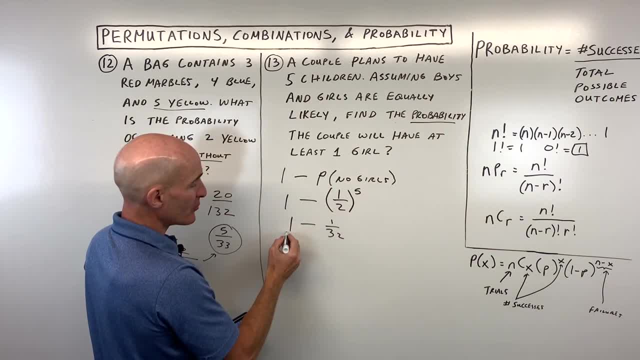 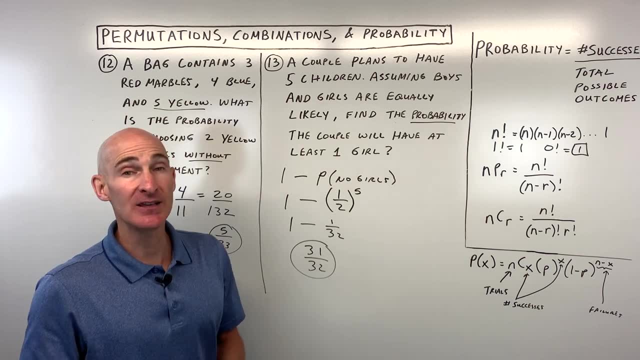 half to the fifth is one over 32.. One is like 32 over 32. minus one would be 31 over 32.. So that would be your probability of having at least one girl. Okay, before we do these last two problems, 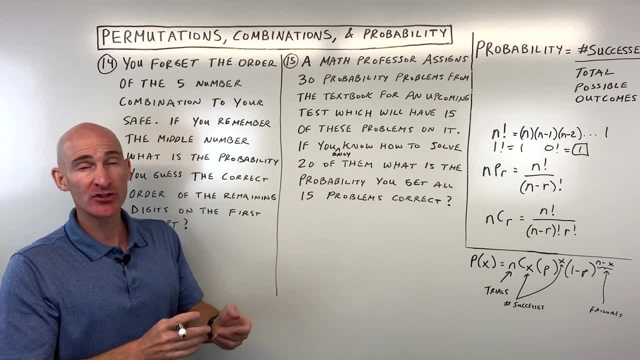 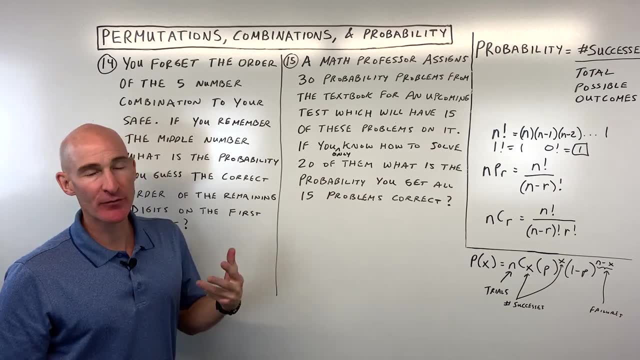 I'll indicate at the end of this video another video that you can click on if you want more practice and more problems, to kind of work on A video that I did similar to this: different problems, obviously for more practice, But let's do these last two problems. It says you. 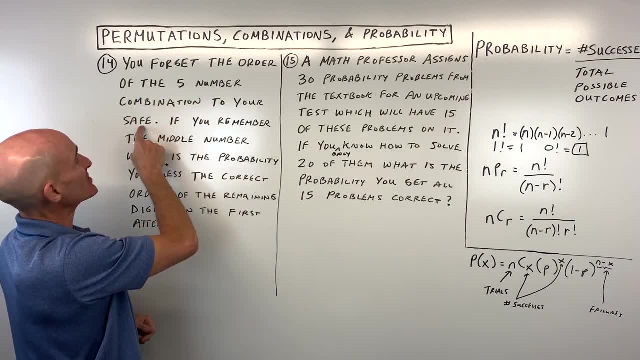 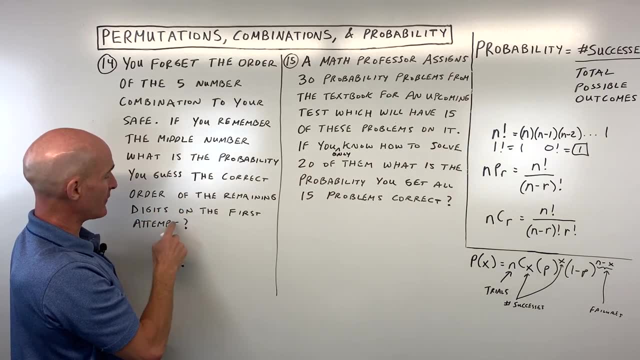 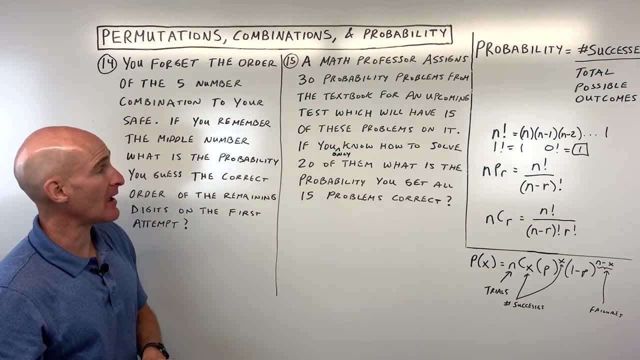 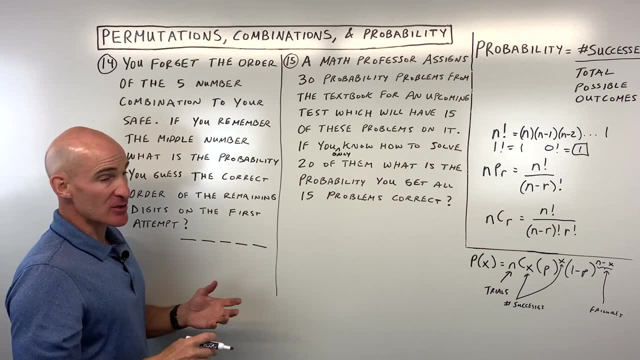 first attempt. Okay, that's interesting. So what do you think for that one? Well, let's kind of diagram this out. So you've got one, two, three, four, five numbers. Now you know all five of the numbers. okay, It's just that you forgot the order. 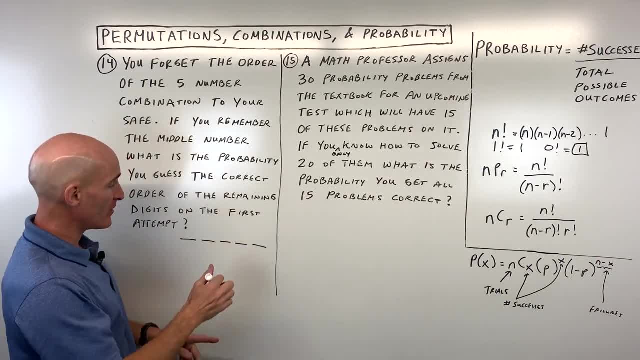 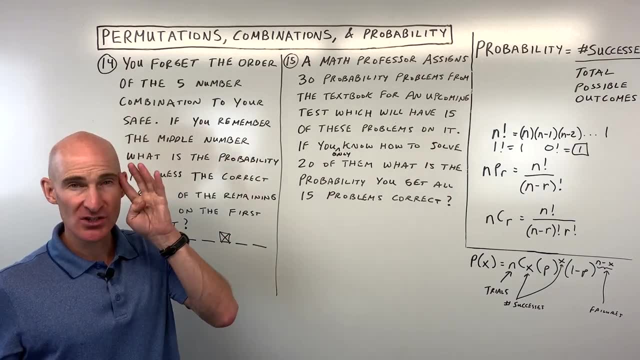 of those five numbers, But you do remember what the middle number is, So you know what. this guy is right here. So let's kind of X, that one off. So really, of these four digits that you have in your head, you just have to remember what order to put them in right. So how many different ways. 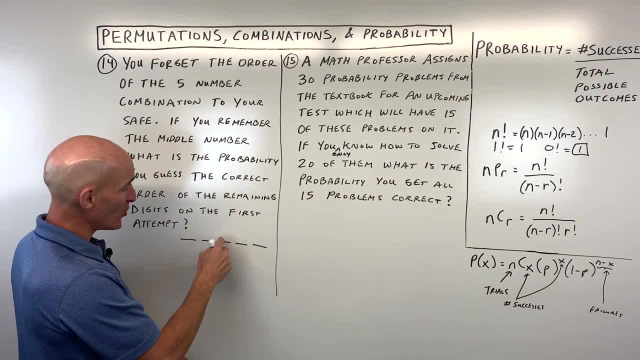 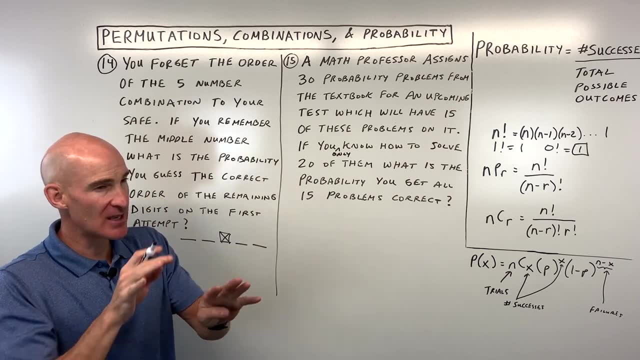 But you do remember what the middle number is, So you know what this guy is right here. So let's kind of X, that one off. So really, of these four digits that you have in your head, you just have to remember what order to put them in right. 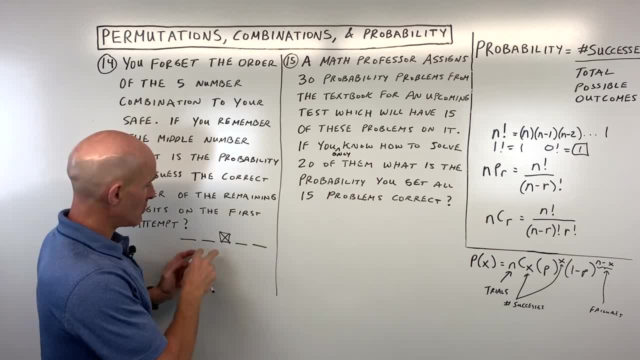 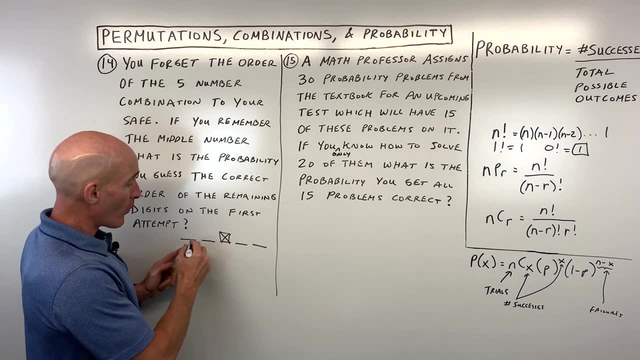 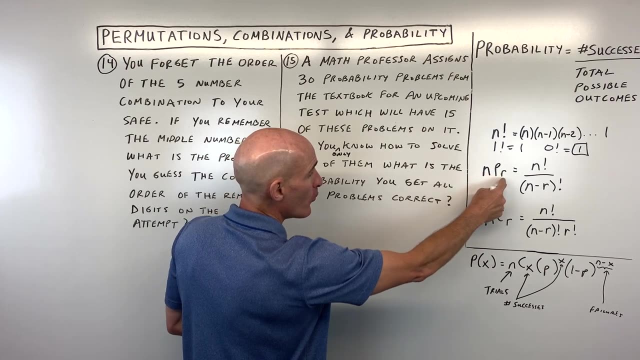 So how many different ways could you order these four remaining numbers? Okay, now the order is important, right? So we could do this as 4 factorial- See, that's the number of ways of ordering four items. We could also do 4p4.. 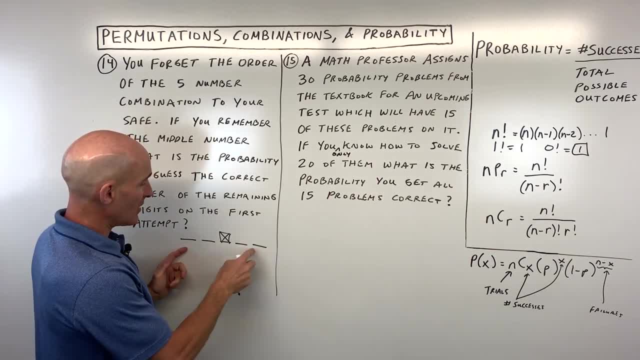 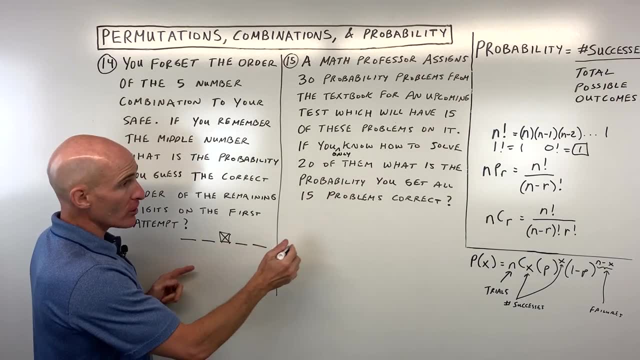 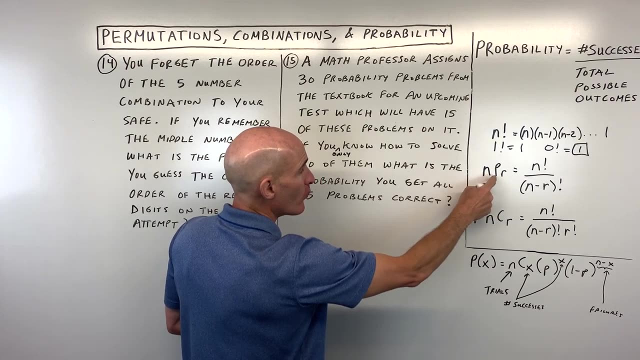 could you order these four remaining numbers? Okay, now the order is important, right? So we could do this as a four factorial. See, that's the number of ways of ordering four items. We could also do 4P4.. 4P4 is the same thing. 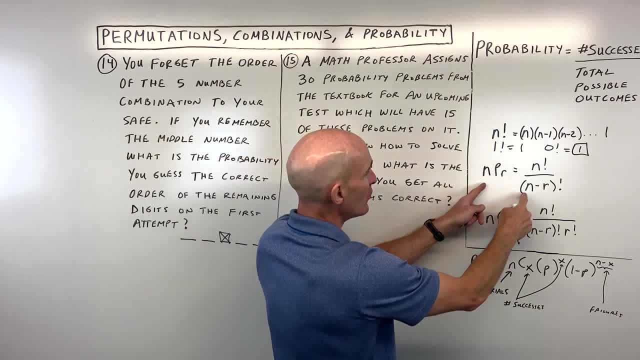 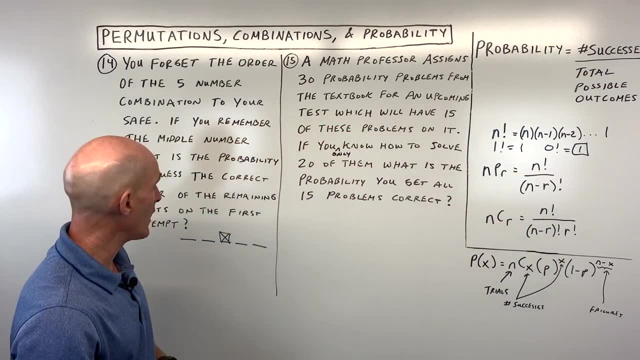 thing as four factorial, And the reason that is is because when you do four minus four, that's zero factorial, And zero factorial is one which is just going to give you the numerator n factorial or four factorial. Or you can use the fundamental counting principle. You can say: 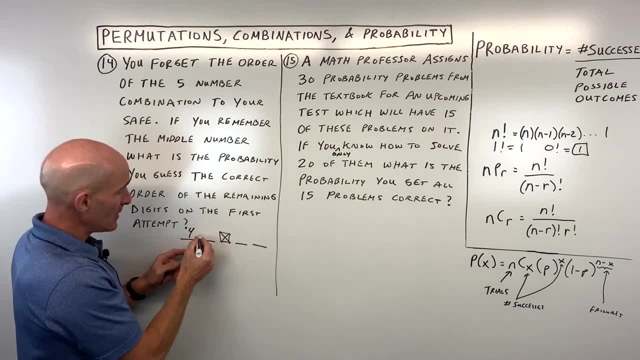 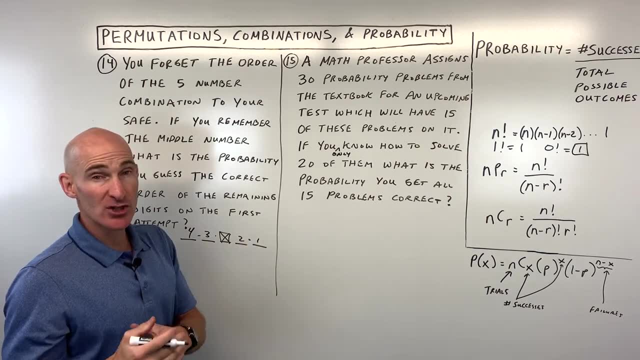 there's four choices, for which one I try for the first number, then three for that next number, two for this one and then one for this one. So that comes out to four times three times two times one, which is 24.. But only one of those is correct, right? So the probability when you think. 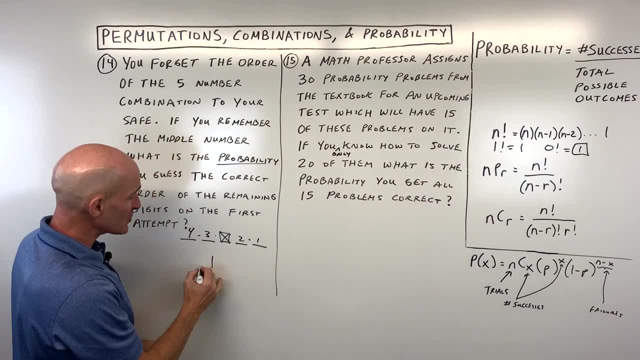 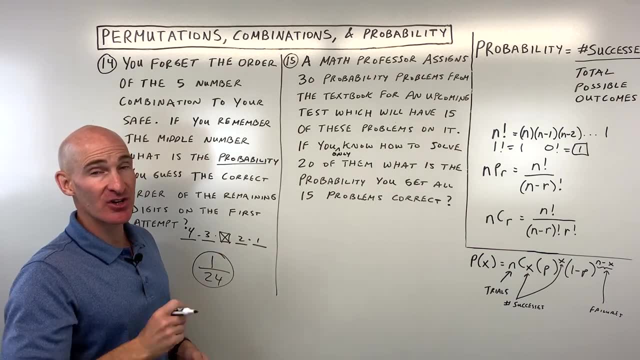 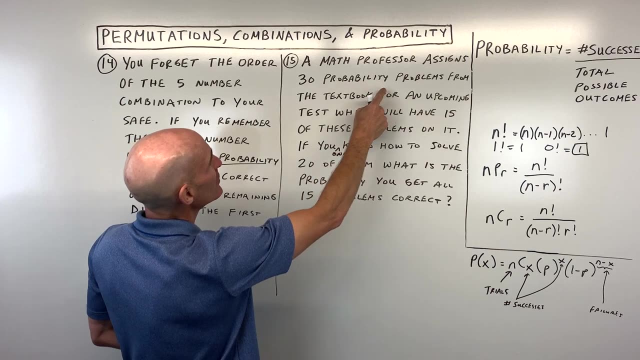 of the number of successful outcomes over the total possible. so this is going to be one over four, factorial, which is 24, so a 1, 24th chance it's going to work before the alarm goes off. right, Okay, so number 15.. A math professor assigns 30 probability problems from the textbook. 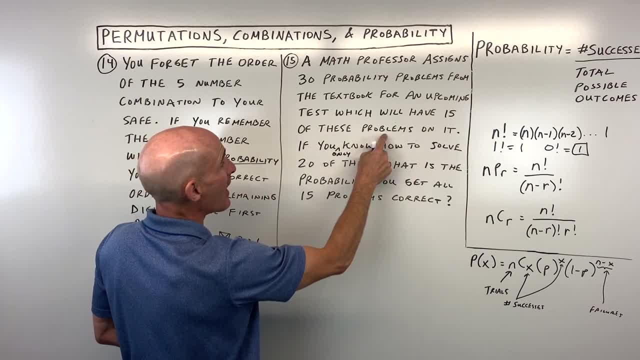 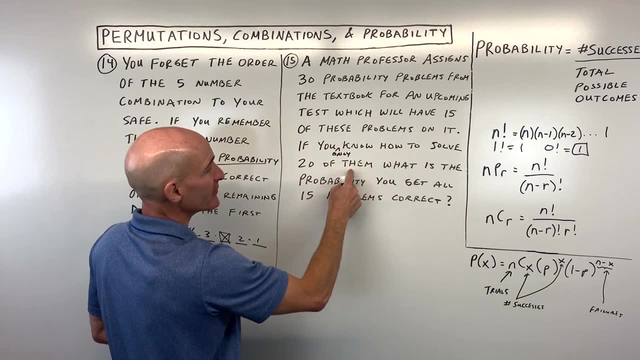 for an upcoming test which will have 15 of these problems on it. I should have written these exact problems on it. If you only know how to solve 20 of them, okay, 20 of the 30, what is the probability that you get all the 15 problems correct on this test? 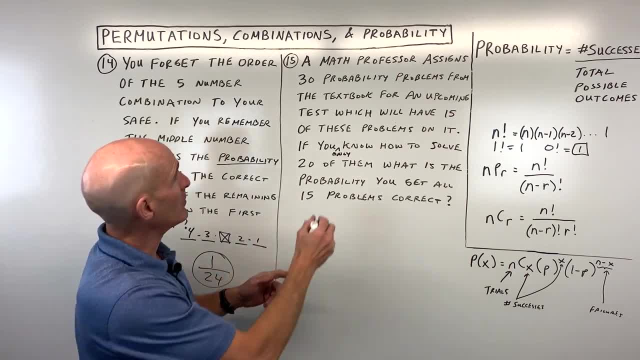 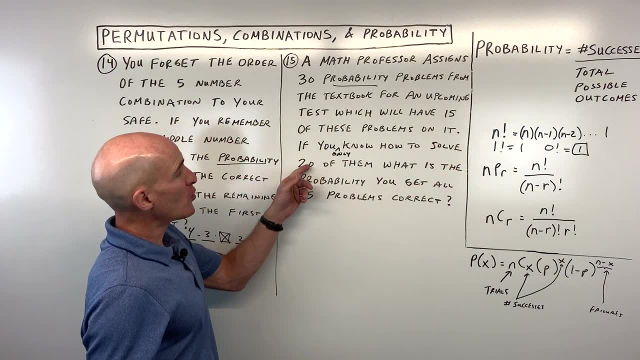 So what do you think about that one? So it's definitely a probability problem. So we want to think about this as number of successes over the total possible, And you know 20 of these problems right? So if you're teacher by some crazy chance, 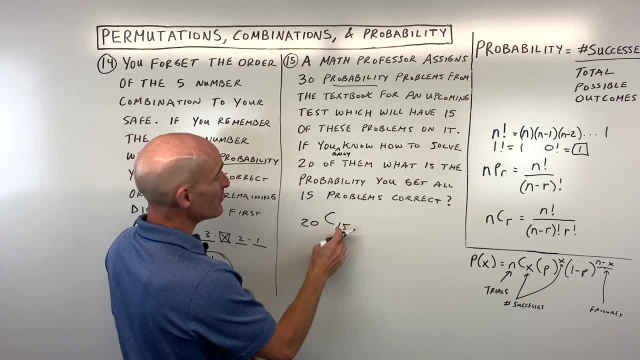 they give you 15 of those problems from the book out of the 20 that you do. So i'm going to get rid of for now. right, I missed one yet and I'm going to think I do. you know how many ways could that happen? right Again, the order doesn't matter. 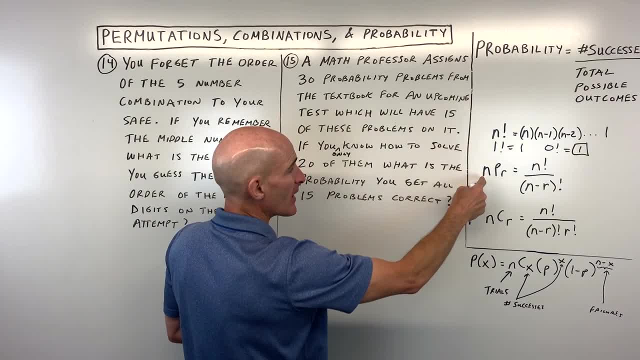 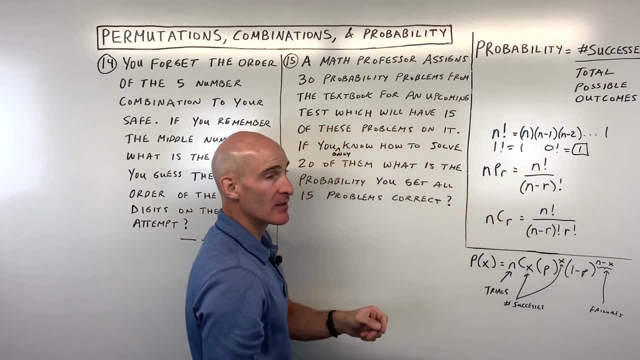 4p4 is the same thing as 4 factorial, And the reason that is is because when you do 4 minus 4, that's 0 factorial, and 0 factorial is 1, which is just going to give you the numerator. 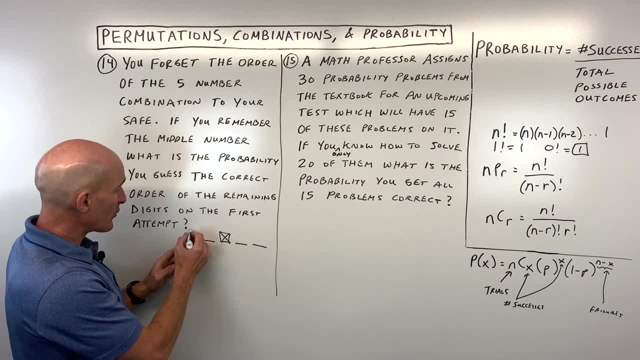 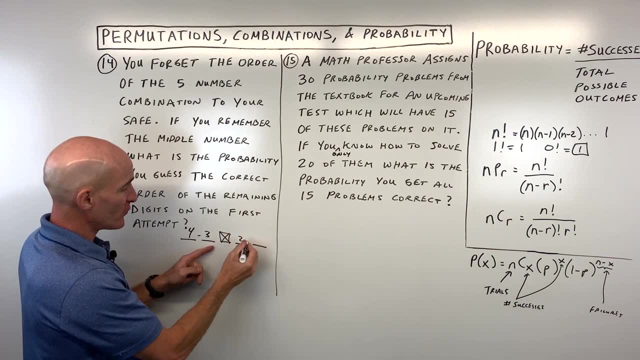 n factorial or 4 factorial, Or you can use the fundamental counting principle. You can say: there's four choices, for which one I try. for the first number, then three for that next number, two for this one and then one for this one. 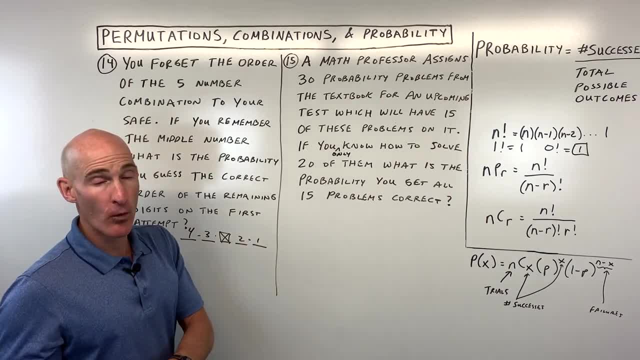 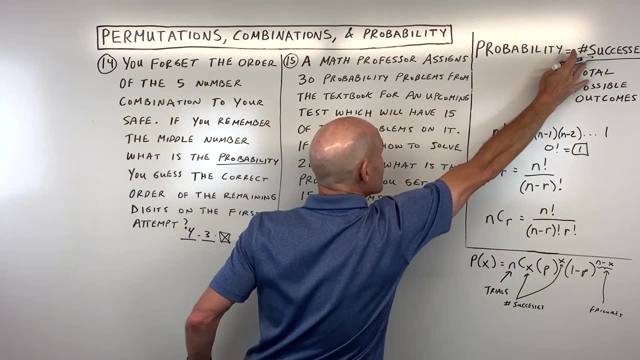 So that comes out to 4 times 3 times 2 times 1, which is 24.. But only one of those is correct, right? So the probability, when you think of probability, it's the number of successful outcomes over the total possible. 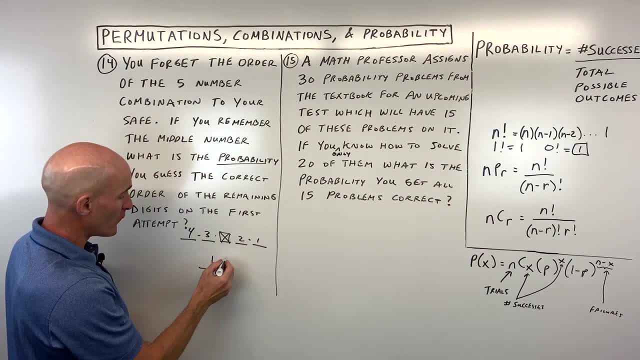 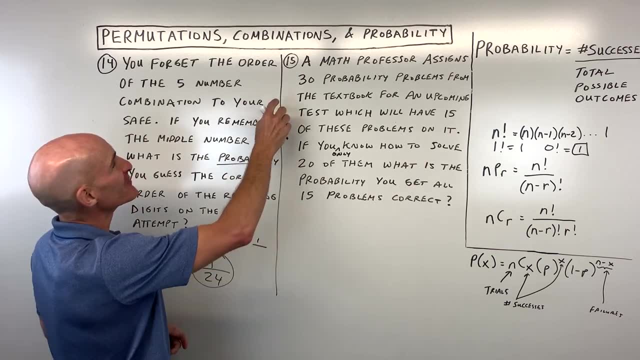 So this is going to be 1 over 4 factorial, which is 24, so a 1 24th chance It's going to work before the alarm goes off. right, Okay, so number 15.. A math professor assigns 30 probability problems. 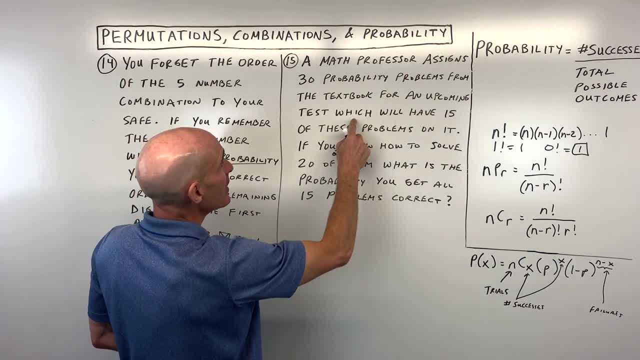 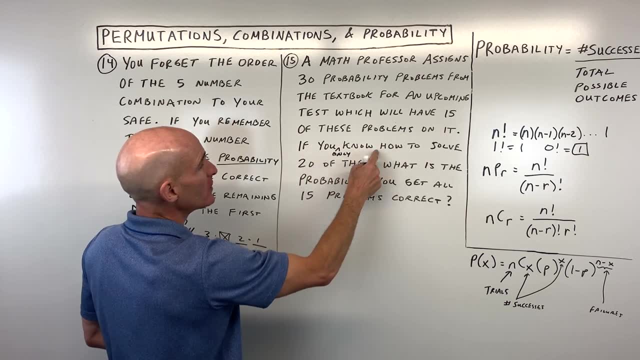 from the textbook for an upcoming test which will have 15 of these problems on it. I should have written these exact problems on it. If you only know how to solve 20 of them, okay, 20 of the 30, what is the probability that you get? 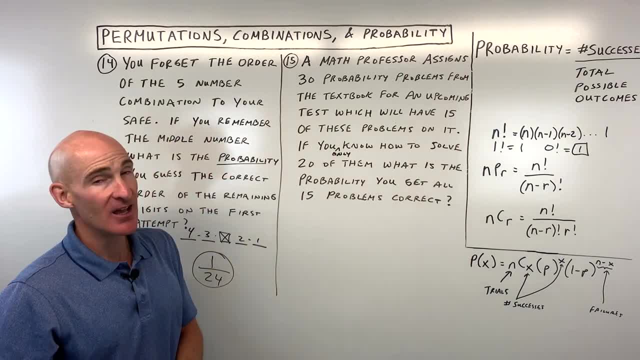 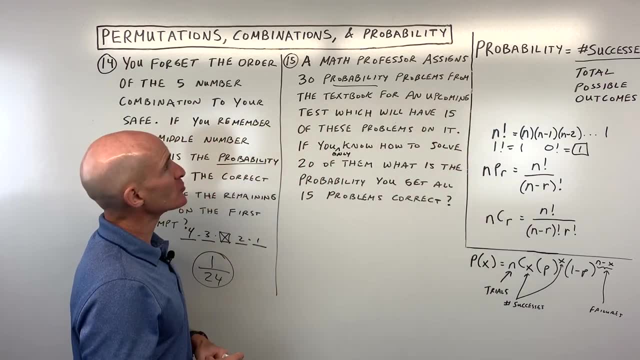 all the 15 problems correct on this test. So what do you think about that one? It's definitely a probability problem, So we want to think about this as number of successes over the total possible, And you know 20 of these problems right. 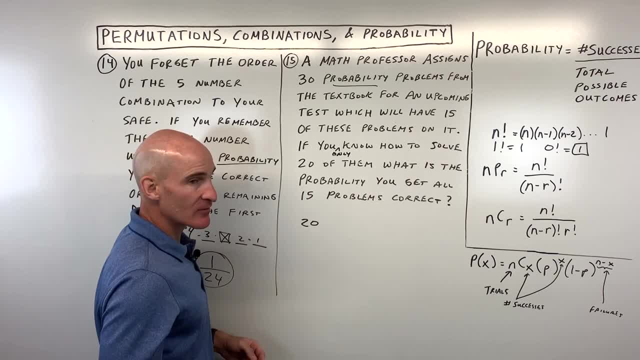 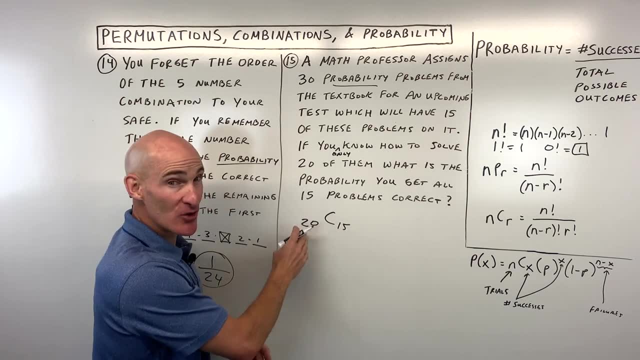 So if your teacher, by some crazy chance, they give you 15 of those problems from the book out of the 20 that you know, how many ways could that happen? right Again, the order doesn't matter, They're just going to be on the same test. 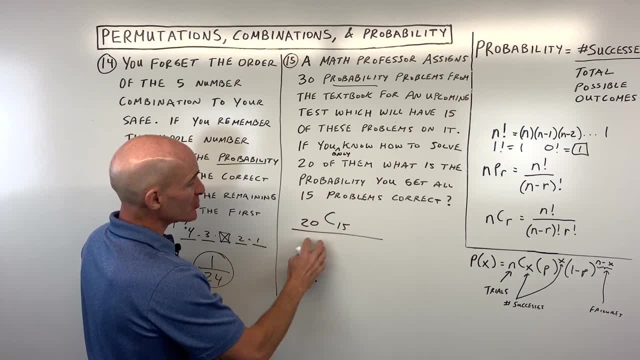 It doesn't matter what order they're in, So that's why we're using combinations, But the total ways that a professor, a math professor, could choose 15 problems out of 30, how many ways could that occur? So these are the number of successes. 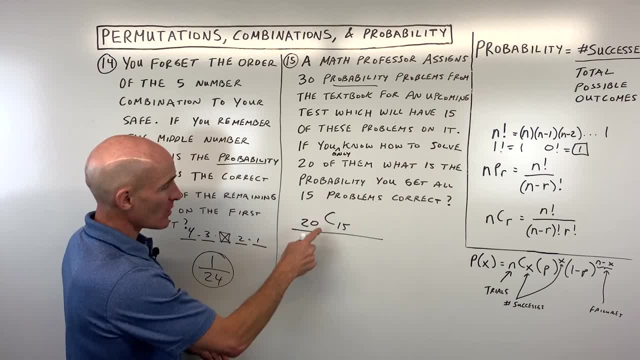 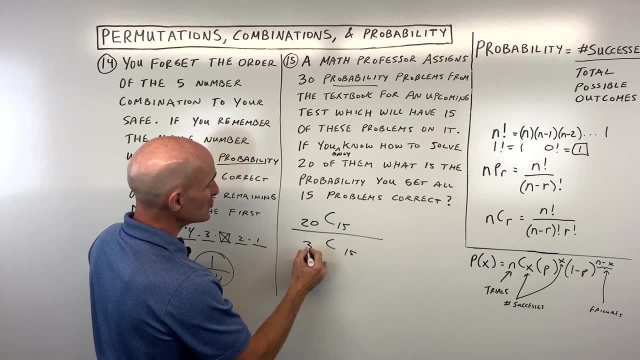 They're just going to be on the same test. It doesn't matter what order they're in. So that's why we're using combinations. But the total ways that a professor, a math professor- could choose 15 problems out of 30, how many ways could that occur? So?